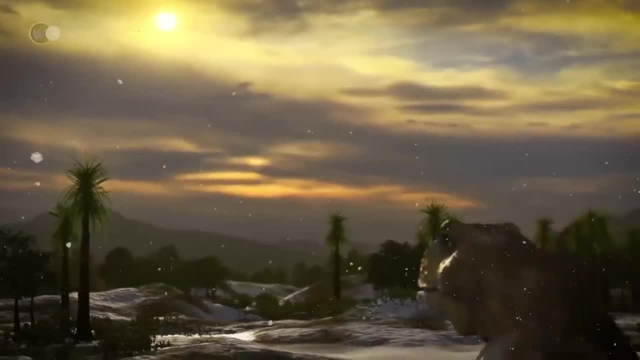 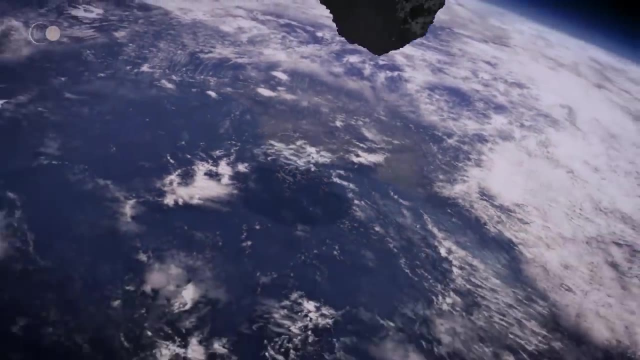 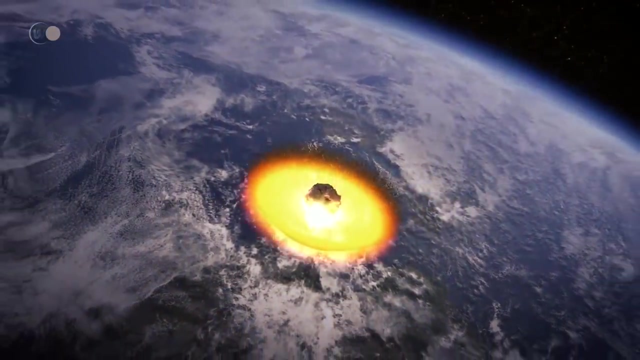 The Earth has, on five occasions, been confronted with great upheavals that have had a fundamental impact on its subsequent history. When they disappeared during the fifth mass extinction, the non-avian dinosaurs left an immeasurable void. But one man's loss is another man's gain. 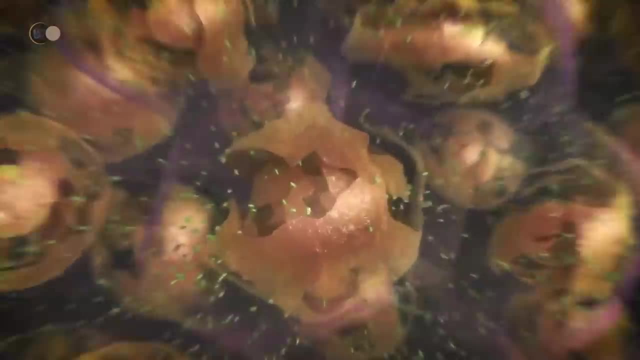 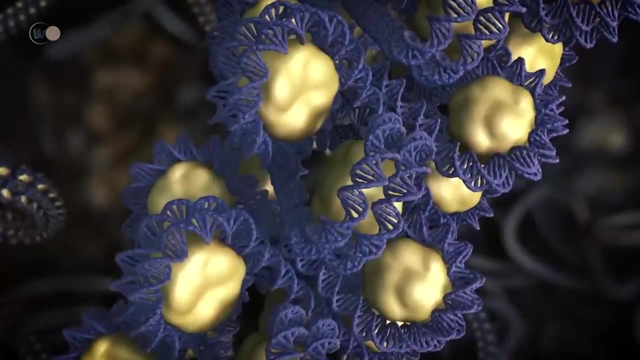 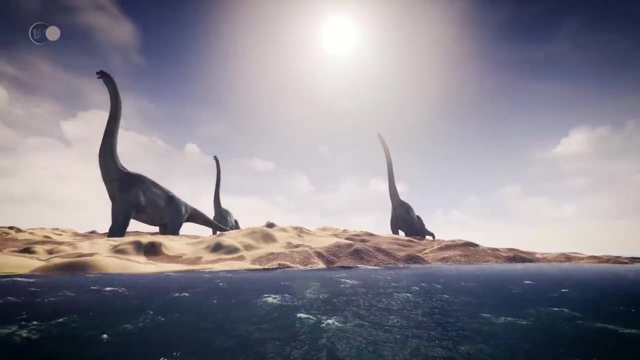 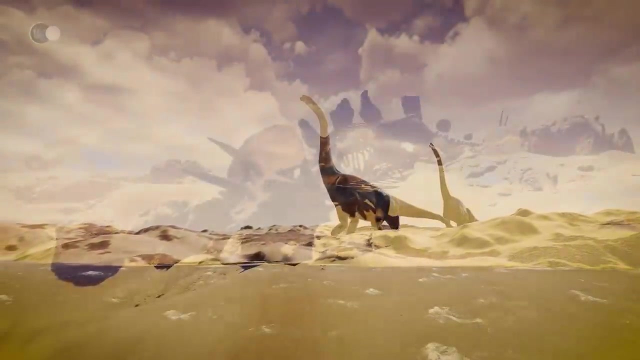 and this void allowed the evolution of mammals and birds, which are now highly diverse groups of animals. Without this extinction, dinosaurs would probably have continued to dominate life on Earth and other animals would not have had the opportunity to make their way. Mass extinctions change the rules of the game and reshuffle the deck. 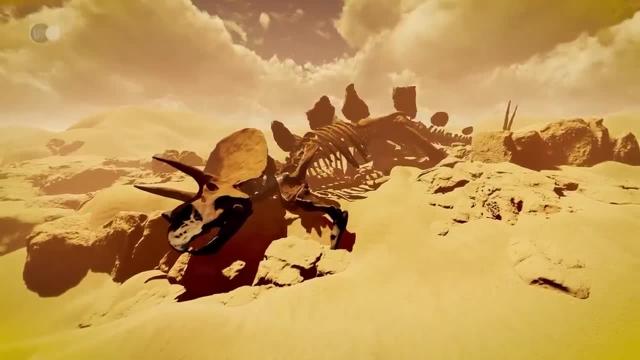 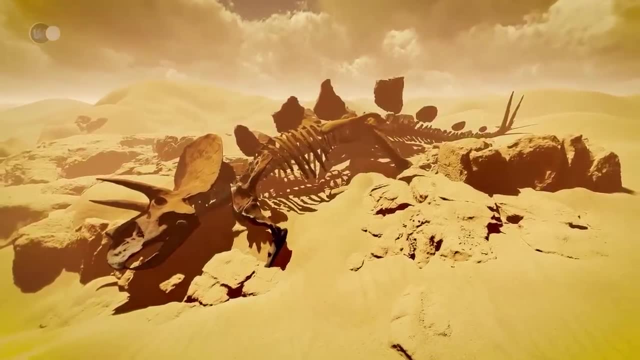 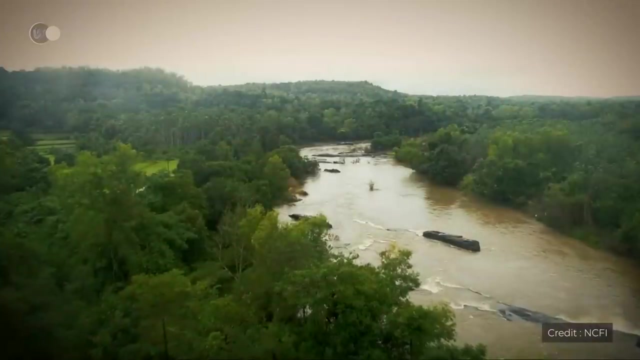 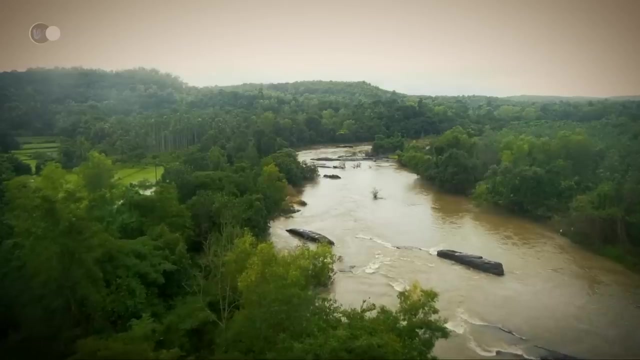 dooming some groups and giving new opportunities to others. When the dinosaurs disappeared, our distant ancestors survived. Dear traveler, welcome. Today we're going back in time to find out what the Earth was like after the dinosaurs became extinct. But before you leave for a new adventure, 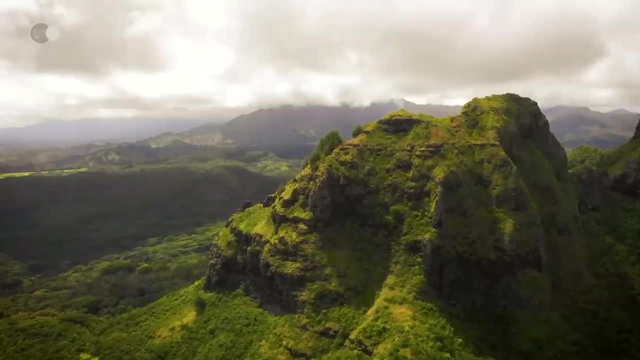 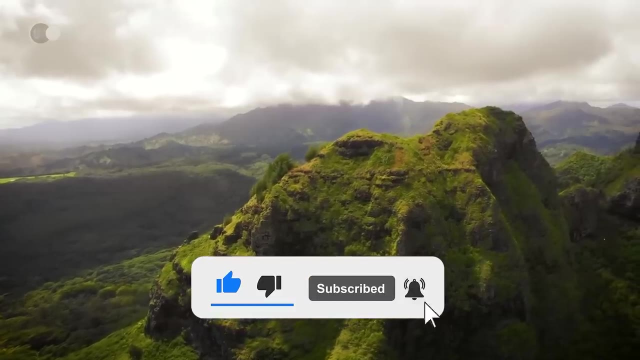 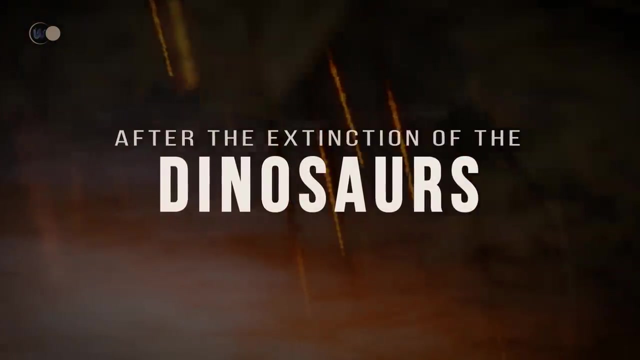 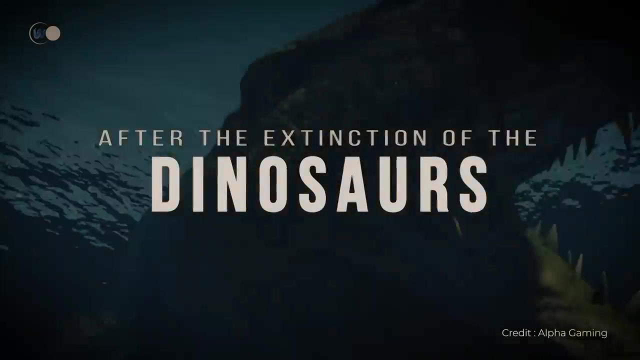 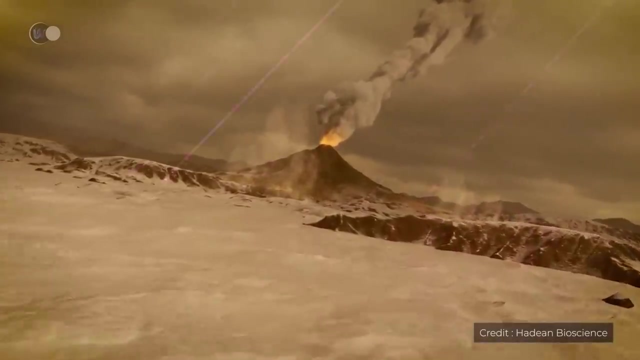 don't forget to like the video and subscribe to the channel so you don't miss anything. Thank you and welcome to Life Before and Life After the Dinosaurs. A mass extinction is an event that resembles a relatively brief biological crisis on the geological timescale. 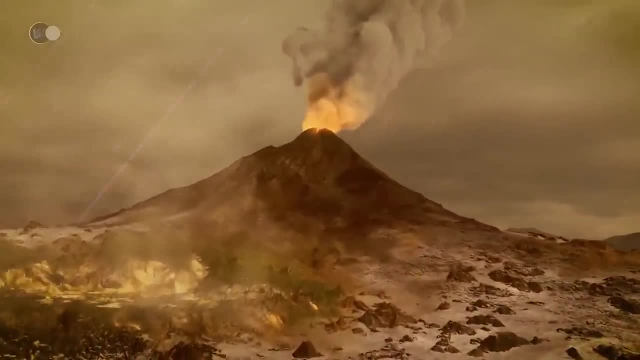 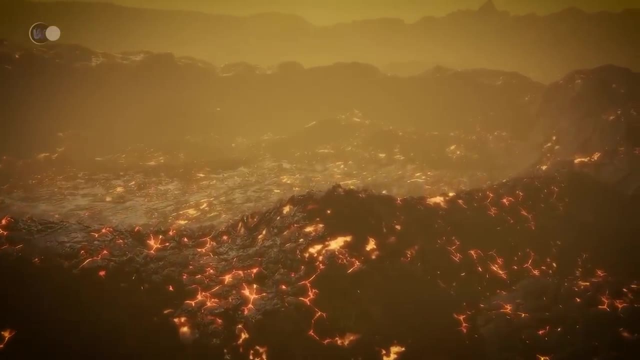 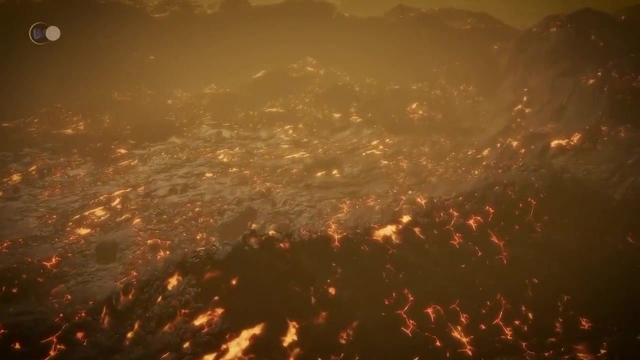 At least 75% of all animal and plant species disappear from the Earth's surface. In the last 500 million years, life on the planet has undergone five mass extinctions. 75 to 90% of all terrestrial species have disappeared in catastrophes of titanic proportions. 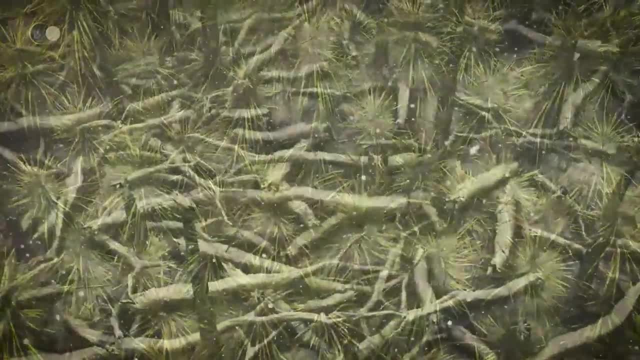 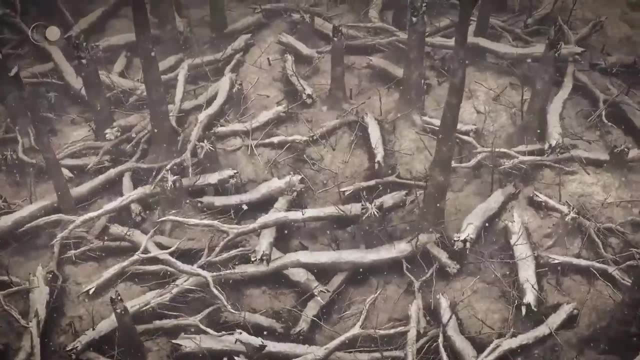 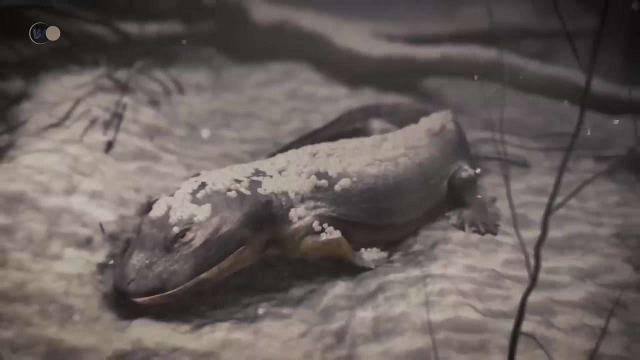 Today, more than 99% of all organisms that have ever lived on Earth have disappeared. The phenomenon of species extinction is no longer surprising. Species are deadly. Each of the great mass extinctions has played a role in the history of the living world. 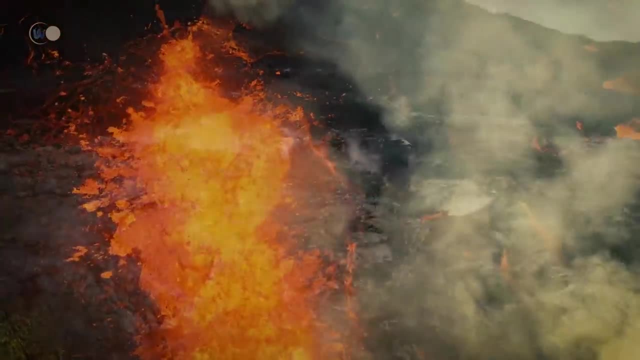 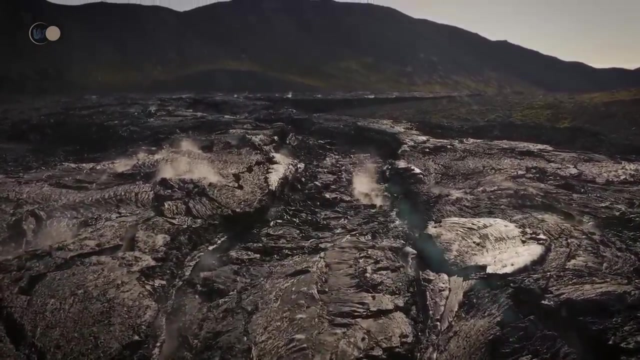 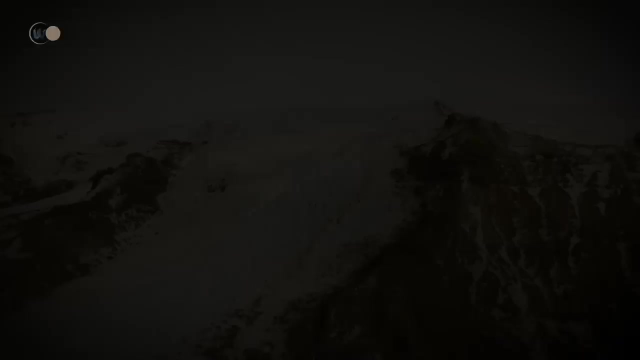 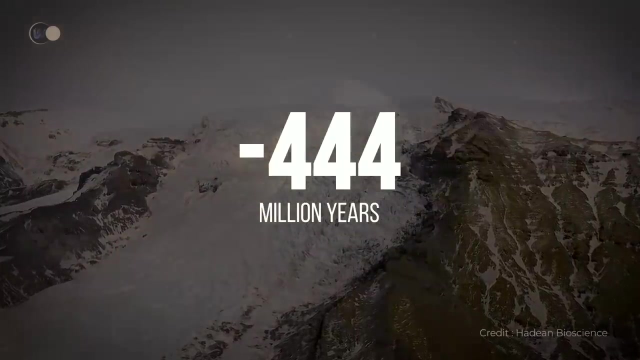 leading it down new paths, as the decimated fauna and flora are forced to evolve. These deadly events, however, pave the way for new forms of life. The Ordovician-Silurian extinction occurred 444 million years ago. A geological event caused an episode of glaciation. 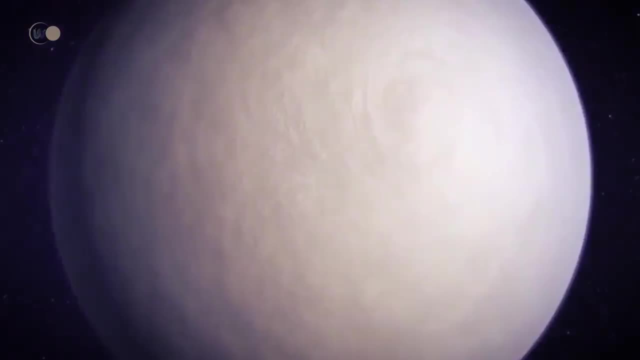 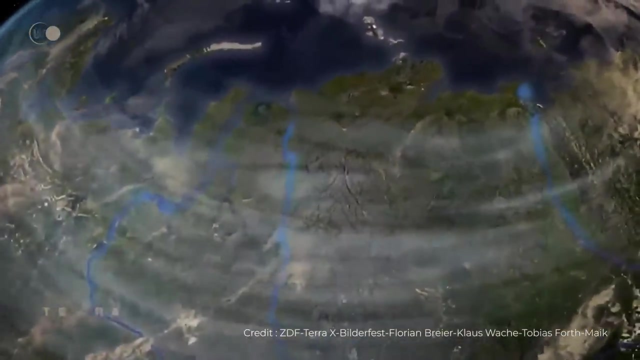 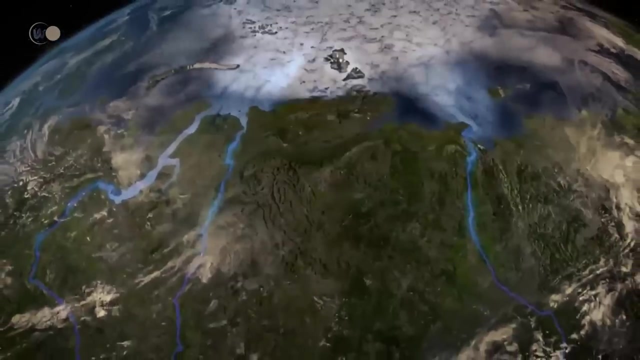 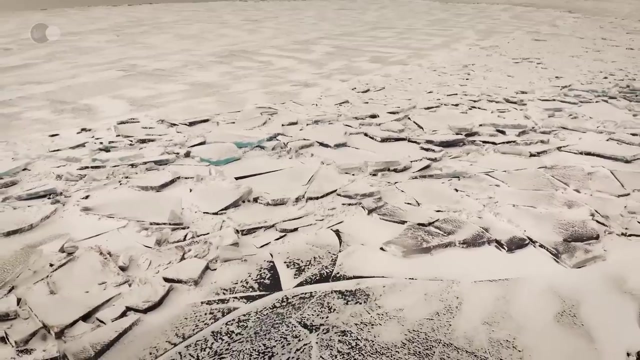 Considerable quantities of water were trapped in an ice cap occupying three times the area of present-day Antarctica. The carbon dioxide present in the atmosphere was sucked out because of the alteration of the rocks, and the temperature on Earth decreased considerably. Sea levels dropped and marine creatures saw their habitats cool and shrink. 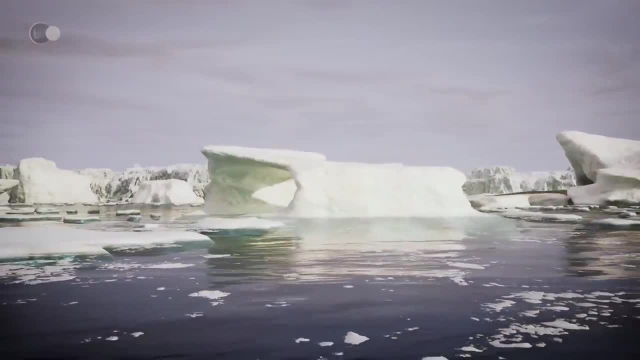 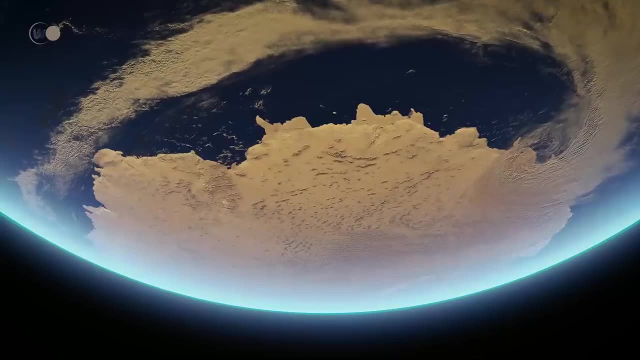 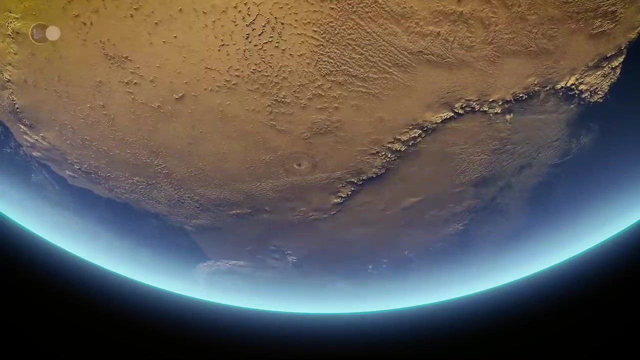 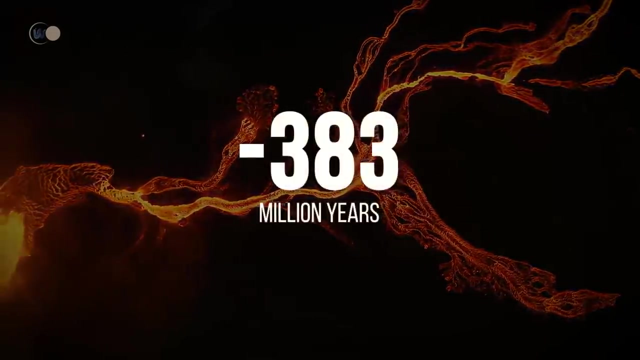 Once sea levels began to rise again, the levels of available oxygen in the water dropped, resulting in higher concentrations of dissolved toxic metals. This event resulted in the extinction of 85% of all terrestrial species. The Devonian extinction began 383 million years ago. 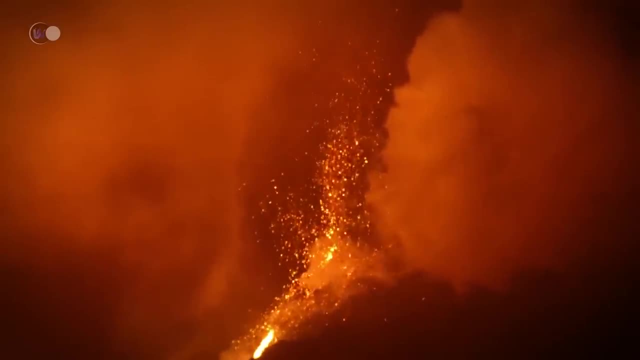 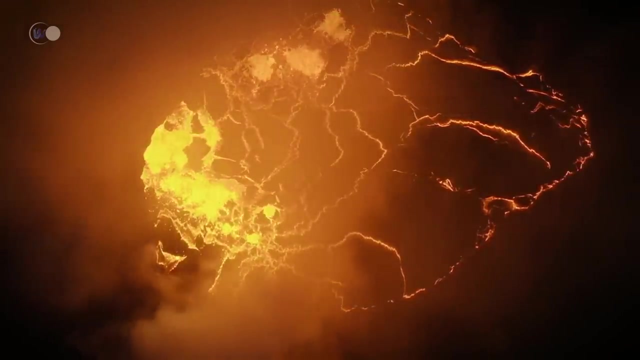 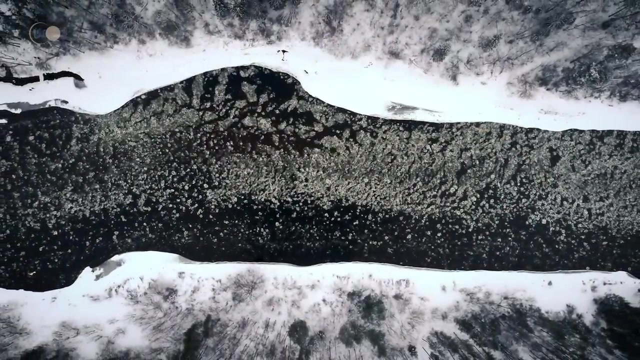 Probably due to a strong volcanic episode, pulses caused the oxygen level in the oceans to drop sharply. This was a real catastrophe for the marine fauna and flora. The Earth suddenly froze again, but this episode was shorter, lasting less than a million years. 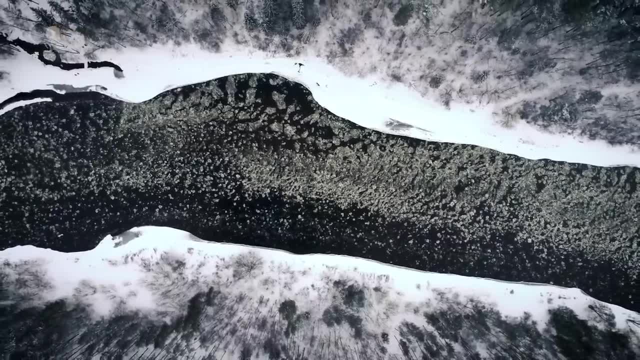 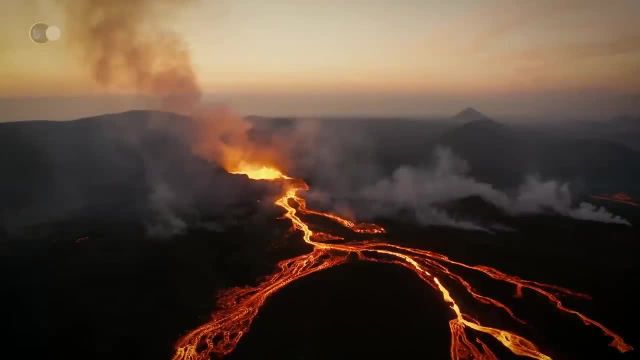 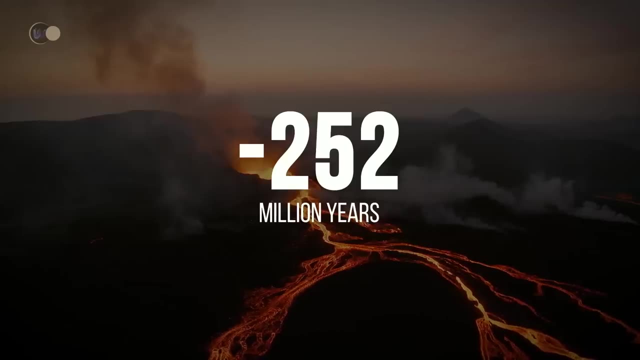 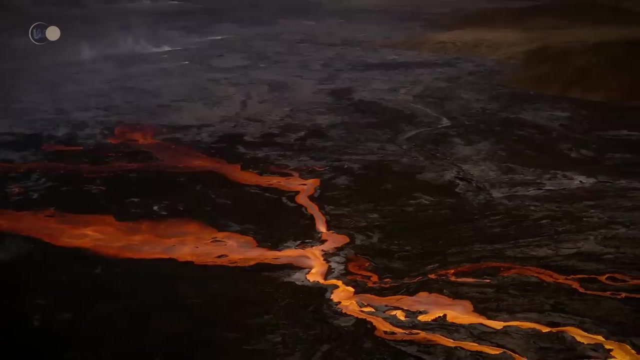 75% of the species disappeared during this mass extinction. The third mass extinction, the Permian-Triassic extinction, took place 252 million years ago. It was the worst catastrophe that life on Earth has ever known. More than 90% of the species were killed. 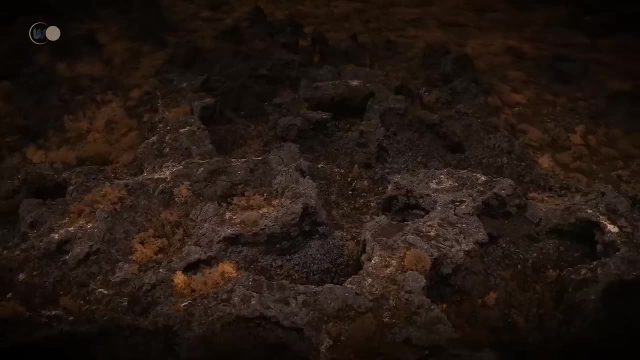 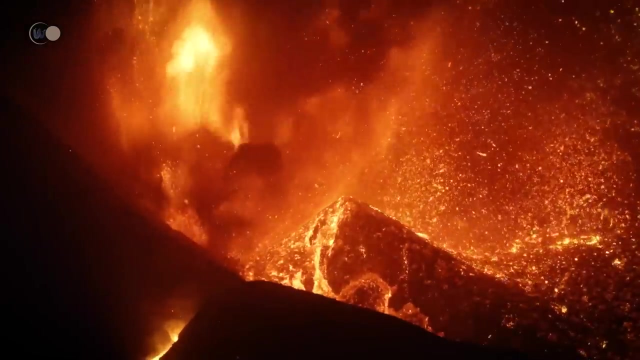 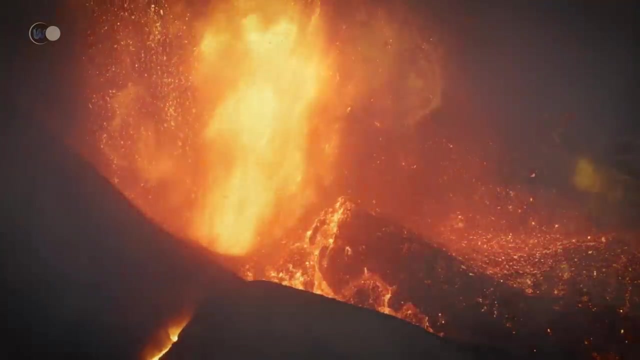 The destroyed forests will need more than 10 million years to recover. Huge lava spurts occurred during volcanic eruptions, releasing billions of tons of carbon. The magma then seeped into the coal fields towards the surface, causing other greenhouse gases, such as methane, to evaporate. 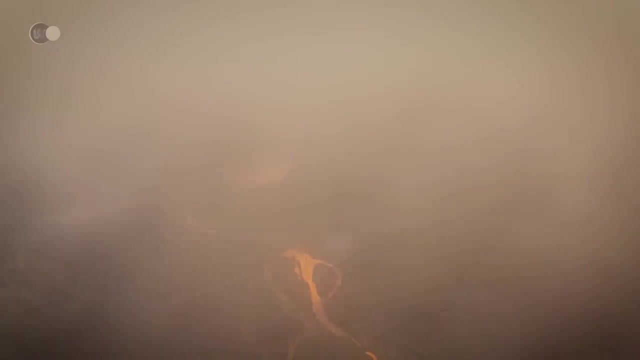 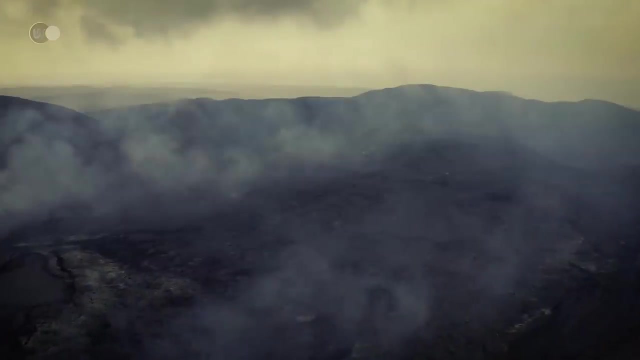 As a result, global warming of an inordinate magnitude occurred. Seawater and surface temperatures at the Earth increased by several degrees. The Earth's rocks were rapidly altered by acid rain. Oxygen in the oceans decreased by about 76%, harming marine life. 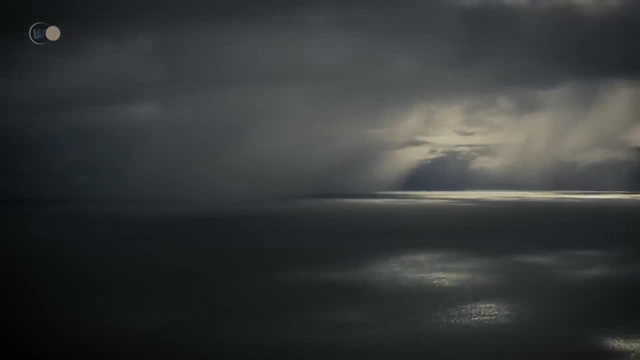 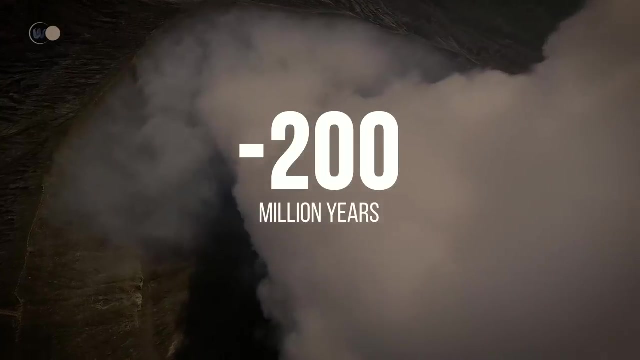 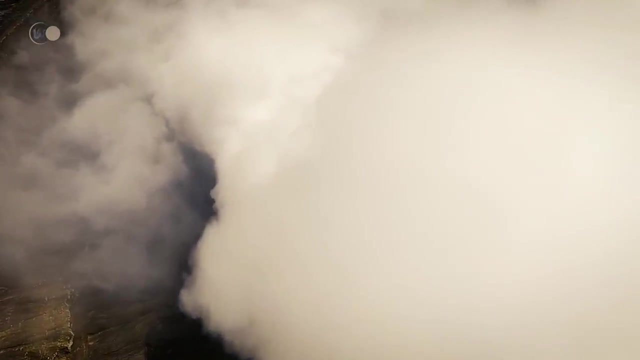 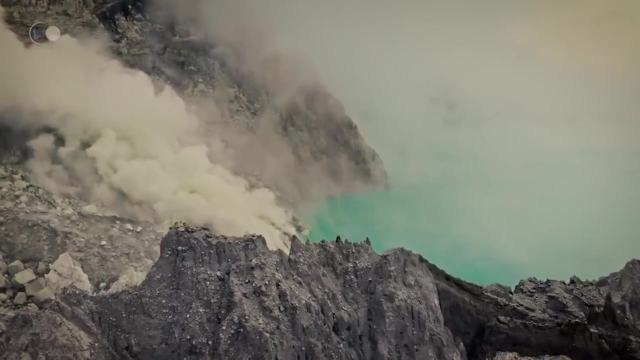 About 200 million years ago, the Earth underwent the Triassic-Jurassic extinction. Geological events caused a warming of the Earth's surface and an increase in the concentration of carbon dioxide in the atmosphere. The oceans have become acidified, preventing marine species from developing properly. 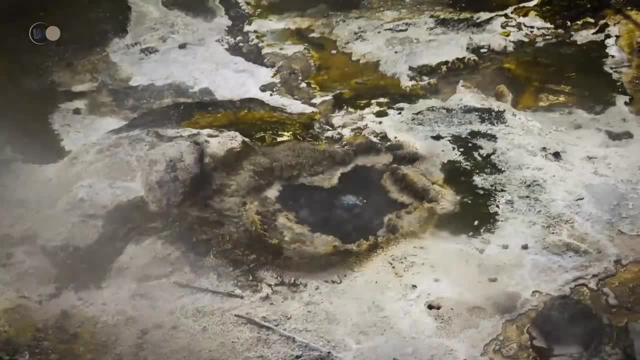 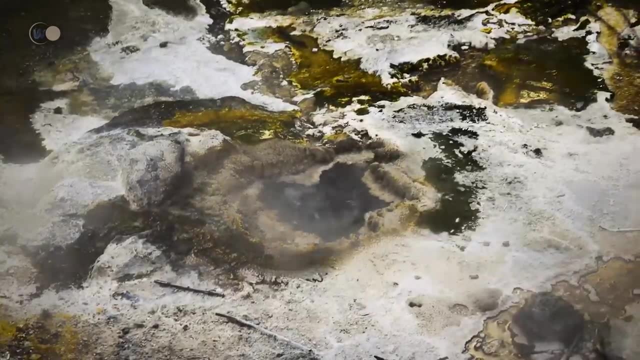 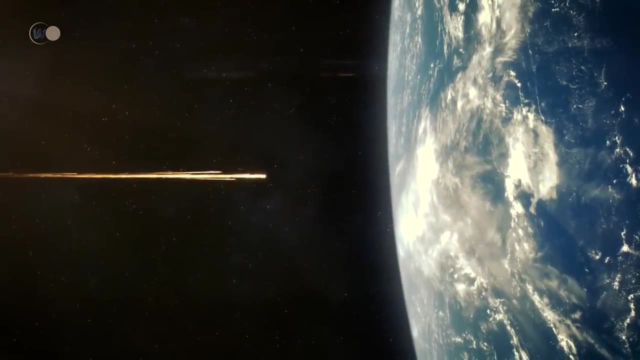 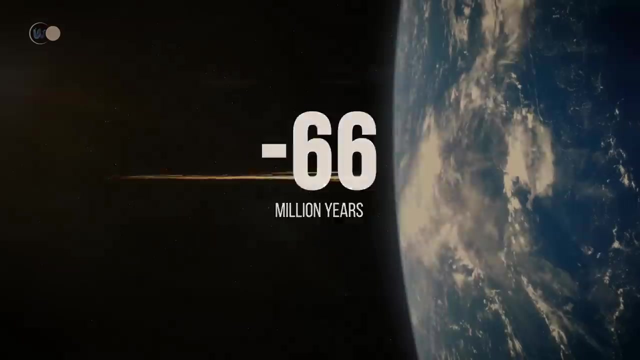 This is a new blow for life on Earth, which is losing up to 80% of terrestrial and marine species. The fifth and last mass extinction is that of the Cretaceous Paleogene, 66 million years ago. It was caused by the major impact of an asteroid. 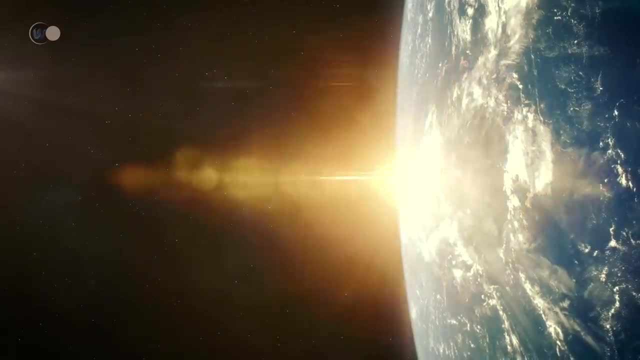 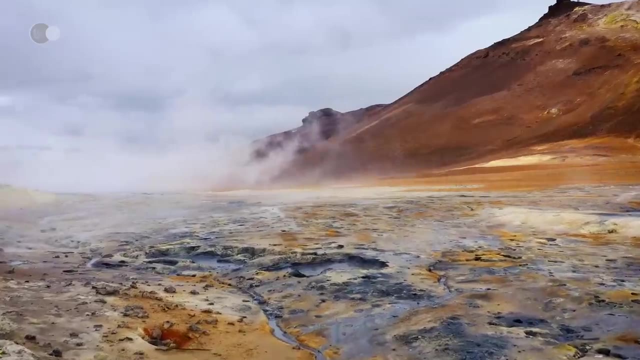 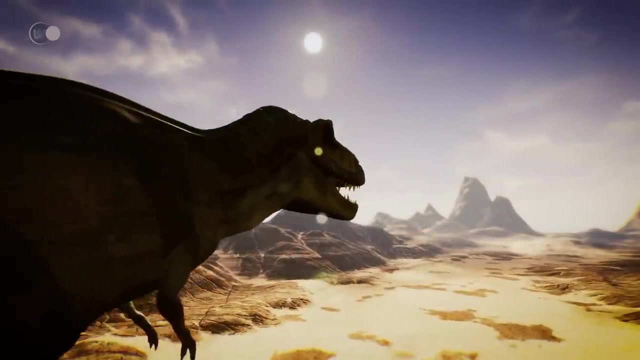 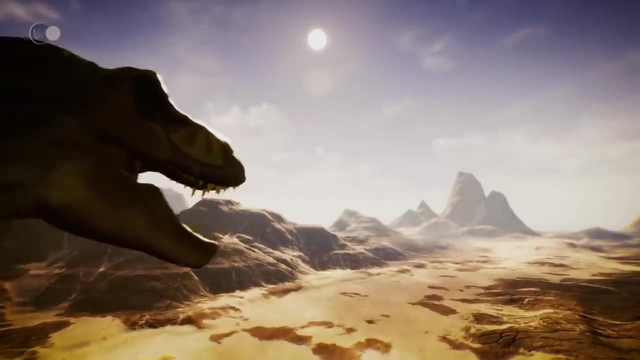 and nearly 65% of the species in the biosphere disappeared. But if this catastrophe remains the most famous, although not the most deadly, it is because it saw the disappearance of all species of the famous non-avian dinosaurs. The end of the dinosaurs is an event that marks the minds. 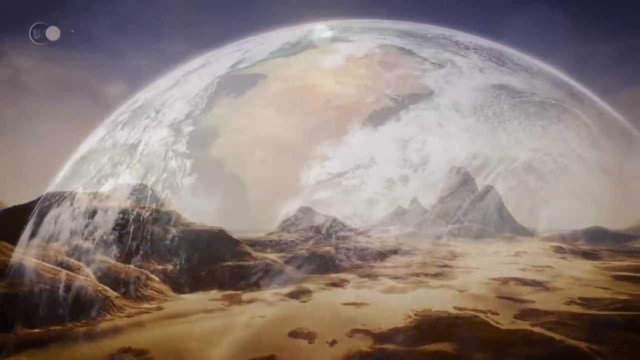 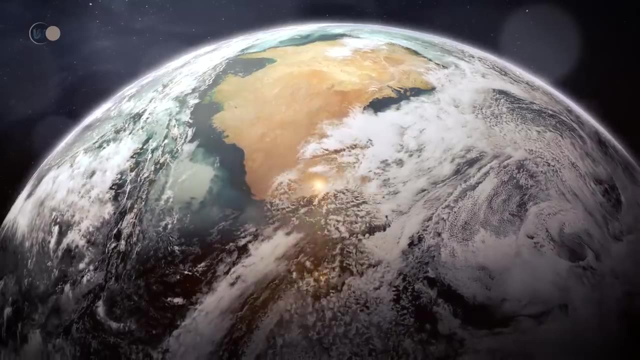 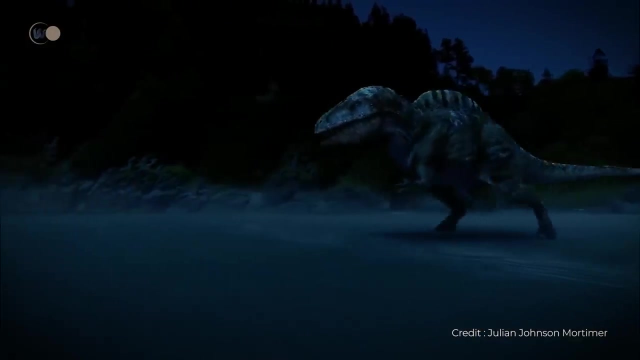 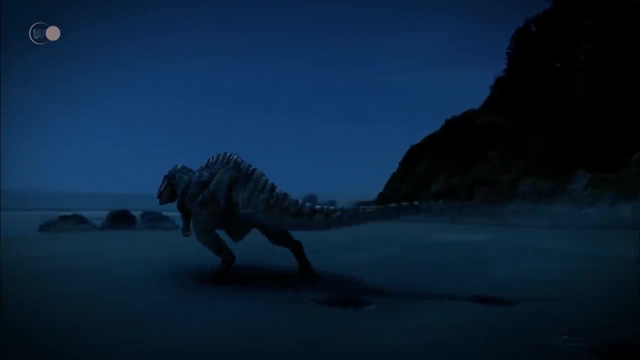 However, man had no part in it, since nearly 60 million years separated the last dinosaurs from the first being that could be described as almost human. This extinction evokes the drama of the great disappeared civilizations. The dinosaurs reigned supreme for more than 165 million years. 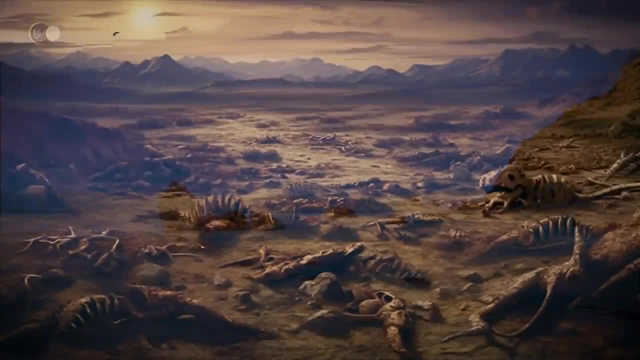 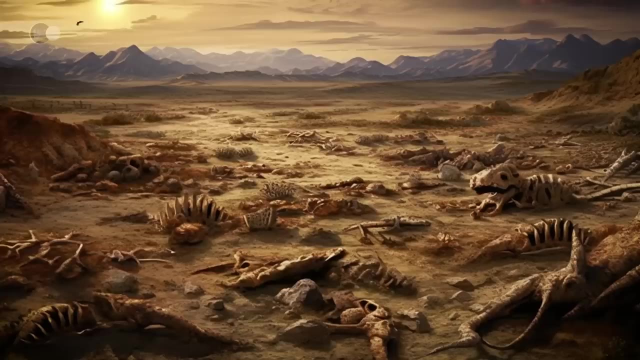 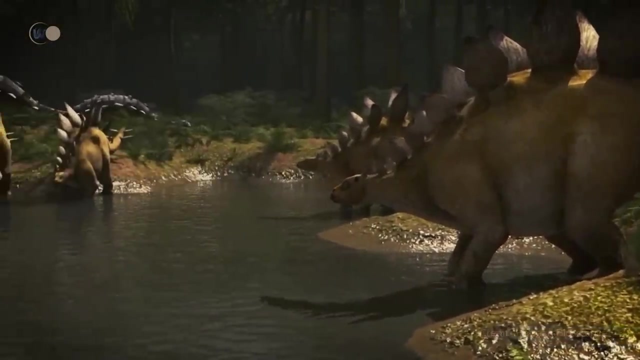 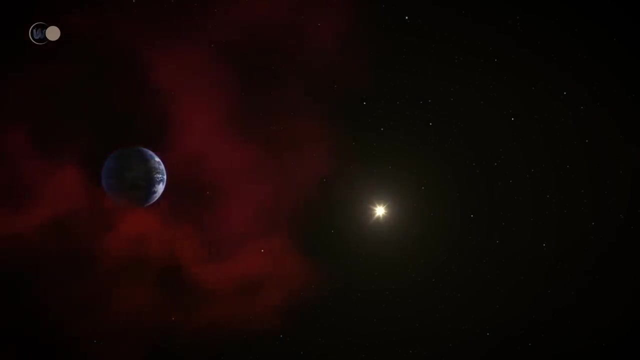 and dominated all the continents. This great extinction has long remained mysterious and remains one of the great enigmas of the history of the globe, Even if scientists agree on a possible scenario. But before going into details, let's see what the world looked like at the time of the dinosaurs. 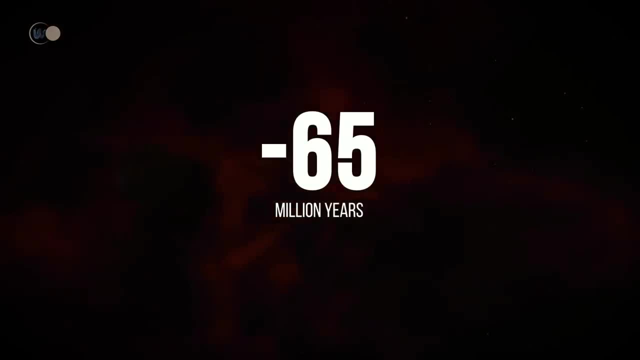 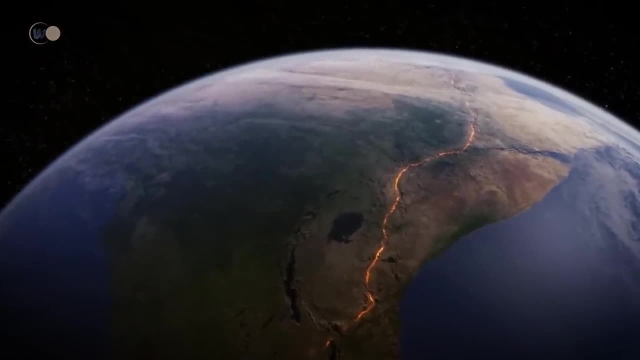 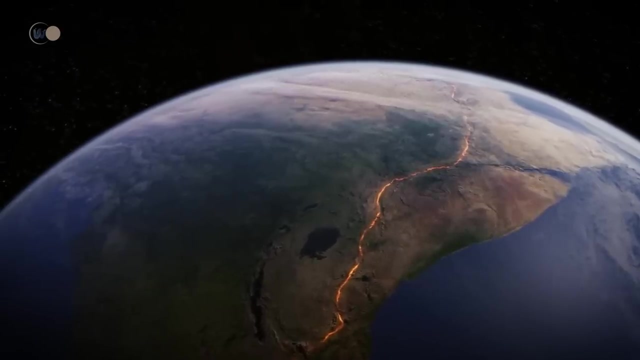 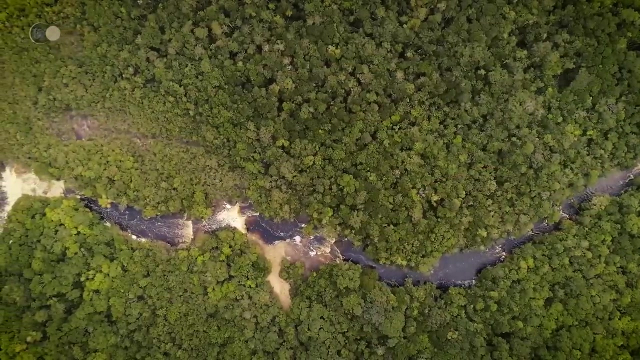 We are in the Cretaceous period, a little over 65 million years ago. Seen from the sky, the Earth appears somewhat familiar. The supercontinent Pangea has already split into two continents: Laurasia and Gondwana. Later Laurasia splits into two parts to reveal the future North Atlantic Ocean. 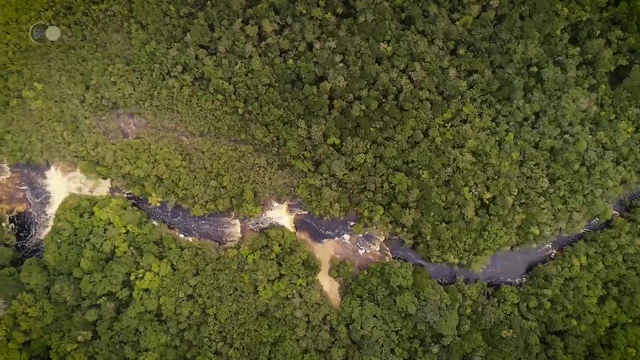 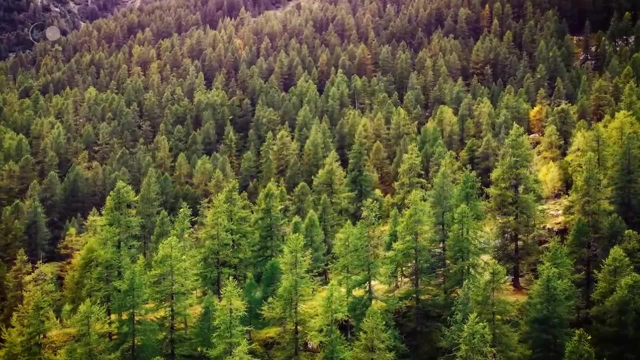 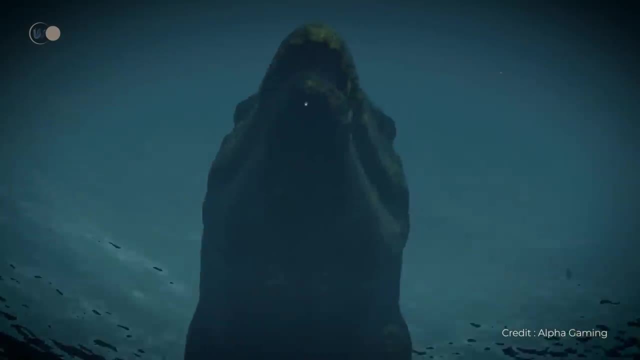 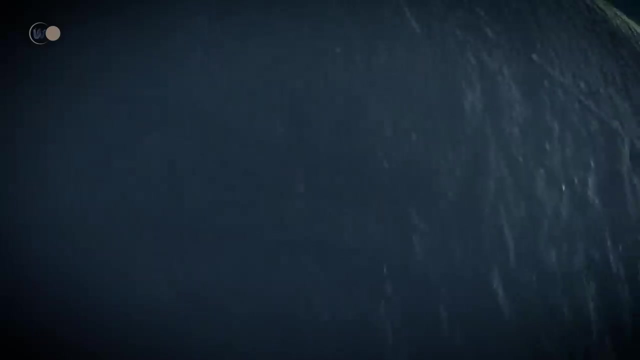 The general climate is rather hot and humid. The sea level is high. The vegetation is highly diversified. We find ferns, conifers, but also flowering plants which dominate, thanks to the help of insects, In the seas and on the land. it is time for gigantism. 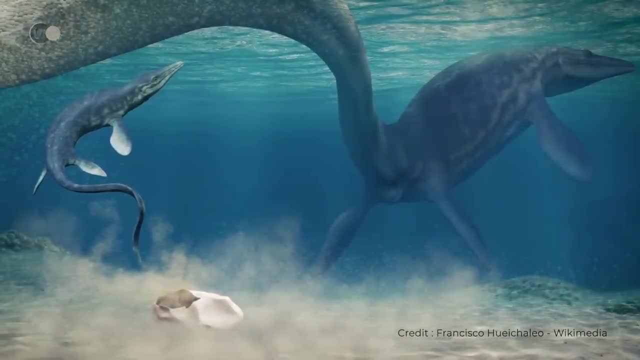 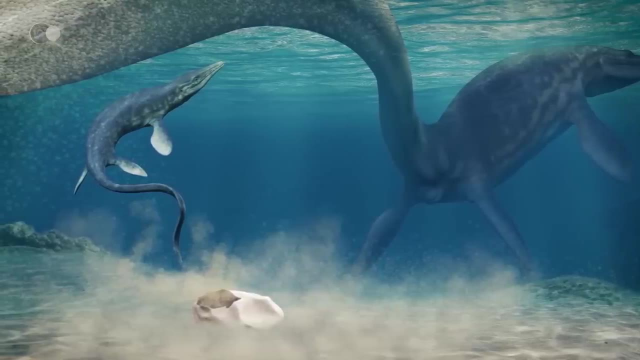 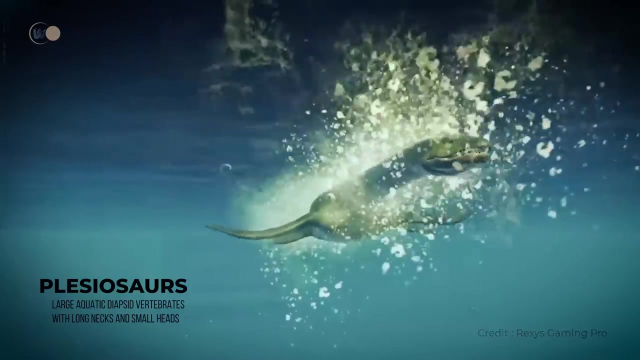 The great family of marine reptiles is the master of the Cretaceous waters. These reptiles occupy all environments, from the coastal reefs to the open sea. The Pleisosaurs do not swim with their tails, but use their legs, transformed into a swimming paddle. 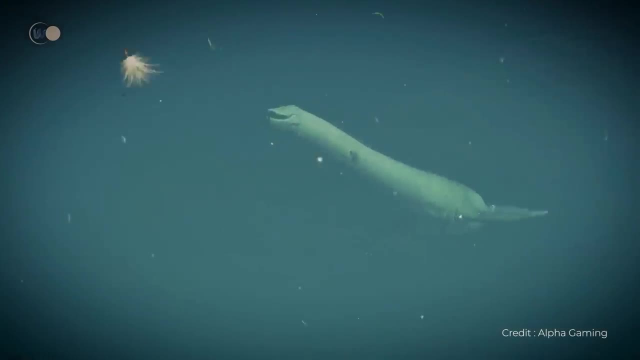 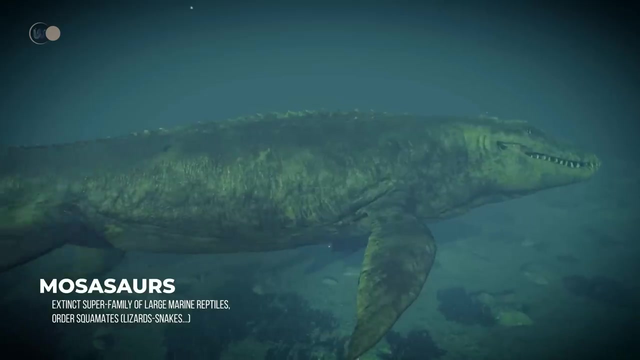 They feed on ammonites, fish and other marine reptiles. Mosasaurs are cousins of lizards and monitor lizards. They measure between 1 and 15 meters long, or between 3 and 50 feet Thanks to their long, vertically flattened tail. 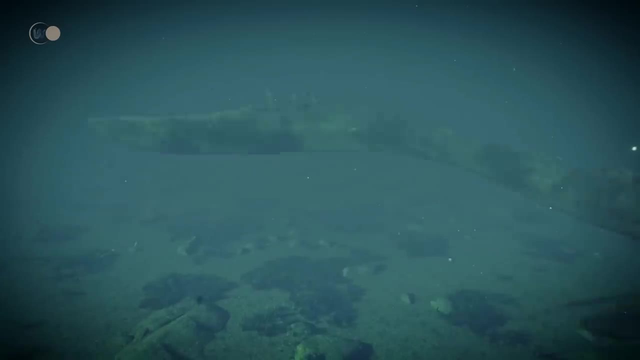 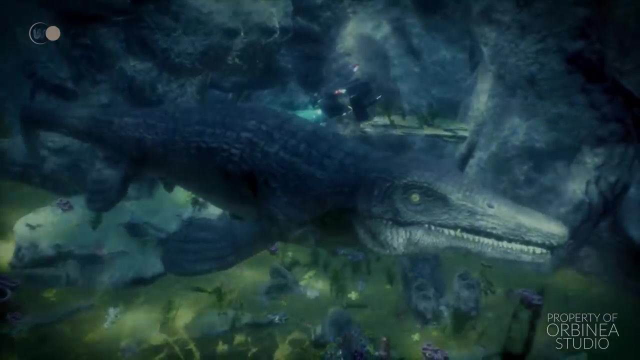 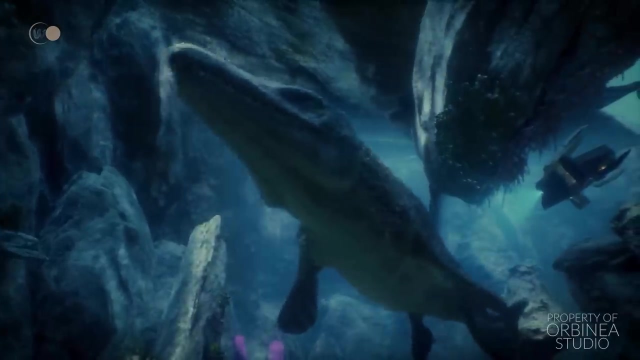 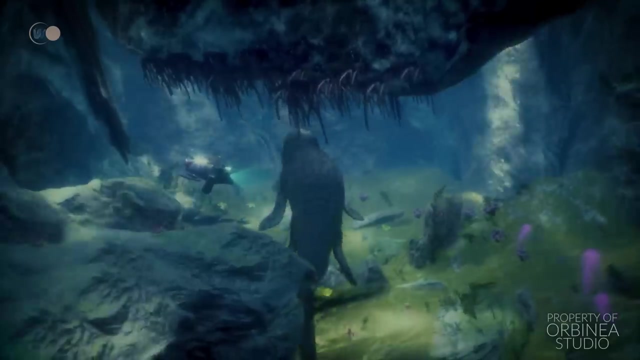 they can propel themselves underwater. Their limbs are transformed into a swimming paddle, giving them the ability to swim. They feed on fish and other reptiles. All these reptiles breathe with lungs and not with gills. They must therefore regularly come to the surface to renew their air supply. 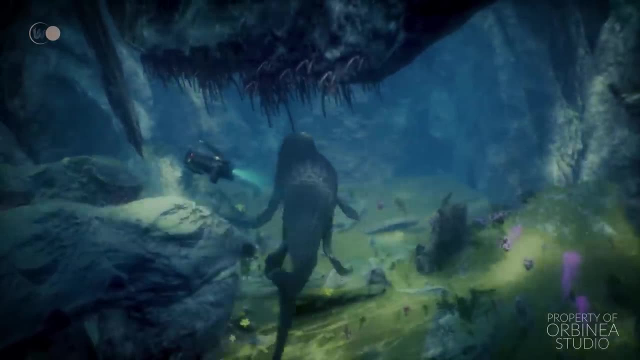 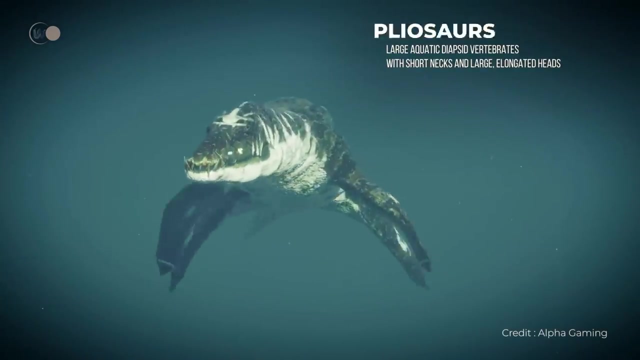 Some species, however, have nostrils that are too small for this. like the Pleiosaurs, They swim with their mouths half open, letting the water pass through openings in the palate and out through the nostrils. The odors are analyzed in passing. 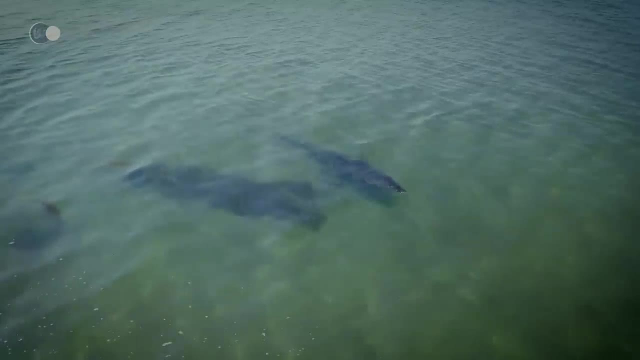 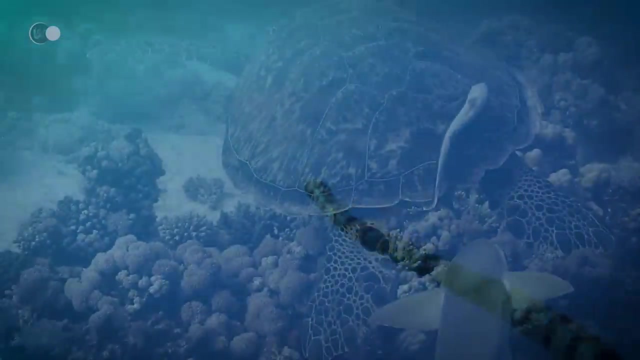 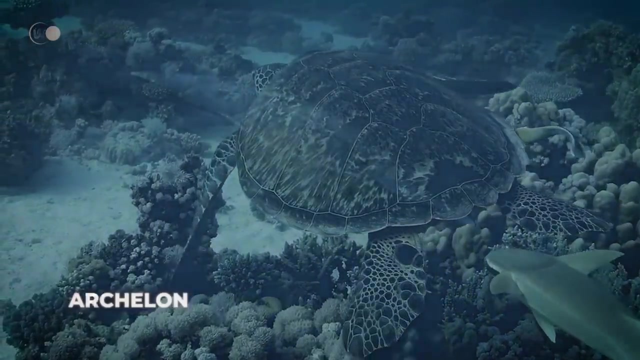 Other, more famous species are found alongside these reptiles, such as marine crocodiles, flat-bodied snakes and sea turtles. Archelon is a sea turtle that lives in the shallow sea. It is the largest sea turtle known to date to have lived alongside dinosaurs. 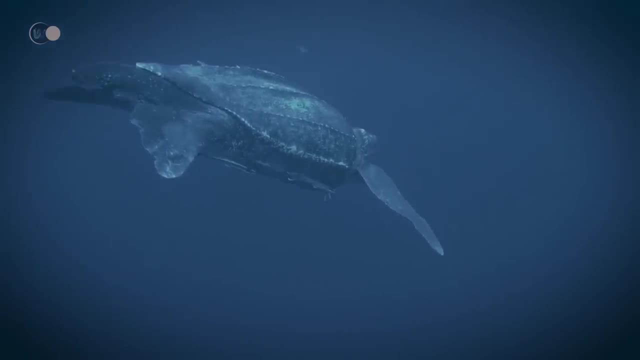 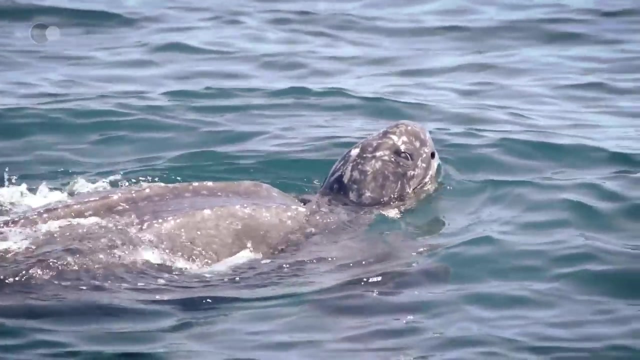 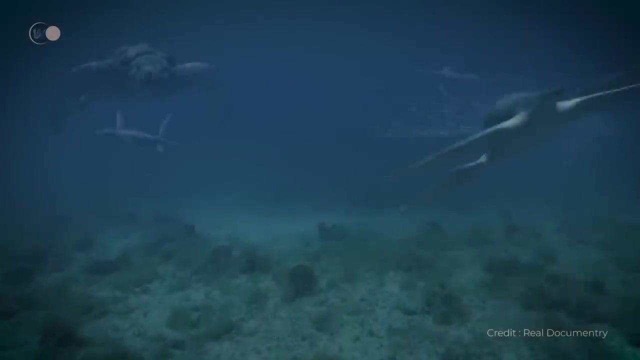 It is over 4 meters or 13 feet long. With its strong beak it is able to break the shells of ammonites, belemnites, bivalves and other crustaceans. It can also tear off tough seaweed and grass. 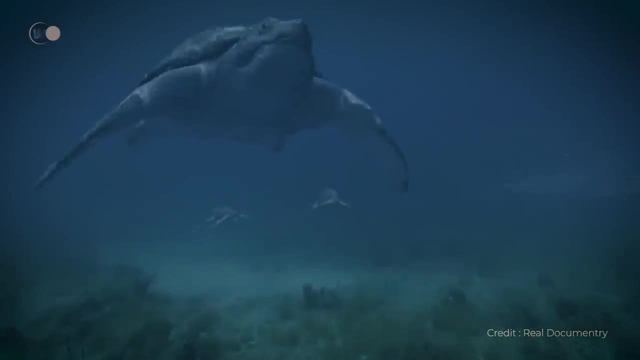 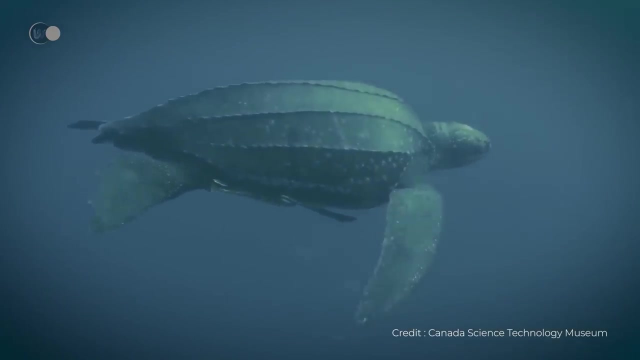 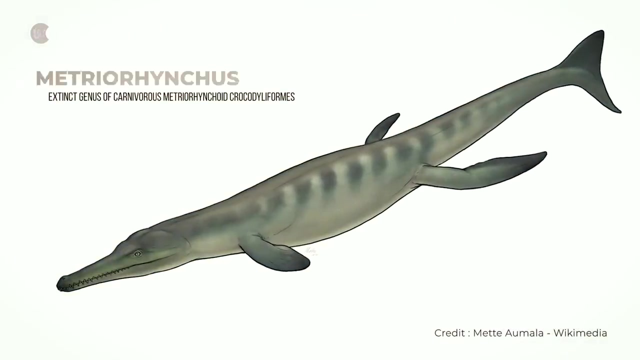 Its skeleton is light. Thanks to its large fins, it can move very quickly underwater to catch its prey or escape its predators, such as mosasaurs. Metriorhynchus is a kind of carnivorous crocodile form, exclusively marine. 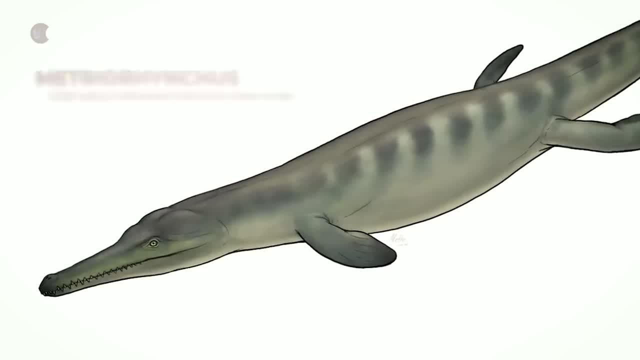 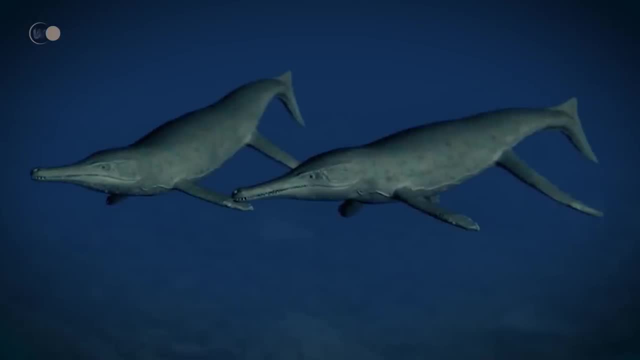 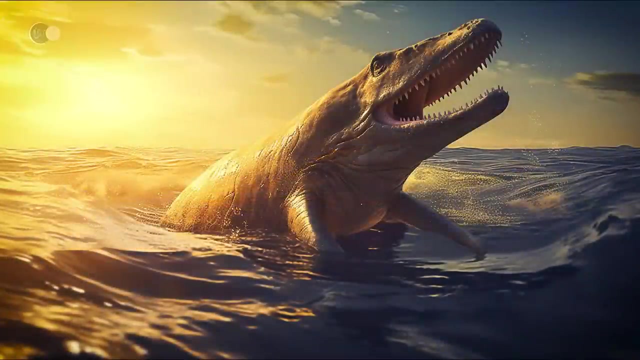 It can reach up to 3 meters or 10 feet long. Its body is equipped with a caudal fin in the shape of a moon, making it a much more efficient swimmer than modern crocodile species. Its legs have taken the form of short, flat fins. 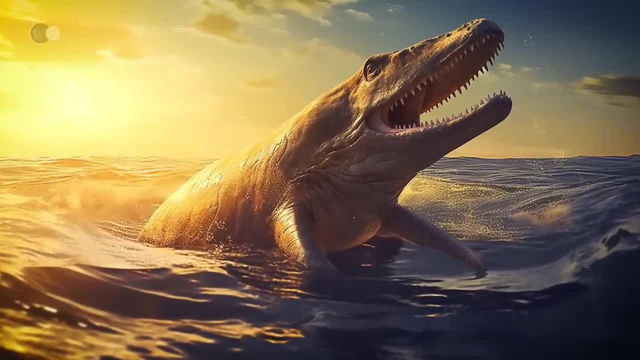 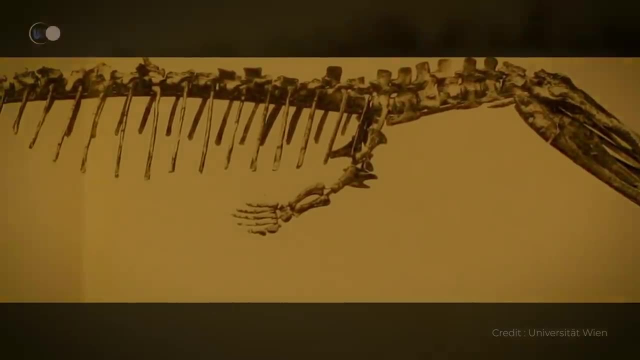 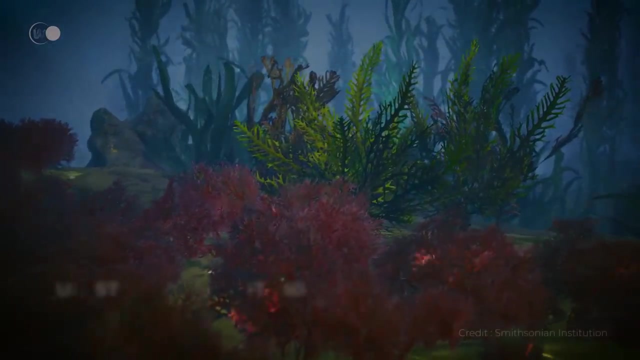 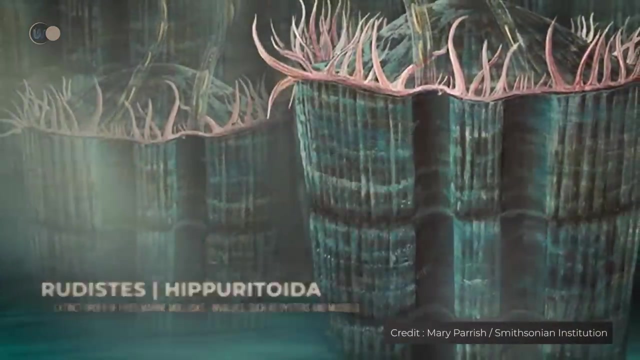 in which all the fingers of a single limb are united in a single membrane. The marine fauna includes smaller creatures living quietly alongside the giants. The rudists are a family of bivalves that were very present during the time of the dinosaurs. Some are solitary. 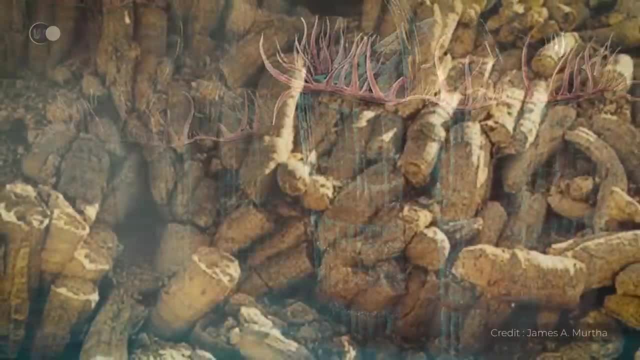 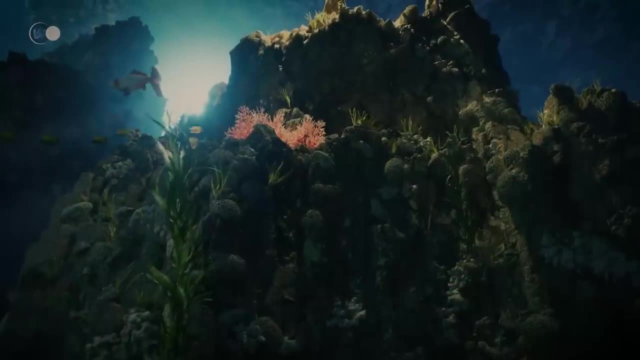 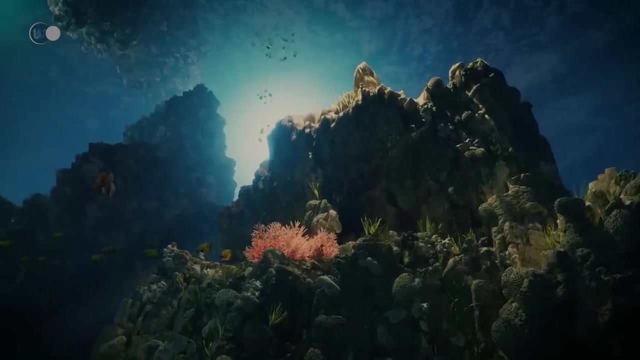 and others form dense colonies and build real reefs offering shelter to fish, shrimps or even sea slugs To feed themselves. they filter the seawater and capture plankton and debris in the water. Plankton contains, among others, 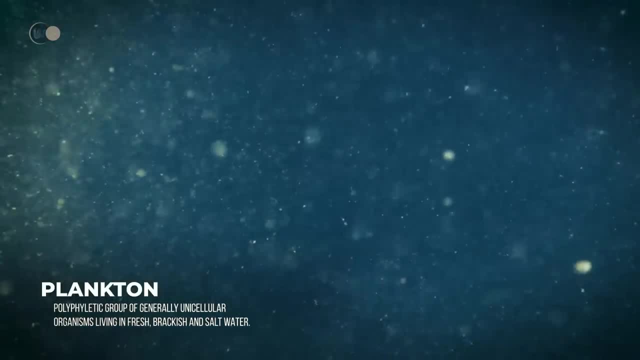 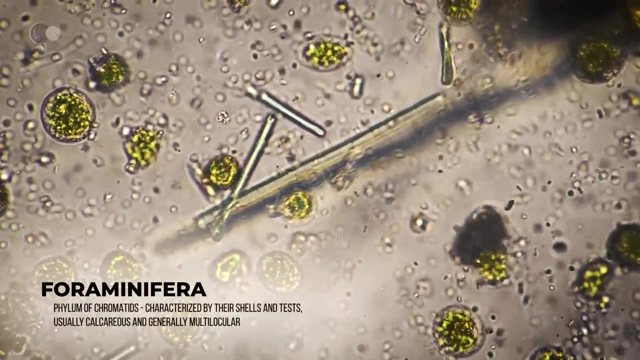 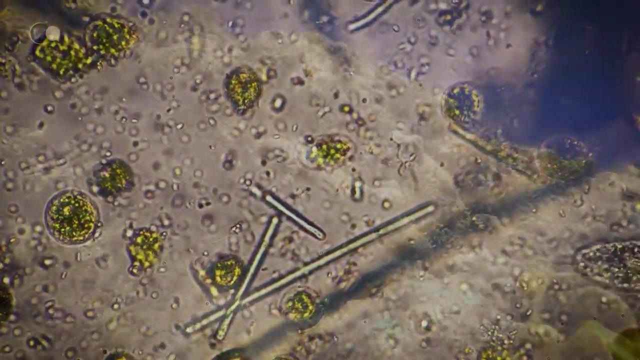 foraminifera. These are single-celled animals protected by a shell rolled up on itself. Even if they contain only one cell, they can reach up to 8 centimeters or 3 inches in diameter. There is no shortage of fish, of course. 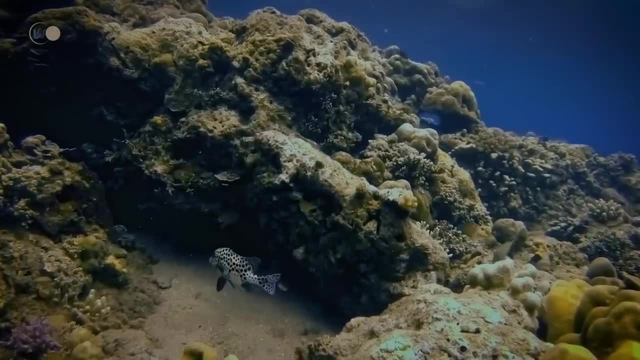 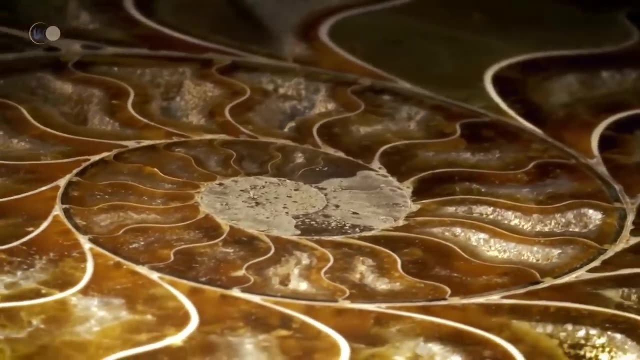 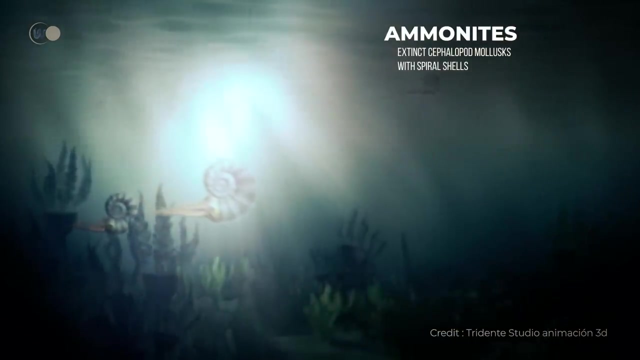 The representatives of our modern fishes appear at this time, even if they are not yet very numerous. The seas are also inhabited by mollusks and ammonites are strongly represented, Protected by a spiral-shaped shell and made up of a series of chambers. 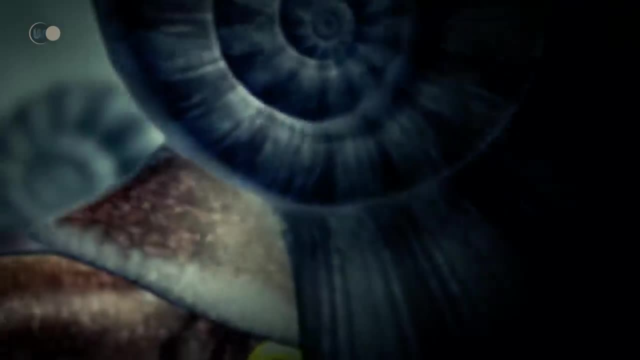 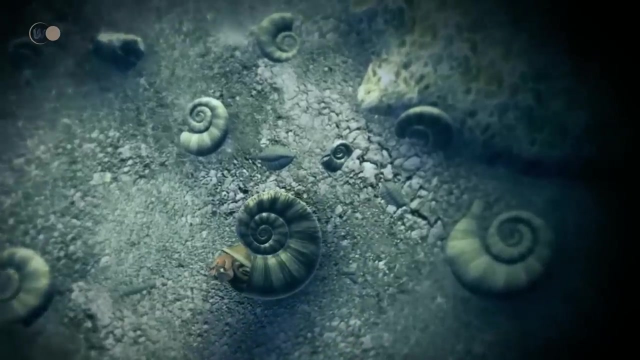 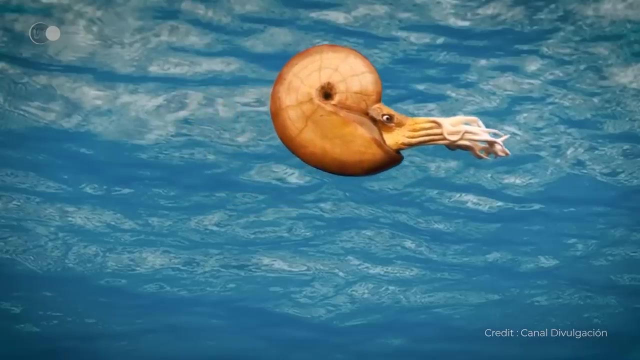 the animal stands in the last chamber, which is often the largest. It moves by means of a small tube which it can direct. Its tentacles are equipped with suction cups, thanks to which it can seize its preys. It crushes them then thanks to its jaws. 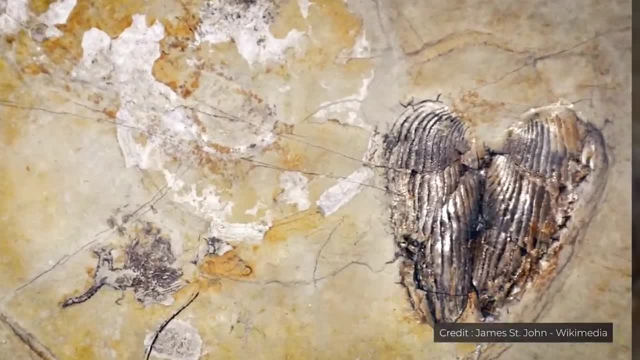 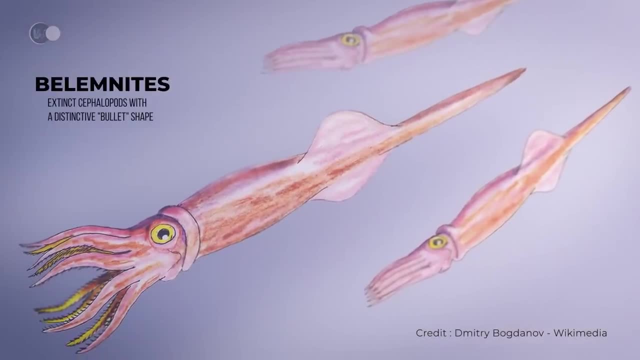 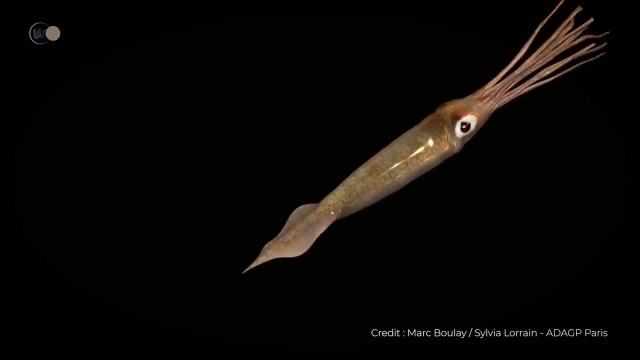 which look like a beak of a parrot. At that time, there were more than 5,000 species of ammonites. Beside them, the belemnites are cephalopods whose shell is internal. Their hydrodynamic body allows them to reach a high swimming speed. 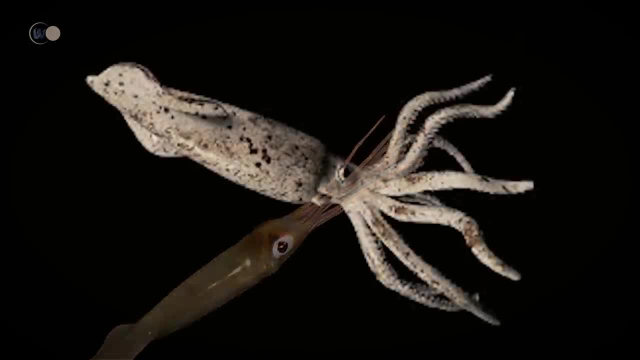 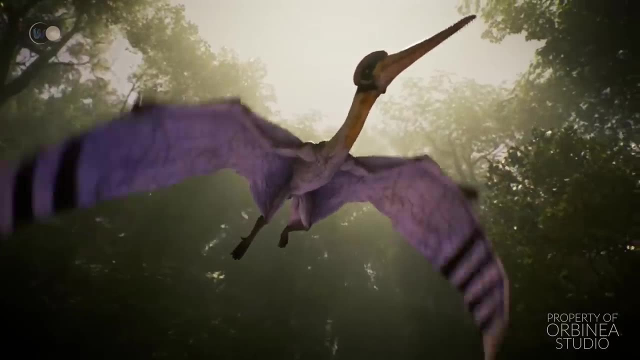 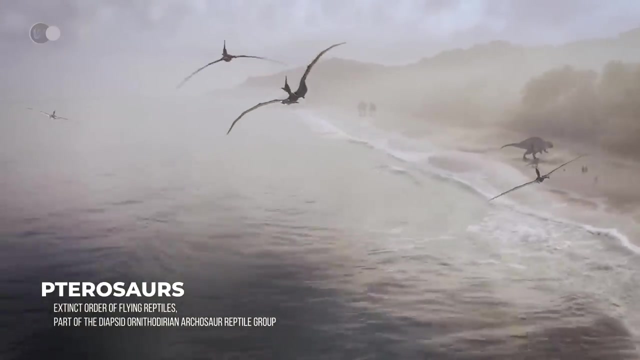 These carnivorous specimens capture fish. with their ten tentacles decorated with hooks, Birds and pterosaurs share the air. Pterosaurs are an order of flying reptiles that lived alongside the dinosaurs. One of them stood out for its impressive size, since it could reach up to 12 meters. 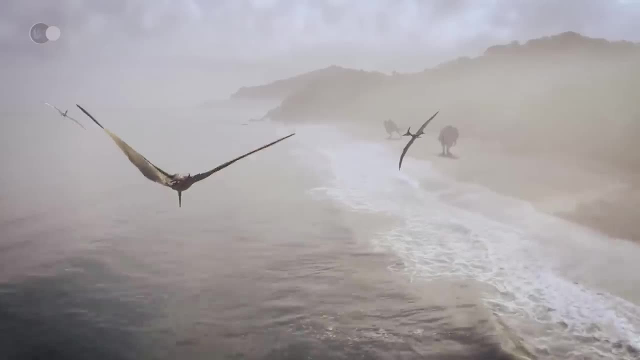 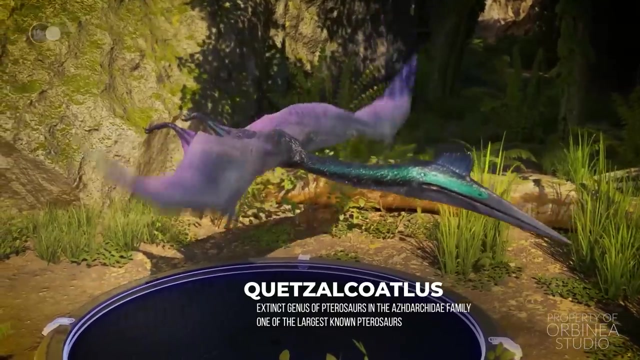 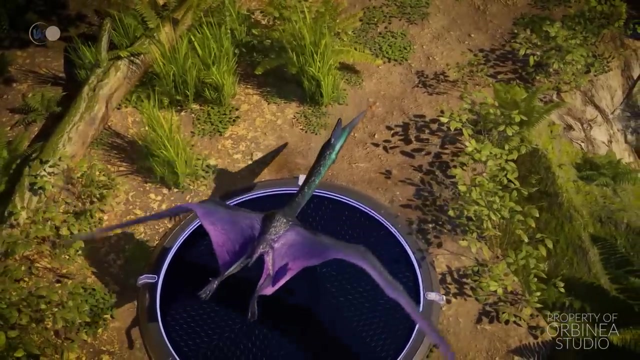 or 40 feet wingspan, It is the Quetzalcoatlus. It is affected by the gigantism of the time. Pterosaurs are great lovers of fish. Not being able to swim underwater, they are content to fish in flight. 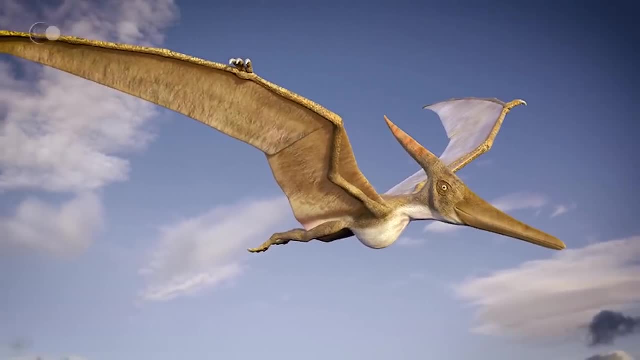 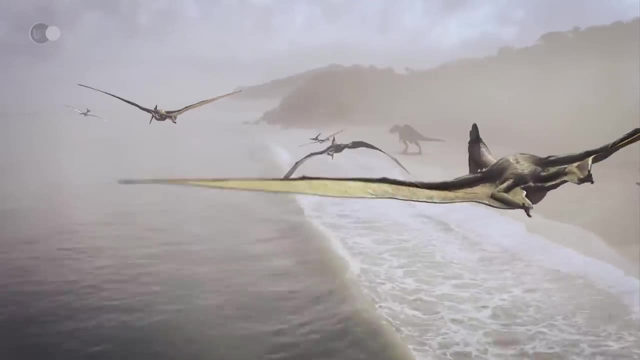 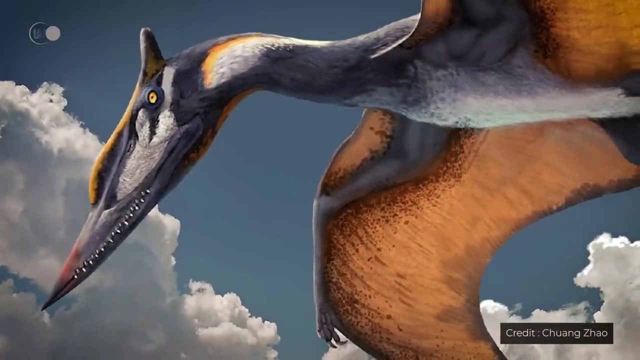 by sliding their beaks just on the surface of the water. Depending on the species, the beaks of pterosaurs are very diverse. Some have long, fine teeth to filter plankton, while others have no teeth and are more like scavengers. 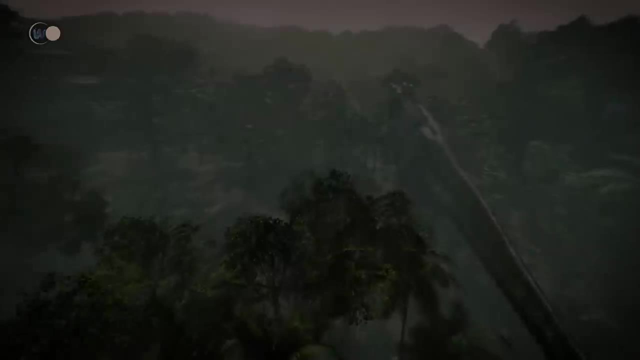 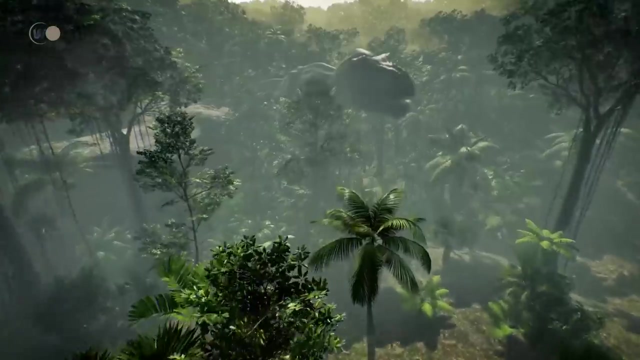 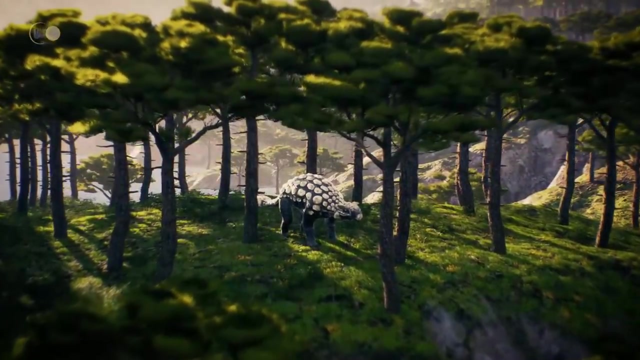 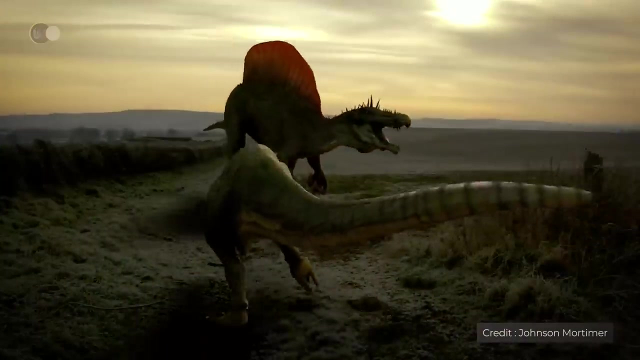 On land, dinosaurs are the dominant animal group. Thanks to their extraordinary size and weight, they diversified and evolved on all continents. Dinosaurs are the pride of the Cretaceous period. With their dragon heads and their long, sharp teeth, they never cease to fascinate. 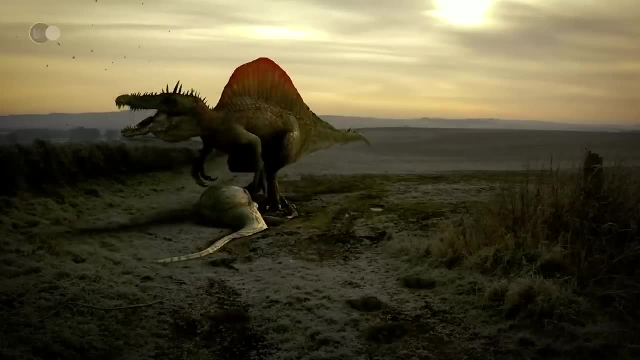 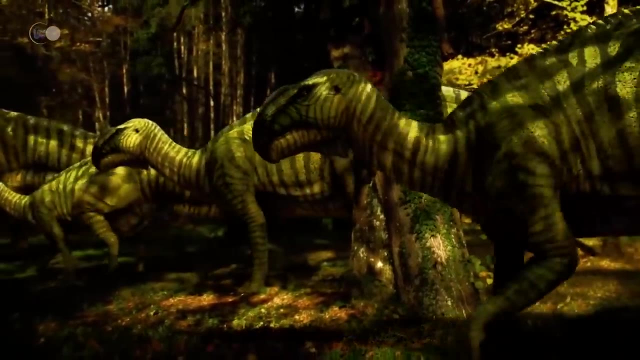 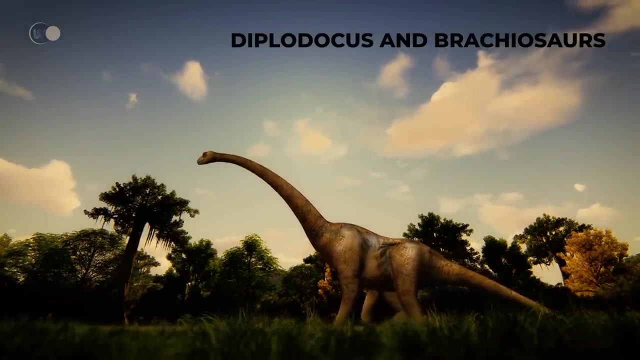 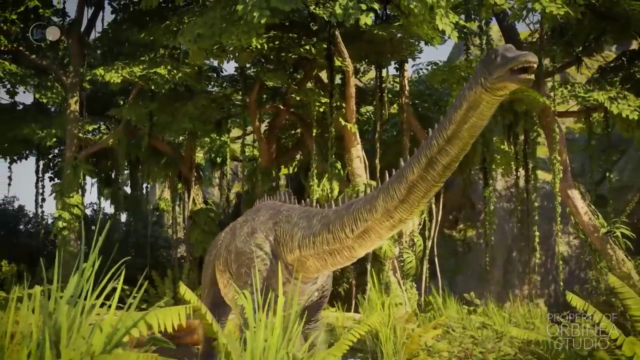 Beyond this popularized image, the world of dinosaurs remains a world apart. Diplodocus and Brachiosaurus are the largest land animals of all time. During their reign, they probably reached the size limit for a land animal on planet Earth. As an animal grows, its bones lengthen. 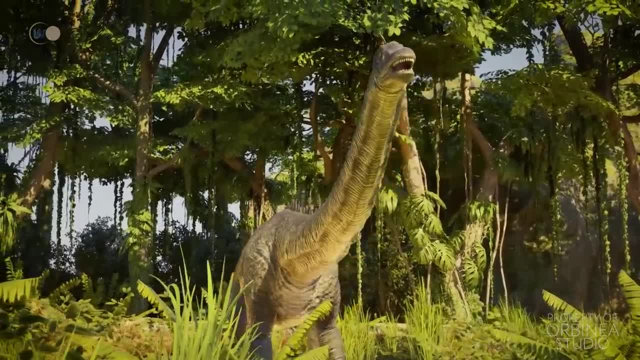 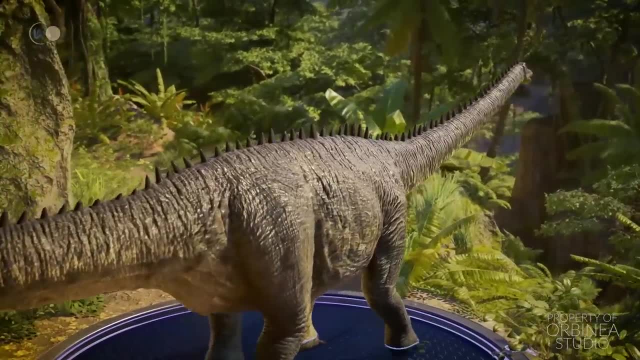 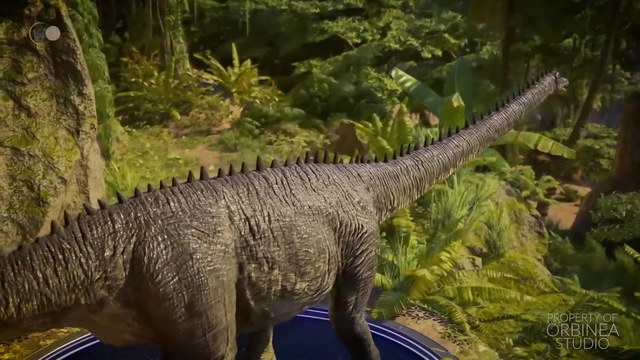 but they must also grow in order to remain strong enough to support its weight. The limbs become thicker and thicker and therefore heavier and heavier, further increasing the total weight of the animal. The maximum size of a land animal is therefore limited In Diplodocus and Brachiosaurus. 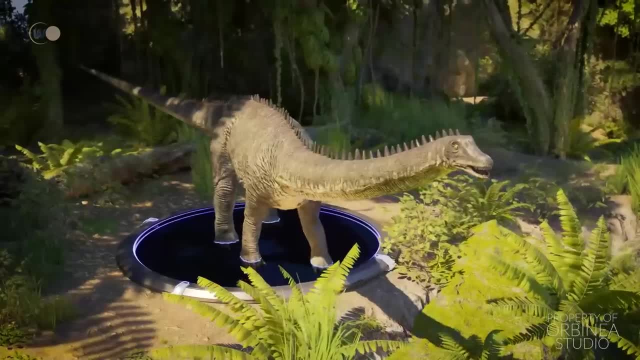 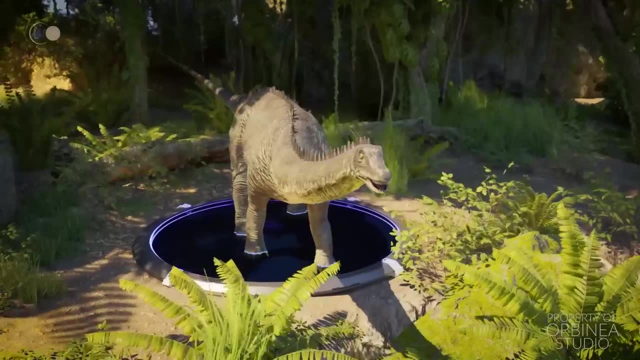 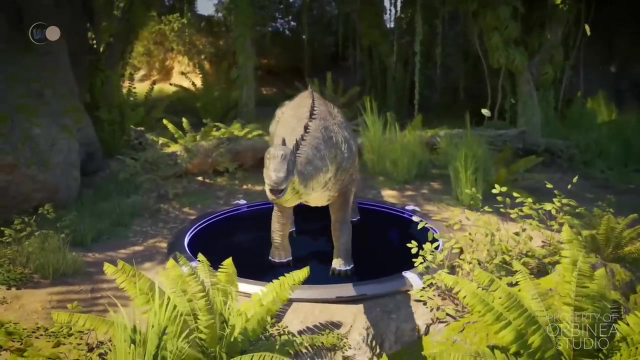 the vertebrae and ribs are hollowed out with multiple cavities. This makes the skeleton lighter without reducing its strength. However, it seems that no dinosaur could have exceeded a length of 40 meters or 130 feet and a weight of 100 tons. 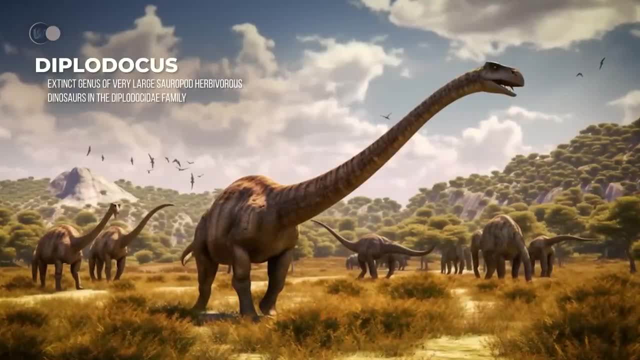 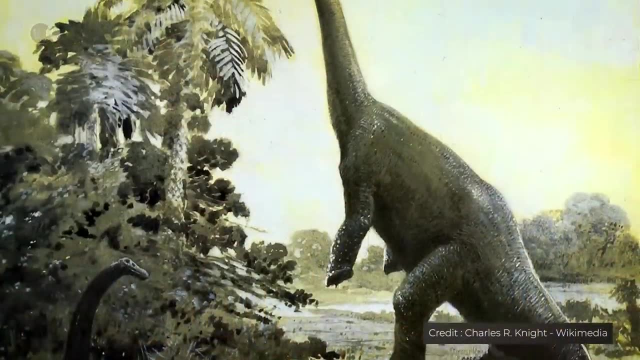 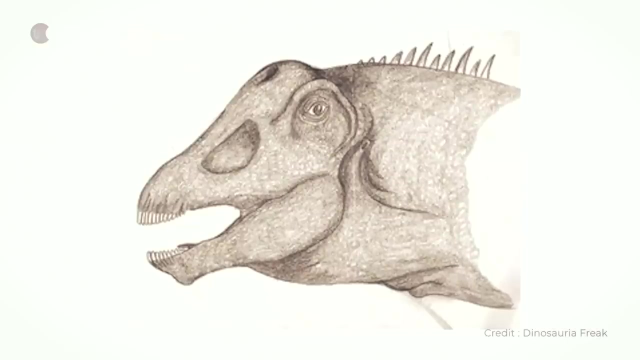 The Diplodocus is known throughout the world. It can measure up to 27 meters or 90 feet in length. Its skull is elongated and its snout is projected forward. Its nostrils are located more to the rear, above the eye sockets. 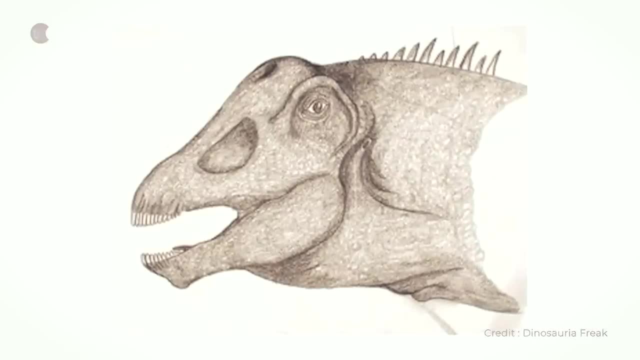 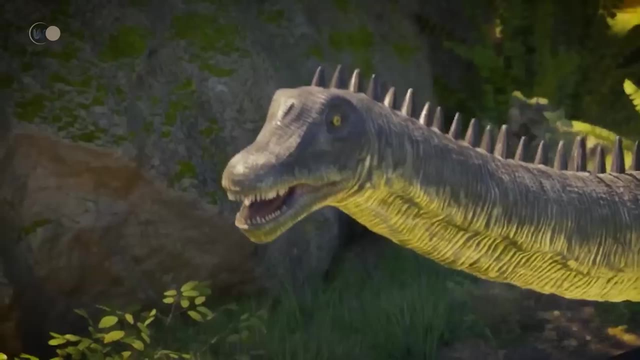 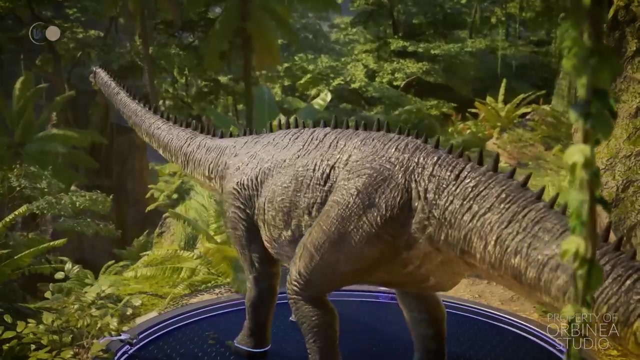 The air follows a complex path that allows the animal to meticulously analyze the odors of its environment. Its well-aligned teeth are located at the front of the jaw. When they wear out, they are replaced by new teeth. Its huge pelvis, reinforced with five welded vertebrae. 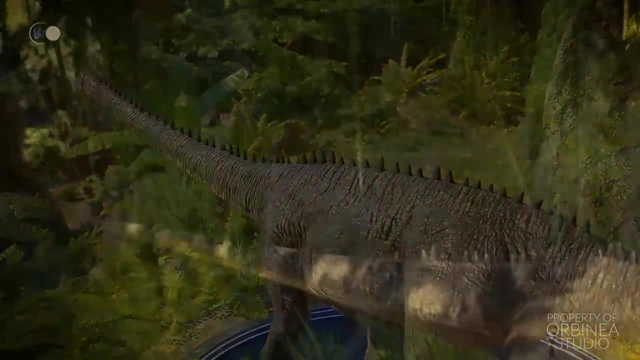 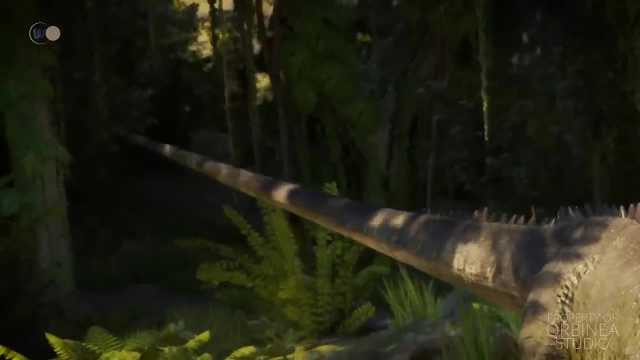 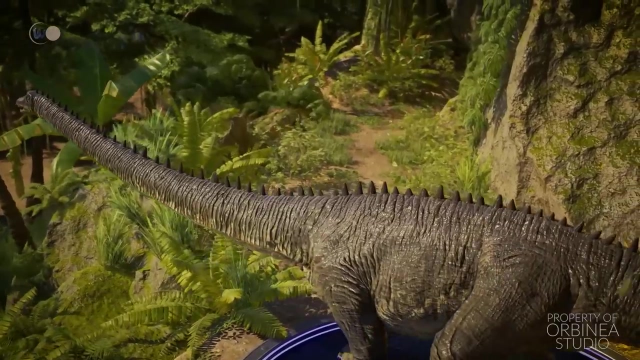 supports its weight of about 10 tons. Its long tail is used to counterbalance the weight of its neck. It ends in a tapered whip and allows him to use it as a defensive weapon by snapping it like a wind. Its neck contains 19 vertebrae. 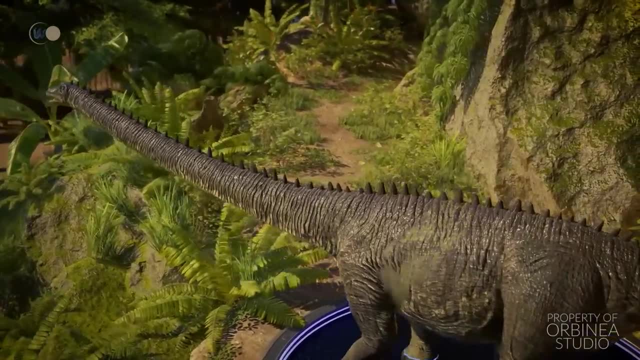 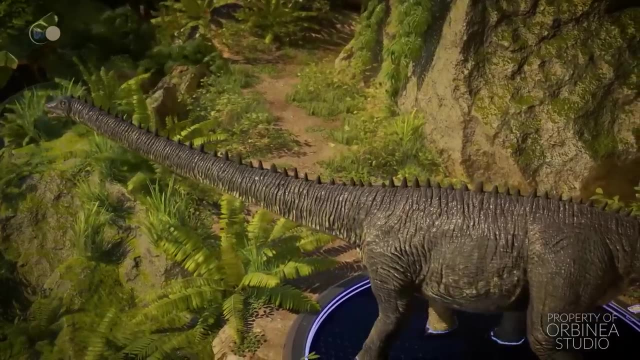 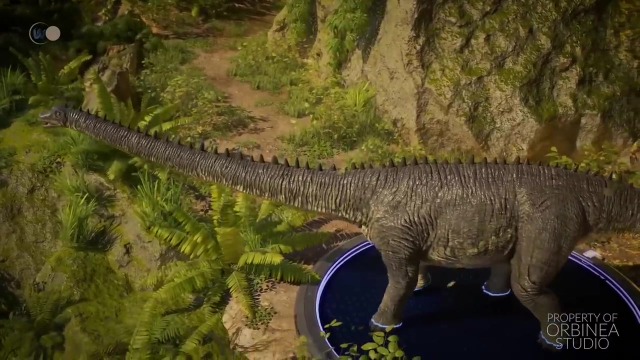 and can reach 15 meters or 50 feet in length. While being a giant can have advantages such as having access to more food and being able to defend themselves more easily, these animals are also forced to eat more than others and must support their own weight. 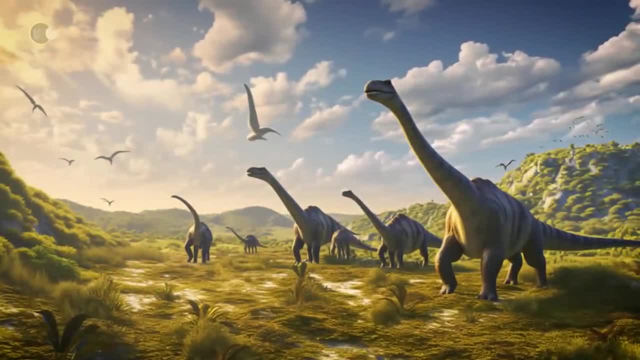 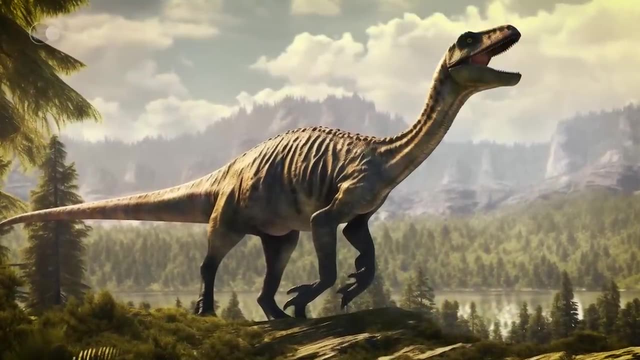 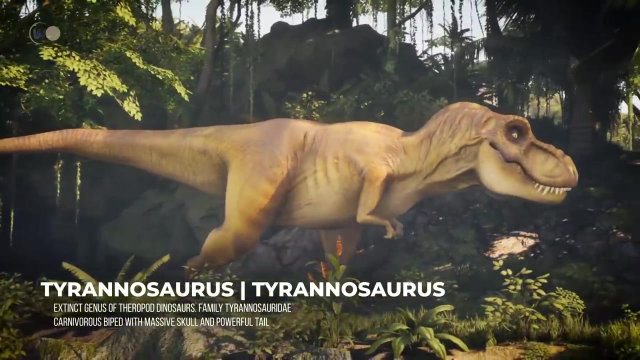 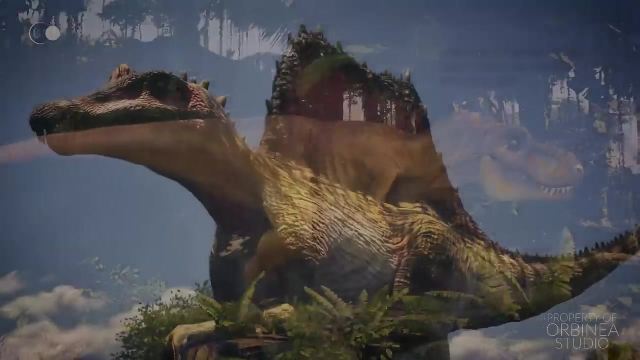 Against these herbivorous giants, carnivorous dinosaurs are very diverse, From large scavengers to small, agile predators. Tyrannosaurus is a true star of predation. Lesser known but equally powerful species live alongside it. The Spinosaur family is distinguished. 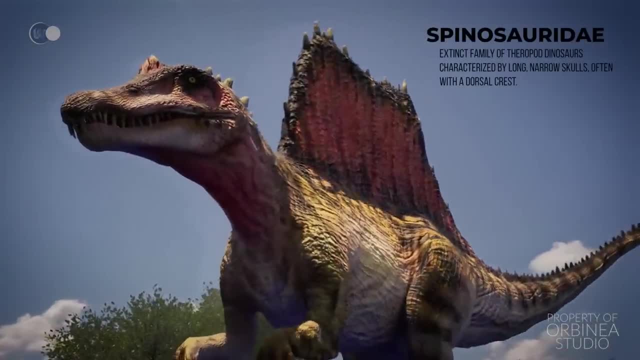 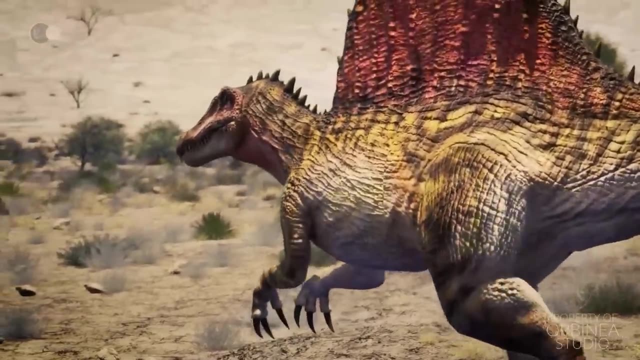 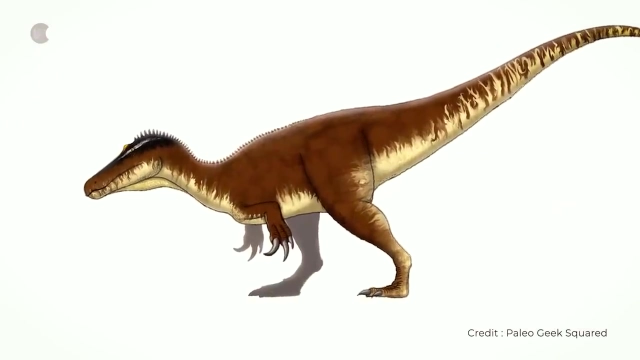 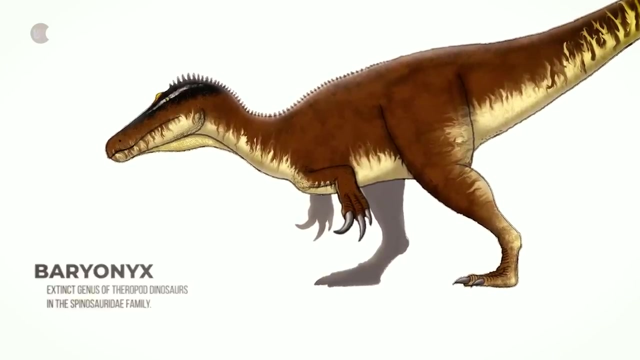 from other theropods by its long snout, numerous small teeth and thumb with an impressive claw. The Baryonyx is a Spinosaur measuring nearly 10 meters or 30 feet long. Its name means powerful claw. This large carnivore moves on two legs. 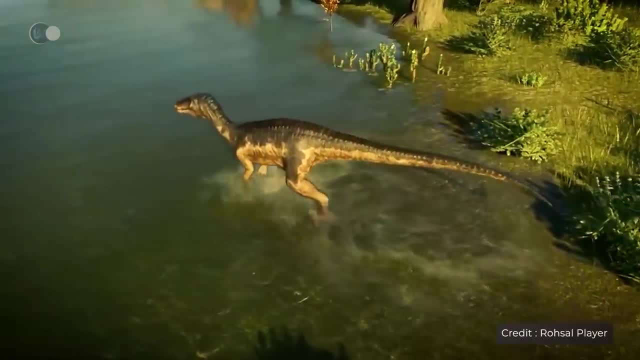 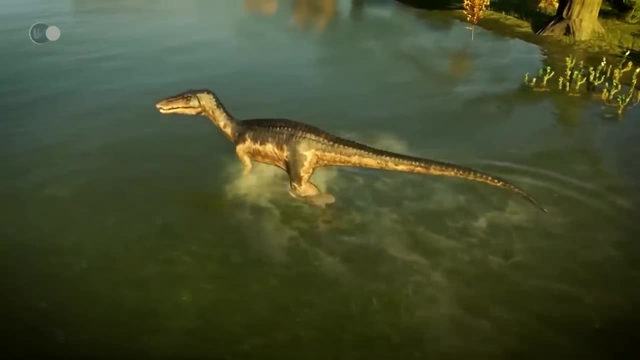 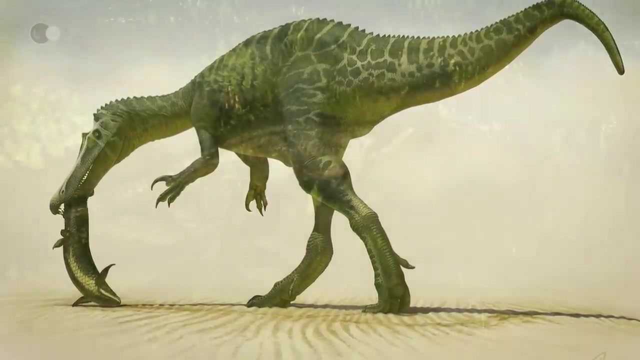 Although it is not completely aquatic, it spends a lot of time near water to hunt fish. Its powerful arms are used to catch and control its prey. His crocodile jaws make him a formidable predator. It does not only eat fish, It is also an active hunter of other land dinosaurs. 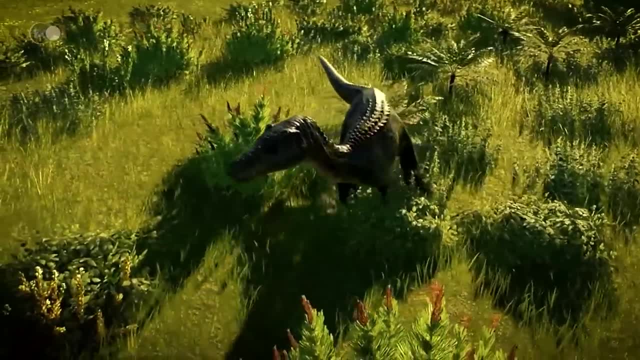 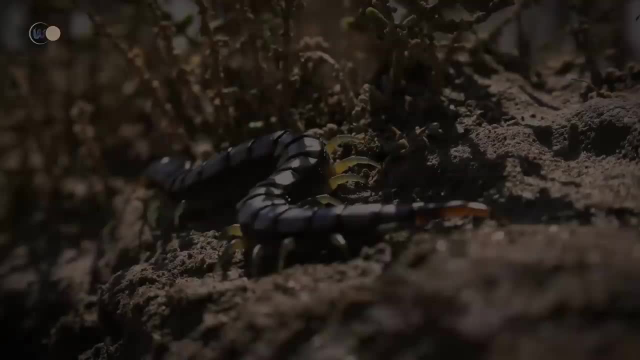 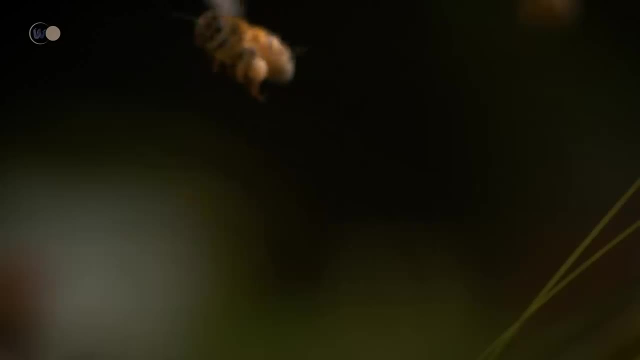 and a scavenger. It has a long tail that allows it to balance. The world of dinosaurs is teeming with insects that dig the earth, crawl on the ground or fly through the air. Bees, ants and butterflies appeared at this time. 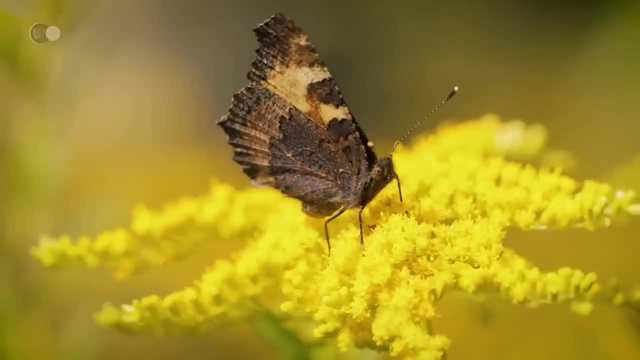 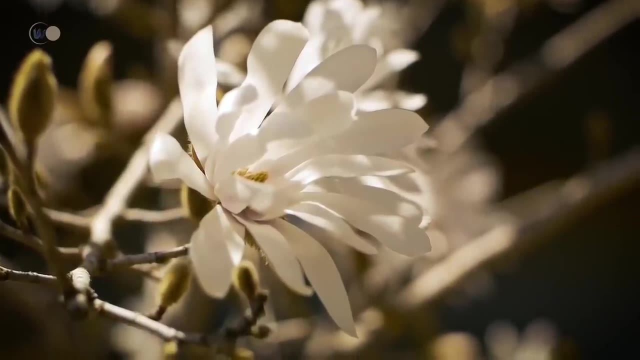 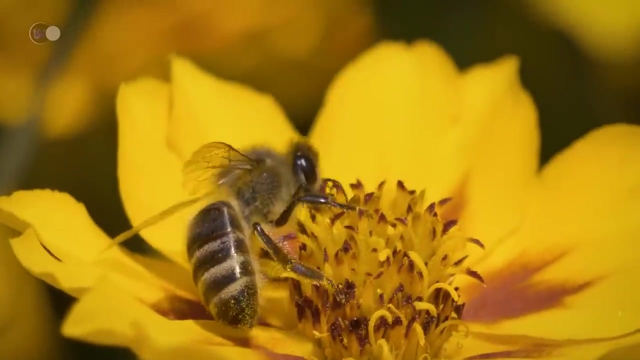 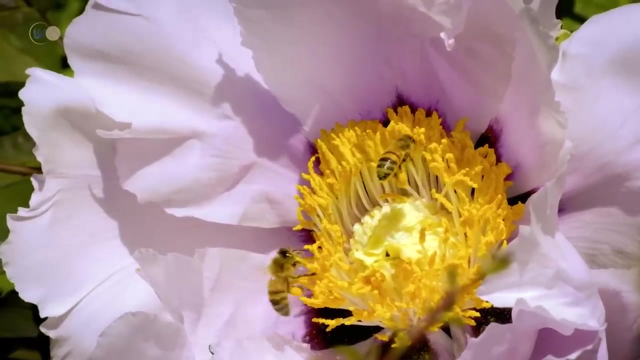 Under their tiny legs, the world is covered with flowers. The first flowers look like our modern magnolias with large petals. The flowers will then transform and specialize. The petals acquire various shapes and colors. The flowers produce a perfume which attracts insects. 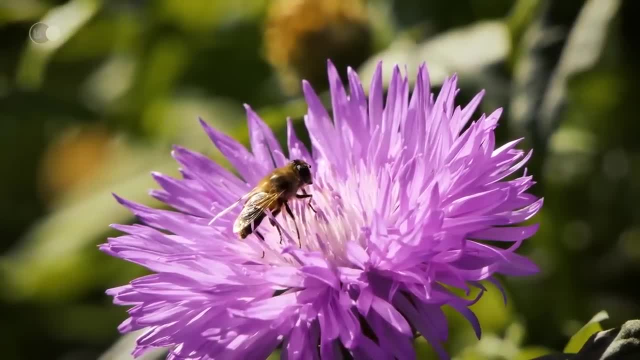 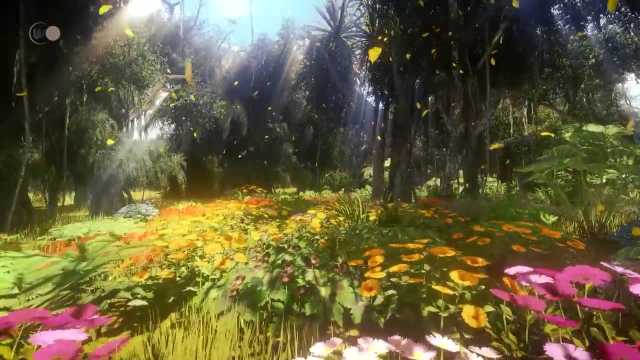 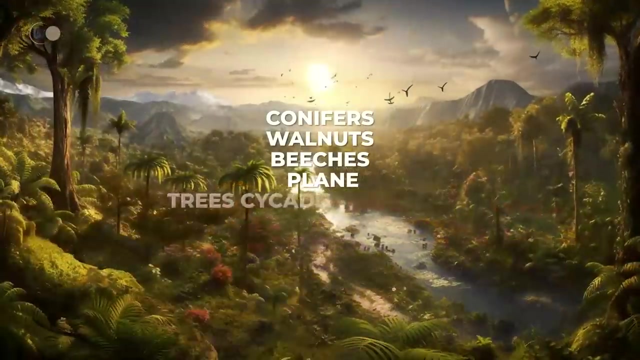 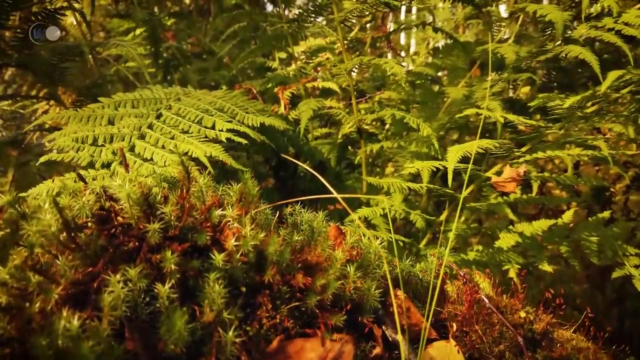 Insects will find nectar, a nourishing liquid, and pollen to consume. These flowering plants become dominant. They dress the landscape alongside conifers, walnut trees, beech trees, plane trees, cycads and tree ferns. The wind or the rain transport the pollen. 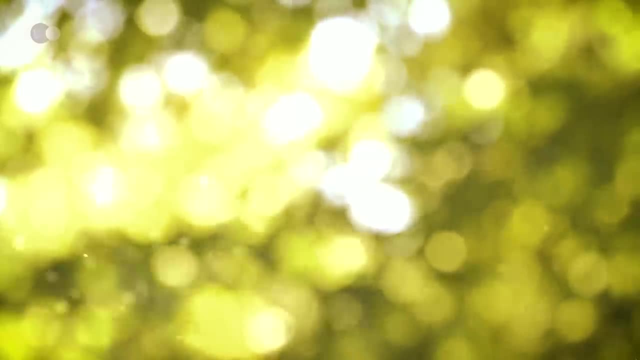 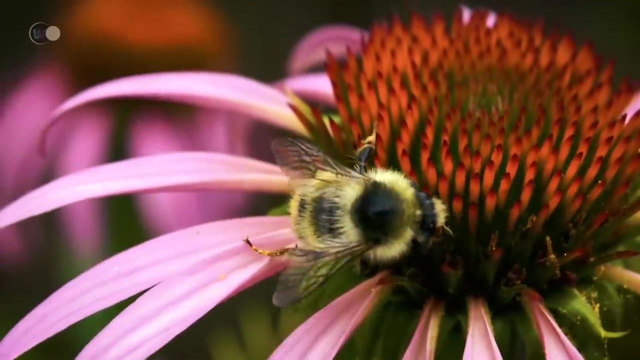 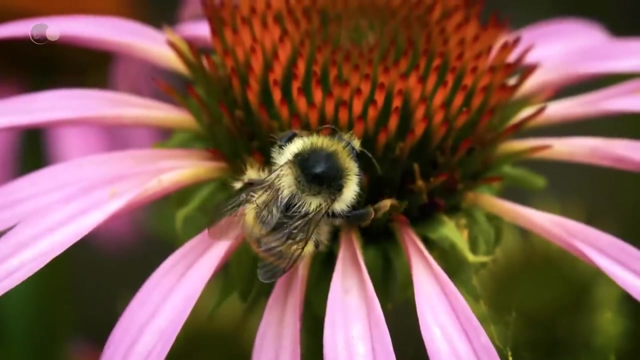 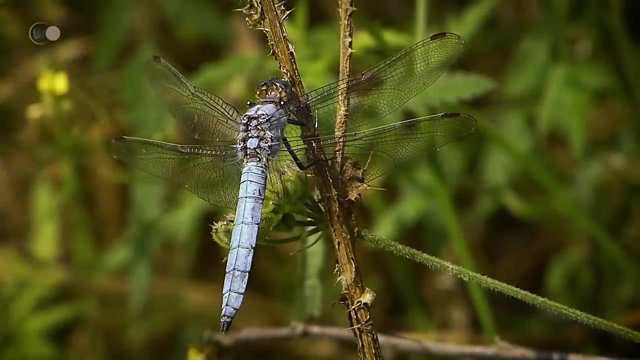 emitted by the male organs. These grains are carried at random to the ovules of other individuals To ensure the reproduction of the plants. Insects coming to feed on pollen carry it from flower to flower. The association between plants and insects becomes increasingly close. 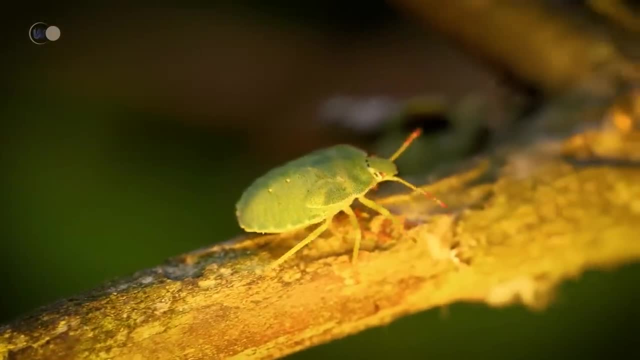 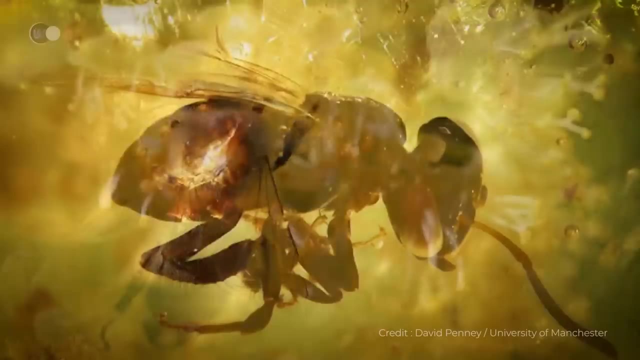 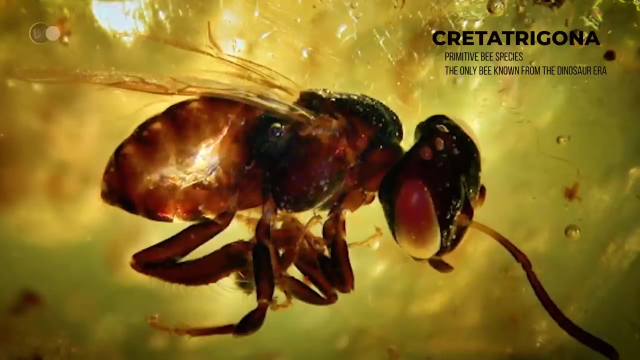 Dragonflies, cockroaches and bugs also appear. Creta trigona is the one known bee from the dinosaur era. It looks very much like some of today's tropical bee species. It has special bristles on its leg that are an adaptation for pollination. 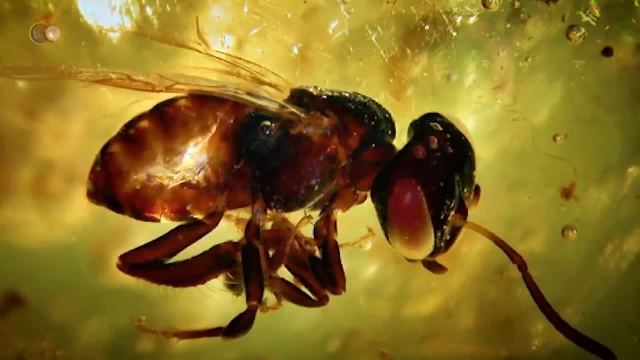 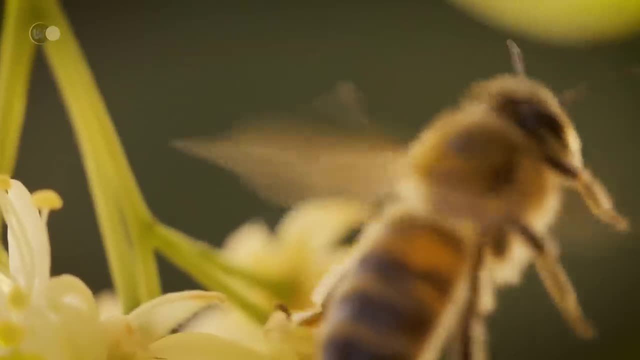 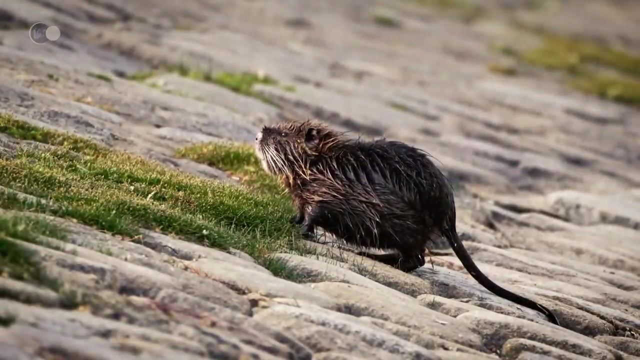 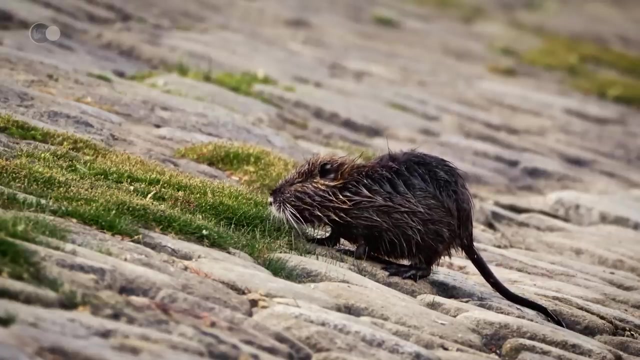 since they fix the pollen when it lands on the plant. Mammals, although modest and reserved, live alongside the dinosaurs Like tiny, fearful critters. these primitive creatures thrived and diversified within extremely severe limits. Dinosaurs and reptiles occupied most. 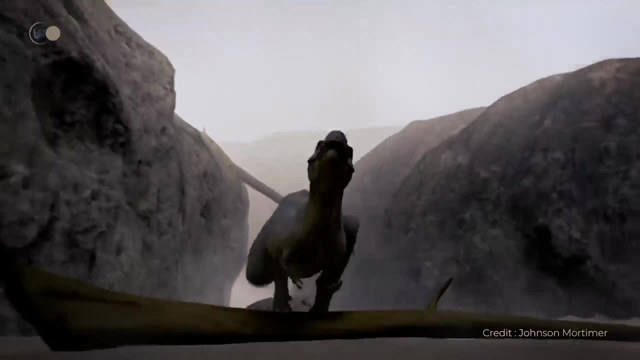 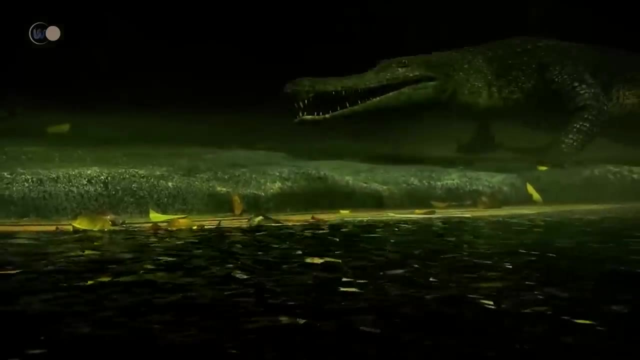 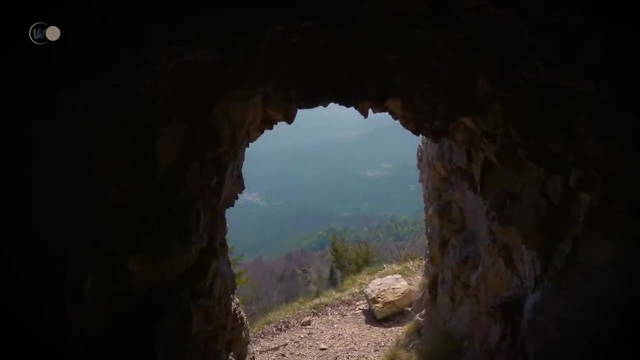 of the ecological niches and left very little space for other creatures. They are left to survive in caves, grottoes or in hollows in trees and under the ground. Constraints on their size and their way of life have naturally imposed themselves. 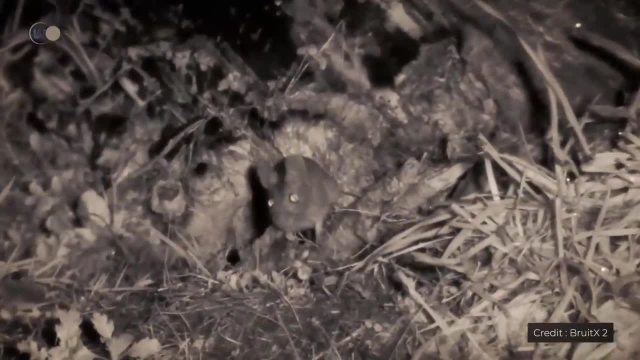 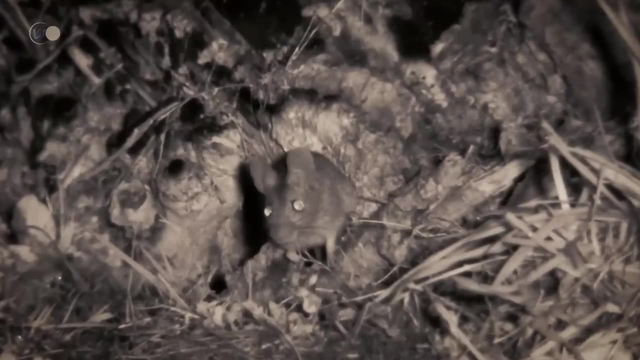 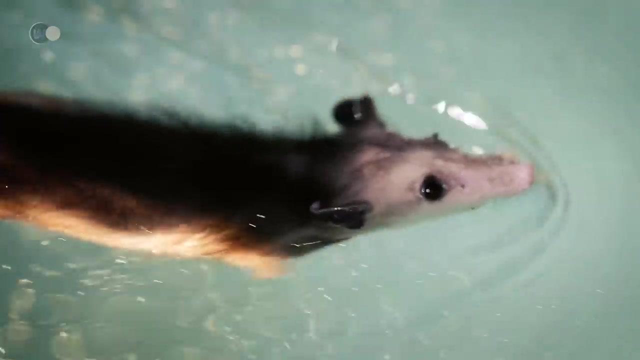 Reptiles being less active at night, mammals have adapted to a nocturnal life. They have good eyes, good ears, a good sense of smell and whiskers to sense their way. The intensive functioning of all sense organs requires a larger brain than that of reptiles. 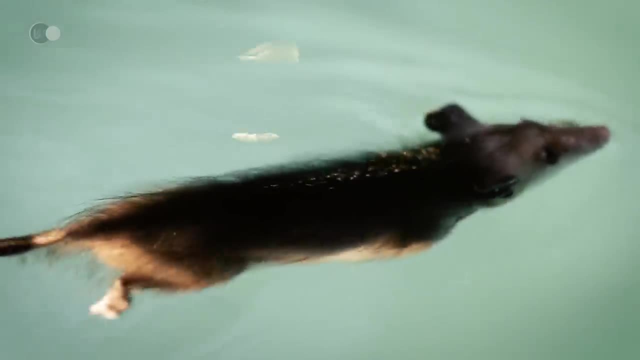 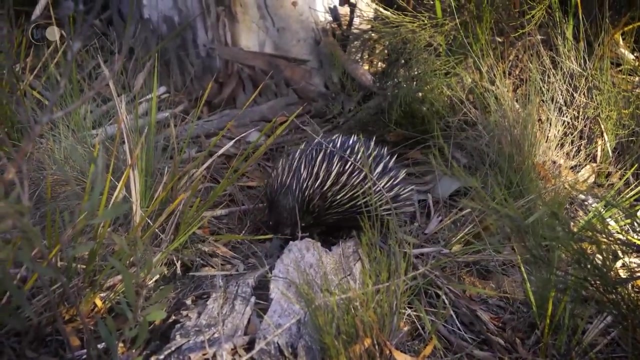 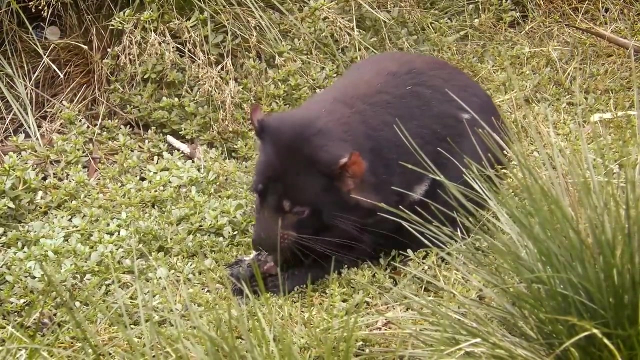 The energy burned by the brain must be constantly renewed. Warm blood and insulating coat appear, Mammals will prioritize protein-rich foods. They feed on insects, other invertebrates and plant seeds In order to release energy very quickly and to digest food quickly. 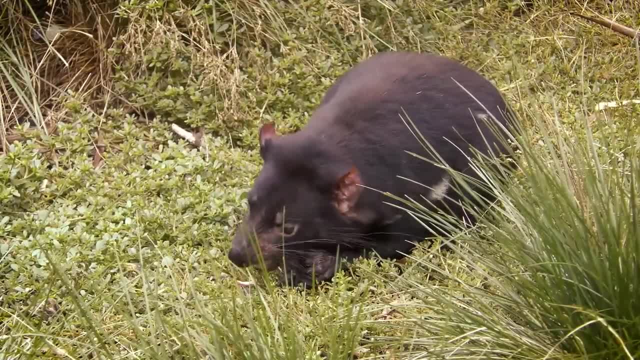 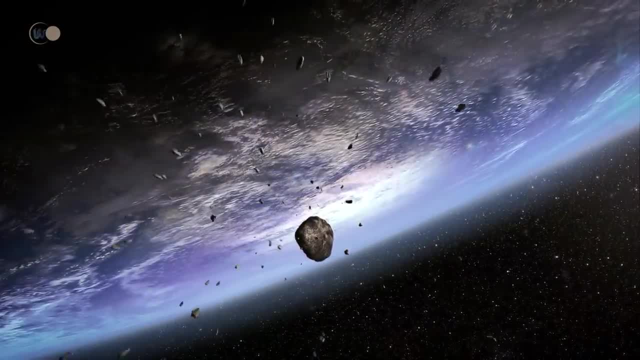 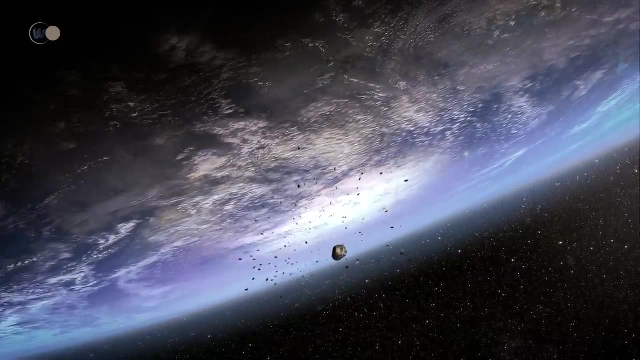 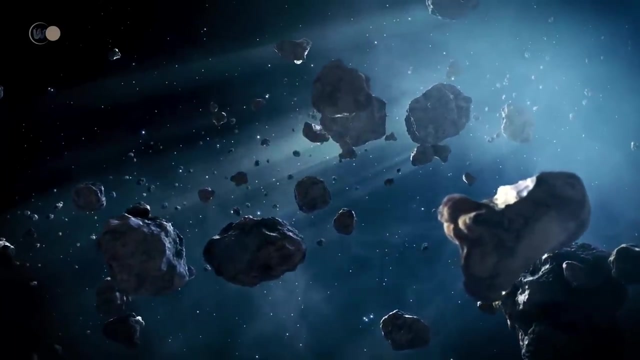 sharp teeth appear. They can catch, kill, grind and crush food. Life as it is at this time will be turned upside down by a cataclysm. The meteoric impact that took place at the Cretaceous-Paleogene boundary is a perfectly established fact of Earth history. 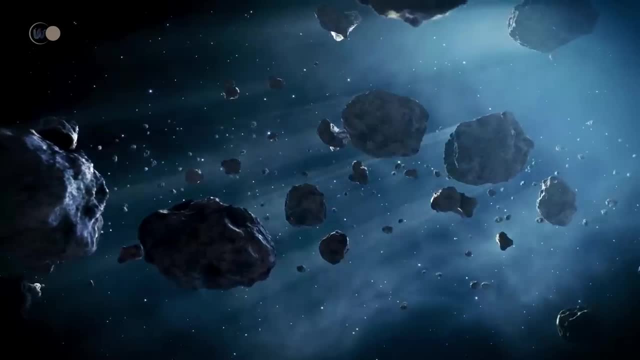 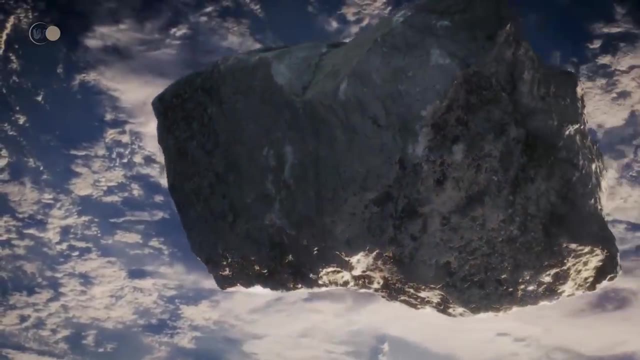 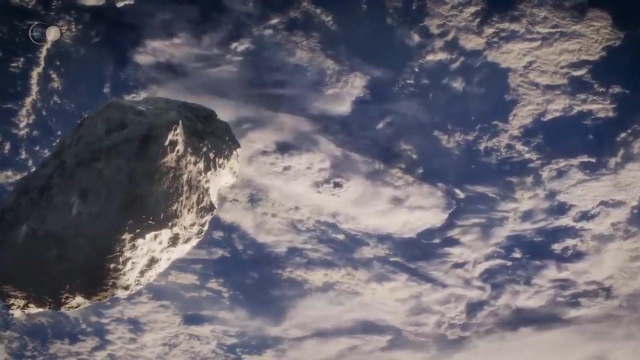 A huge asteroid the size of Everest hits the atmosphere At an exceptional speed of nearly 65,000 km per hour, or 40,000 miles per hour, With its diameter of more than 10 km or 6 miles and its weight of a billion billion tons. 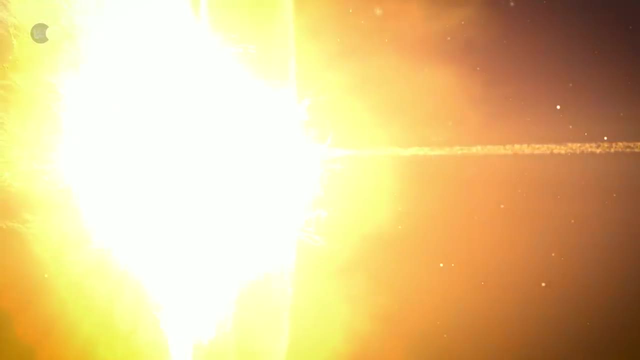 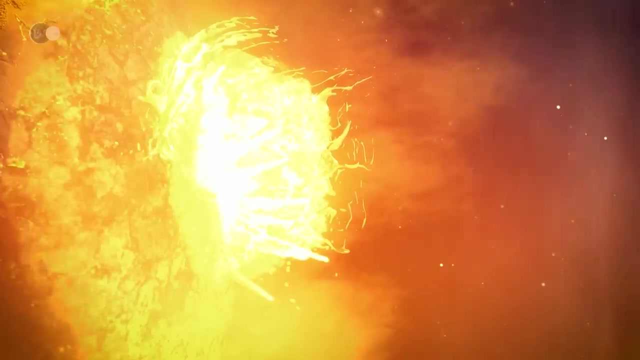 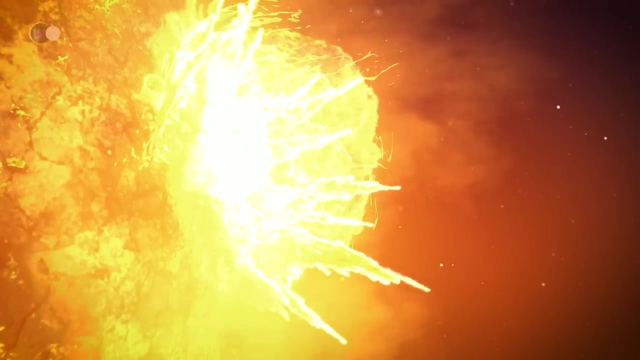 it smashes into the province of Yucatan in the Gulf of Mexico. The energy released is immeasurable. This asteroid hits the mainland and forms a crater 30 km or 20 miles deep. The impact is so great that the rock of the Earth's crust liquefies. 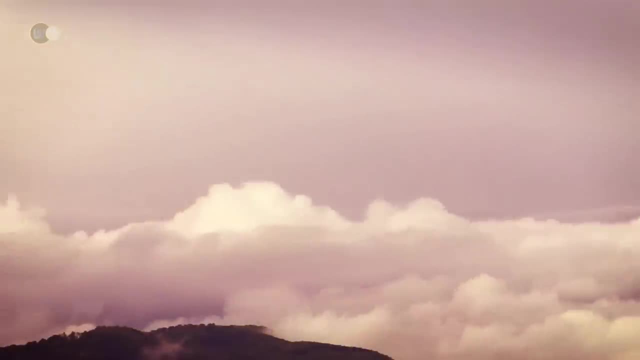 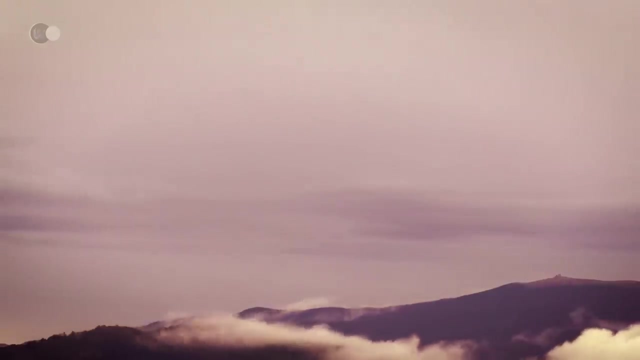 Within a radius of 60 km or 40 miles around the impact. all the existing water is transformed into vapor. The thousands of animals that were there at the time are killed immediately. Everything happens so fast that they don't even have time to feel anything. 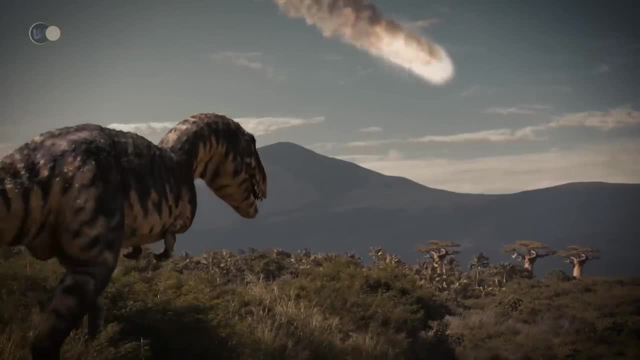 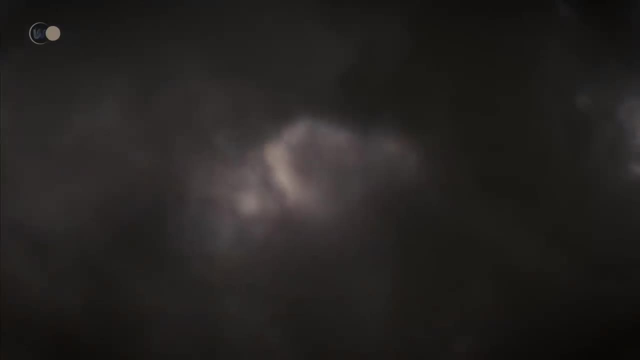 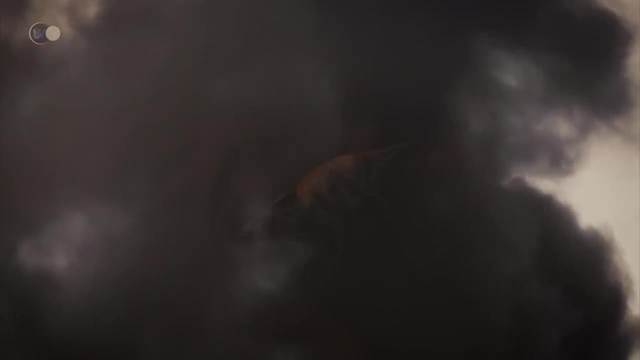 These animals die a gentle death, but not those further away who only see a flash of light. A few seconds after the impact, the shock wave takes shape like a cloud of vaporized rocks which advances quickly on the ocean. The unbearable heat evaporates everything around. 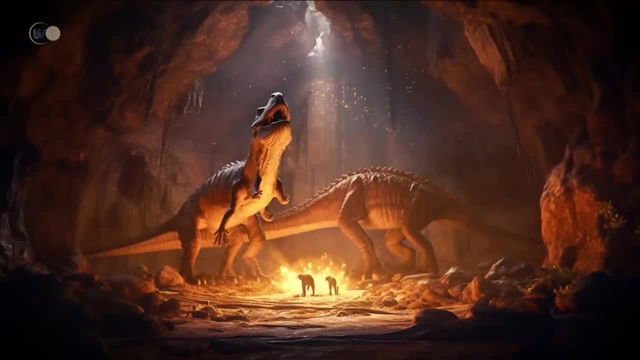 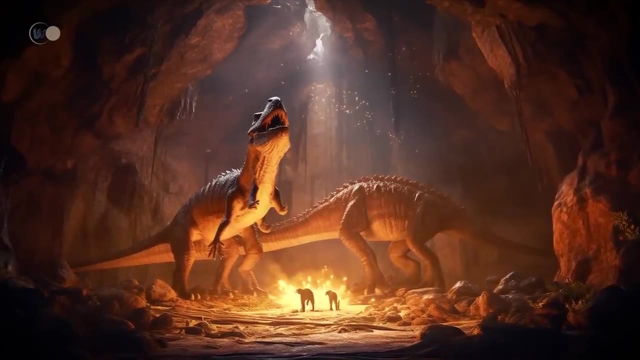 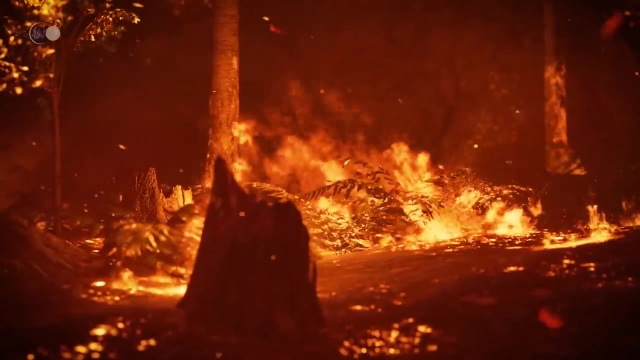 Most animals are killed by the violence of this wave. The most vulnerable are those who can't find shelter quickly. The animals living in caves on the side of a hill and being able to take refuge in a safe place have a chance of survival. Fires break out. 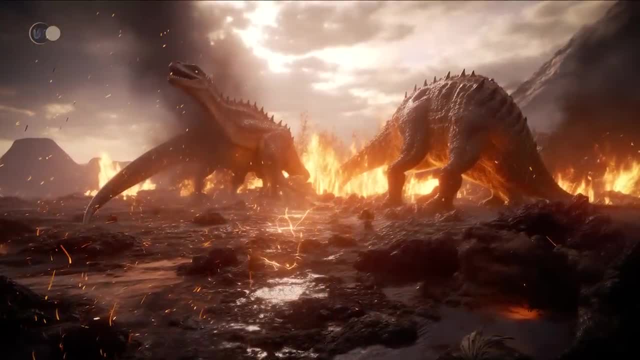 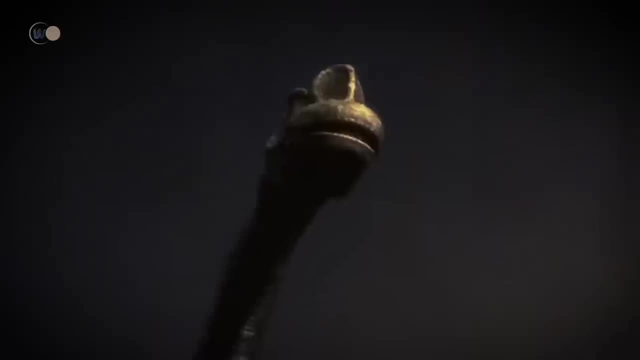 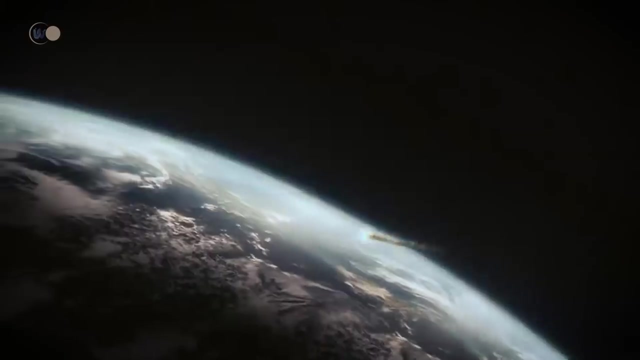 The Earth goes up in smoke. Dinosaurs, because of their gigantic size, have a lot of difficulties to find a refuge and are vulnerable. The shock wave releases all its energy in about 10 minutes, but it did not cover the whole surface of the Earth. 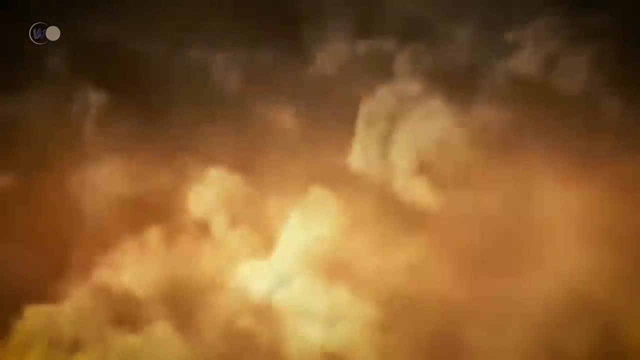 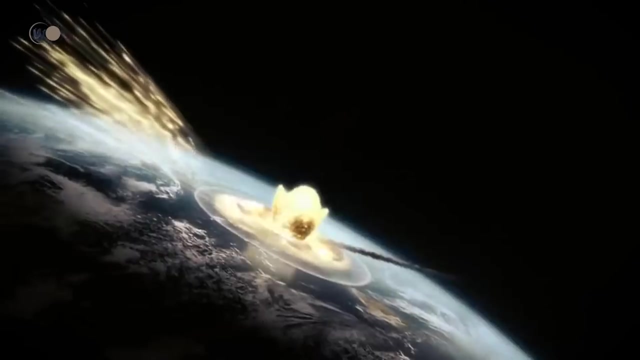 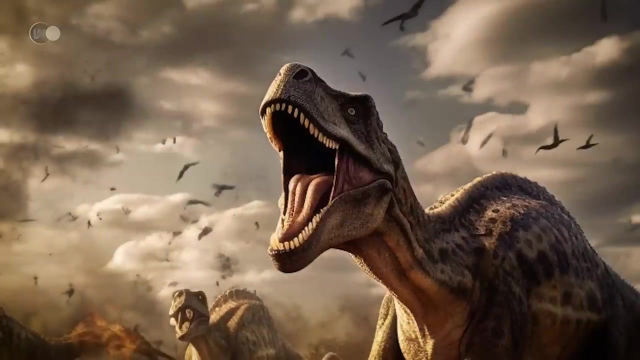 Some animals are unaware of the catastrophe that has just occurred. The consequences will catch up with them. The impact of the meteorite causes a major earthquake. A violent tremor is felt, Cracks appear and landslides occur. The earthquake crosses the whole planet. 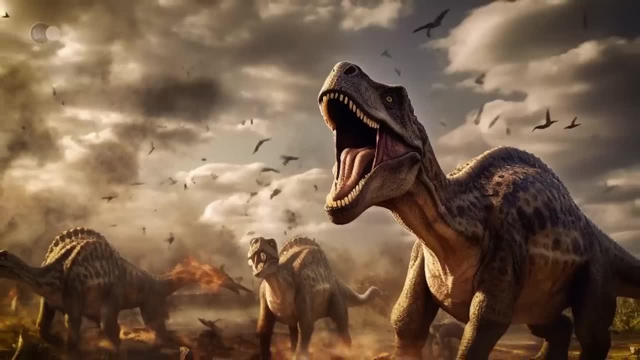 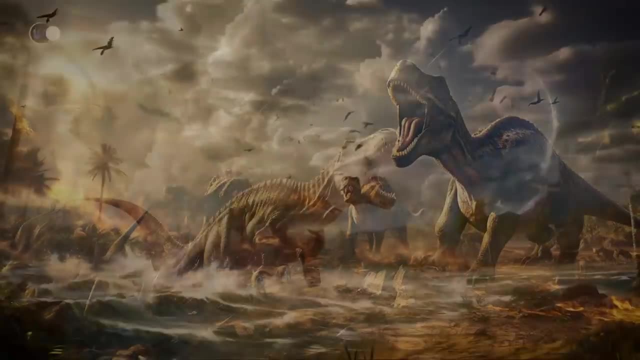 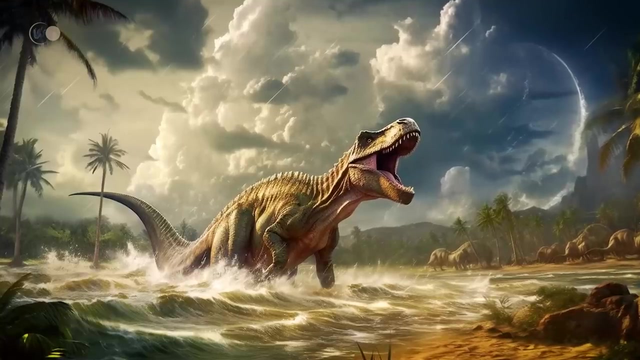 The tremors of the earthquake are felt for several days, but the worst is yet to come. A giant tsunami, as big as a mountain range, advances towards the coast. It crossed the Atlantic at almost 1,000 kilometers per hour, or 620 miles per hour. 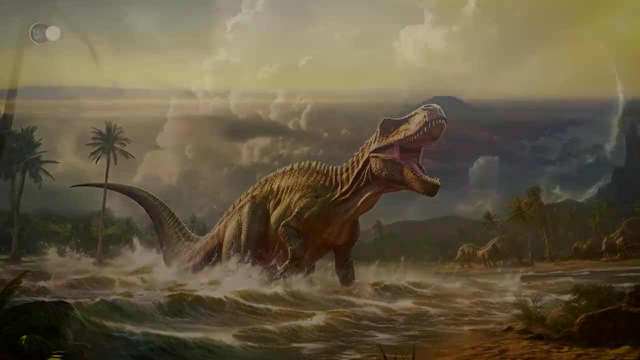 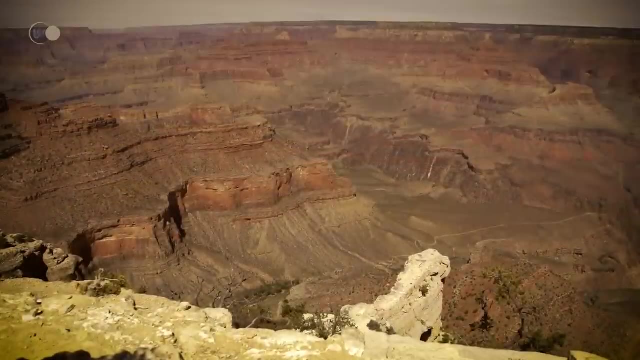 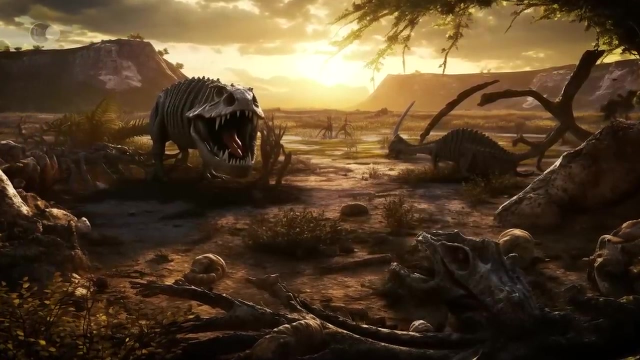 The wave comes close to the coast and then crashes on land, carrying animals, trees and debris in its path. It then retreats with such force that it shapes a new geological landscape: Hills, valleys and canyons are formed. Dead animals are scattered. 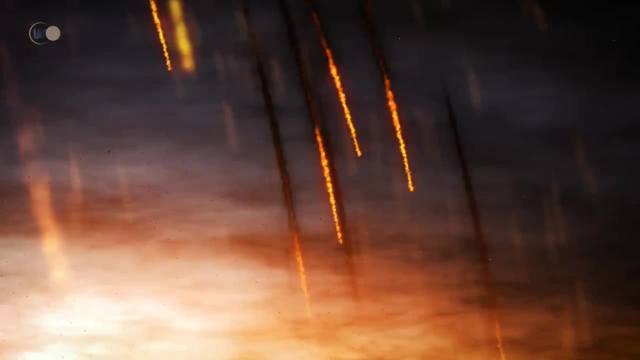 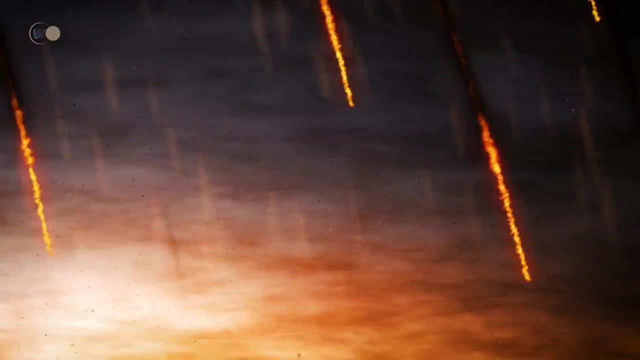 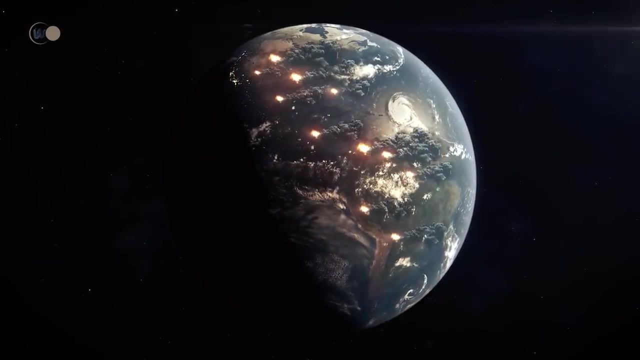 or washed back into the sea. The tsunami subsides, but the millions of tons of rock that were propelled into space by the impact now fall, as meteorites ranging in size from a pea to a house Boulders hit the surface of the Earth. 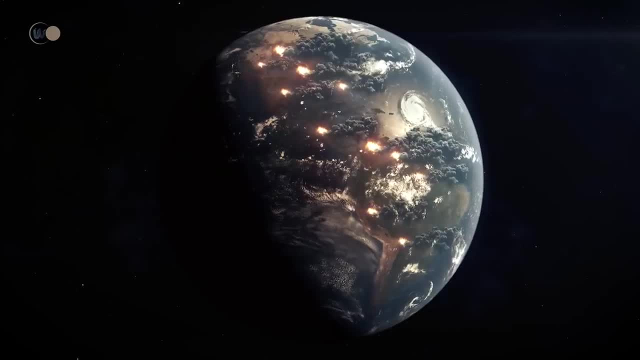 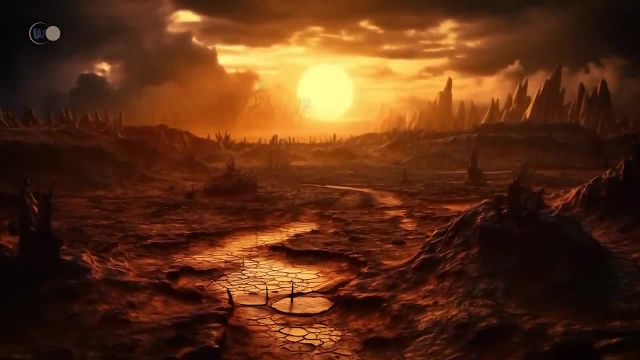 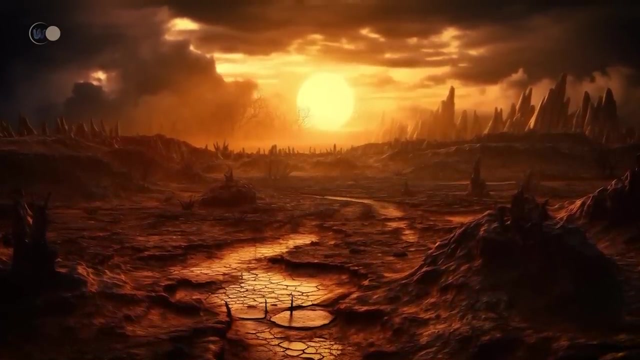 for several hours, causing the temperature to rise sharply. In less than a day, the cataclysm exterminated almost all the life on planet Earth. Millions of animals are burned alive, Oxygen levels rise on the Earth, The heat increases and the burning accelerates. 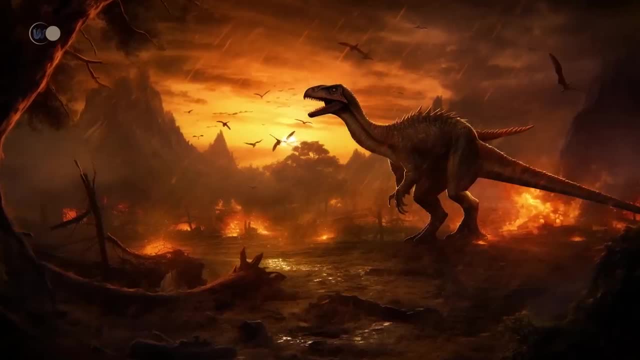 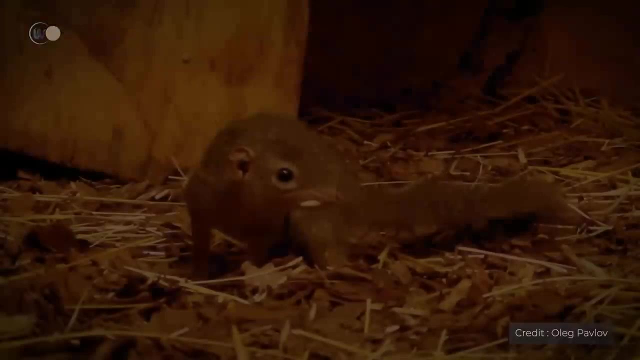 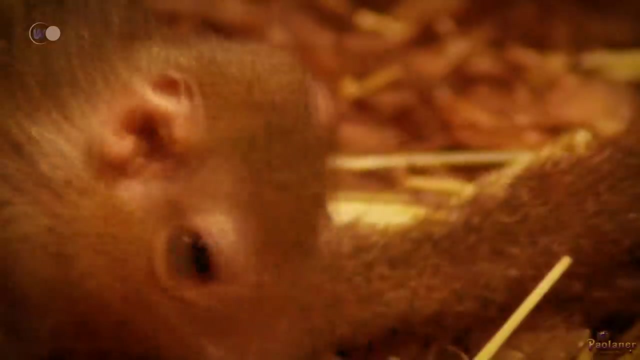 Amidst the corpses, a few survivors persevere. A few isolated dinosaurs still roam the apocalyptic landscape trying to survive. The Purgatorius, an ancestor of today's primates, wanders through the flames While for millions of years, 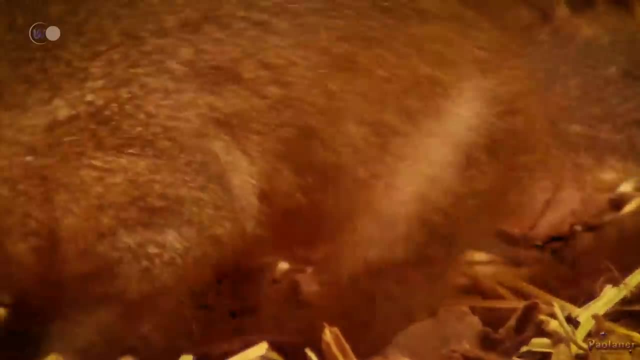 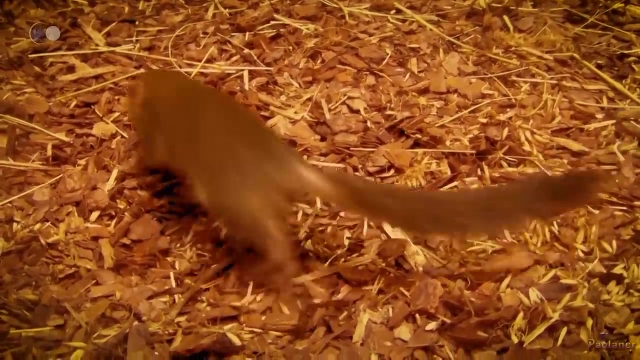 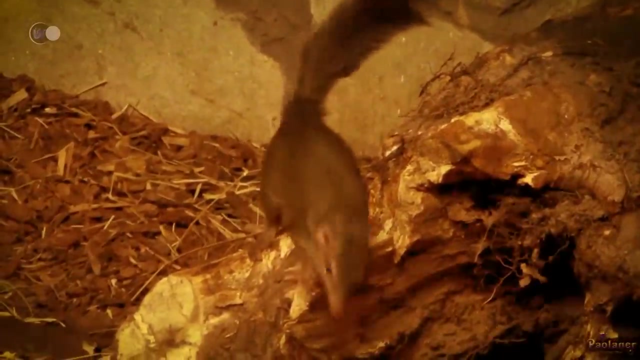 it has been preyed upon by dinosaurs. it seems that its physical conditions give it an advantage in surviving the catastrophe. This small mammal is similar to a large mouse that climbs trees. It is at the base of a group that led to species including the great apes and man. 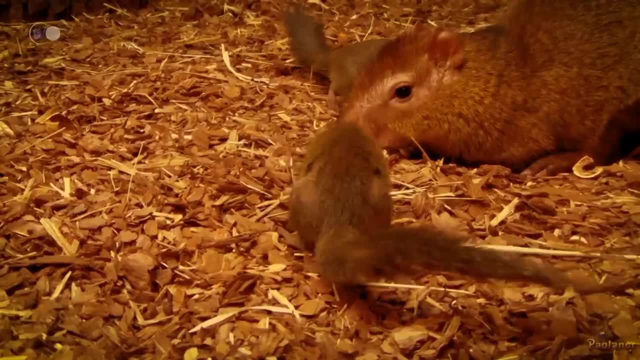 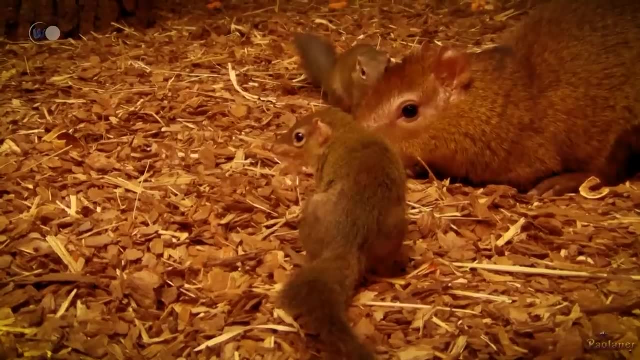 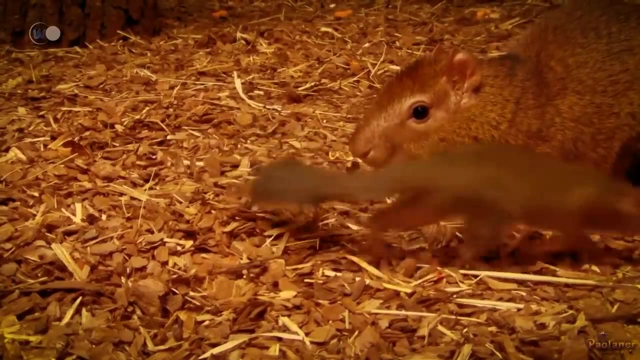 This small animal lived in the shadow of the dinosaurs. It organized its life discreetly by feeding on insects and fruits found in forest habitats. It can now take advantage of the ecological niches left free by the dinosaurs to diversify Clouds of ash and chemical elements. 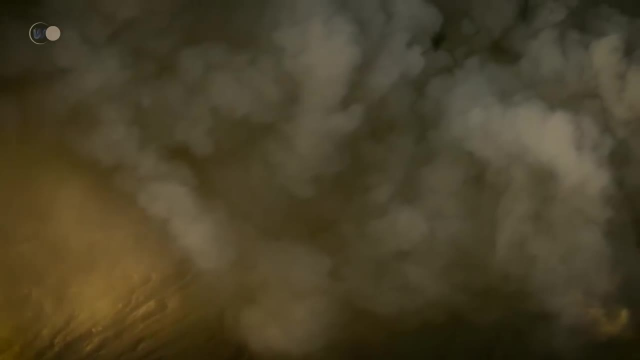 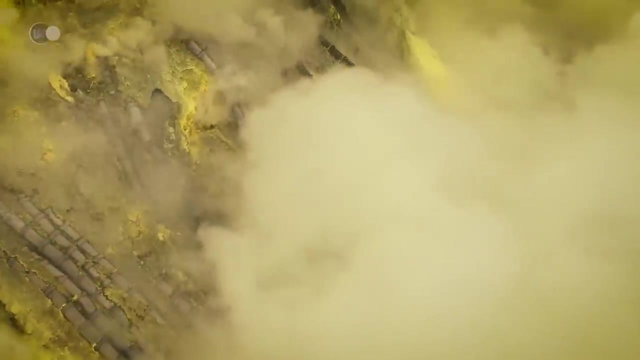 released during the impact clump together and gradually veil the sky. Sulfur was produced in large quantities during the impact. This element now comes into contact with the water in the atmosphere and is transformed into sulfuric acid. A deadly rain falls on the earth. 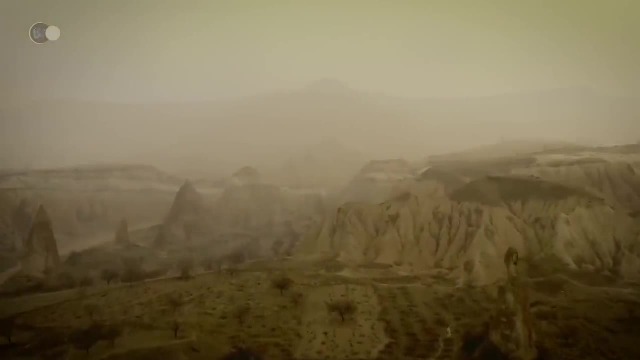 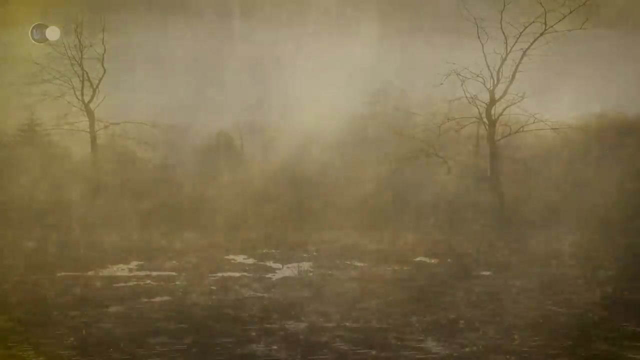 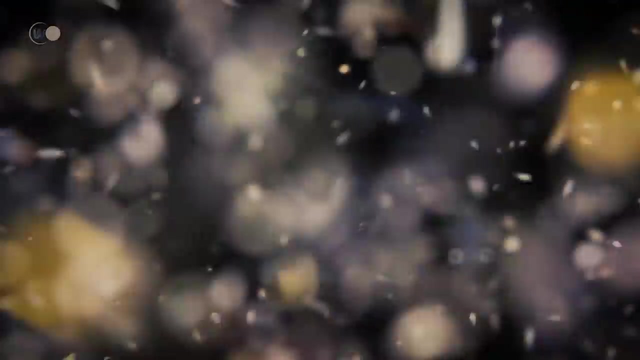 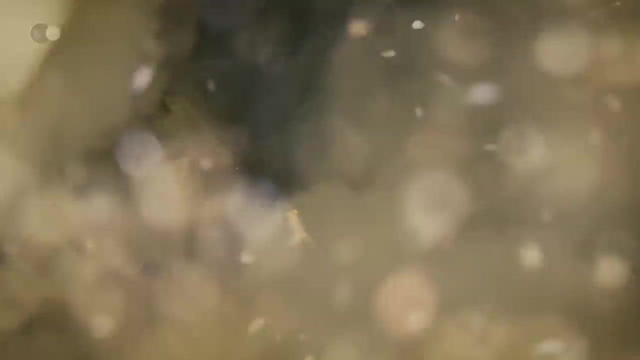 The surviving animals must take shelter because the sulfuric acid burns the skin and flesh. The showers also hit the ocean. The clouds present in great quantity gradually mask the sunlight. The earth is plunged into darkness. The plankton that needs constant light is slowly dying out. 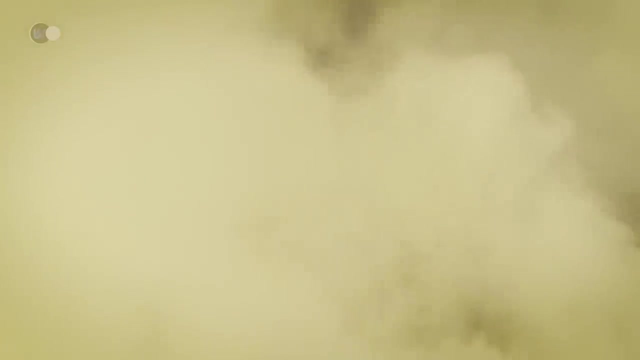 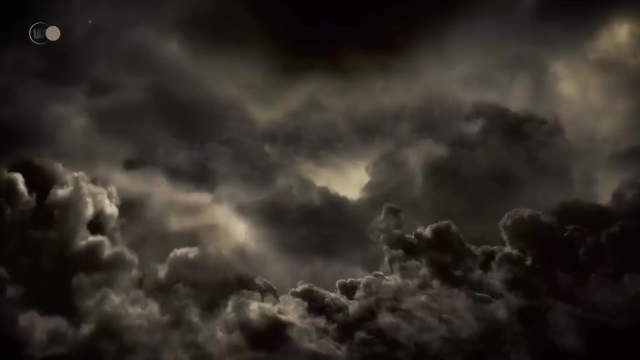 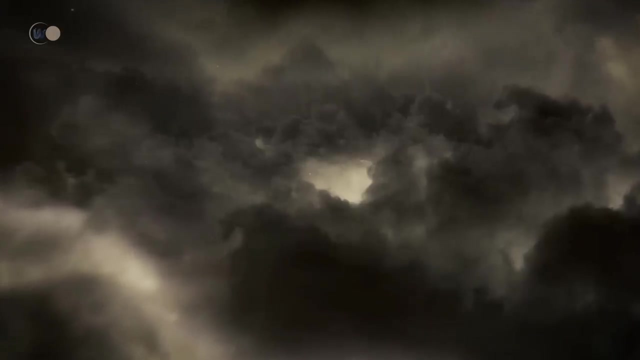 The dinosaurs, which use their visual sense for the most part, are heavily handicapped by this new condition. Darkness will reign for several weeks. The small mammals that lived alongside the dinosaurs had already developed nocturnal faculties. Indeed, they hunted mostly at night. 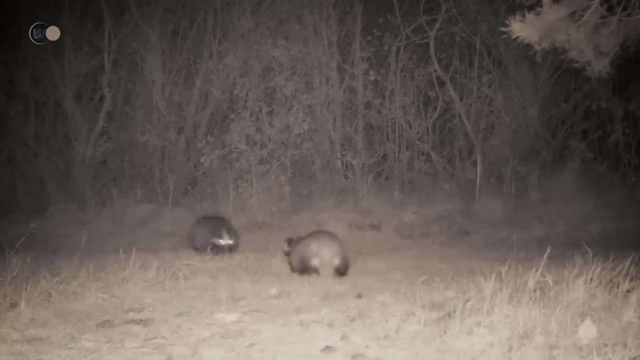 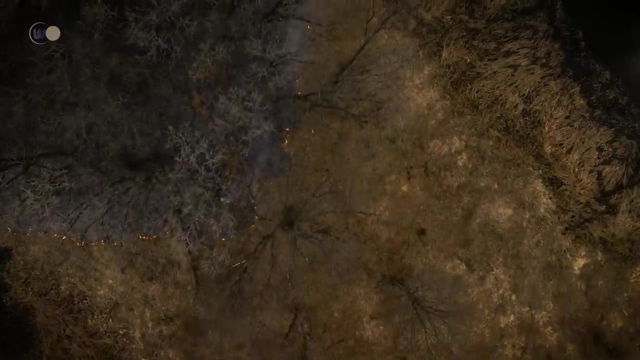 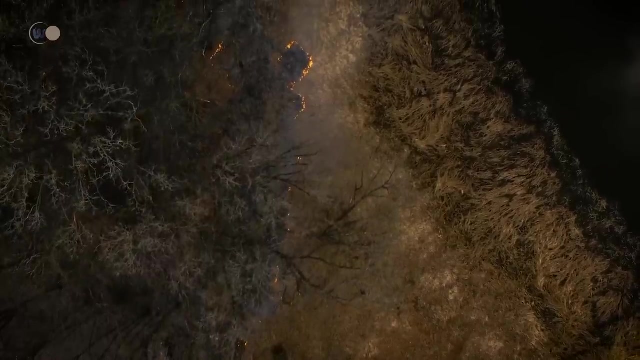 to avoid being preyed upon by the giants. They therefore have a major advantage in facing the interminable night that sets in. The vegetation also suffers the effect of the cataclysm. The plants that had not yet succumbed to the fire are now deprived. 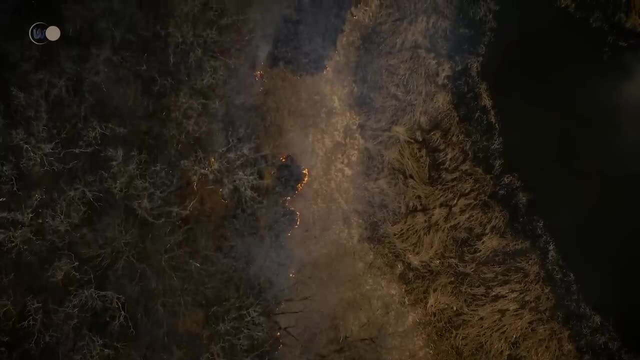 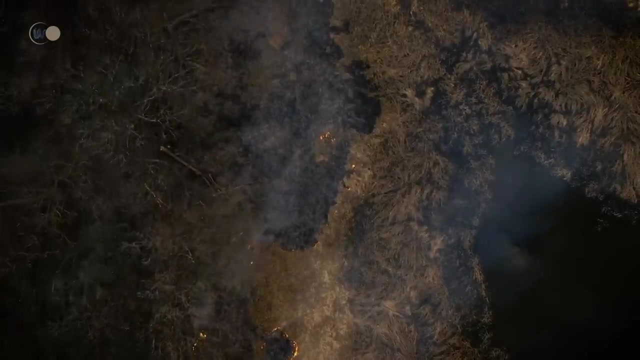 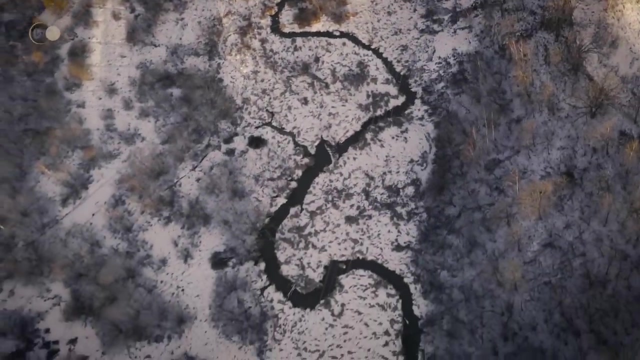 of sunlight and stop growing. The large herbivores that survived until then see their food sources diminish After a few months. a cold snap sets in The earth. once warm and lush, becomes icy and hostile, The Purgatorius isolates itself. 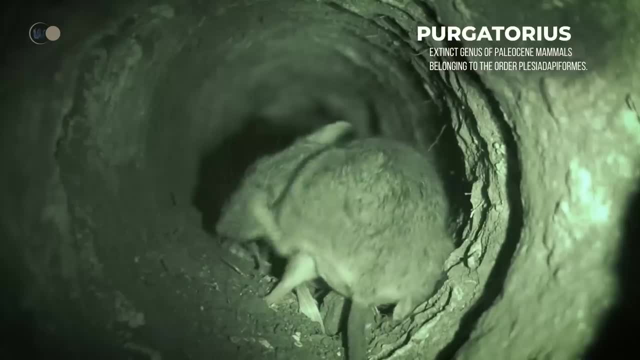 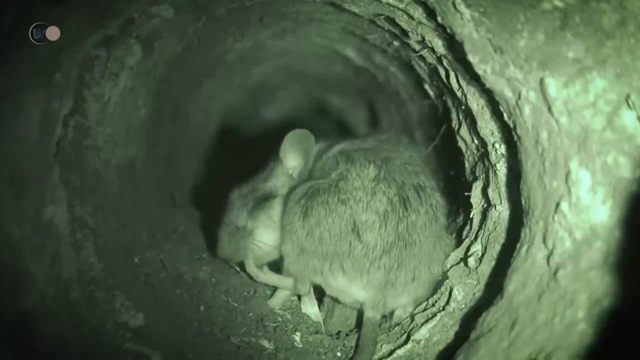 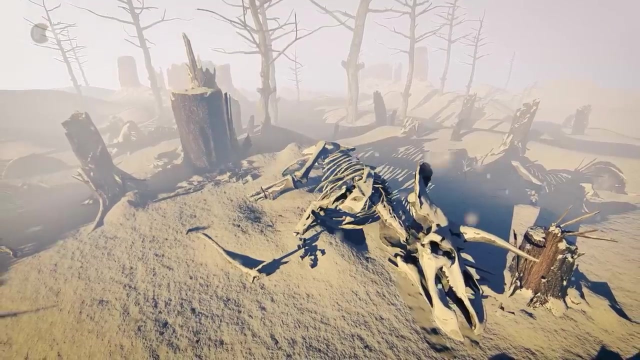 in its burrow to stay warm. It feeds on everything it finds, and this is what will save its life. All the dinosaurs, whether herbivores or carnivores, succumb to this icy environment, Except for the avian dinosaurs In one year. 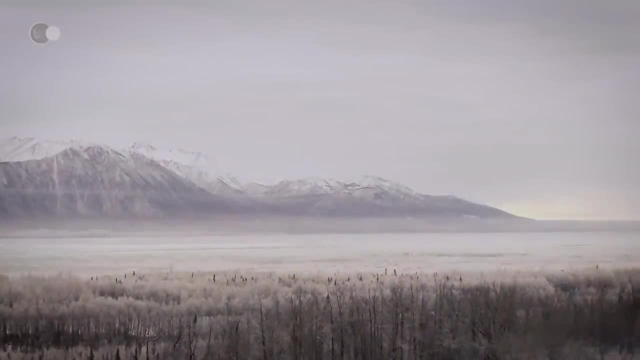 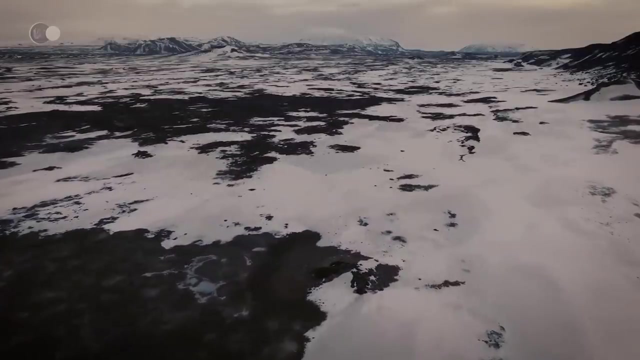 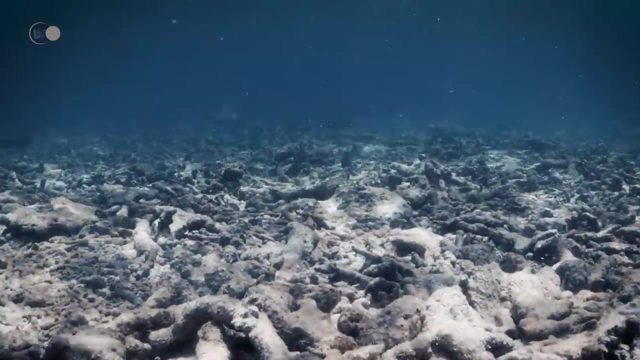 the planet is almost entirely emptied of all life forms. 75% of the species that populated the biosphere disappear. The ocean is empty, except for a few rare species of fish and sharks. Generally speaking, the smaller the animals were, the more likely they were to survive. 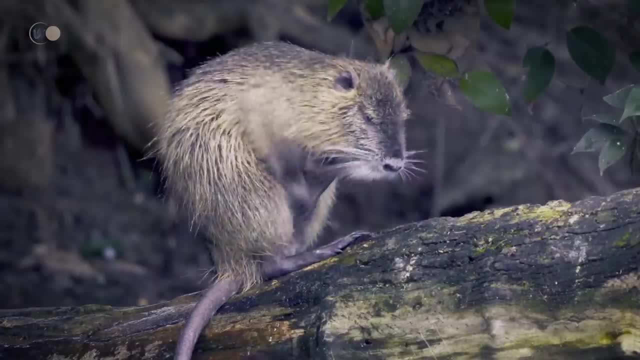 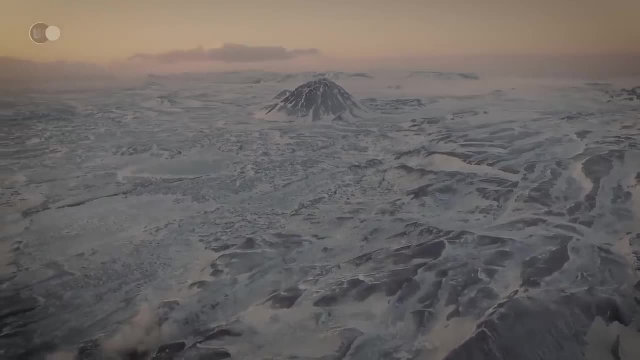 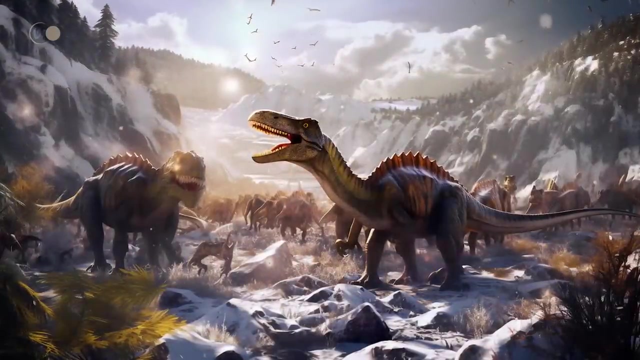 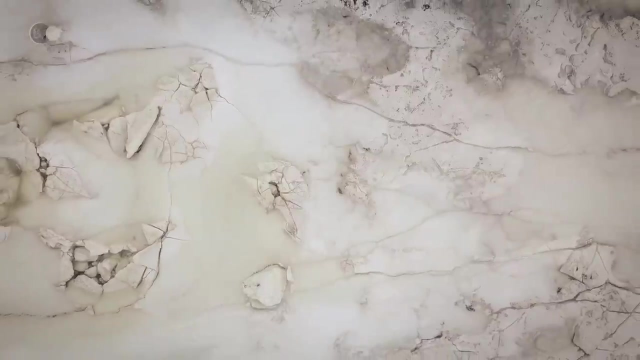 In a few hours, a few days, a few months or maybe a few years, the world of the dinosaurs collapses, implying a fundamental change in the ecosystem, since their disappearance will open the way to our distant ancestors. The earth is like a huge desert. 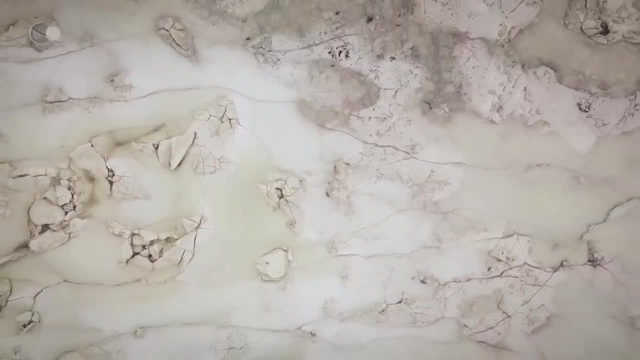 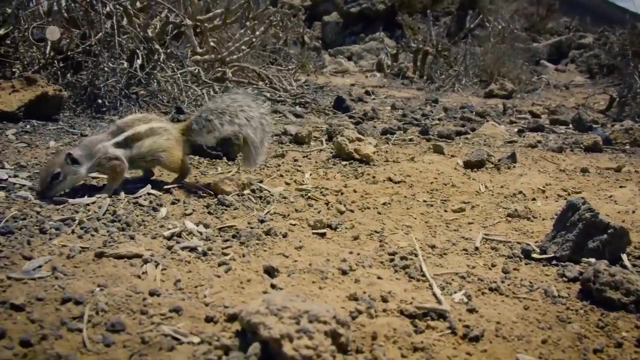 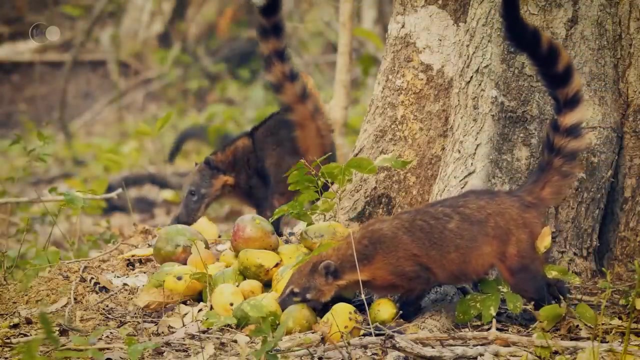 Nevertheless, for the few land animals that survived, it is a new opportunity. Without predators to hunt them down, these few survivors will be able to multiply rapidly, With no more reason to hide. they are ready to settle and repopulate the earth. 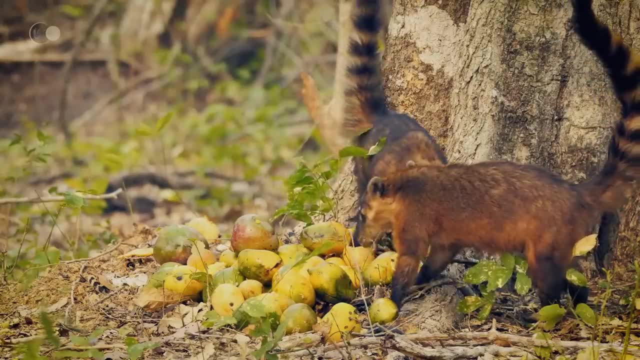 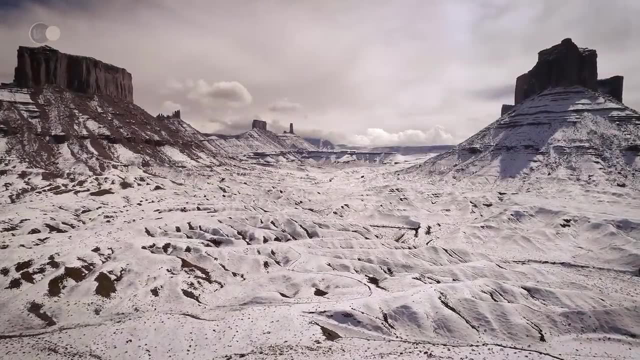 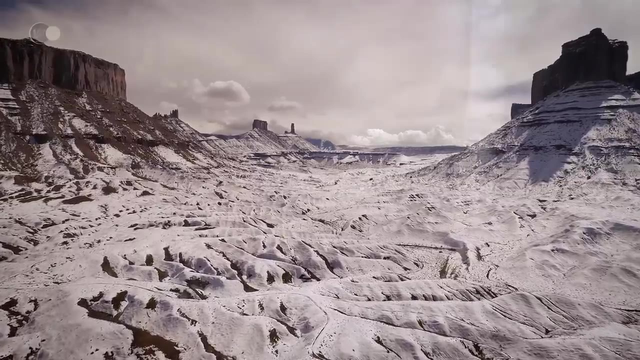 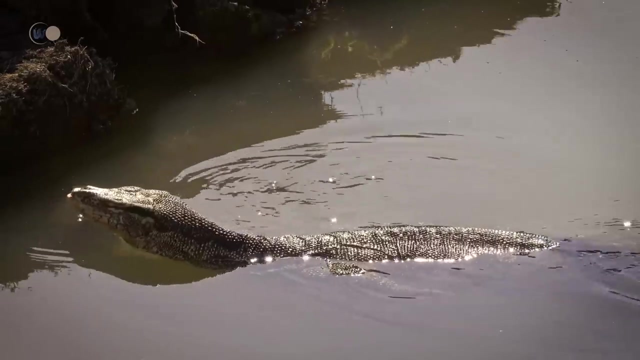 The survivors will write a new chapter in their history. The large reptiles disappear from the face of the earth. Other orders survive with very small populations. Four orders of reptiles remain, with turtles, crocodiles, snakes and lizards. 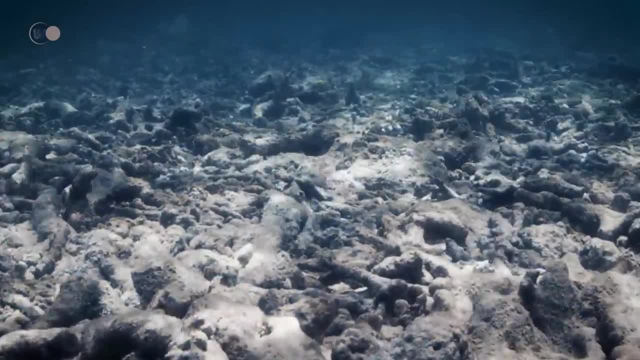 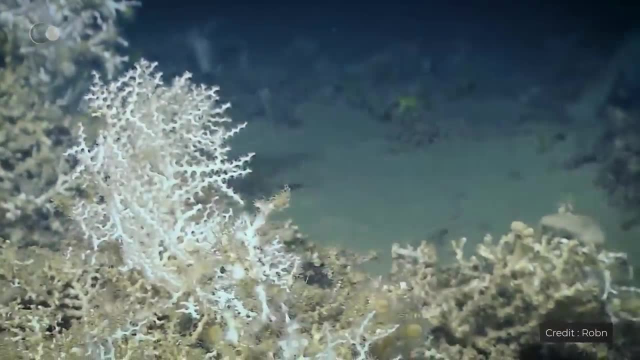 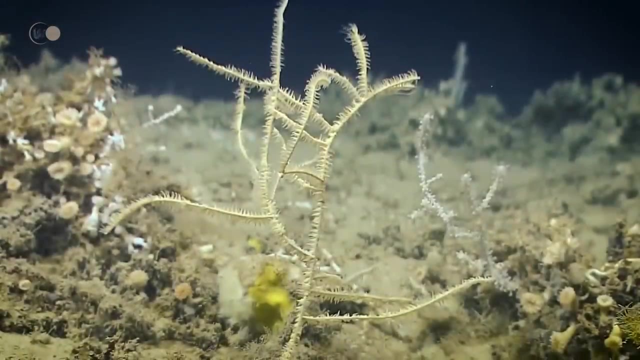 98% of colonial coral species that inhabited warm shallow tropical waters are disappearing. Solitary corals that established themselves in colder, deeper regions have fared better. Cephalopods, echinoderms and bivalves are seeing their number. 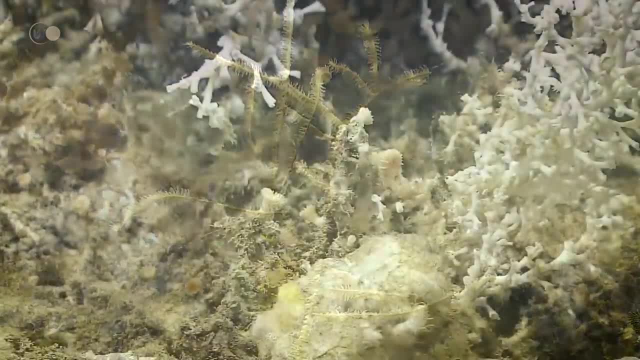 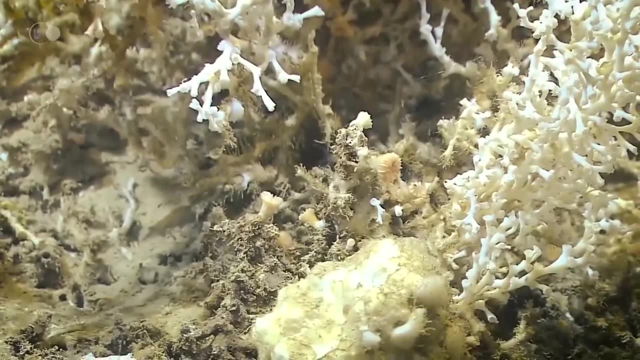 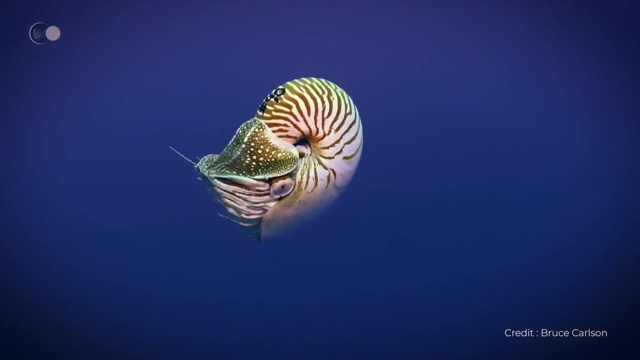 of genera decrease. Ammonites and belemnites disappeared, like all the other species of mollusks of the cephalopod class. The only survivors are the nautiloids, represented today by the nautilus and another group to which the octopods. 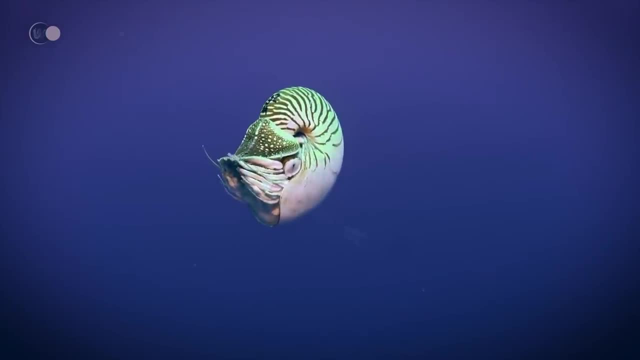 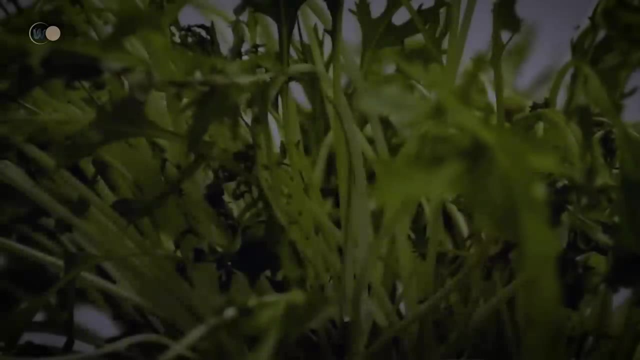 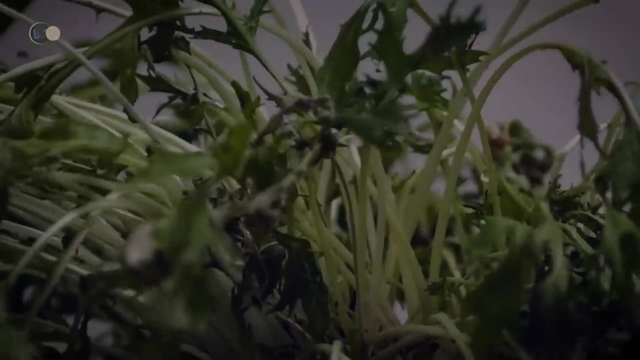 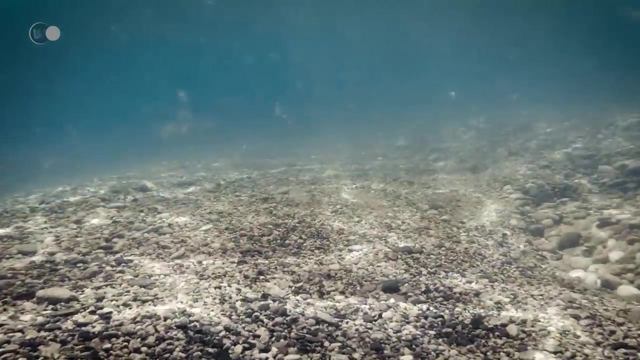 squids and cuttlefish belong. The base of the food chain has been affected. In the absence of light, plants wither away. Large herbivores are deprived of food. At sea, the food chains are disrupted in the same way. The plankton having disappeared, all those who fed on it die of hunger. The small debris-eating animals are used to feeding on plant debris and small animals living in the mud. Even if all the plants die, the aquatic fauna can survive. 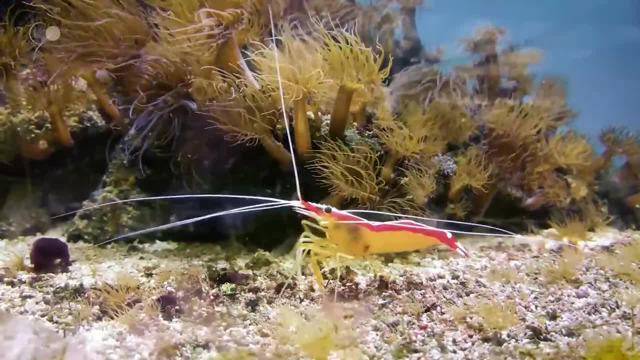 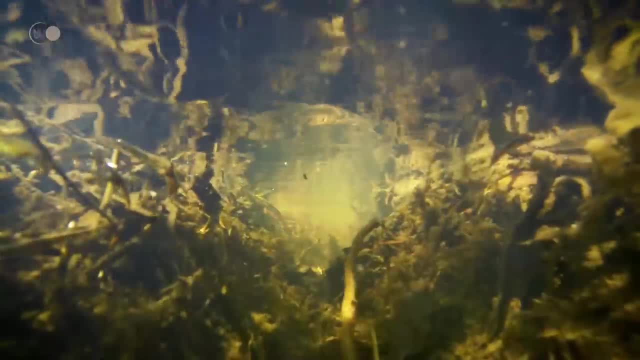 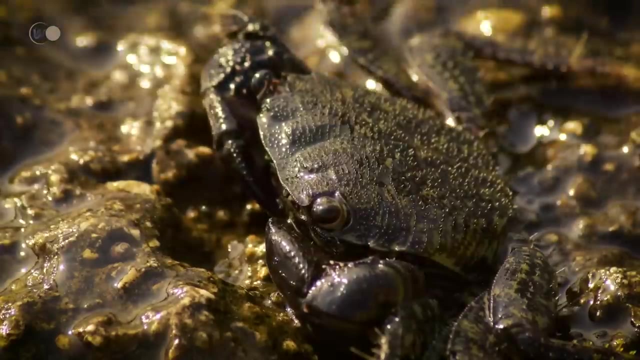 for a long time. Moreover, they are also able to withstand dry spells. Well hidden in the mud of fresh water, they spend their life in slow motion On land. these debris-eaters manage to find animal corpses, seeds or plant debris. 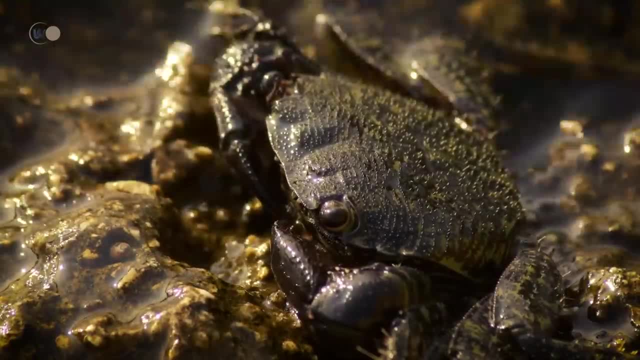 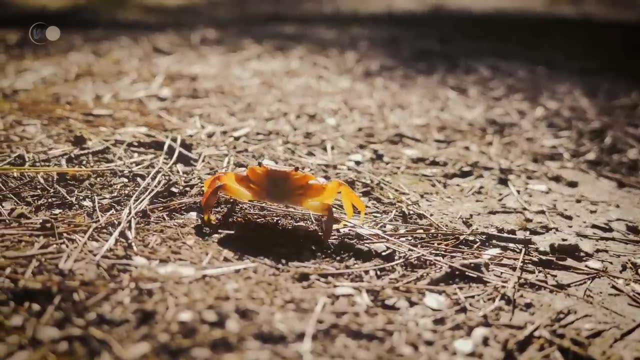 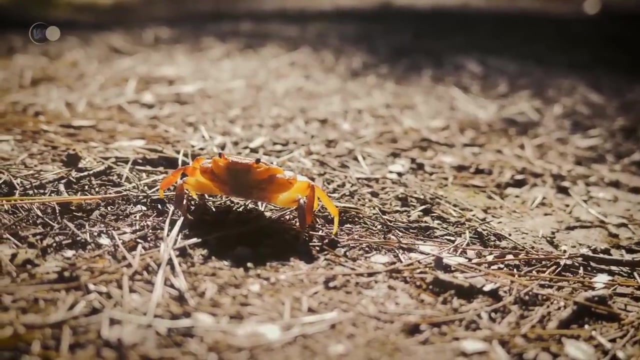 to survive for a few months. Combined with their ability to hibernate, they are more efficient in resisting hostile conditions. Another characteristic may allow some animals to better withstand the consequences of the meteorite fall: Mammals and birds are constant temperature species. 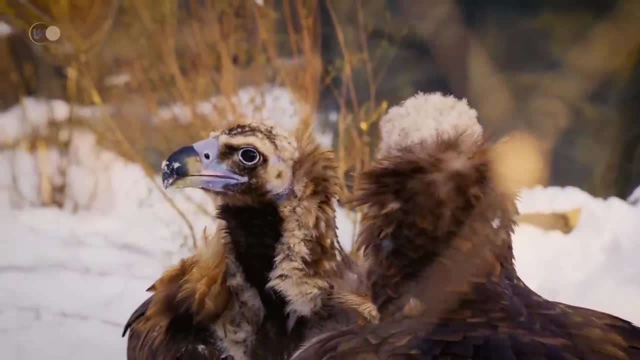 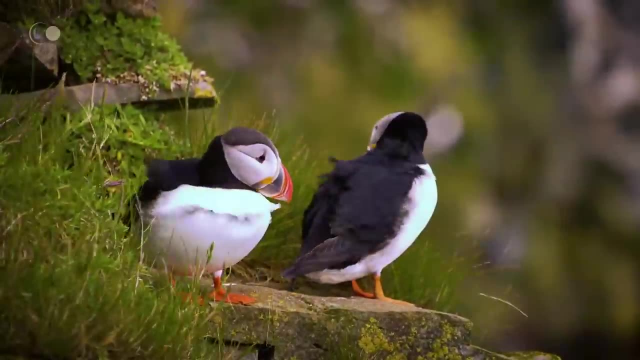 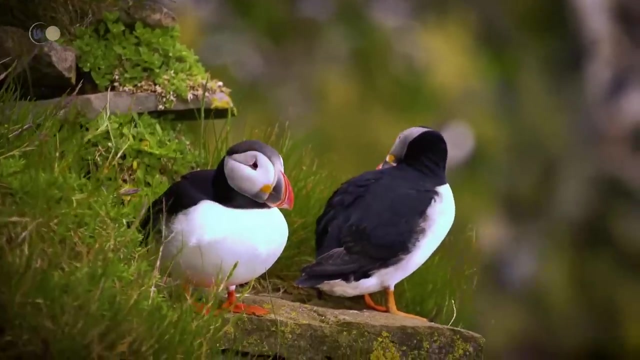 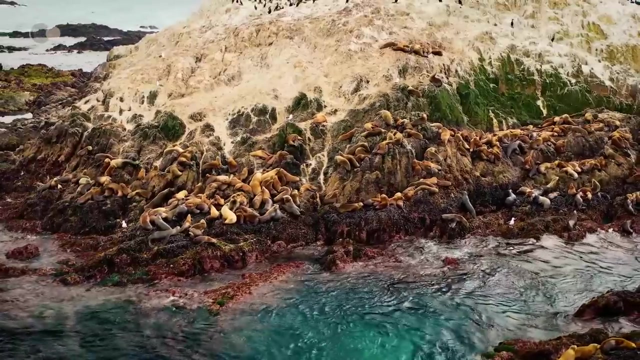 They are less dependent on the outside temperature and are capable of better survival. Similarly, species that live by the sea are better able to withstand major changes in their environment. Is it luck or a real capacity of adaptation For living organisms? it is impossible. 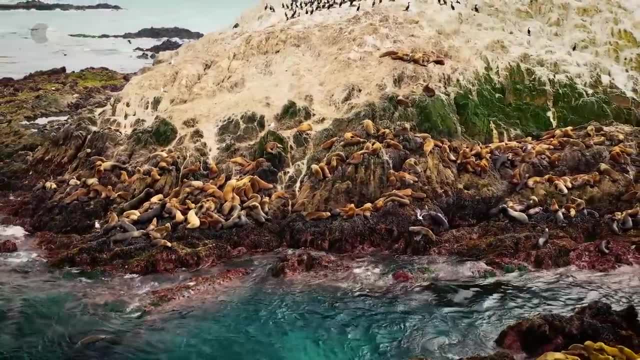 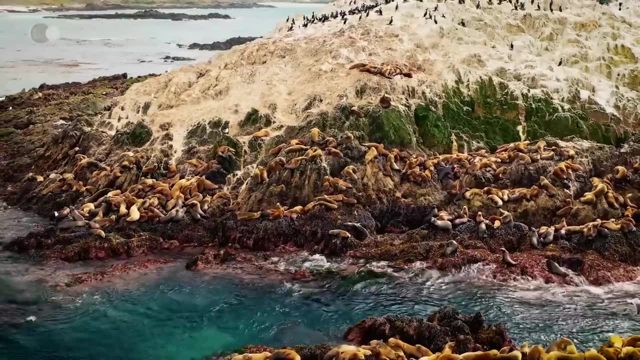 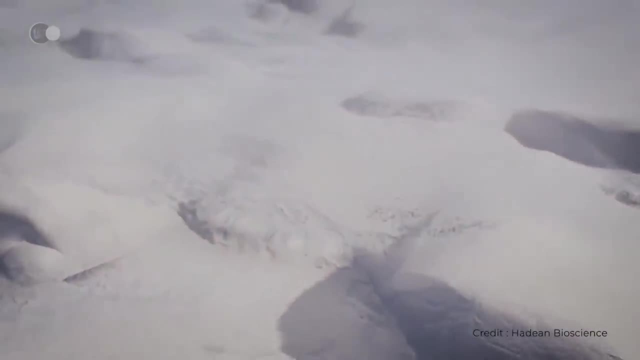 to adapt to such rare and catastrophic events. Natural selection only works if it is slow and weak enough not to cause the immediate death of all the individuals in the species During the Cretaceous paleogene extinction. animals are killed at random If some are favored. 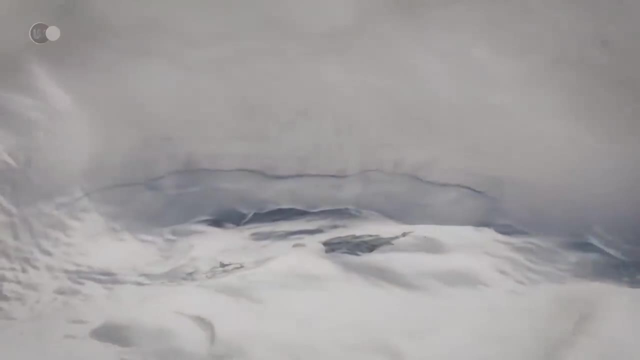 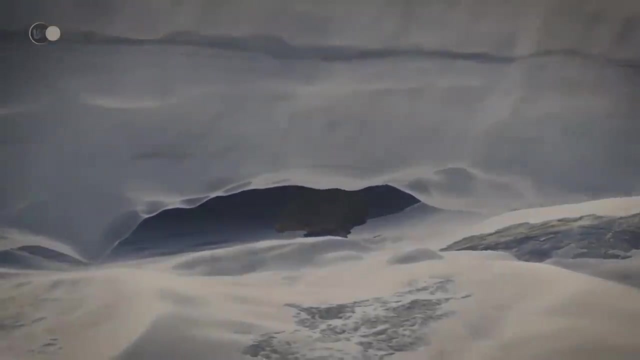 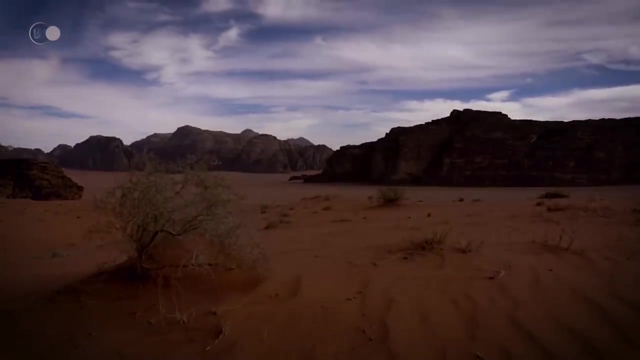 it is because they were better able to resist the new living conditions created by the event. After a warm start, the Earth undergoes a clear cooling trend. Tectonics led to a reorganization of the great ocean currents and raised the great reliefs. 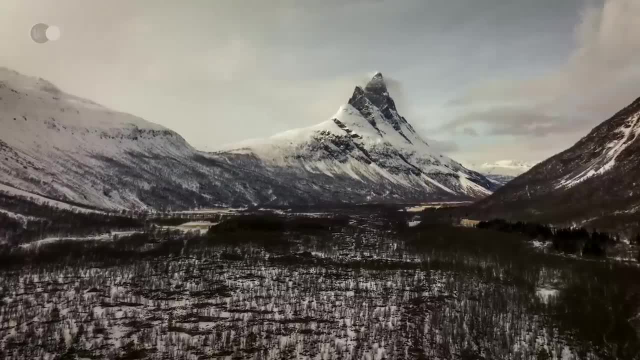 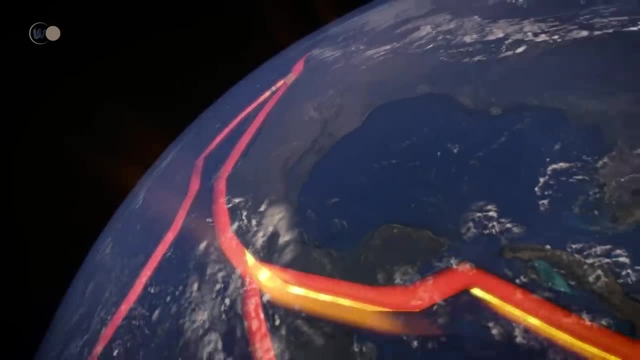 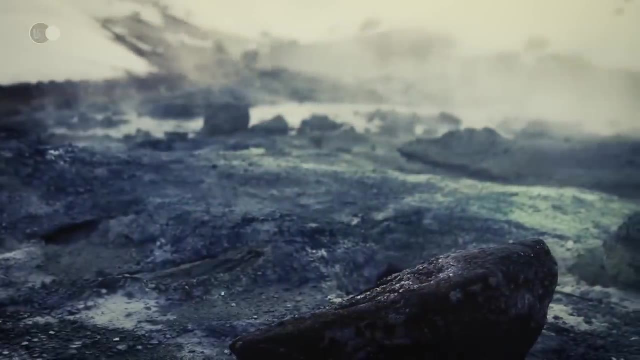 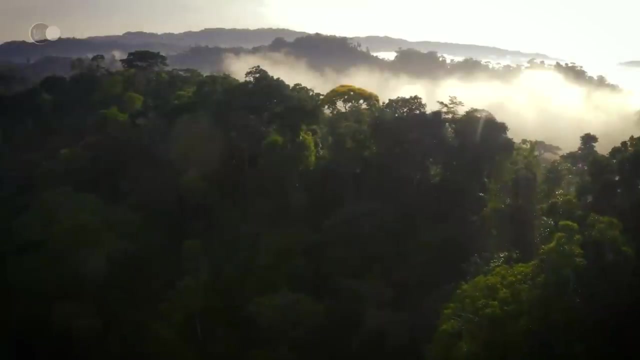 that consume CO2.. Barely 10 million years later, a continental tear in the northern hemisphere releases large quantities of carbon dioxide into the atmosphere and the oceans, causing the temperature to rise by at least 5 degrees Celsius. This warming disrupts ecosystems again. 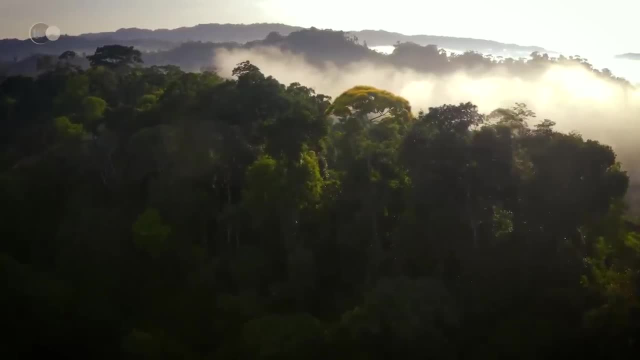 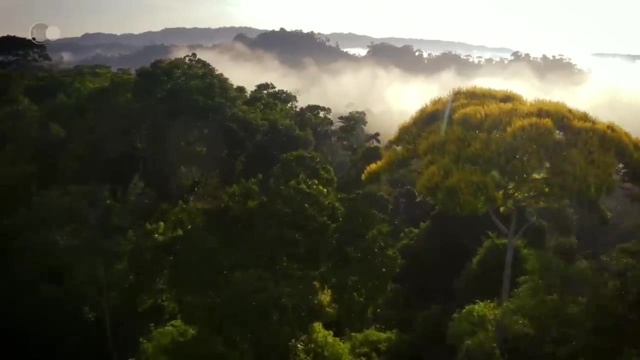 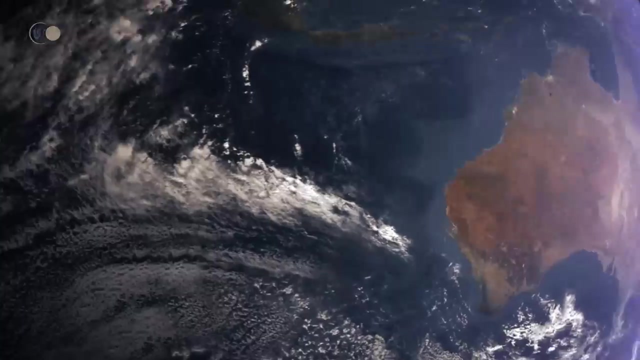 and has an important influence on the evolution of mammals. The vegetation is transformed, The forests become dense, The last remnant of the supercontinent Gondwana breaks up, forming Australia and Antarctica. Australia takes with it a remarkable fauna and flora, of which we still find. 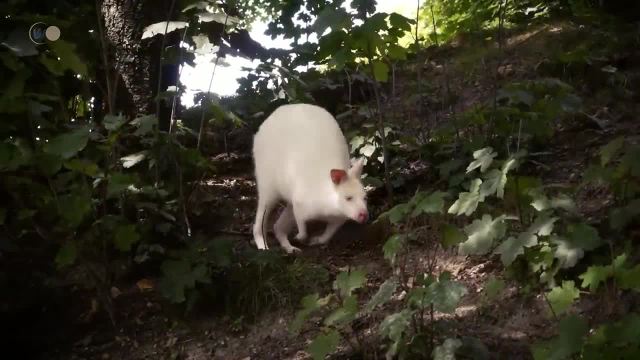 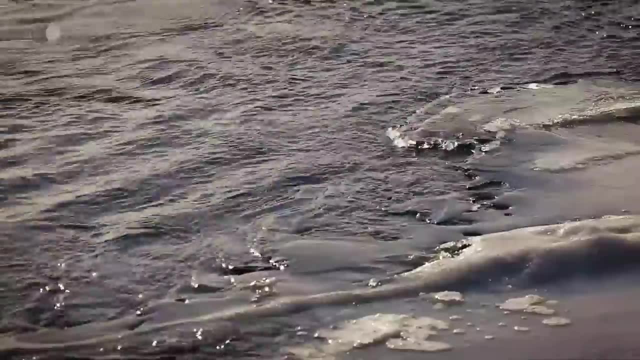 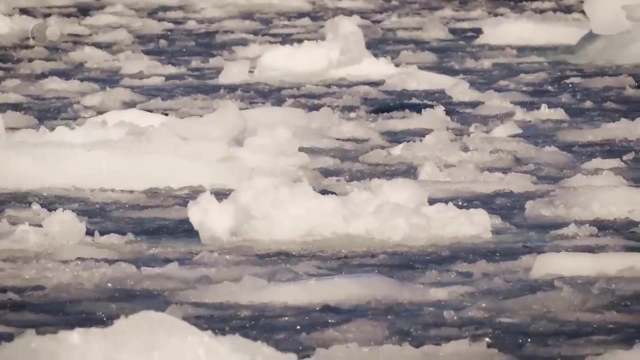 some specimens. today, This separation causes the creation of a circum-Antarctic current that will isolate the southern continent from warmer waters and cause its freezing. The terrestrial world is now dominated by familiar life forms such as flowering plants, songbirds and mammals. 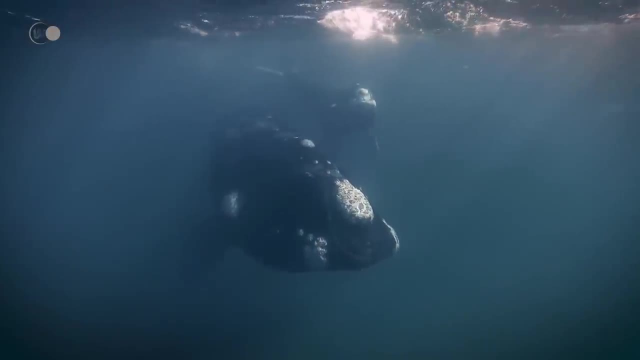 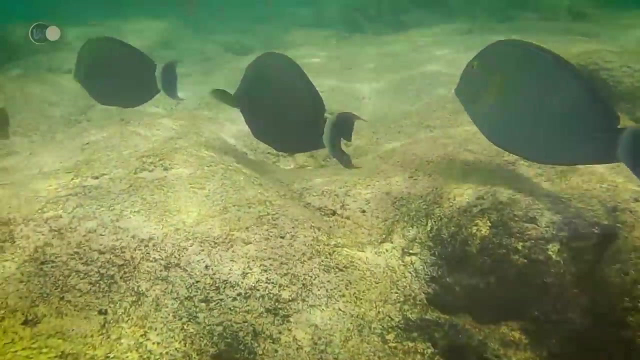 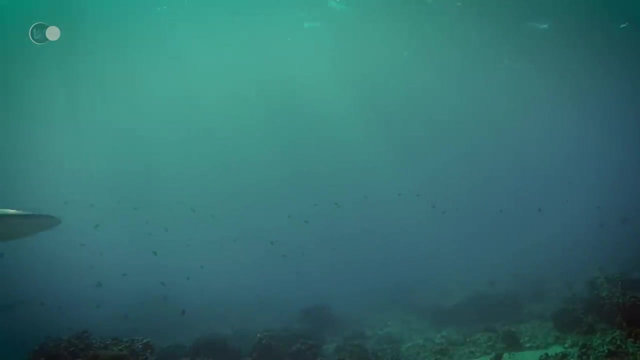 and many more. In the waters, mammals predominate, with whales, seals and a myriad of modern bony fish. They share the ocean with sharks, which were already present. The explosion of all these groups created the biological world of today. 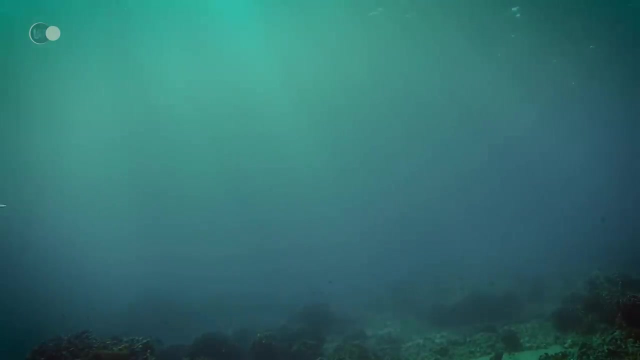 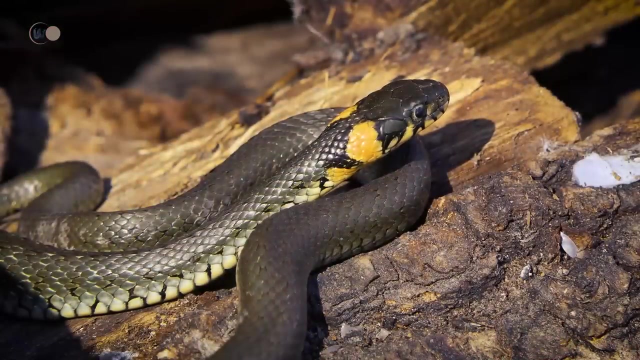 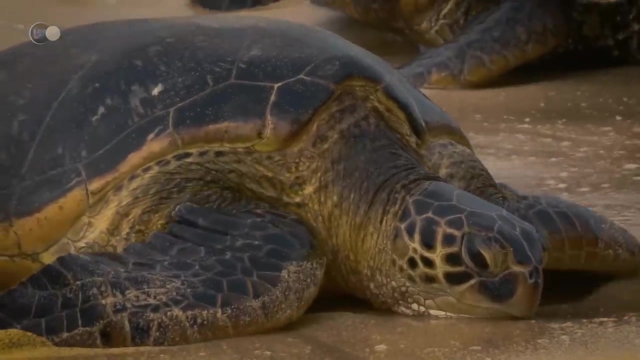 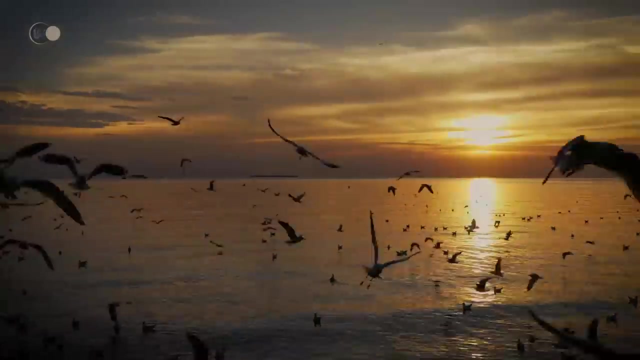 Most of the larger animals have disappeared. The surviving reptiles are rather modest in size, with a few snakes, lizards, small crocodiles and turtles. Only birds impose themselves by their size and try to reign on the animal world. The Gastornis paraceensis. 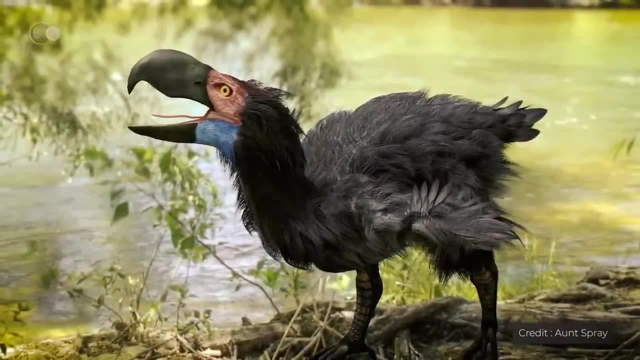 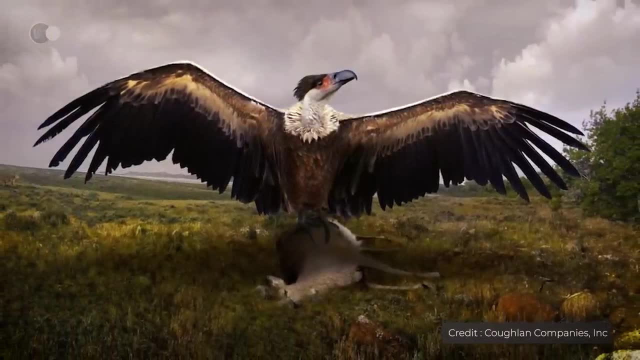 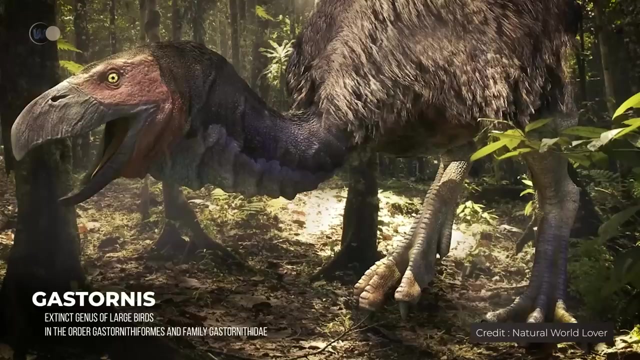 also called diatrioma, and the Pterotornis incredibilis are birds with impressive sizes. The Gastornis is the largest bird of its time, growing up to 2 meters or 7 feet for the largest specimens. It has short wings. 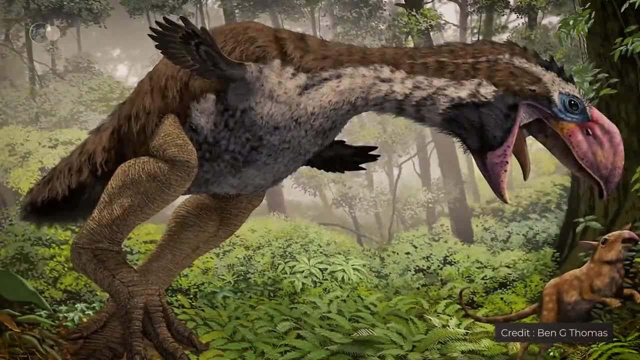 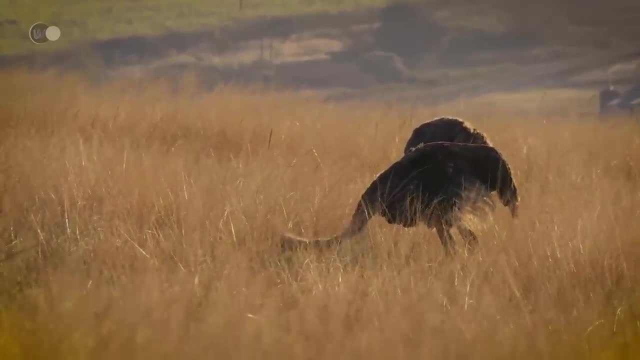 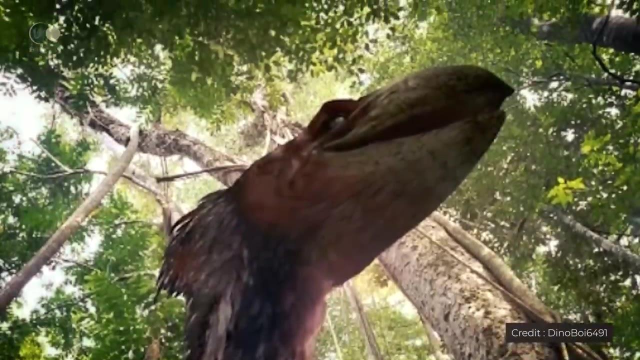 long legs and a thick beak. It moves in the manner of today's ostriches, since it is unable to fly. He likes the forests and swamps in the tropical climate At that time. it is not a prey, because its potential predators 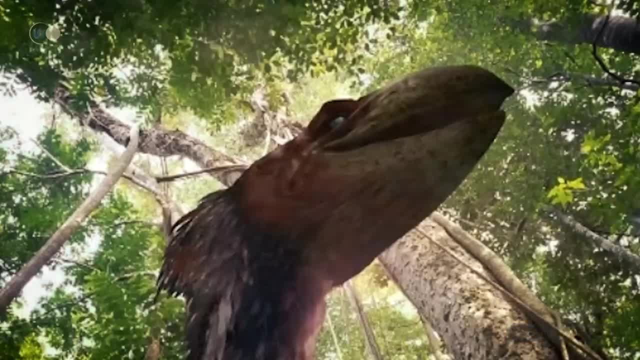 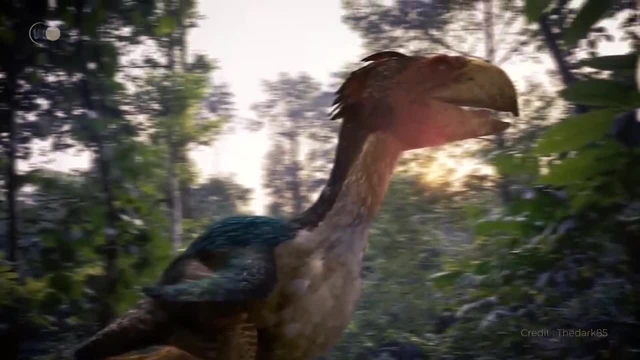 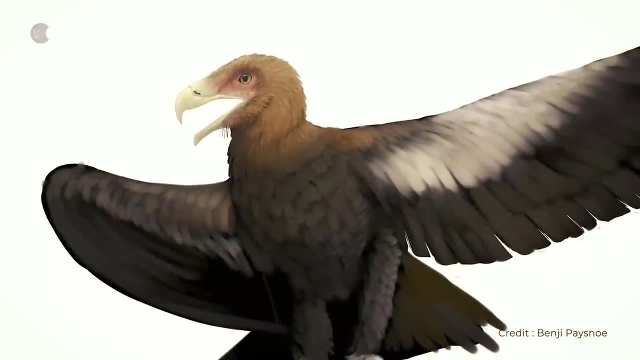 mammals or crocodilians are smaller than it. Its robust beak and powerful claws allow it an omnivorous diet. The Pterotornis is nicknamed the monster bird. Its wingspan can reach up to 5 meters or 16 feet. 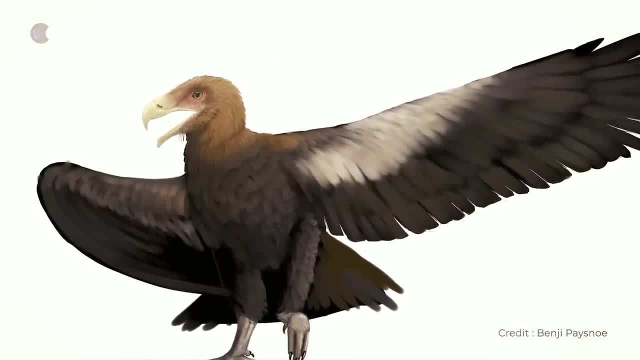 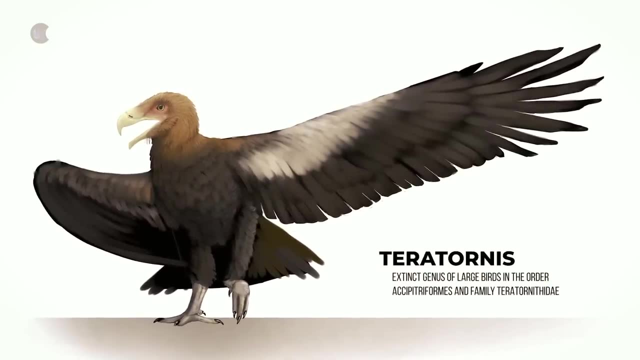 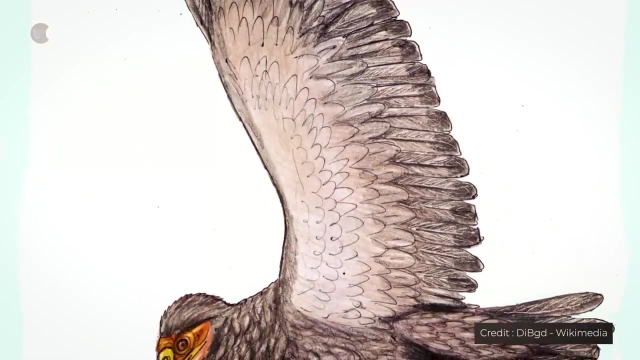 and the surface of one of its wings reaches 17.5 square meters, or 190 square feet. At the time, it was the largest bird able to fly. Its strong legs and powerful feet allow it to snatch and catch prey with a very strong grip. 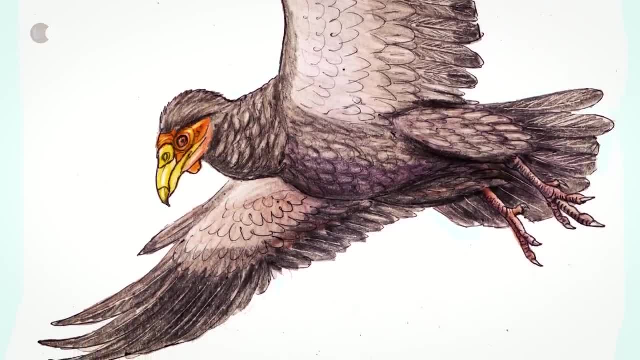 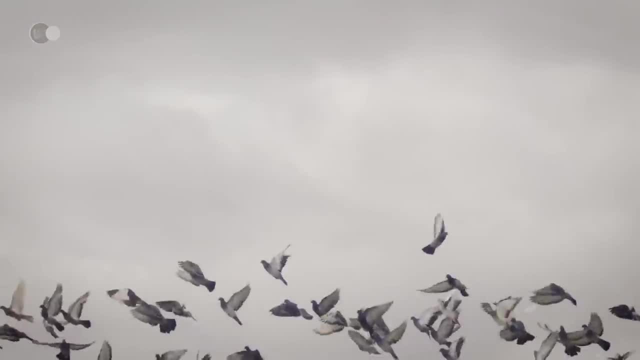 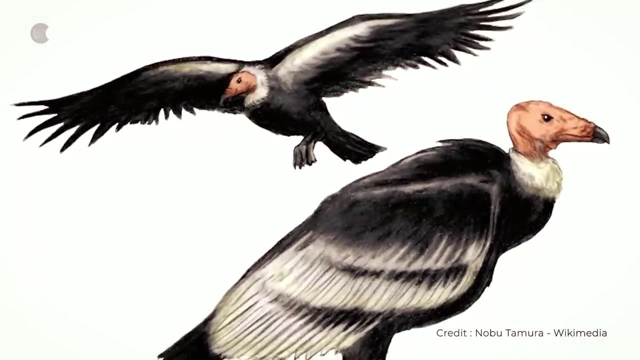 These two specimens are only fleeting on the Earth, and the birds that will endure will sport more modest sizes in the future, But for now, these terrifying raptors haunt the savannas. They prefer sparsely vegetated environments that allow them to chase their prey. 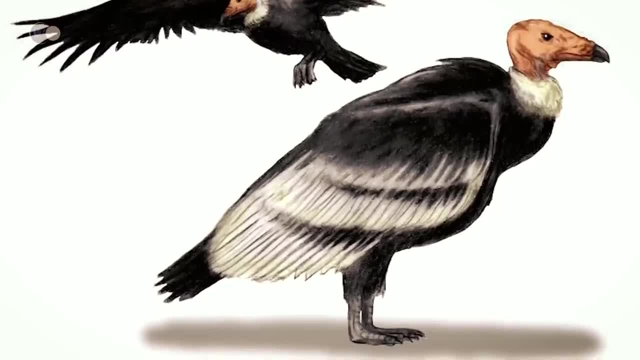 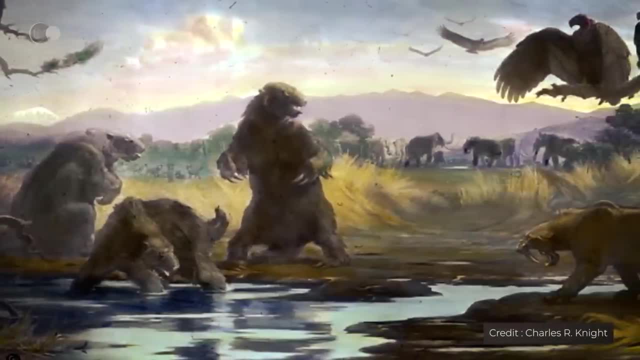 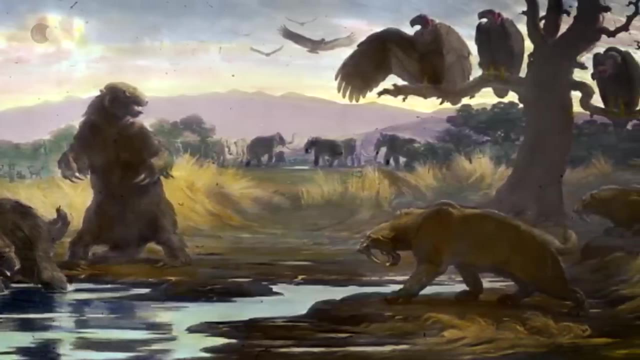 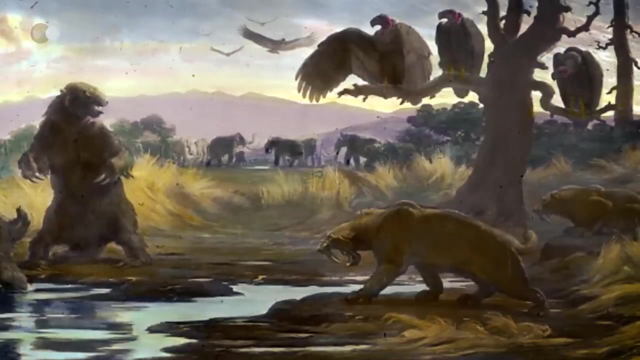 They capture and devour small mammals such as primitive horses, but also corpses like modern vultures, As long as mammals remain too small to act as predators. these giant birds have no serious competitors and remain at the top of the food chain, The Perissodactyls. 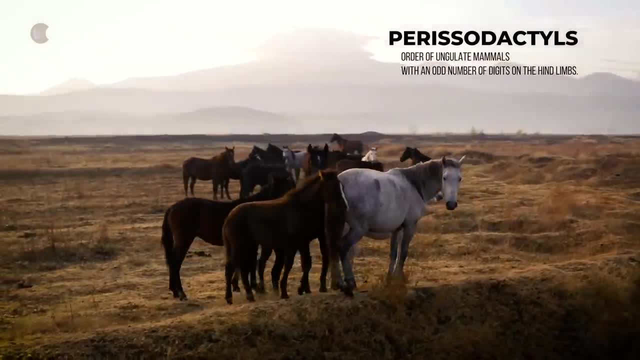 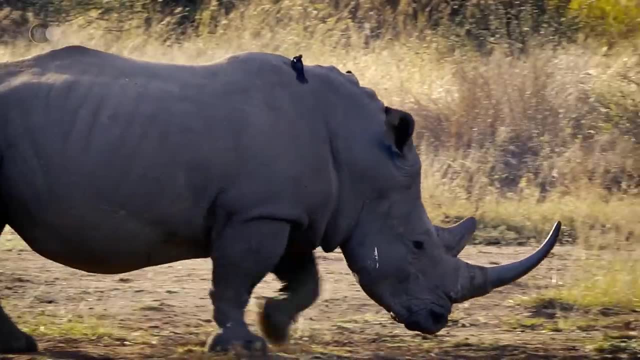 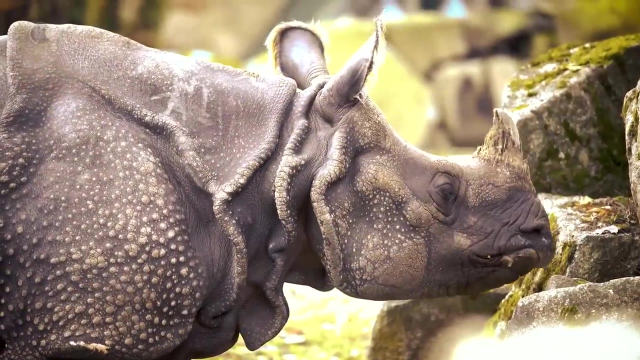 will be very successful and will include the ancestors of horses, tappers and rhinoceroses. The three lineages were one at the time. These animals are different today, but their ancestors were very similar, although they do not occupy the same environments. 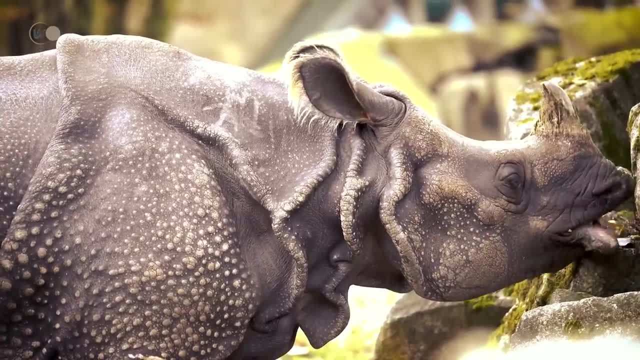 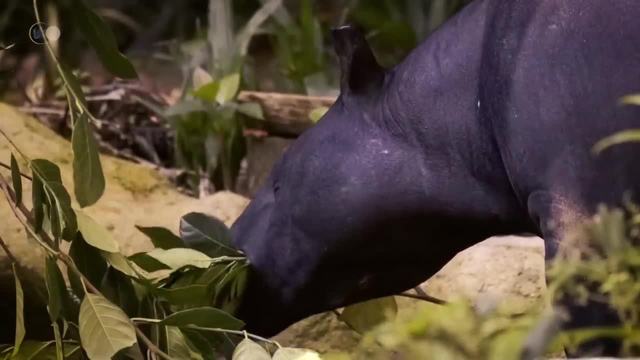 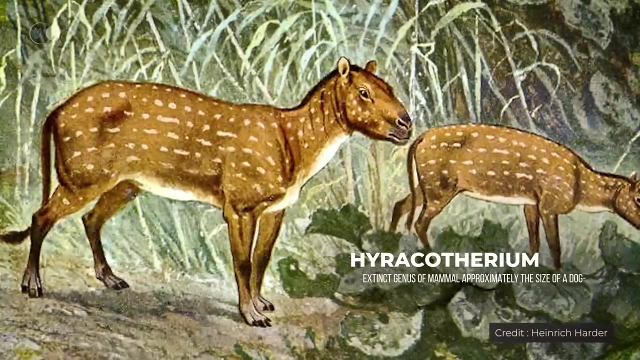 They do not eat the same plants, which avoids too much competition that could lead to the disappearance of some species. The Hyracotherium is often attacked by these dangerous birds. Although it is a member of the evolutionary lineage of the horse, it is more like a dog. 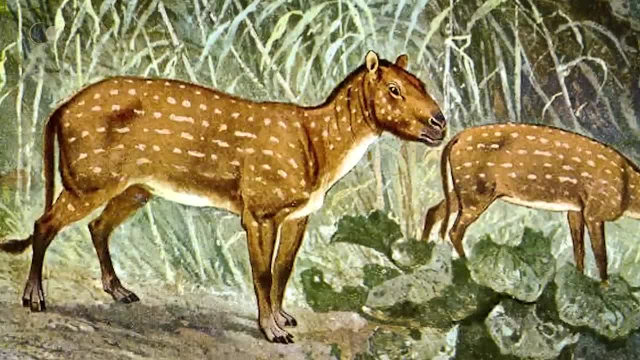 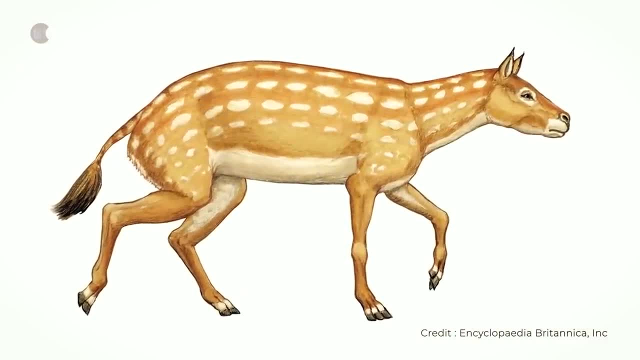 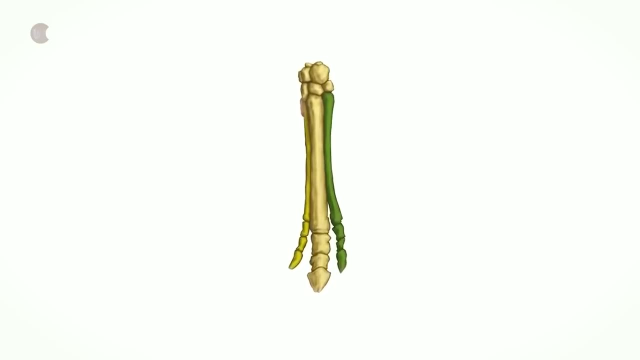 at the time About 60 centimeters or 20 inches long and no taller than 20 centimeters or 8 inches. it has four toes on its forelegs and three toes on its hind legs. It does not have hooves. 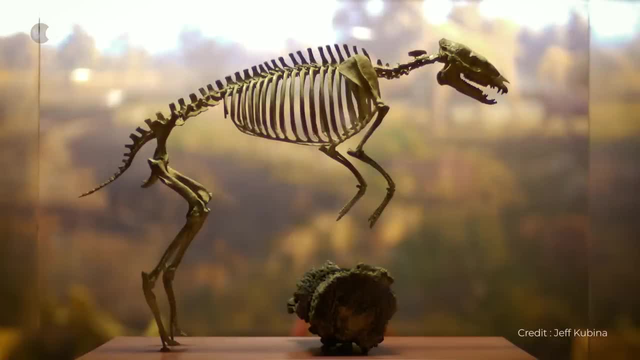 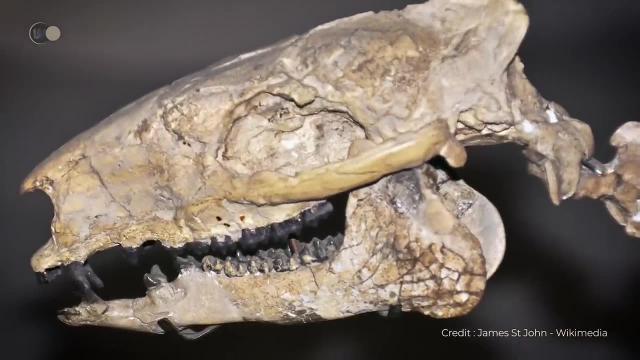 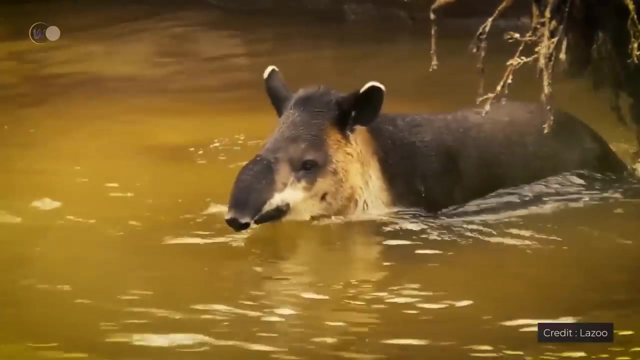 like our modern horses, but a kind of paw pads resembling those of dogs. Its 40 or so teeth are used to crush soft leaves and young plant shoots. since it is a herbivore, Heptadon lives in North America. This primitive tapper. 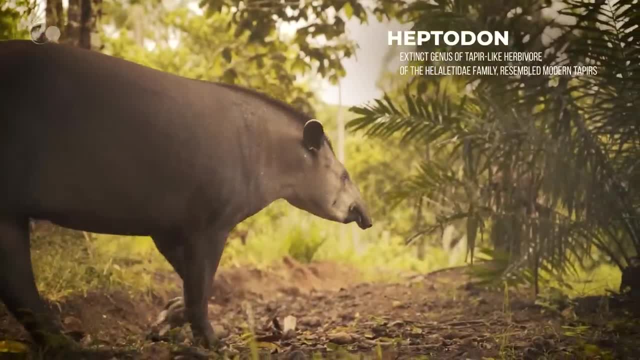 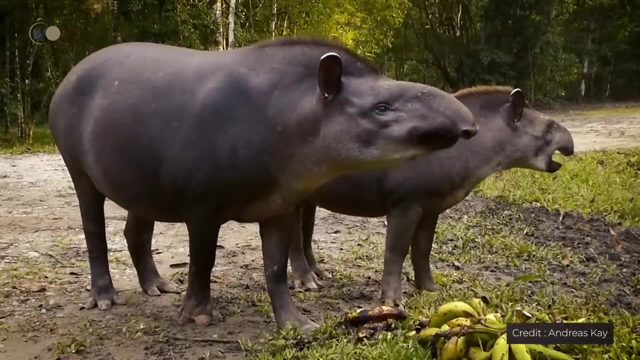 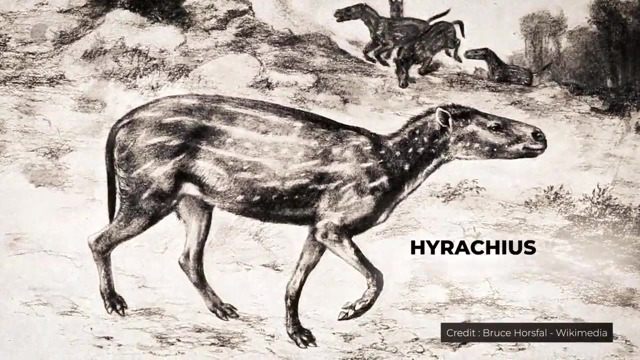 measures one meter long. Although its limbs and its skull are similar to those of the current tappers, it does not yet have their characteristic small trunk. Its close cousin, Hyracius, is one of the first rhinoceroses. It is slightly larger. 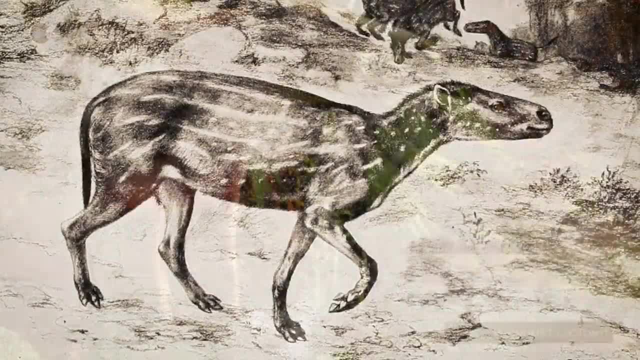 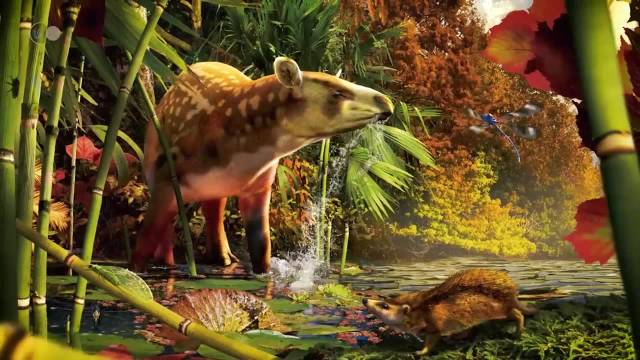 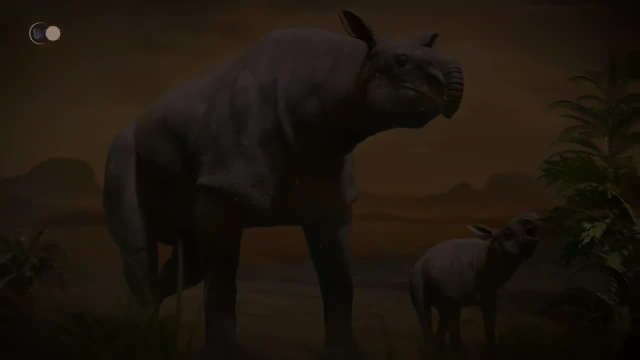 than Heptadon, but does not yet have a horn. Heptadon, Hyracius and Hyracotherium look very similar at the time, but their lineage will then clearly divide. New mammals appear, including Phenocotus. 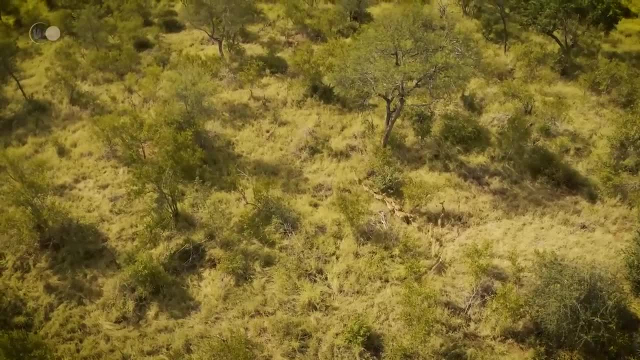 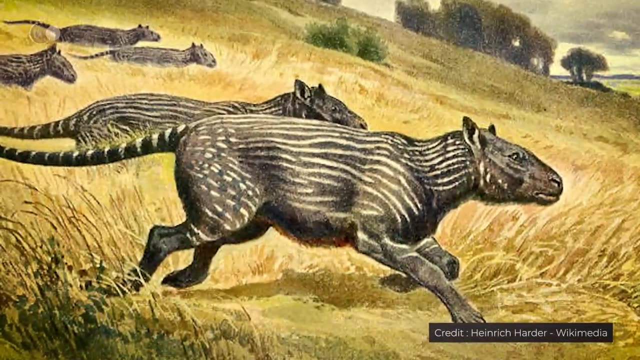 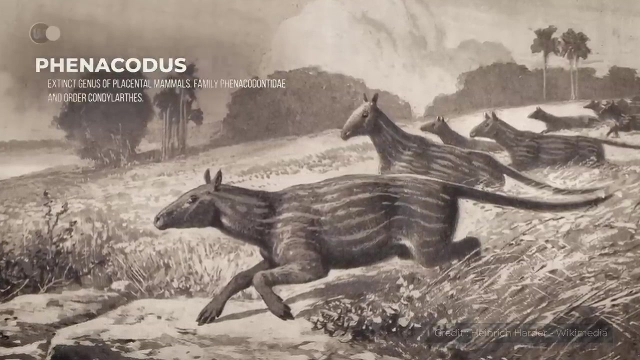 This medium-sized herbivore vaguely resembles a deer or a modern horse. It occupies the root of the ungulate family tree. It has teeth well adapted to the hard vegetation of its habitat. It is up to 1.5 meters or 5 feet long. 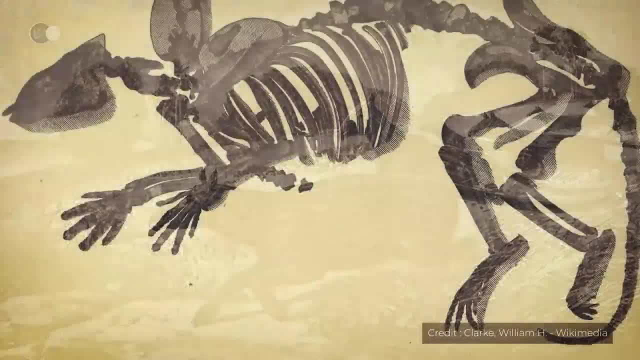 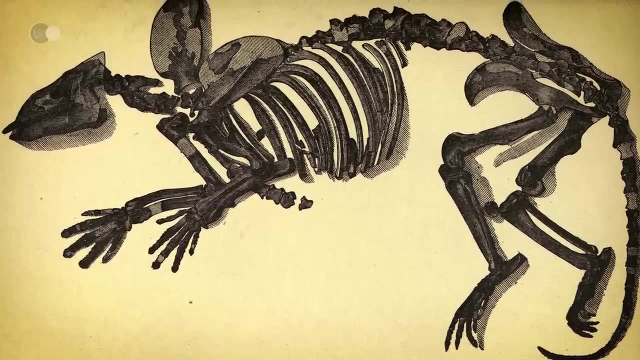 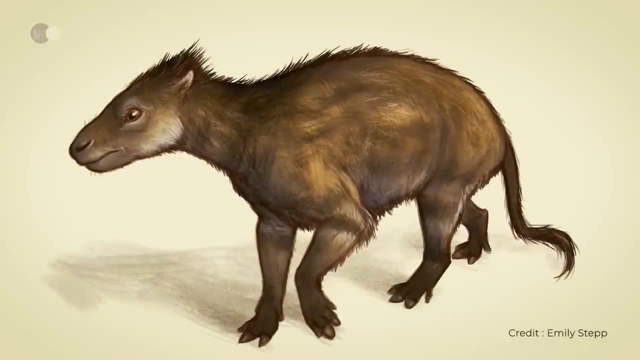 has long, straight legs and a narrow snout. Each of its limbs ends in five full fingers, allowing it to walk like a modern tapper. The 20 claws on its limbs were later modified to become hooves. in modern ungulate species, Biodiversity is still. 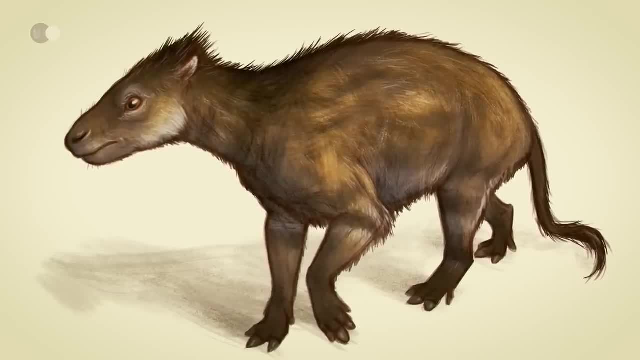 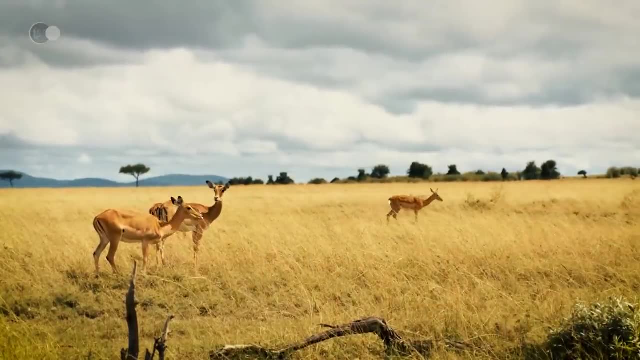 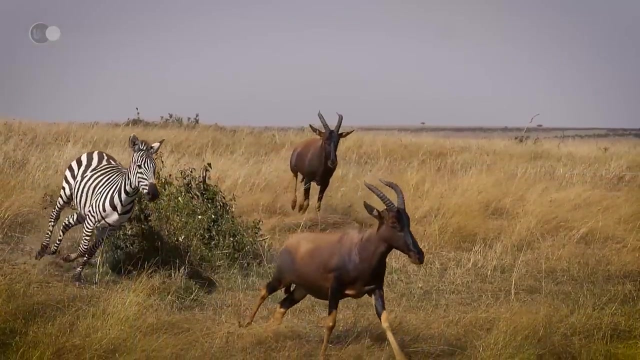 very different from today. Even if the forests are present, the grasslands begin to expand and the herbivorous animals develop. Some families of mammals evolve towards new ecological types, such as runners, gliders, even real flying animals, swimmers. 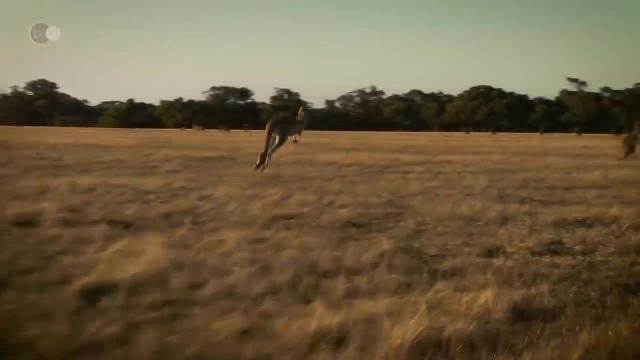 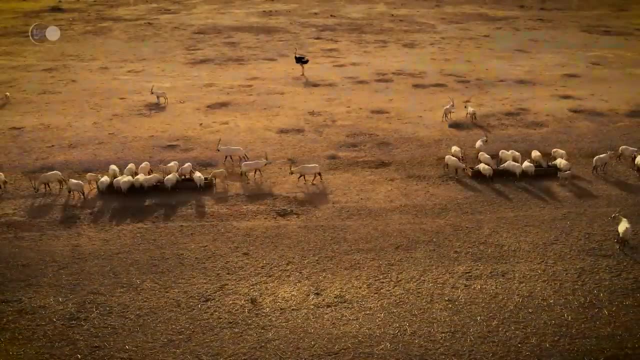 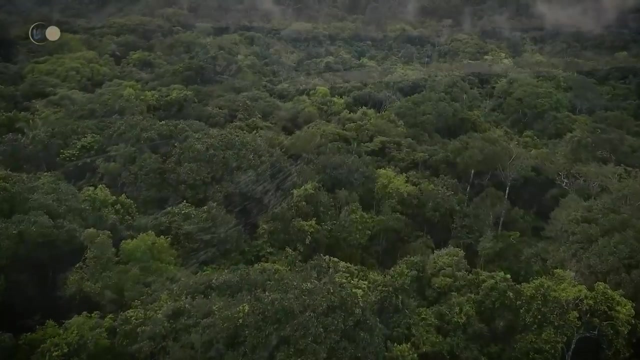 jumpers, burrowers. They are distributed over the entire surface of the earth and occupy all environments, from burning deserts to icy poles. They adapt to treetops, high mountains, oceans and freshwater swamps. Innovations such as 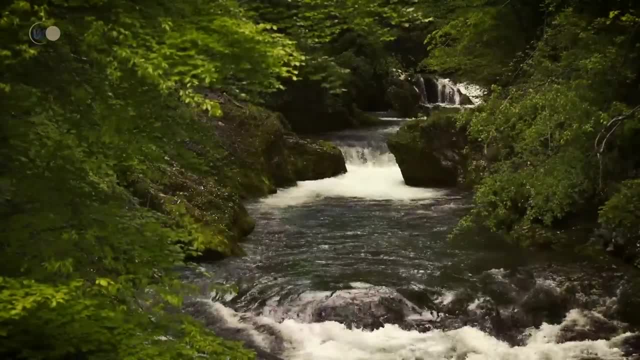 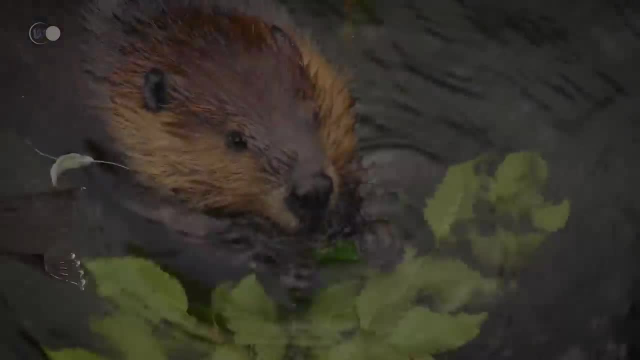 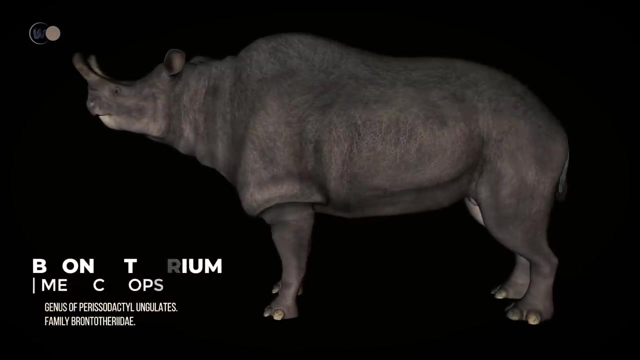 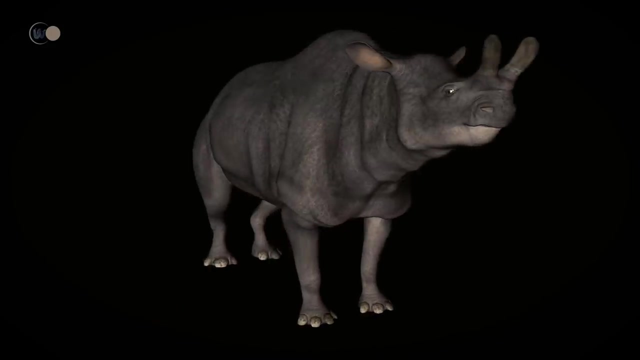 the wings of bats and the large incisors of rodents will prove crucial to their biological success. Brontotherium is a genus of ungulate reminiscent of our modern rhinoceros. It has a pair of horns on its snout, the males being more imposing. 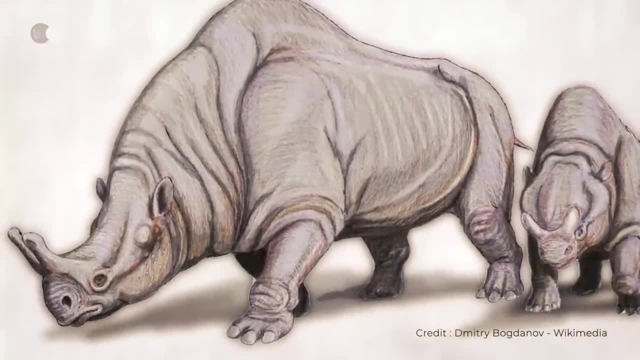 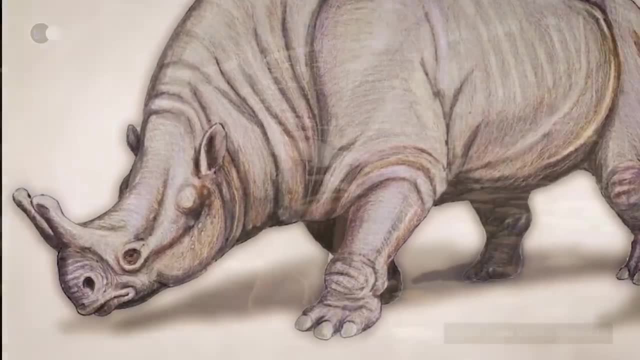 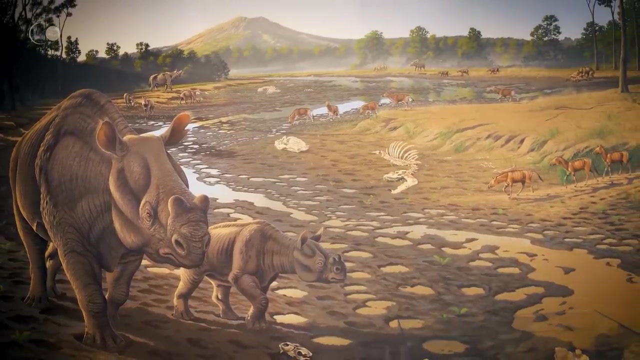 than the females, Although its appearance brings it closer to the rhinoceros. it reaches the size of an elephant. It measures up to five meters in length and weighs up to five tons. This herbivore is fond of tender leaves and young shoots. At 1.5 meters or five feet long, 80 centimeters or 30 inches high and 100 kilograms or 220 pounds, Heracodon looks like a pony. It is, in fact, a species of primitive rhinoceros. 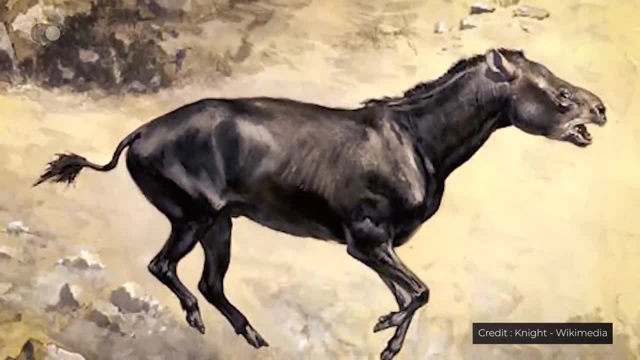 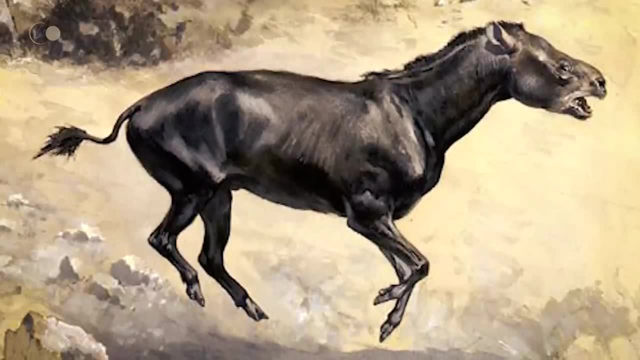 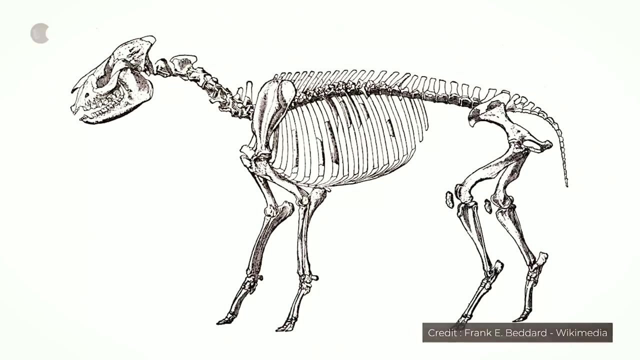 even though it does not have a horn and is a runner at this time. It feeds on a wide variety of vegetation in the steppes and open forests. Its slender legs rest on three fingers and its head is particularly large compared to the rest of its body. 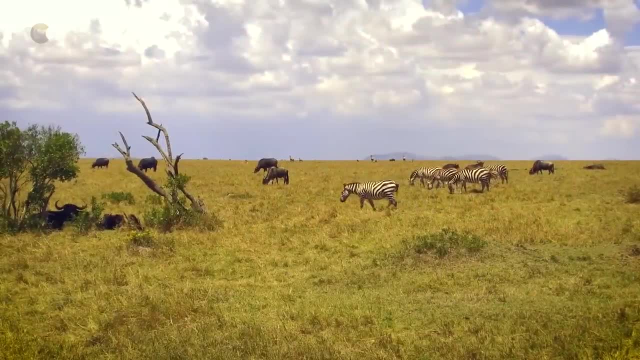 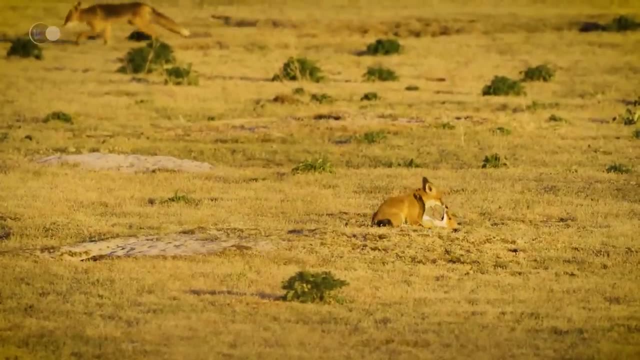 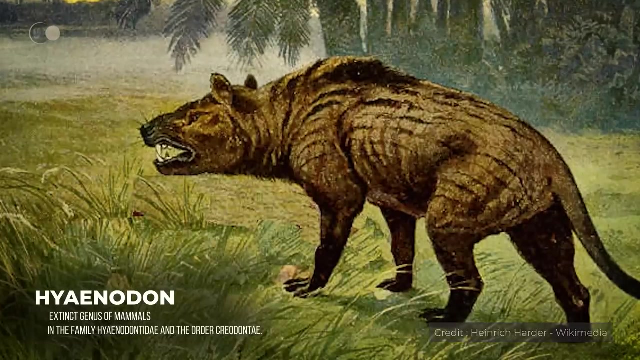 The diversification of herbivores undoubtedly parallels that of carnivorous mammals. Among the groups represented at this time, Hyanodon, whose name means hyena teeth, appears under its feline appearance. Its massive and robust body has a long tail. 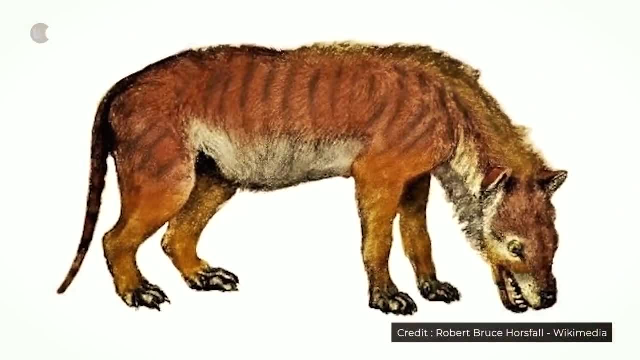 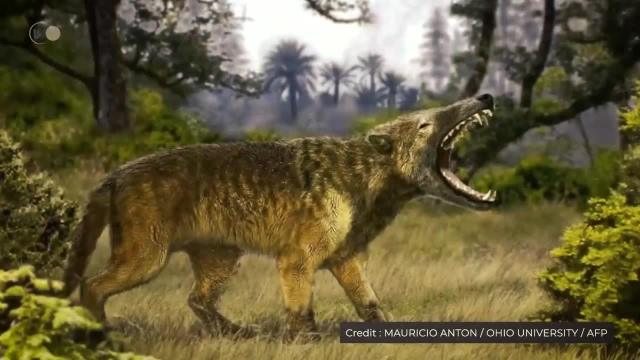 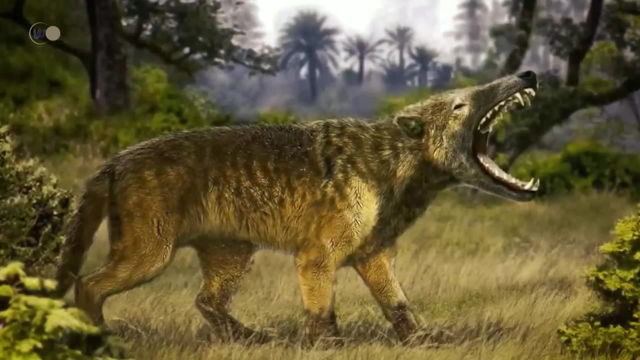 and each of its toes has sharp claws. Hyanodon is an outstanding hunter. Although its brain is small, it has a highly developed sense of smell, a powerful jaw and its speed allows it to hunt many preys. Its sharp and pointed teeth. 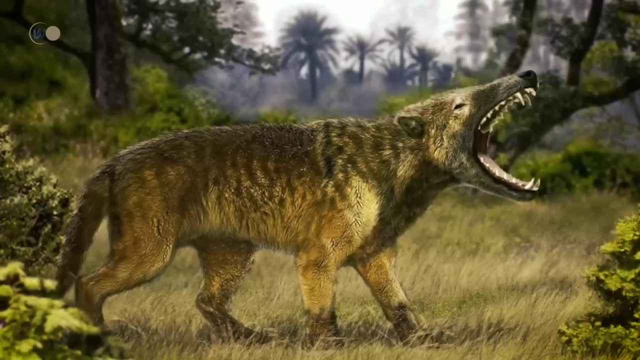 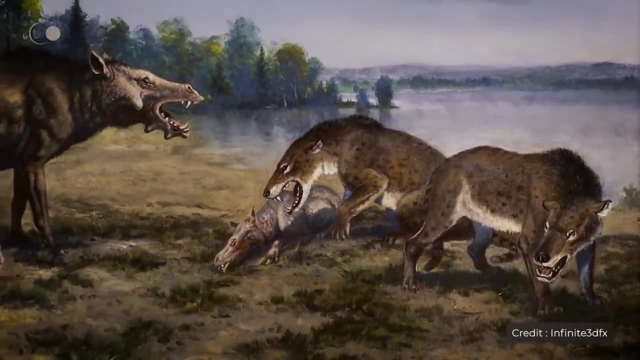 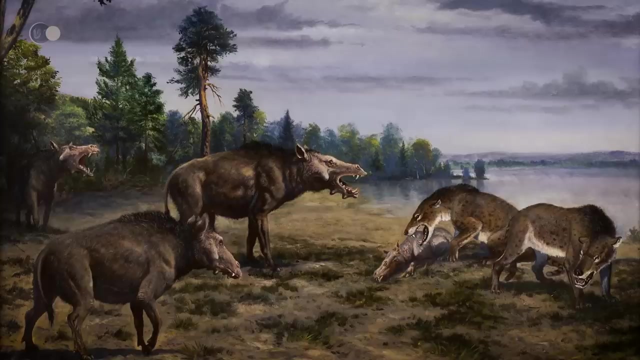 allow it to crush them when it catches them. Hyanodon is also a scavenger. It covers the corpses of animals it finds with excrement in order to mask its smell and avoid other scavenging predators to spot it Standing at 1.50 meters. 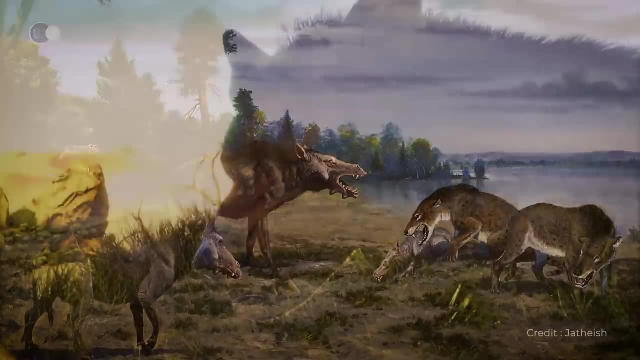 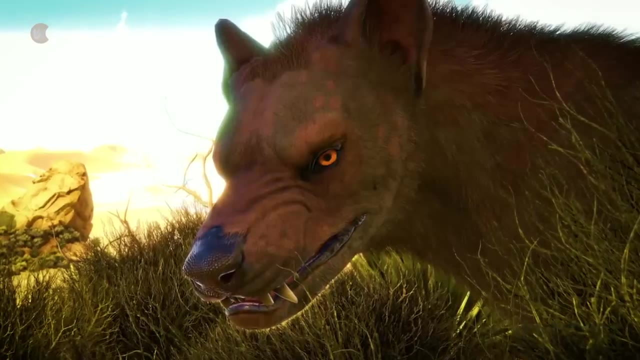 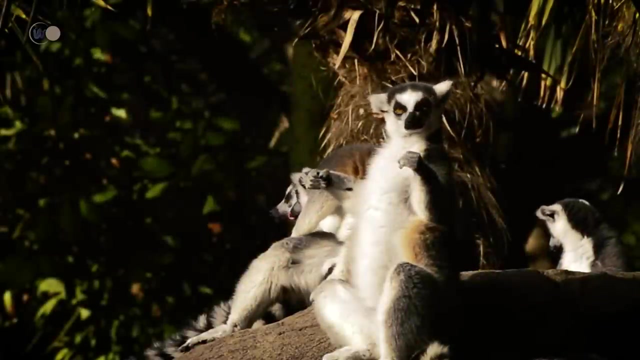 or 5 feet and 3 meters or 10 feet long Hyanodon is not afraid to take on large predators like Gastornis, as it can run at speeds of 55 kilometers per hour or 35 miles per hour. Fifty-five million years ago. 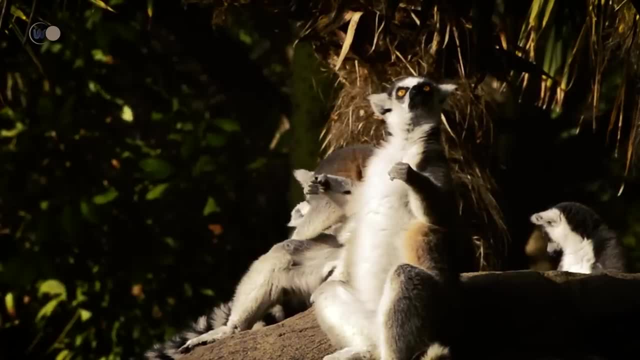 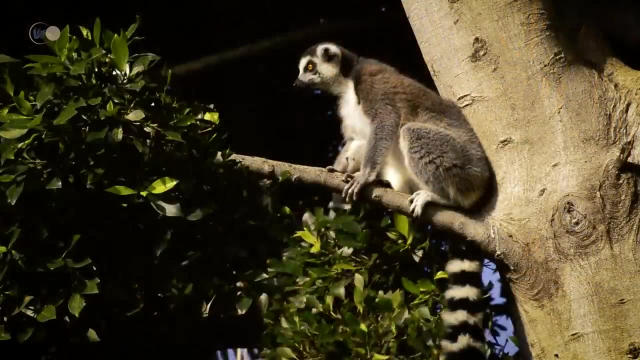 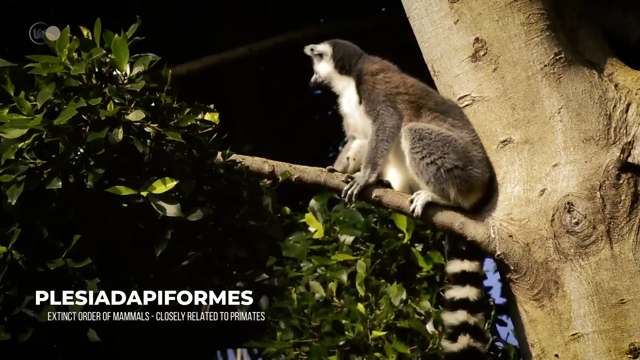 a group of mammals took a different evolutionary path. Equipped with two close-set eyes and opposable thumbed hands, they are the first primates. The precursors are the Plesiodapiformes. These small mammals are Insectivorous and Arboreal. 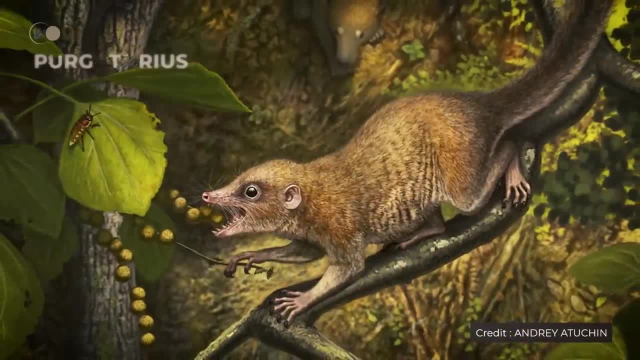 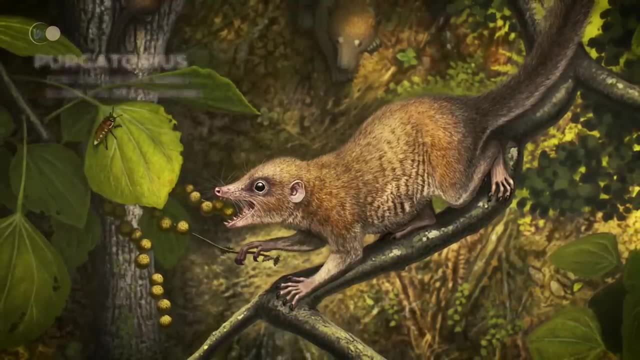 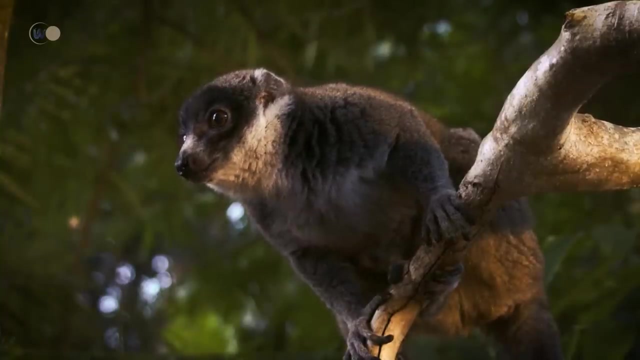 The first specimen is none other than Purgatorius, this small being that hid as best it could during the fall of the meteorite. The Plesiodapiformes diversify until they form a hundred species settled in tropical regions. Their size varies. 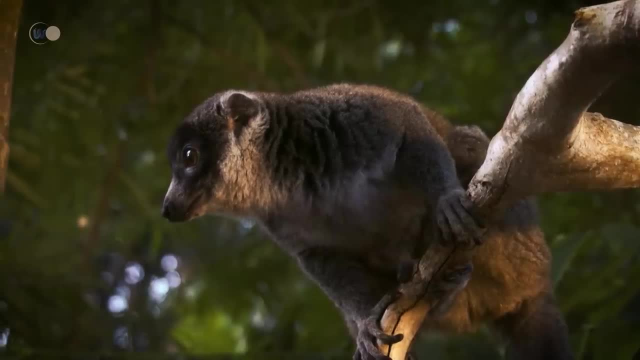 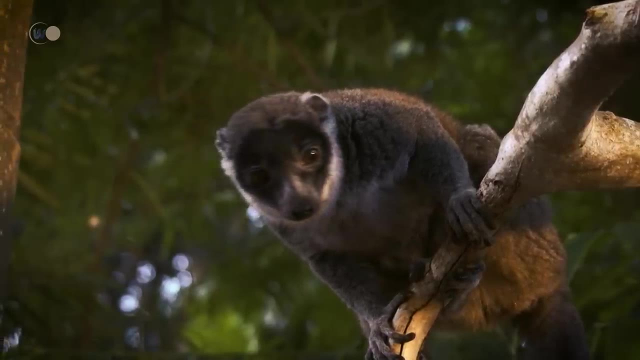 from that of a hamster to that of a squirrel. The primitive architecture of their skull, their small brain and the presence of claws on their legs do not yet classify them as true primates, However, such as marmosets, baboons. 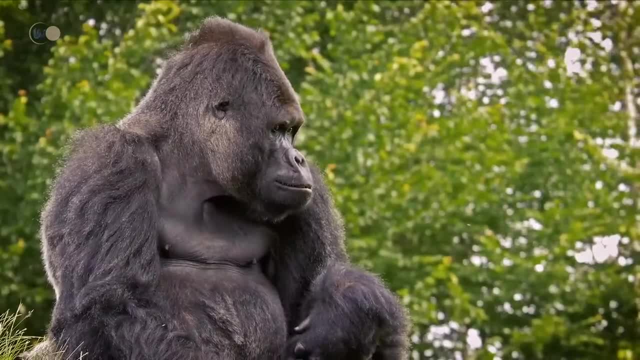 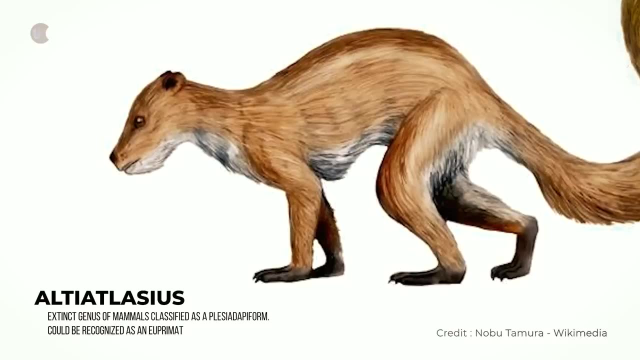 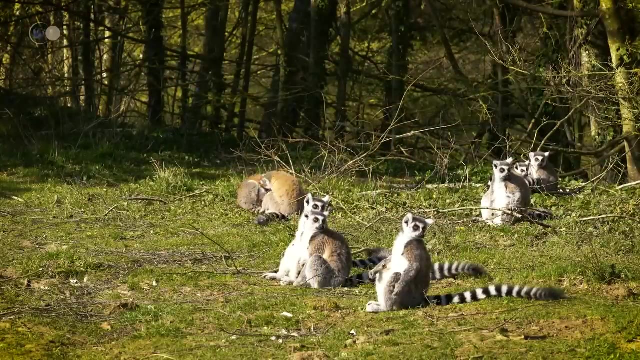 gorillas and humans. The very first known prosimian is named Altia thalassius. From 55 million years ago, its descendants spread throughout the Northern Hemisphere At that time. it is one of the most diverse groups of mammals. 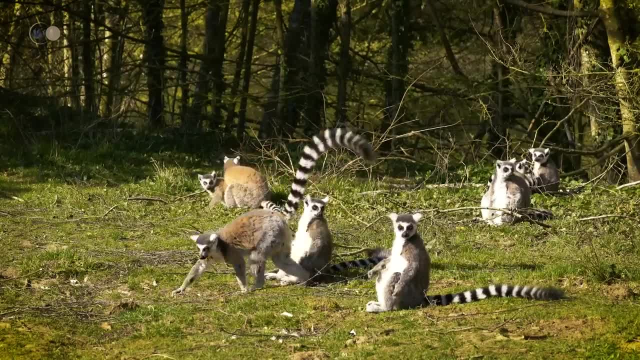 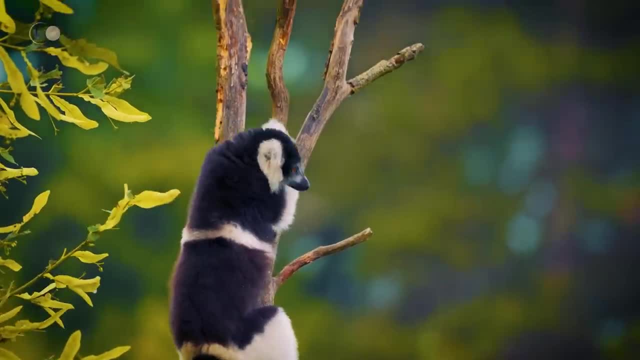 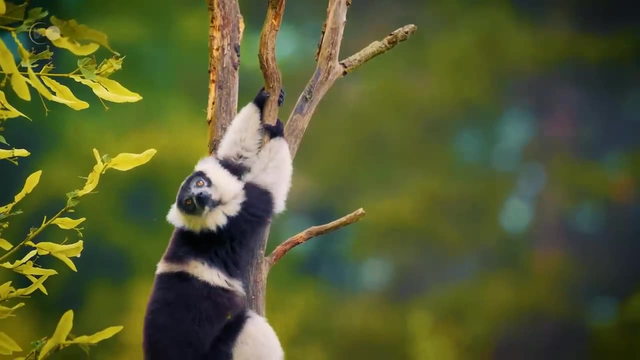 The legs of the prosimians evolve and are now hands and feet equipped with claws that form nails. They are shorter and more flat than those of the Plesiodapiformes. Their thumb is opposite to the other fingers. They can now. 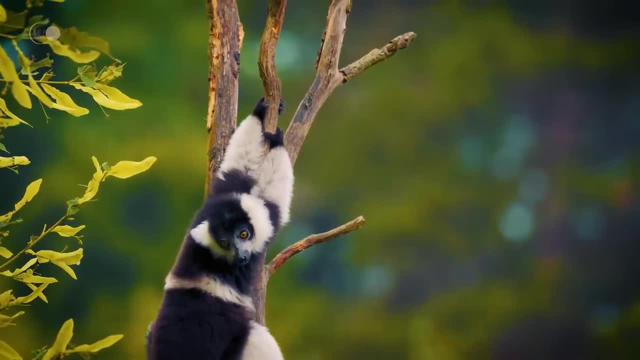 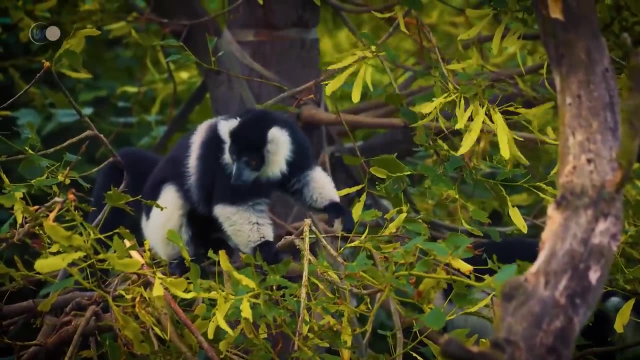 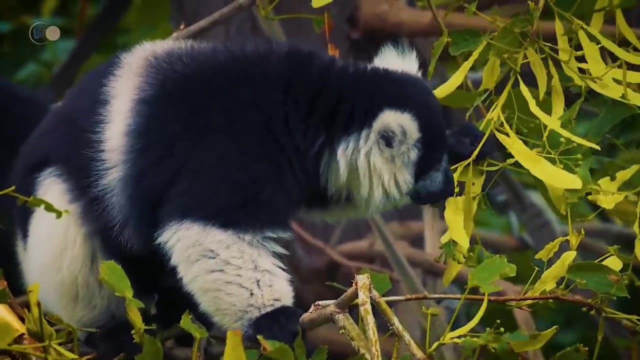 hold on to branches and grasp food. The eyes are located on the front of the face and are close together, Even if this position makes them lose the lateral view, which was a real asset to detect predators. it allows a binocular vision in three dimensions. 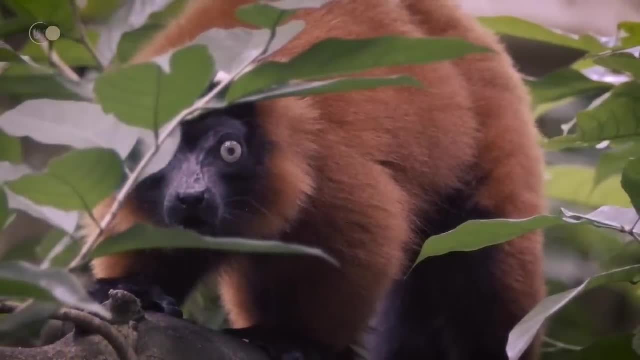 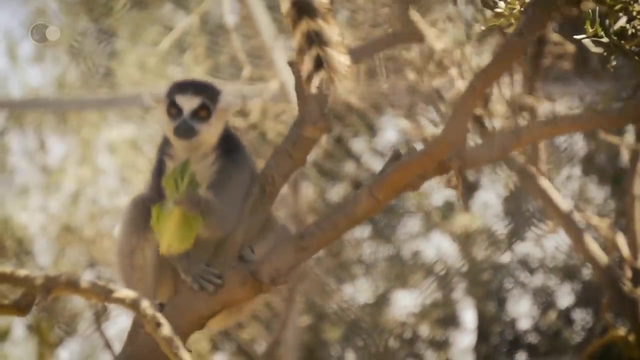 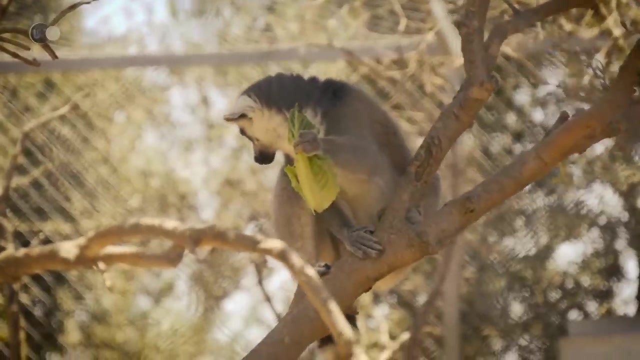 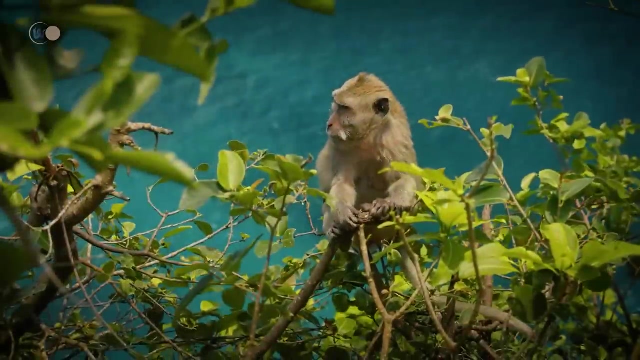 Thus the primates can jump from tree to tree by better evaluating distances and limiting the risks of falling. The whole of the upper cranium is remodeled, contributing to the increase in brain size In Asia. 45 million years ago, the first real apes appeared. 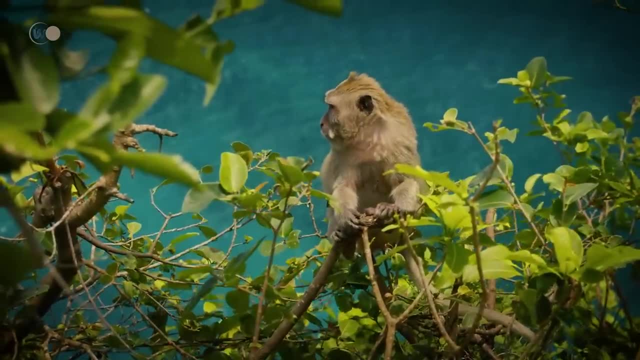 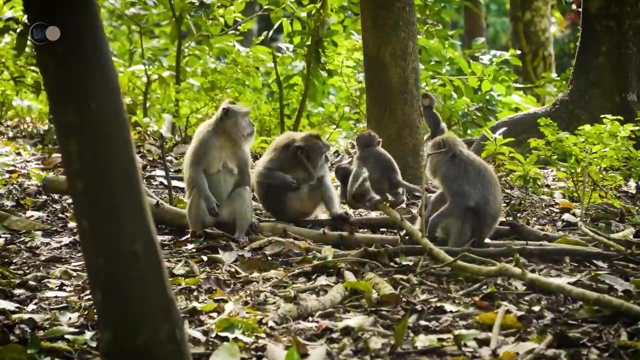 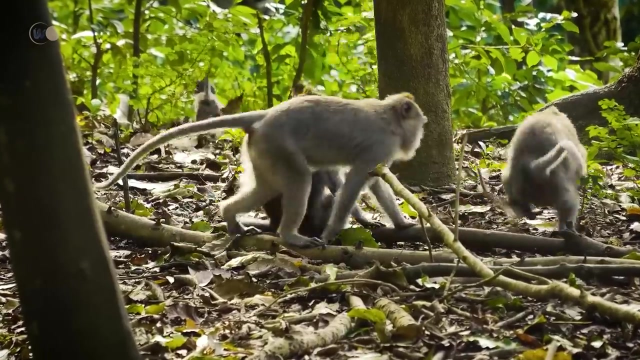 These omnivorous or vegetarian animals have the characteristic of having a large brain and an elaborate social behavior. In the heart of regions covered by vast swampy forests, primitive monkeys rub shoulders with small prosimians. Catapithecus, which lived 36 million years ago. 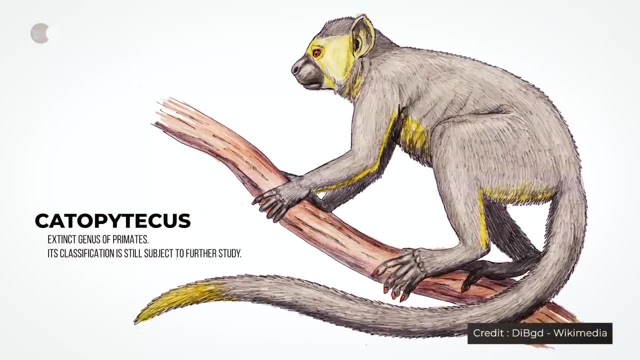 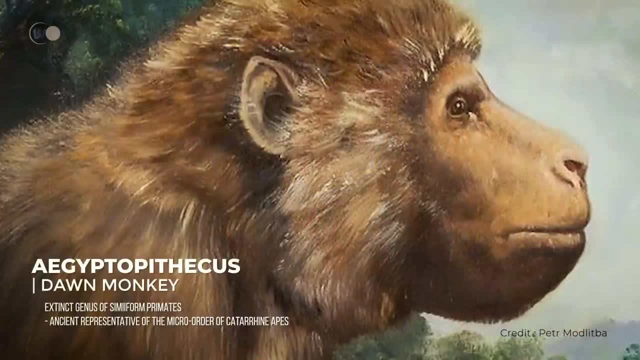 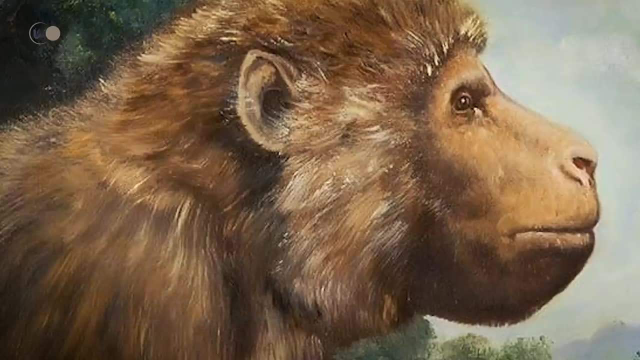 is the oldest of the early apes. The best known and largest is Egyptopithecus. This mammal, weighing 6 to 7 kilograms, or about 13 pounds, inhabits the rainforests that cover North America. It is somewhat similar. 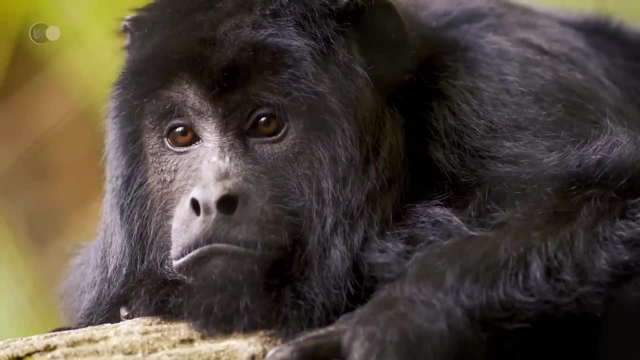 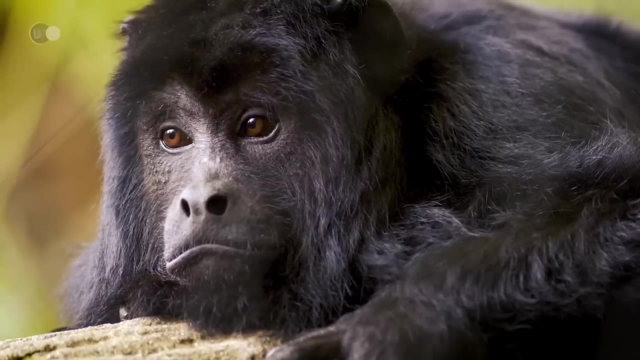 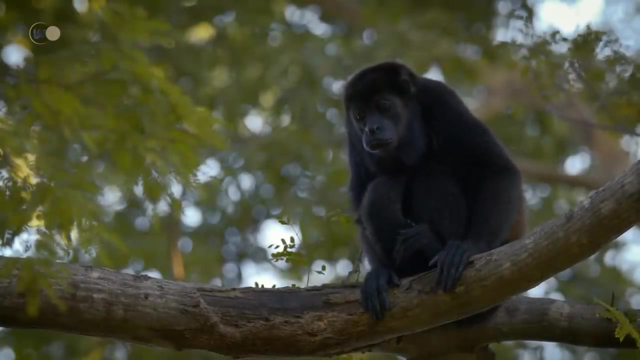 to the current howler monkey of South America. Egyptopithecus climbs trees, crawls on branches and feeds on fruit. It has a diurnal lifestyle. It has all the characteristics that differentiate simians from prosimians: Its cranial cavity. 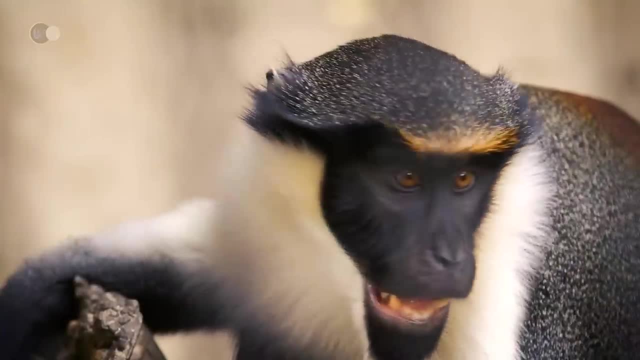 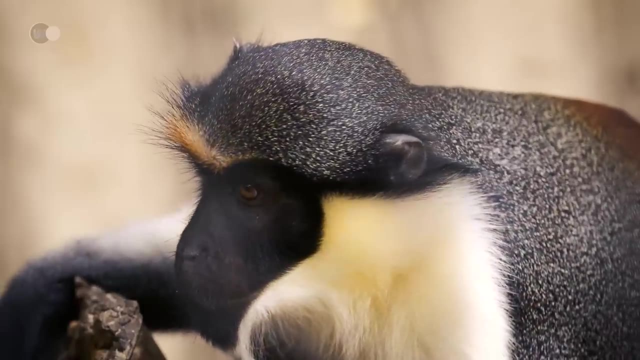 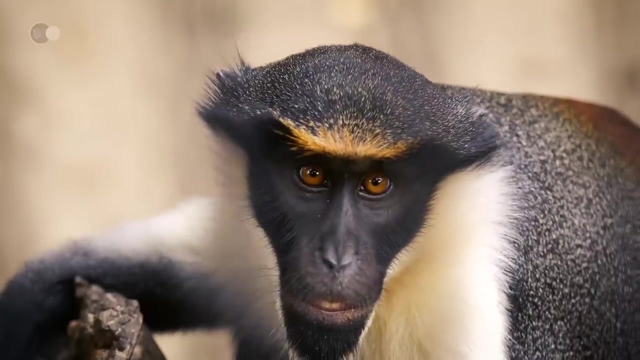 houses a larger brain. The orbit of its eye is totally closed, which isolates the eyeball from the temporal part of the brain. Its eyes are closer together, which has reduced the navel cavity and consequently the olfactory capacities. Its powerful mandible. 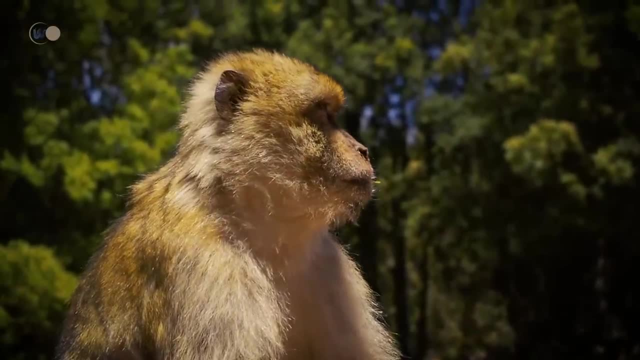 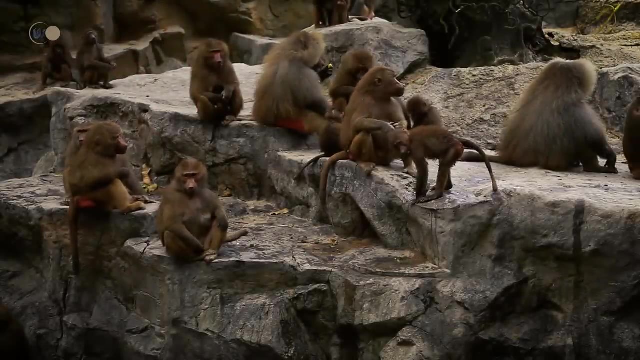 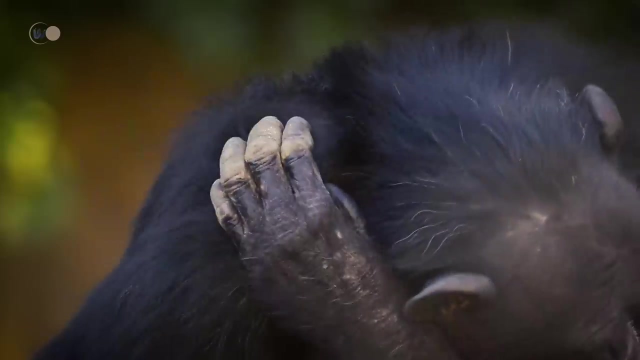 is provided with molars whose crown is relatively flat. The primates will show great diversity, but their anatomy keeps a great unity. Their five-fingered limbs have nails. The hand has an opposable thumb. It has been perfected and is used. 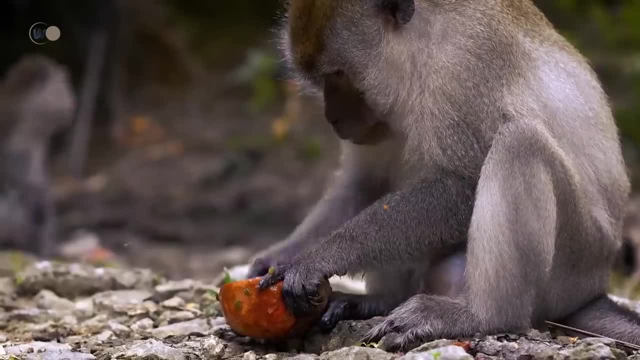 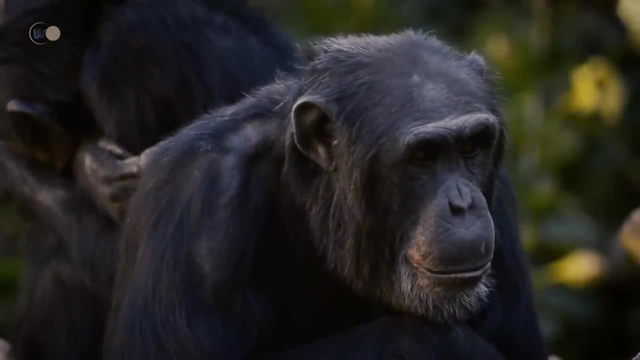 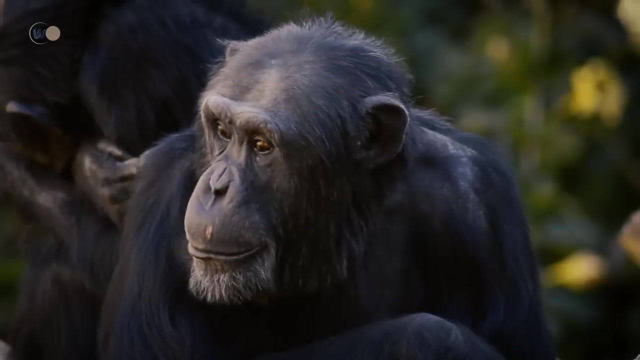 as a gripping instrument and as an organ of touch Sight, evolved and improved at the expense of the sense of smell. The orbits are directed towards the front, allowing a good binocular vision. Their complex social organization is also reflected in prolonged maternal care. 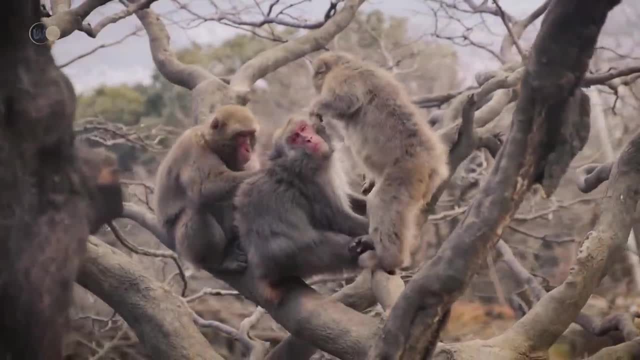 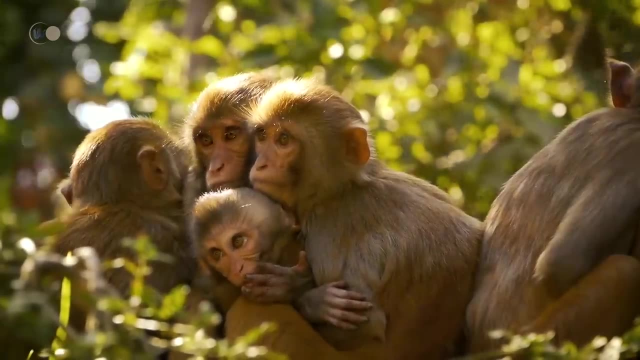 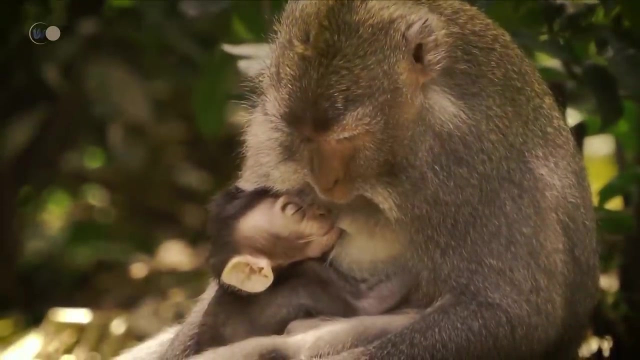 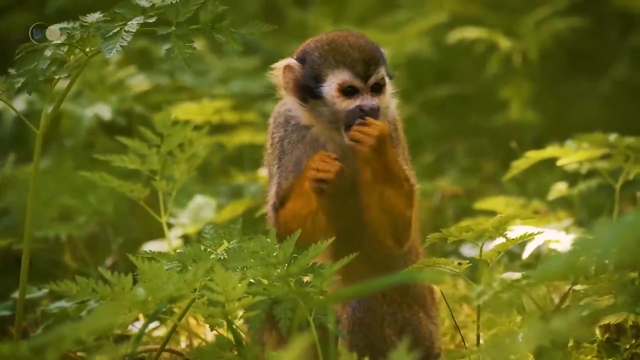 delayed sexual maturity and increased longevity. Primates generally live in groups ranging from a few individuals to several hundred members. Females usually give birth to a single calf, sometimes two. For physiological and behavioral reasons, primates range in size from 50 grams. 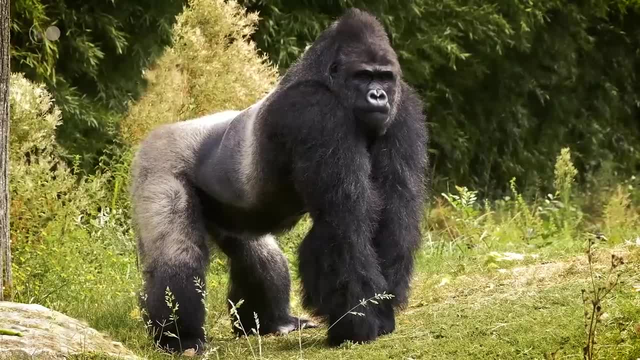 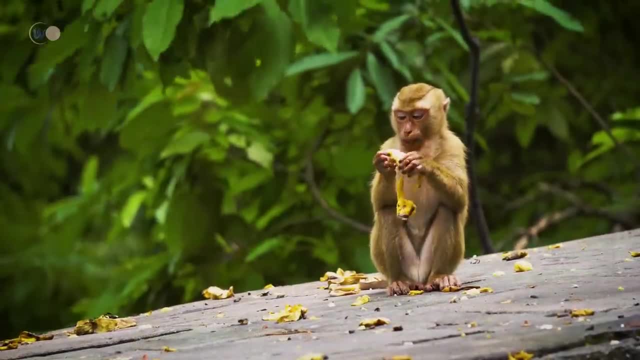 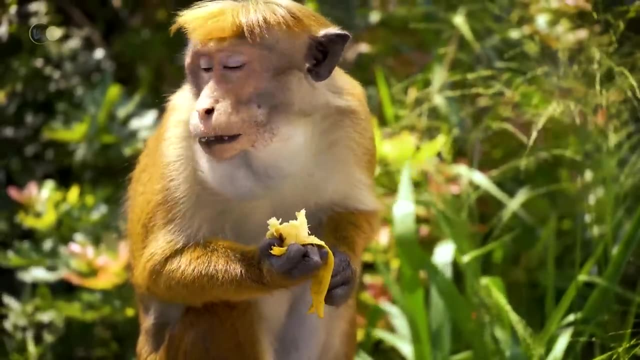 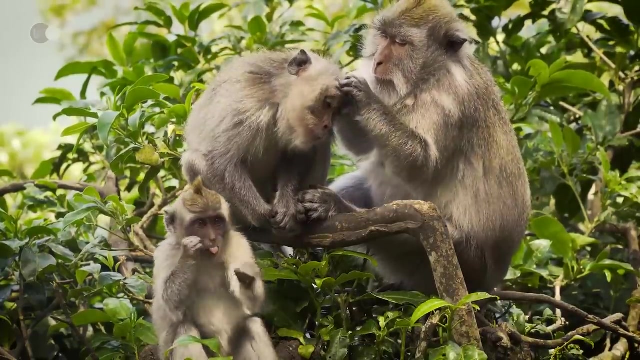 to over 100 kilograms or over 220 pounds. Their diet is diversified. Smaller specimens are more likely to be insectivorous or frugivorous, while larger specimens generally have an omnivorous diet. Primates thrive in tropical and subtropical regions. 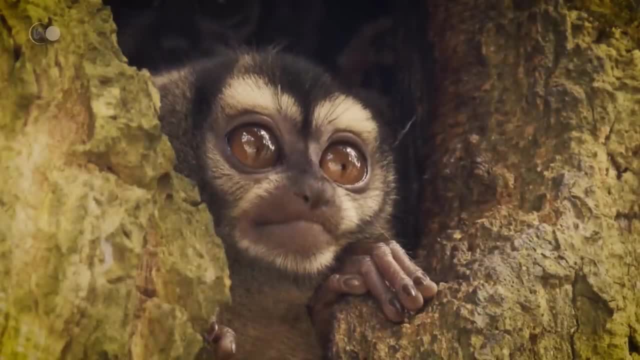 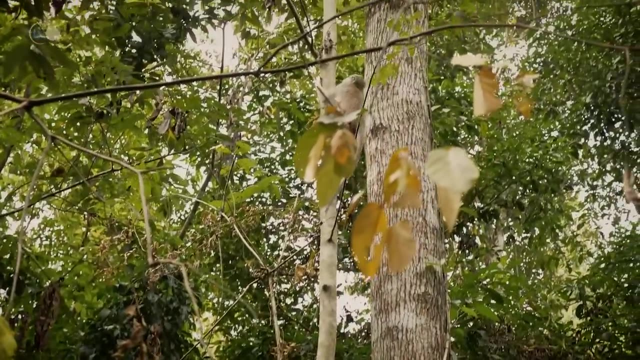 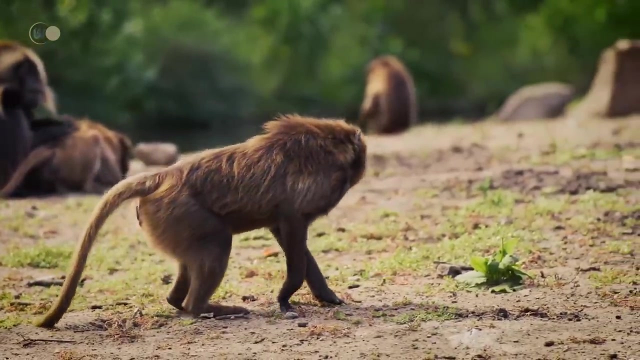 The majority of monkeys are diurnal, while prosimians live at night. Primates have a wide range of postures and modes of locomotion. In trees, some climb and walk on branches. On the ground, they adopt a quadrupedal gait. 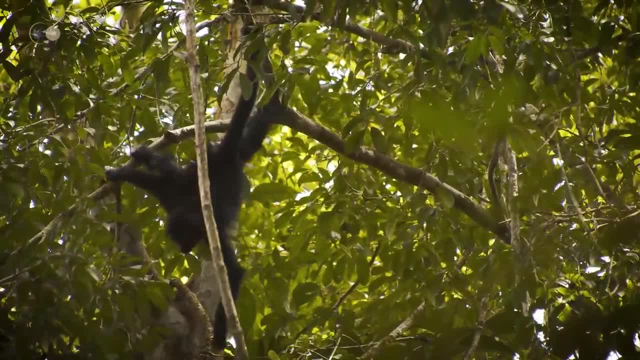 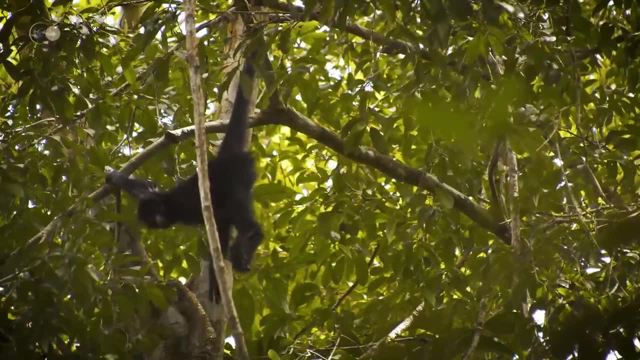 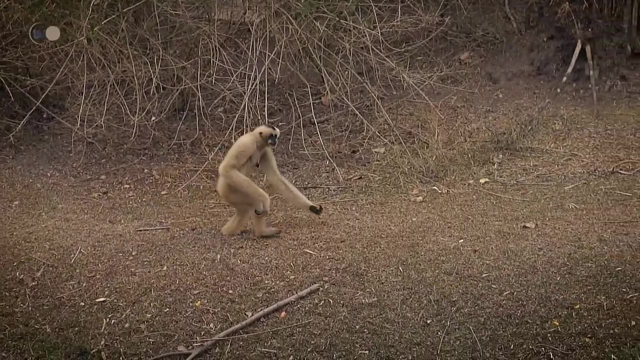 but are also capable of running upright and performing lateral jumps. Some species use their tails as a fifth limb to suspend themselves. Some great apes practice a hanging movement by swinging On the ground. their quadrupedal movement is particular, since they move. 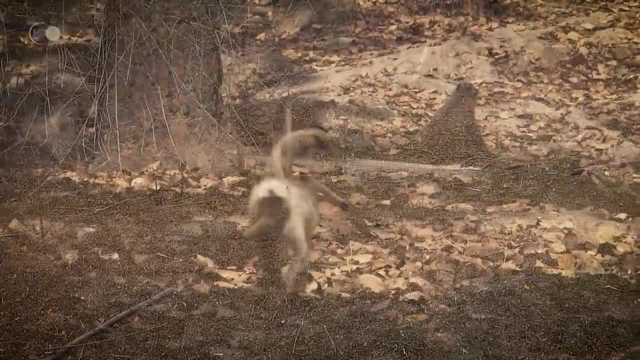 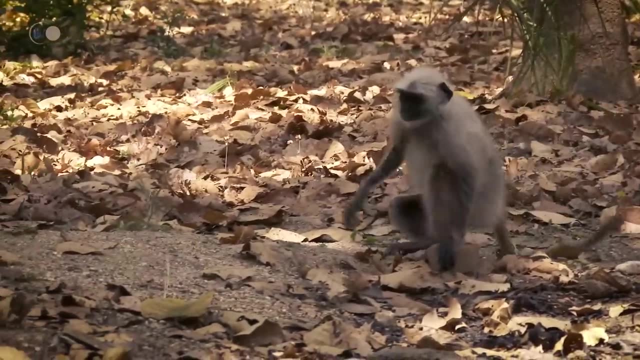 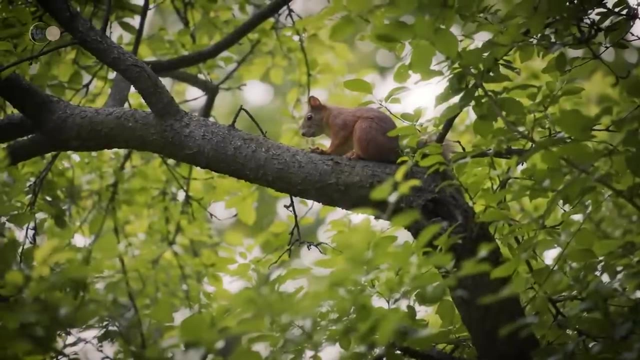 semi-erect by leaning on the second phalanx of the fingers of the hand. They all practice bipedalism. occasionally, Only man makes it his specialty. Some small mammals begin to exploit a new environment, the treetops Up. there is inexhaustible food. 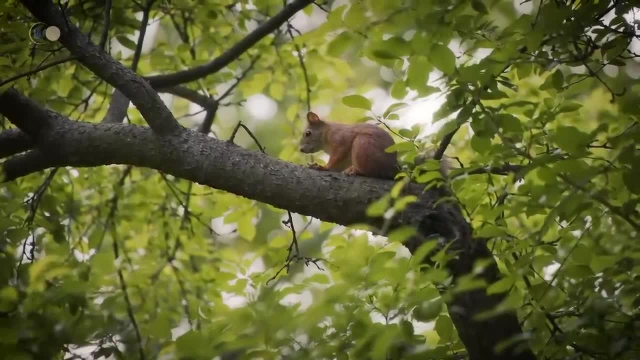 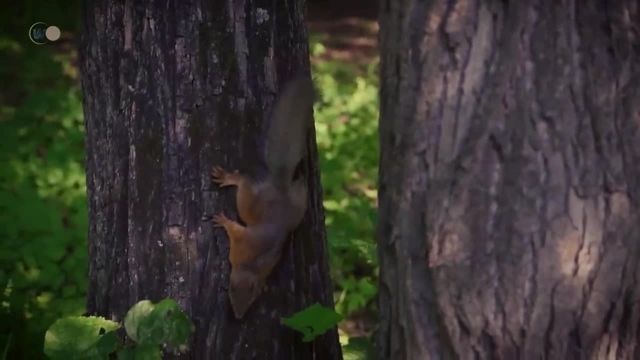 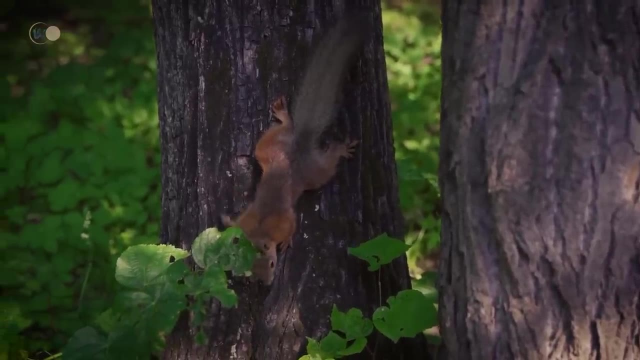 and safe shelter from predators. However, living in the treetops involves three-dimensional movement, not the two-dimensional movement of terrestrial animals. There is therefore an additional danger: the risk of falling. The little people of the high branches will display particular adaptations. 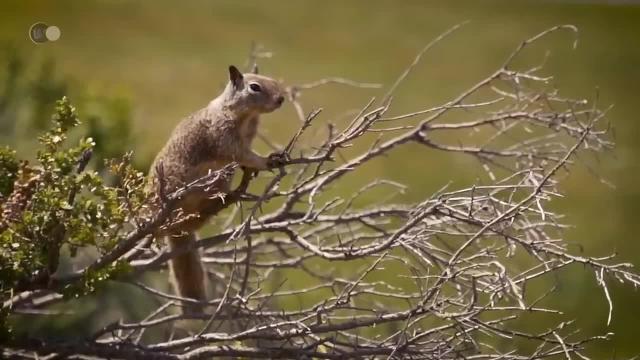 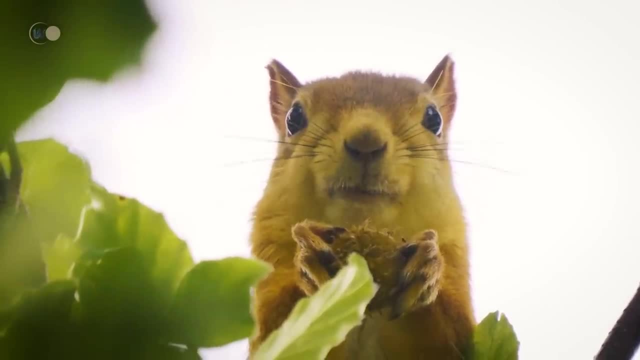 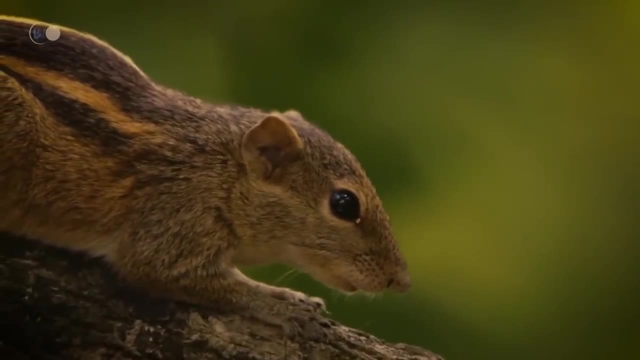 such as a large brain or eyes directed towards the front, allowing to elevate distances precisely. Color vision is also an innovation that allows the animals to easily spot fruits and young leaves more tender and nutritious. Carpalus is a small, hamster-sized mammal. 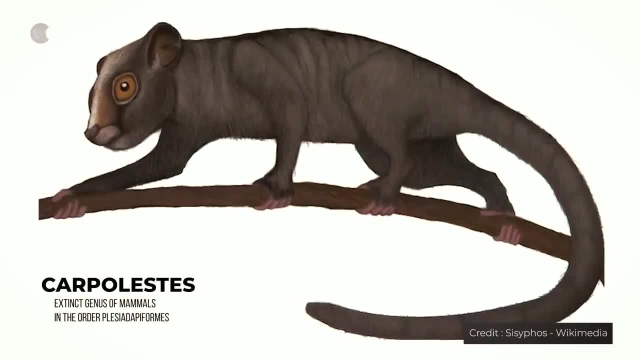 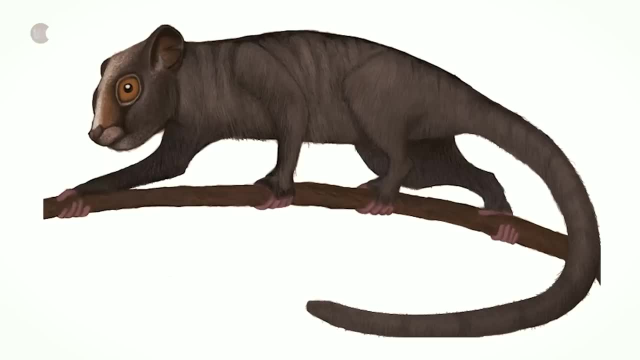 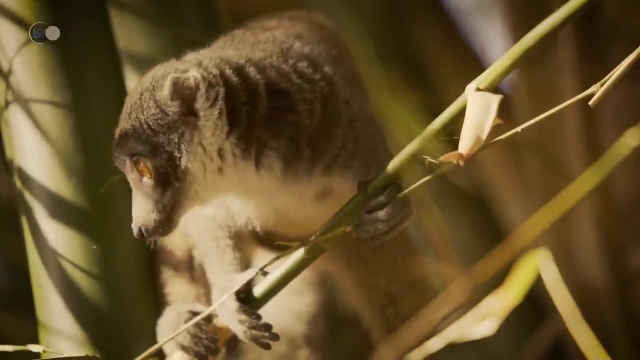 with rodent-like teeth. Its long fingers and opposable thumbs allow it to climb easily to the top of trees. Its elbows are not flexible enough for it to leap from branch to branch. Its eyes, located on the sides of the head, do not allow it. 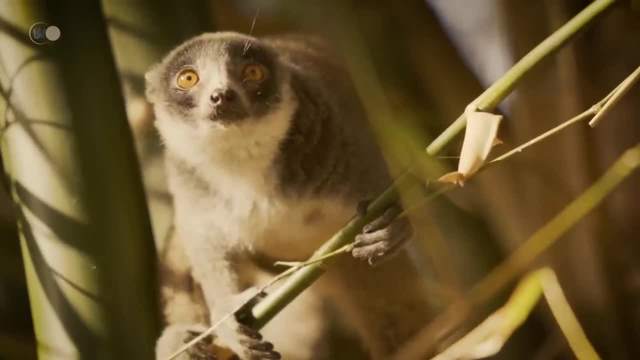 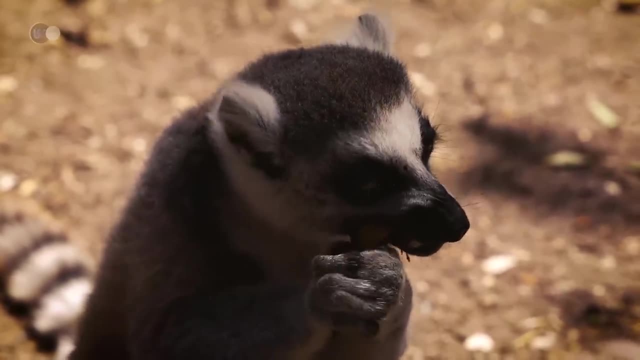 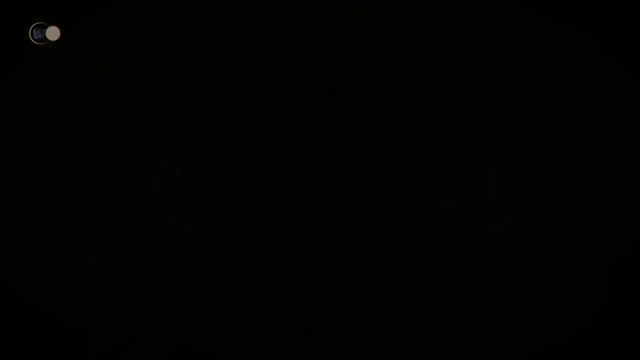 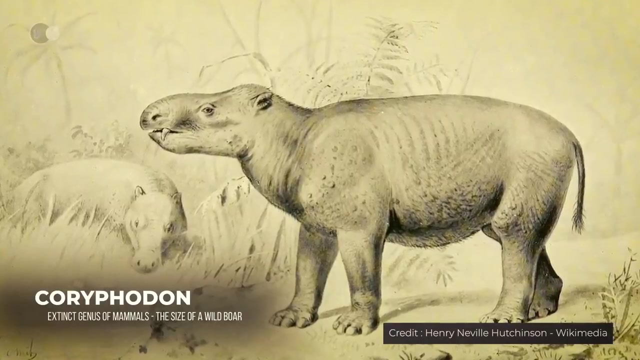 to evaluate distances with great accuracy. Carpalestes is a close relative of the first apes, but is not a true ancestor. Coryphodon is a large amphibious herbivore Like modern hippos. it lives in swamps and feeds on aquatic plants. 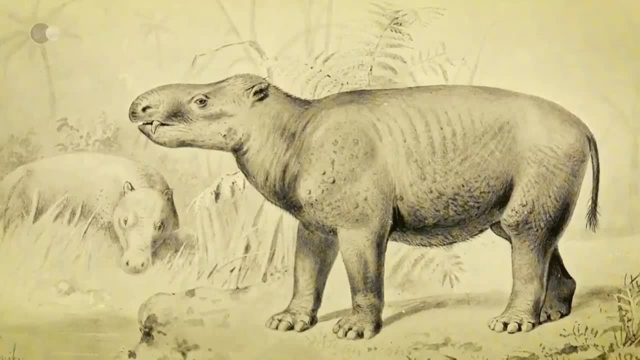 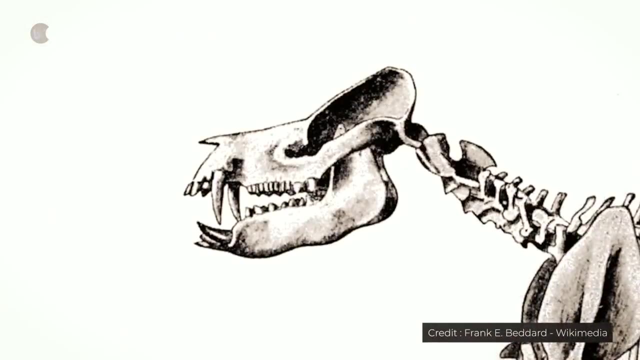 Its size is close to that of a boar and it can weigh up to 500 kilograms or 1,100 pounds. Its two tusks are not very developed At this time. it is considered a large animal compared to the average size of humans. 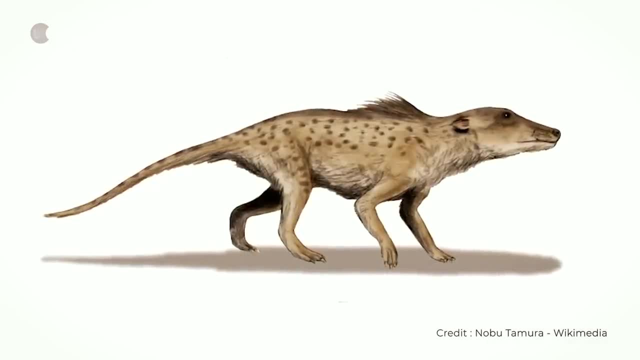 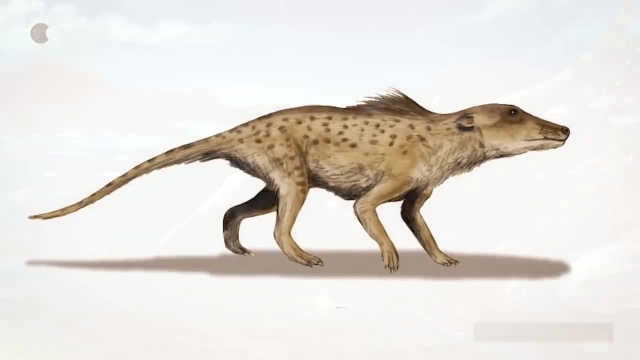 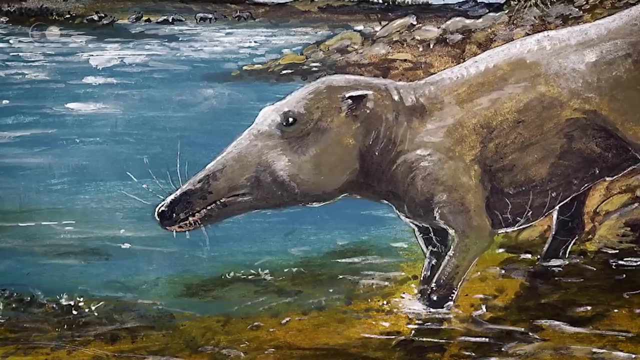 The ancestors of whales and dolphins literally galloped on land. Today, it is difficult to imagine how terrestrial quadrupeds could have turned into cetaceans. Despite its name, which means king of reptiles, Bacillusaurus is a mammal. 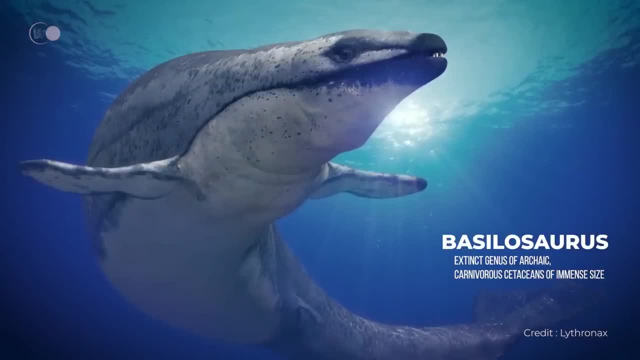 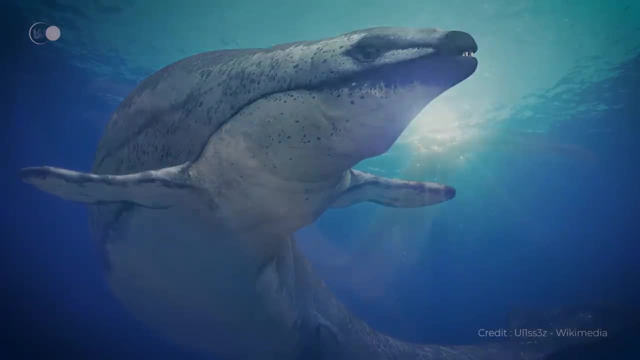 The whale-sized animal has a jaw filled with teeth. It does not yet have blowholes, but nostrils located in the middle of the snout, forcing it to take its head out of the water to breathe. It has two small hind legs. 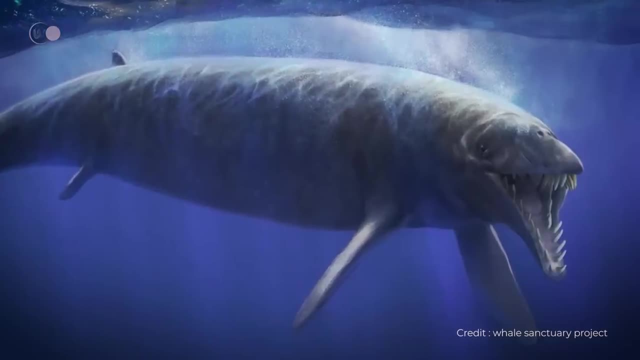 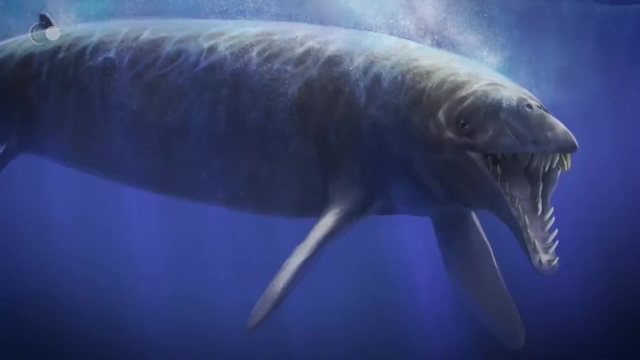 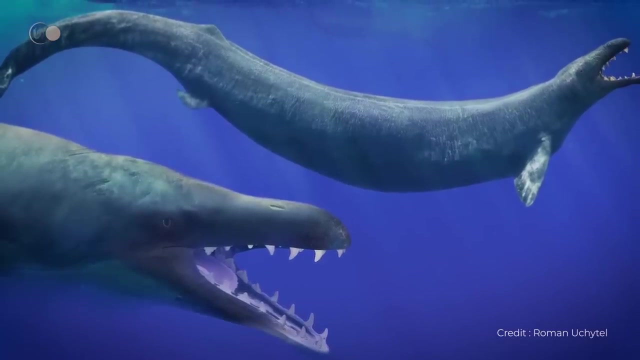 which are not used to walk or swim. Its long tail and its arms, in the shape of fin, help it to propel itself to move. Bacillusaurus, like other cetacean ancestors, exploits the coastal environment and feeds on fish crabs. 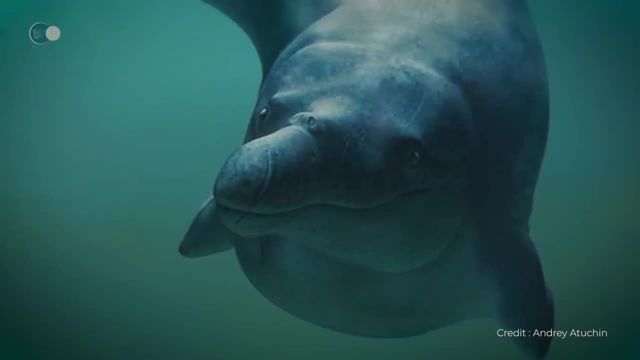 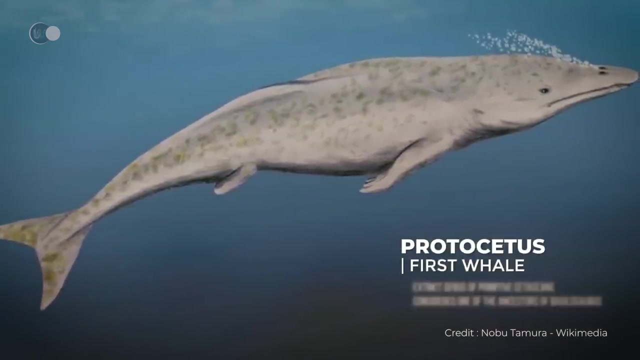 and mollusks. The evolution pushed him to adapt to the marine environment. His hind legs progressively reduce in size and its arms and tail become flippers. Its nostrils migrate towards the top of the head to give the vents. The ear evolves. 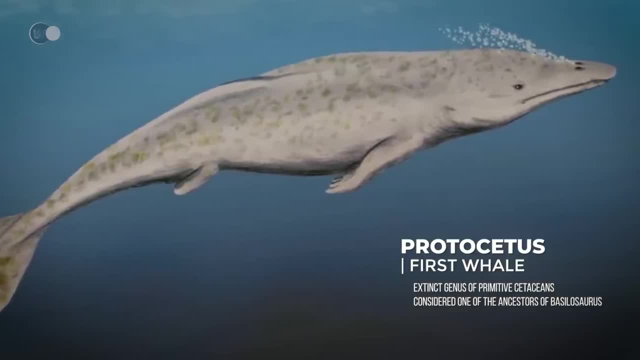 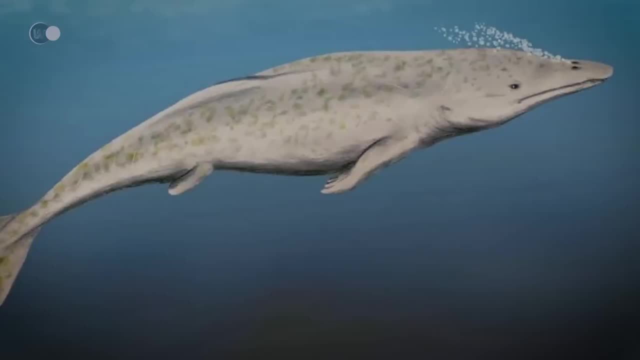 to allow the animals to properly hear sounds. underwater Protocetus is a kind of primitive cetacean. It is 2.5 meters or 8 feet long. Its legs, which it uses as flippers, are rather small, but allow it to move. 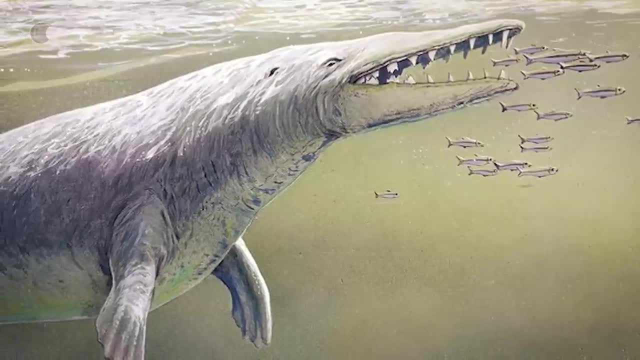 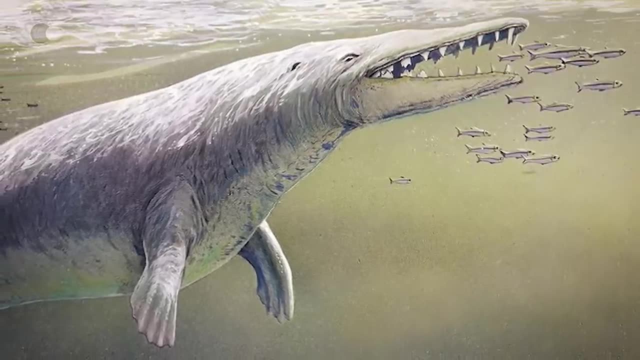 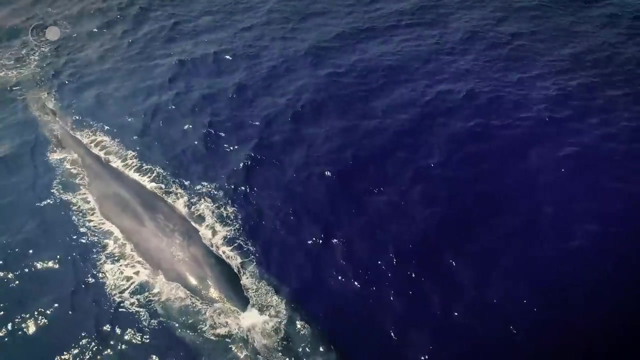 on the ground. Its long jaw has very sharp teeth. The structure of its ear allows it to hear well underwater, but certainly not to practice echolocation. Its nostrils are halfway to the snout, which is the first step on the way to the top. 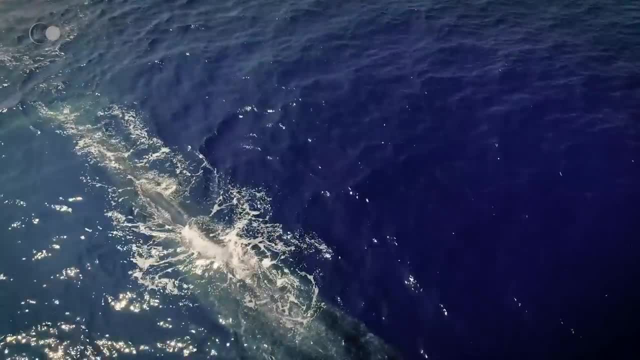 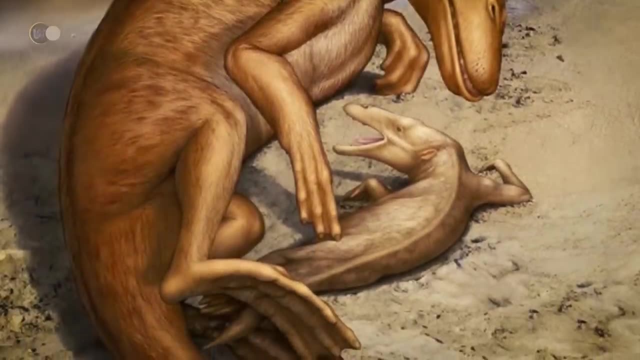 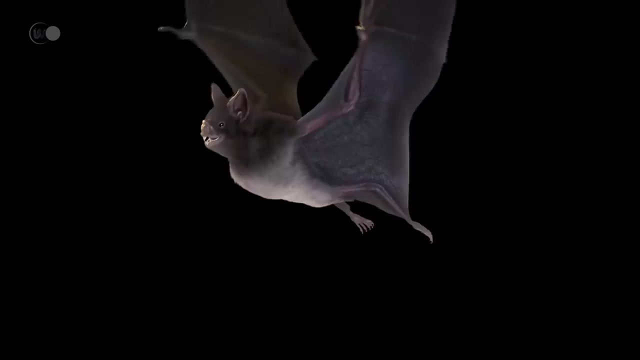 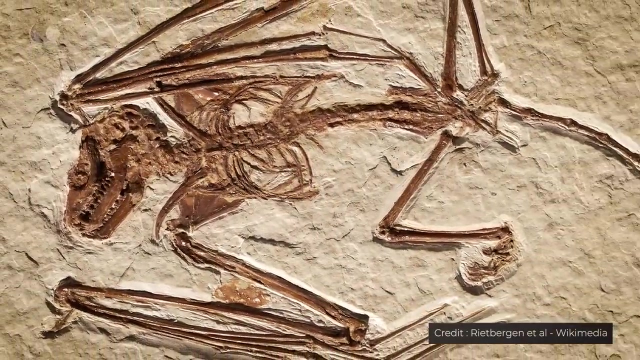 of the skull in modern cetaceans. Amphibious life is still relevant for these primitive animals. Some females still give birth on land. Bats appear with a charonecteris. This animal already has the appearance of modern bats. Its wings can reach. 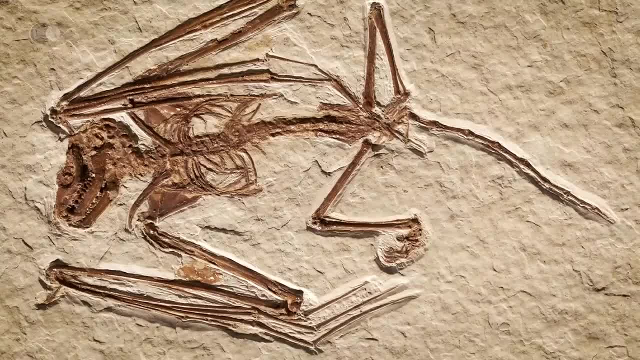 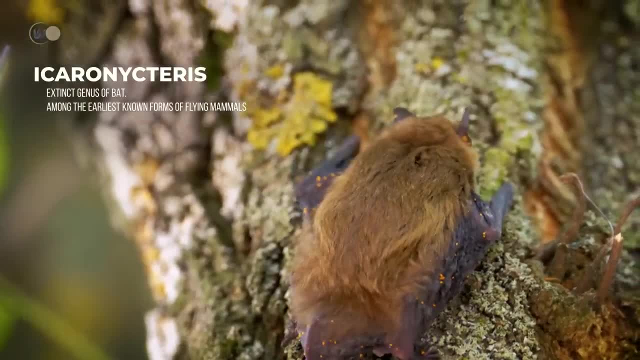 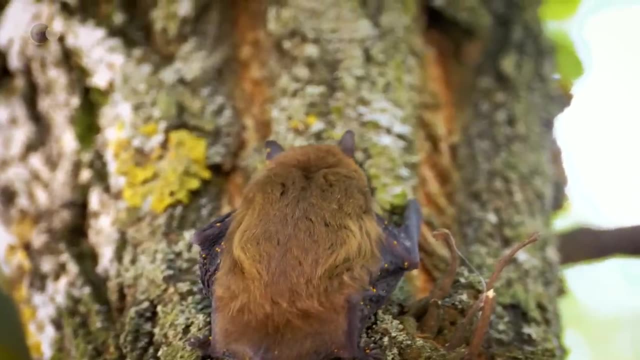 up to 35 centimeters or 14 inches in span. Its long tail serves as a rudder. Its legs are still too small to allow it to hang upside down. It wears a fur, It likes warm climates and feeds on insects, Even the oldest bats. 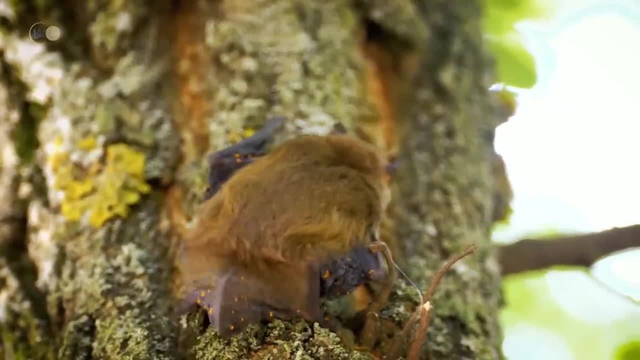 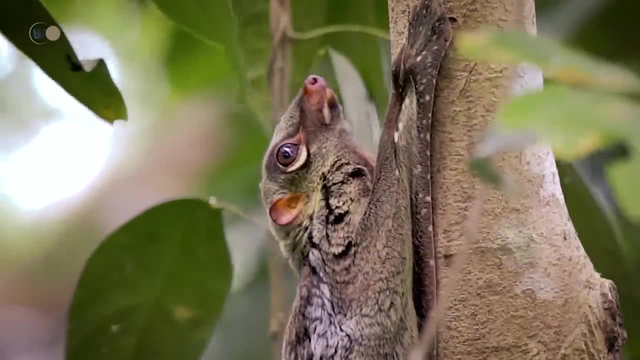 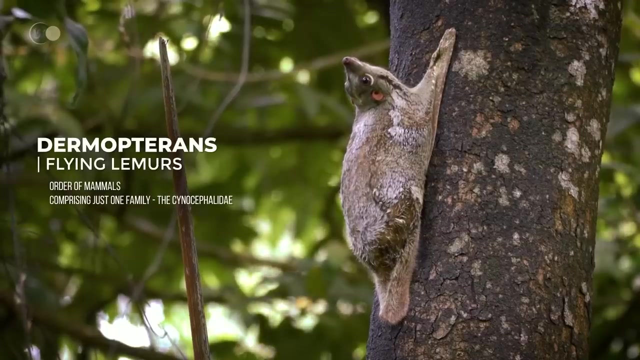 are already able to flap their wings. Dermoptera, or flying lemurs, are an order of mammals. They live in trees and are best equipped for gliding. When they launch themselves from a branch, they extend their four limbs in such a way. 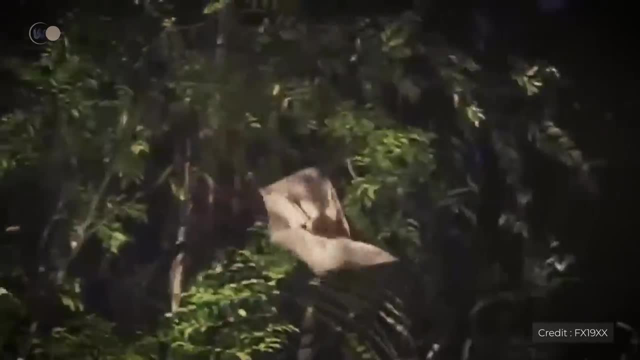 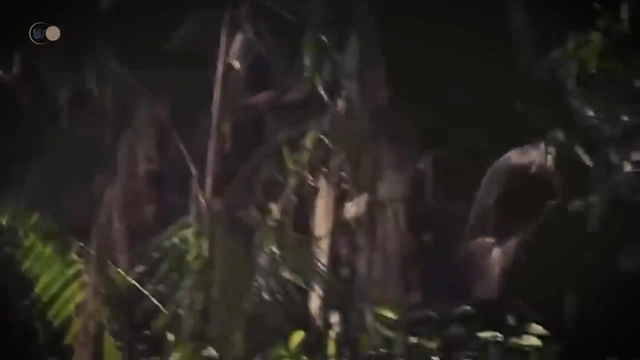 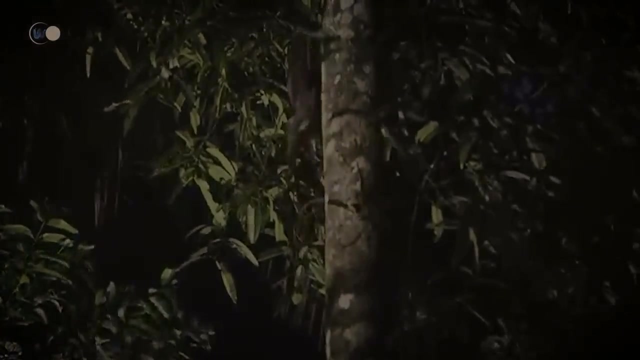 as to stretch a sail of skin that connects their wrists, ankles and tail. This allows them to glide more than 100 meters or 330 feet. Palms, flowering trees and conifers thrive. A group of plants will make its appearance. 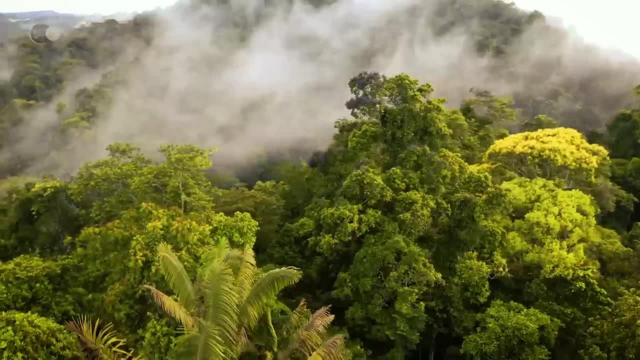 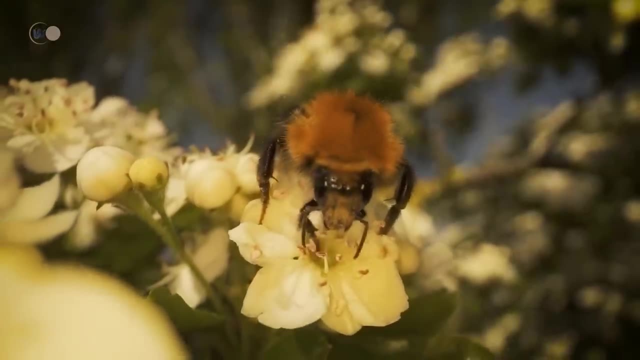 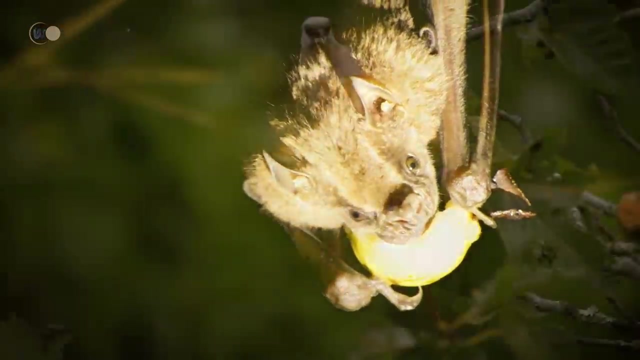 in the plant world. They are the herbaceous flowering plants. Their success is linked to the evolution of pollinating insects. Animals that eat seeds and fruits, such as bats and birds, have also contributed to the spread of plants. Herbaceous plants have a secret. 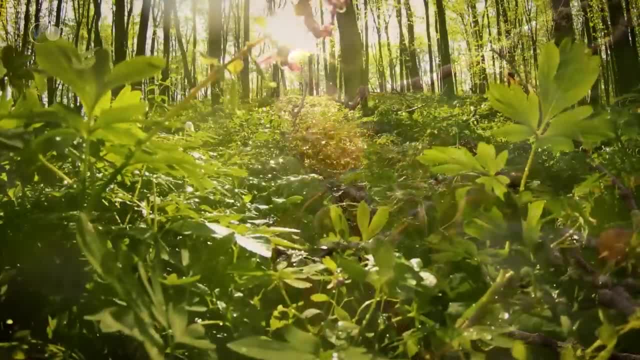 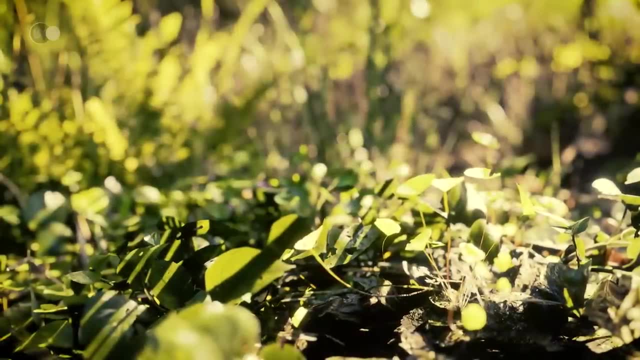 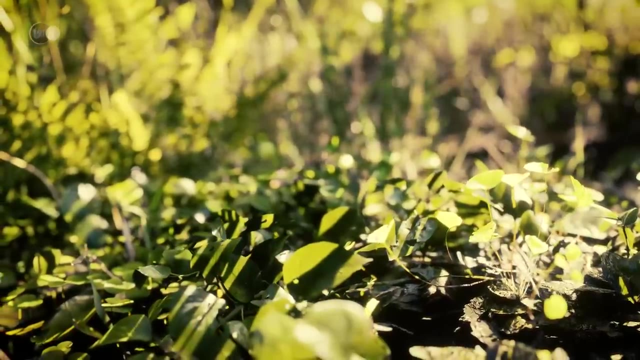 They have the ability to survive and thrive even when cut regularly by animals. Cutting off the tops of their leaves does not damage their growth. They even survive severe harvesting. Expanding grasslands support the survival of herbivorous mammals. Grasses include. 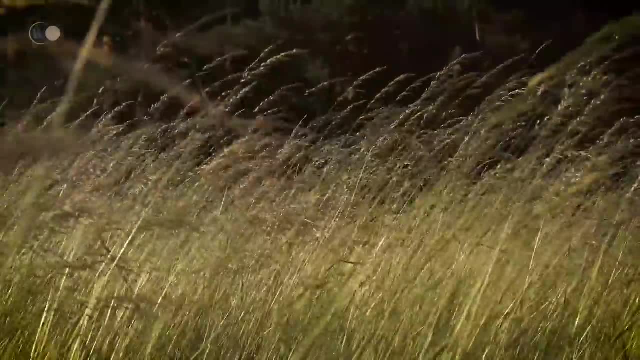 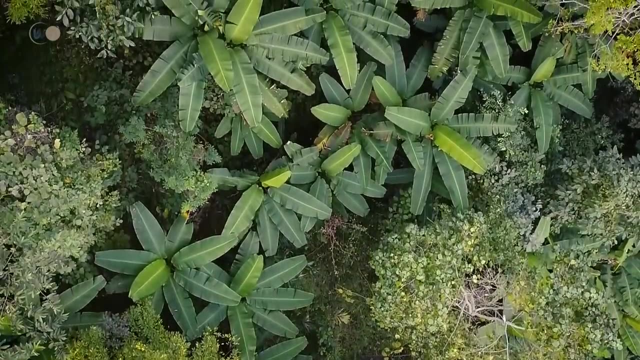 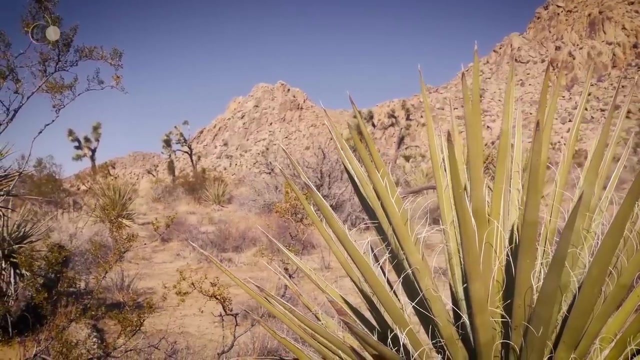 most of the species commonly called grasses and cereals. They are generally herbaceous plants, whether annual or perennial. They will adapt to a wide variety of environmental conditions, ranging from lush rainforests to arid deserts, from cold mountain climates. 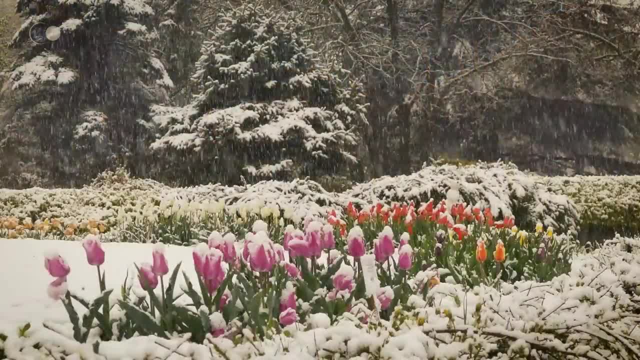 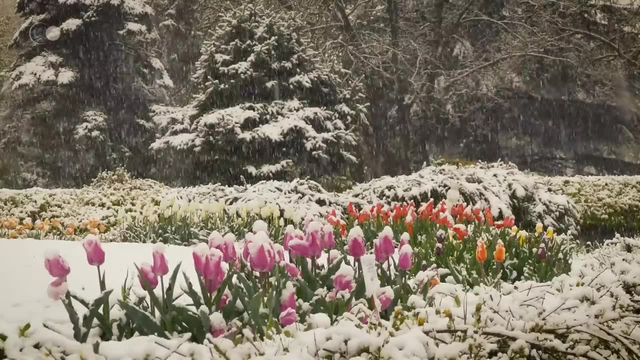 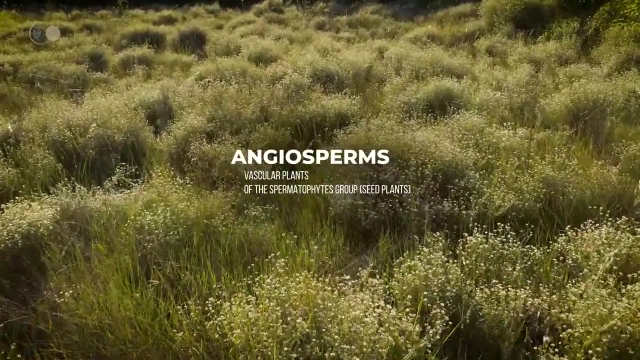 to tropical climates. They are a valuable source of food and energy for wildlife. Grasses are angiosperms. The flower is a complex structure in which the male and female reproductive organs are grouped and enveloped. The female part will give the fruit at maturity. 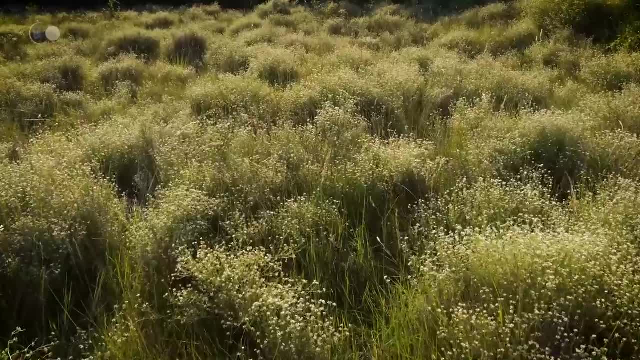 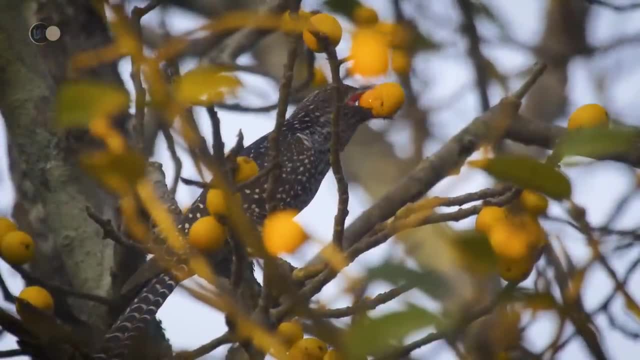 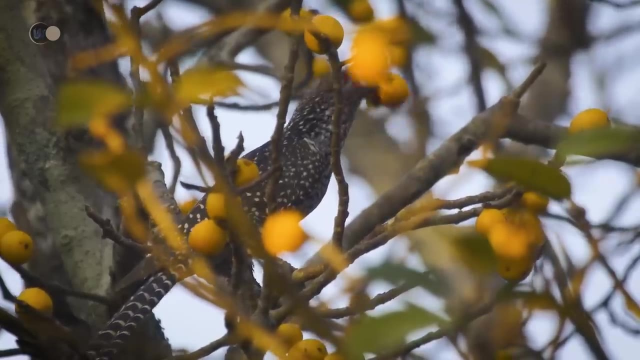 but only after fertilization. It is the fruit that characterizes the angiosperms. It participates in the dissemination of seeds through various animals, wind and water. The plants were able to disperse on the two continents before the total separation of Gondwana. 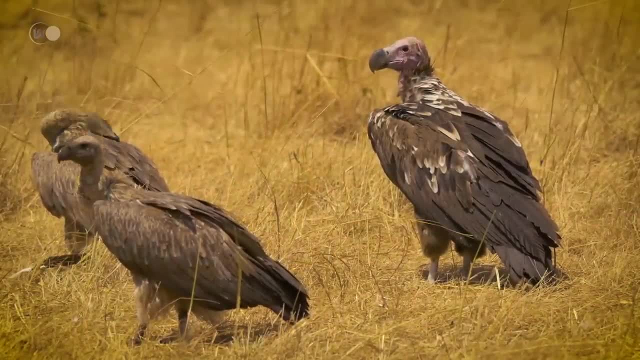 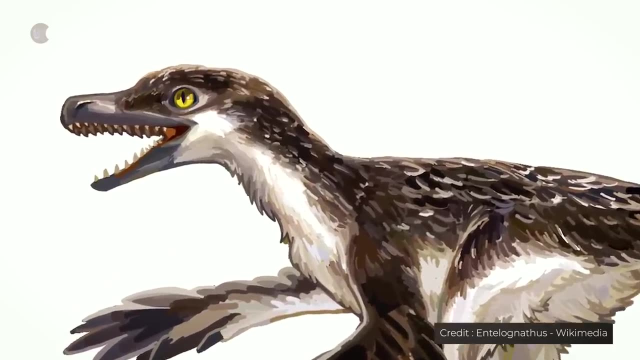 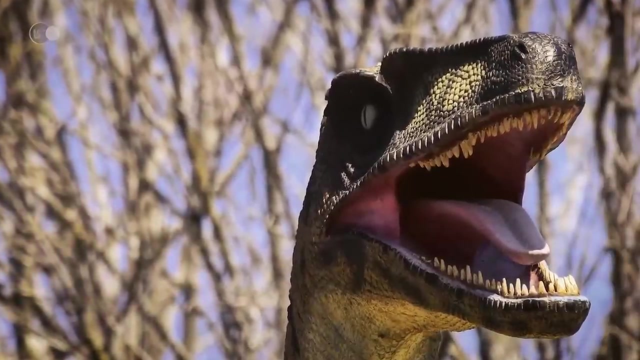 Birds are small feathered flying theropod dinosaurs. Their ancestors were land predators, true hunters of the Jurassic lands. They did not fly. Flight is an adaptation now indelibly associated with birds. The survival of some species can sometimes be surprising. 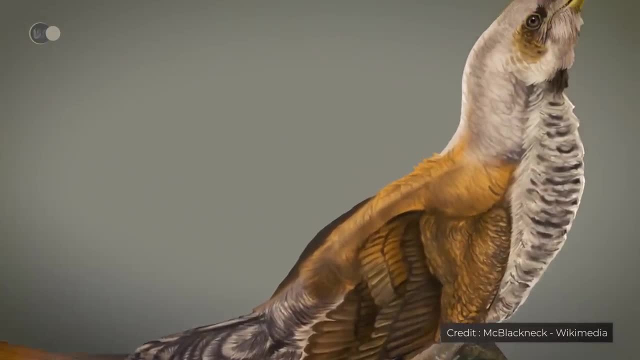 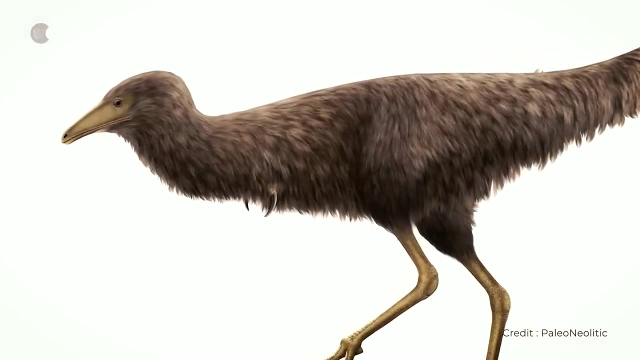 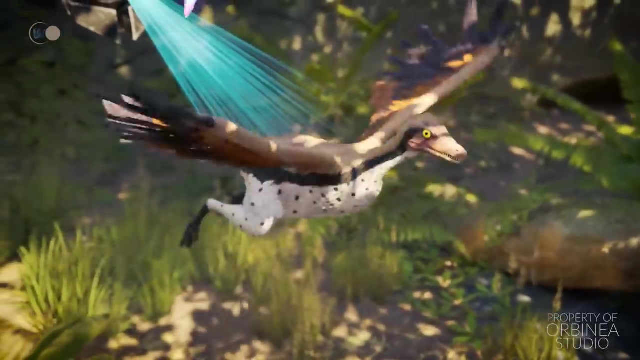 Before the impact of the meteorite, birds already had a long history behind them. The oldest known Archaeopteryx appeared at the end of the Jurassic period, about 150 million years ago. This animal has the body and teeth of a reptile. 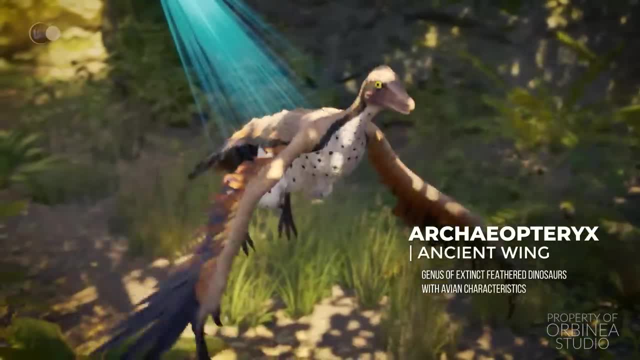 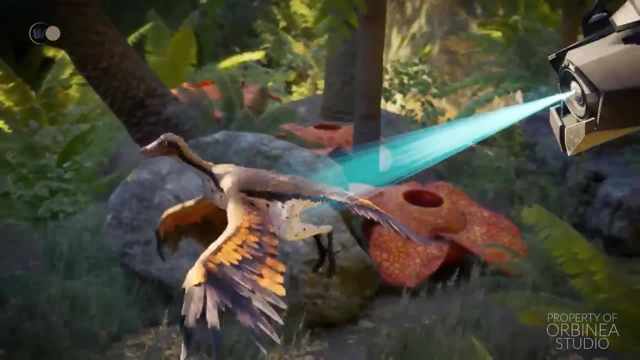 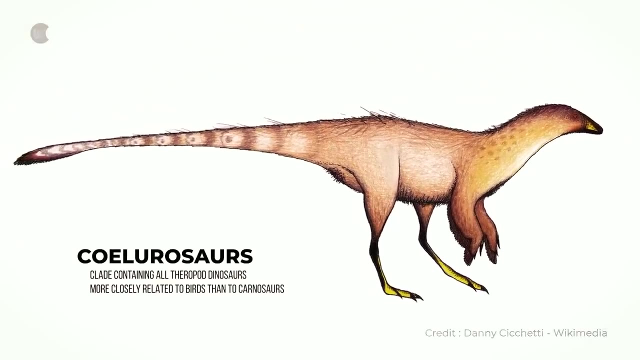 combined with the feathers of a bird, It represents the missing link between reptiles and birds. Archaeopteryx probably descended from a small terrestrial cholerasaur. These hollow-tailed reptiles include small, light and fast carnivores like Companionatus. 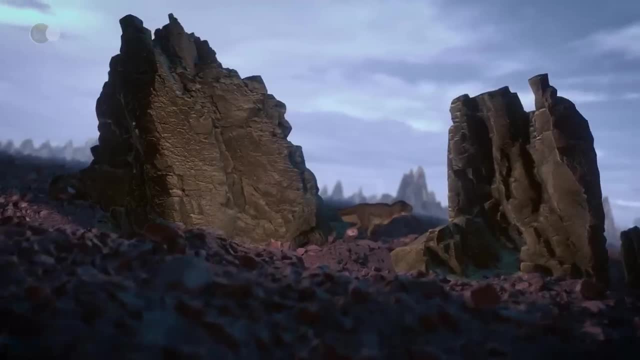 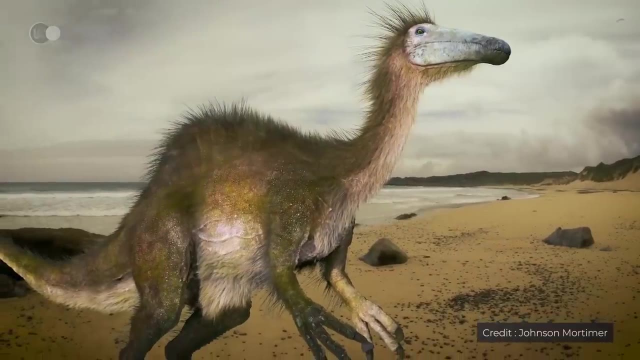 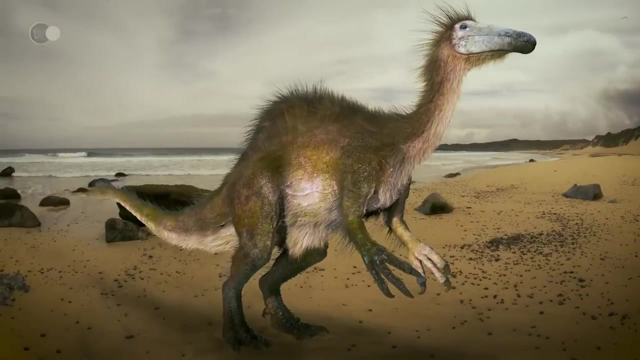 but also the huge and famous Triceratops. The reptiles are known for their huge and famous Tyrannosaurus. Some cholerasaurs were covered with feathers and could fly. Their skeleton is very similar to that of birds- Feathers in flight. 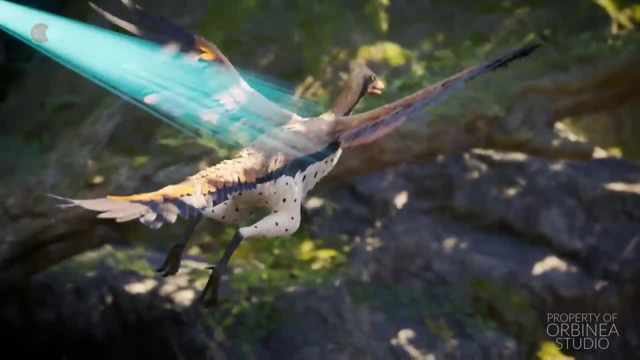 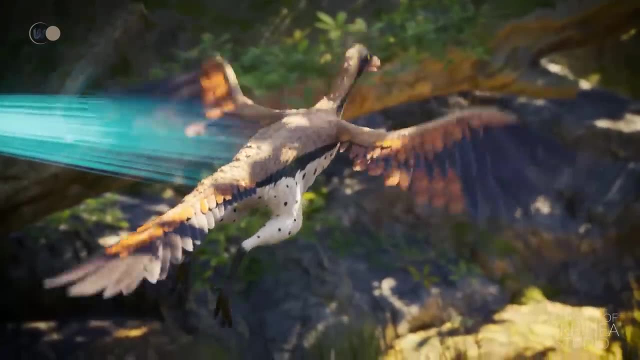 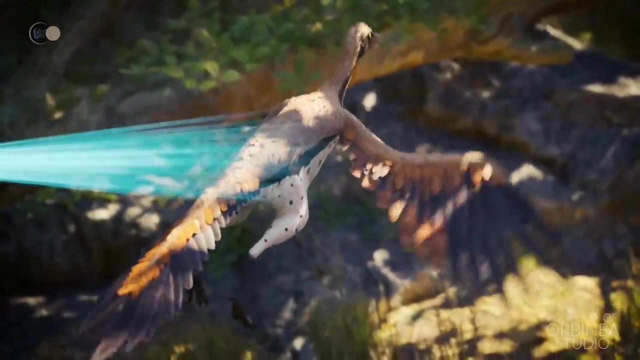 did not appear all at once, but were acquired through evolution. Feathers are, according to some theories, an evolution of reptilian scales Before it became the modern feather as we know it today. the whole form and function of ancestral feathers were different. 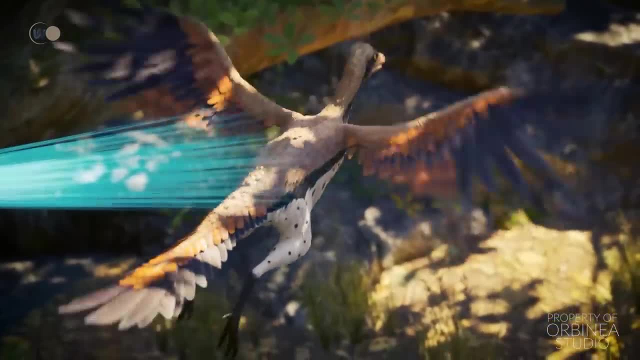 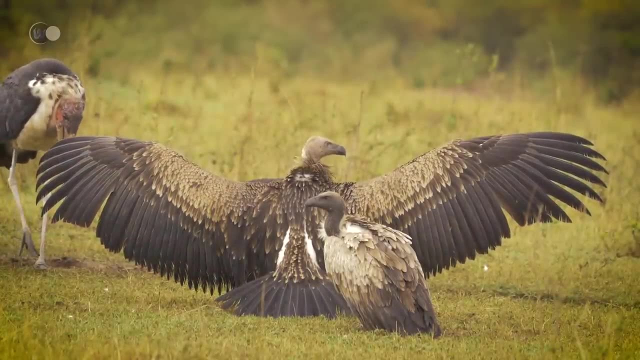 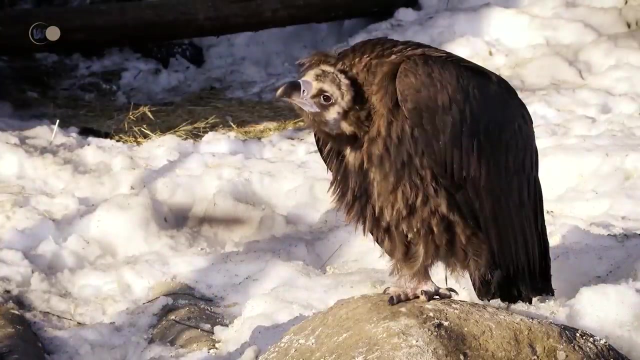 The archaic function of the feather is its insulation. By being covered in feathers, the animal is able to retain body heat and protect itself from the cold. Some of the earliest feathers have a configuration that is no longer seen today. They have a more unstructured 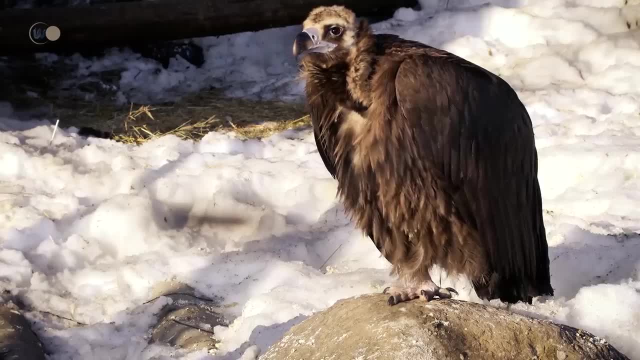 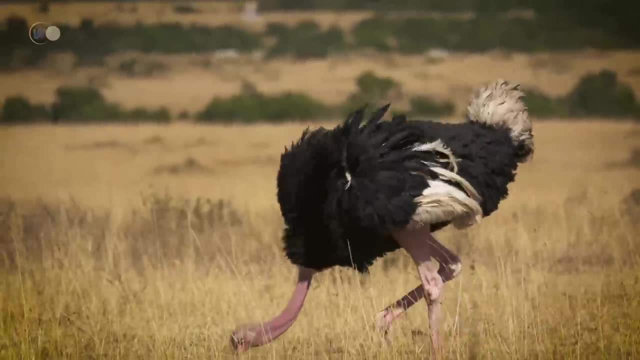 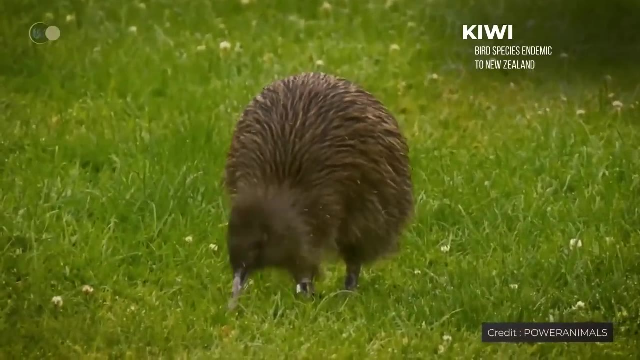 down-like branching and configuration. It is as if a number of filaments had been gathered and fused at their base. The kiwi, a species of bird that is currently unable to fly, has feathers that look like hair, as if they had been simplified. 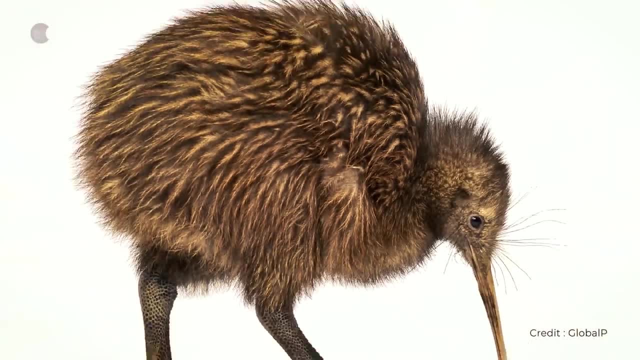 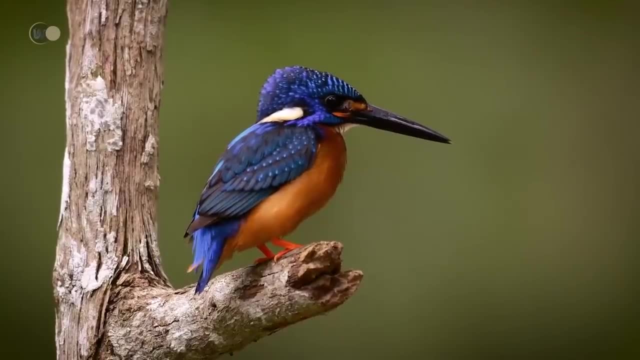 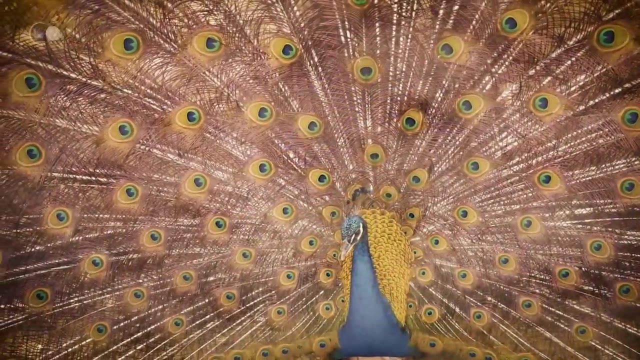 because they are not needed for flight. Feathers also play a role in display or camouflage. They can also be used for recognition between groups of individuals or as mate attraction partners. Feathers are also protective, keeping eggs out of the sun or warming them by trapping. 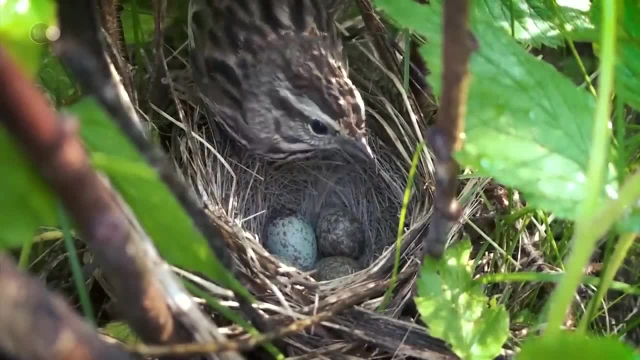 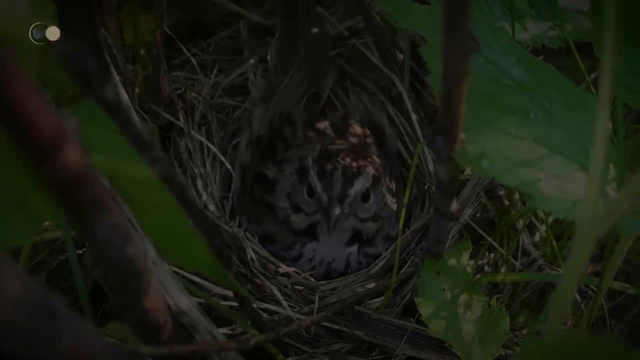 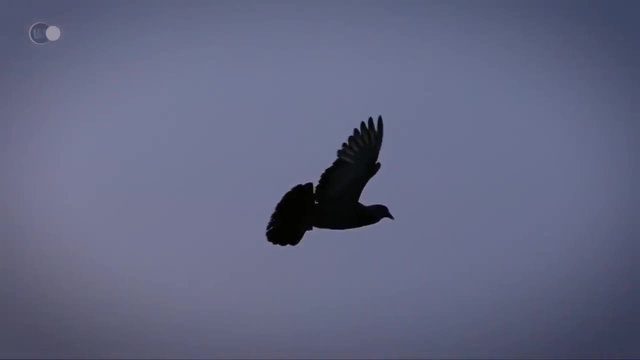 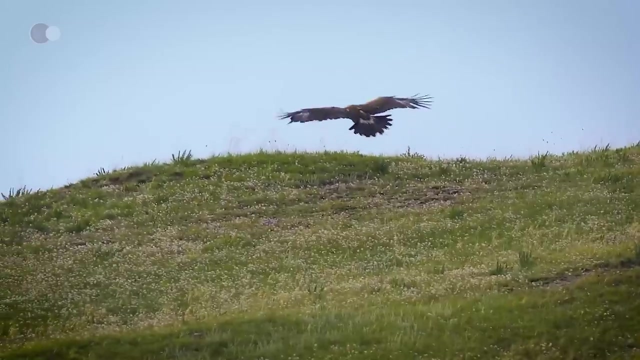 air. They can be used during sexual parade. Flight is defined as the active production of energy that propels the animal through the air using its own power. This requires certain physiological characteristics, such as hollow bones, a strong sternum and a perched foot. 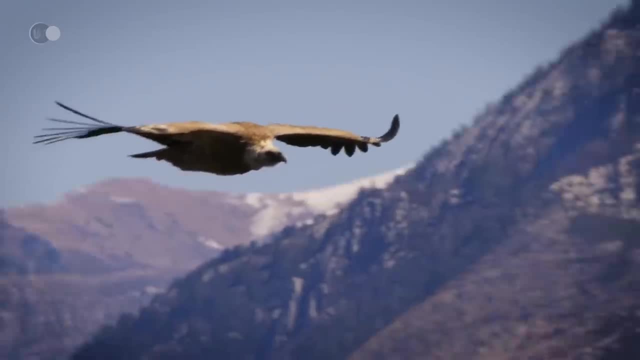 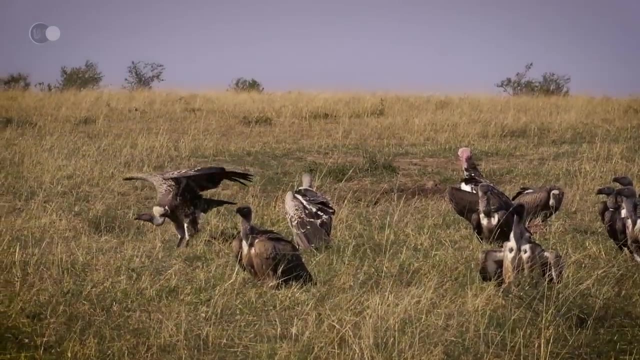 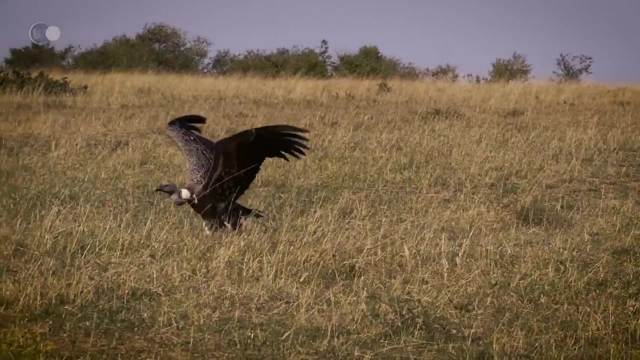 In order to fly, the animal must have an airworthy wing. It must be able to generate a vortex wake that propels it forward. Its neuromuscular coordination must allow it to navigate efficiently and its metabolic level must support flight for long periods. 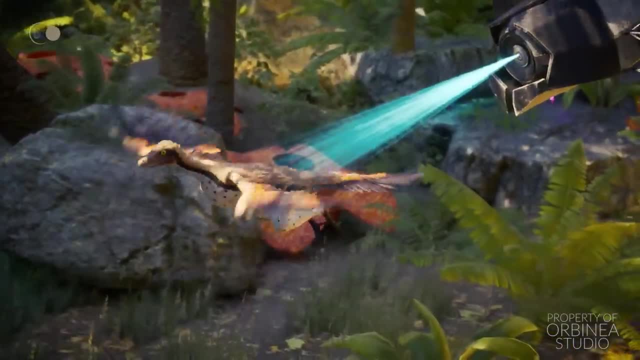 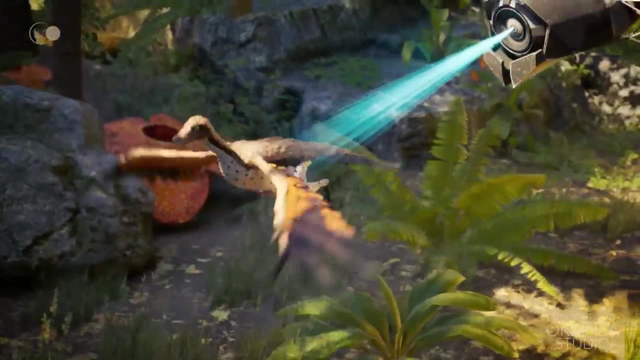 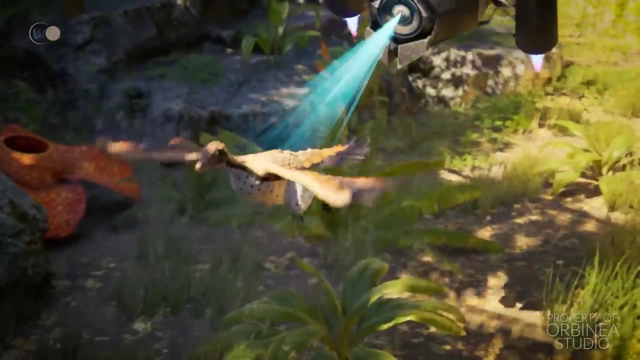 Archaeopteryx already possesses an airworthy wing which makes it capable of generating the flight stroke. It has an ear canal reflecting the ability to negotiate three-dimensional space, which is particularly useful for an animal traveling through the air. It would seem that its capacity 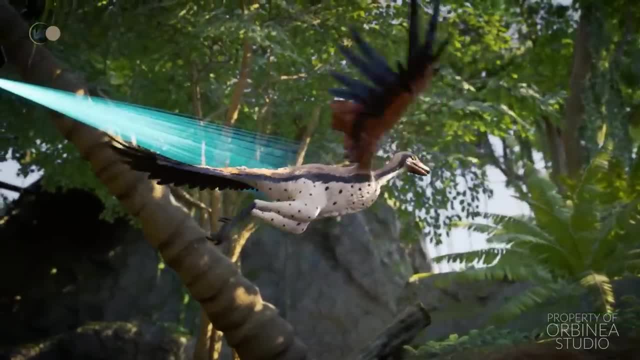 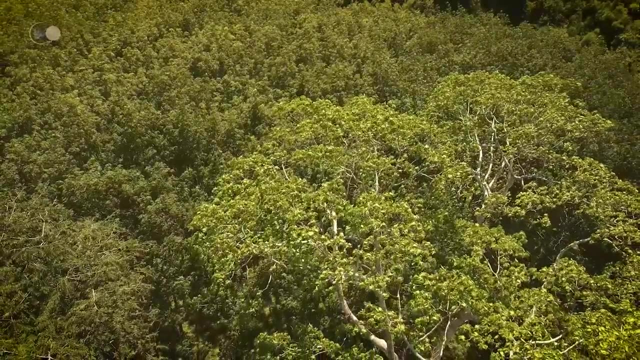 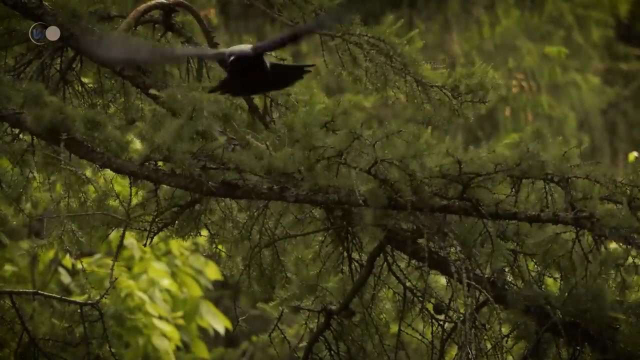 for flight is weak. Several scenarios are possible as to the acquisition and origin of flight. Everything could have started from trees. Some species would have been able to climb high enough to jump, then glide and fly. Another scenario is that some animals would have started. 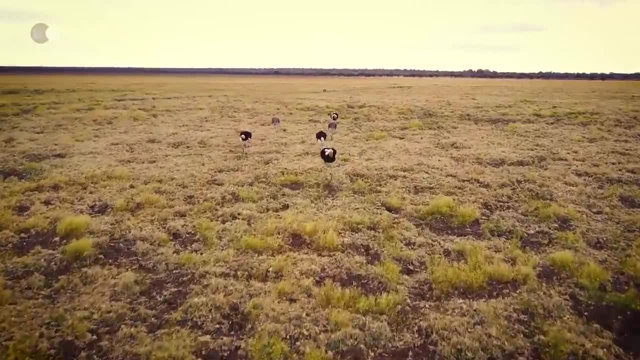 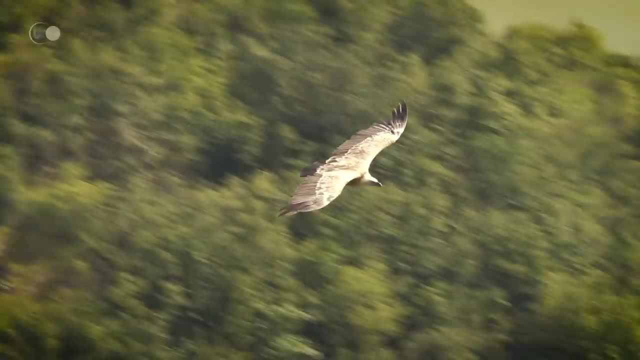 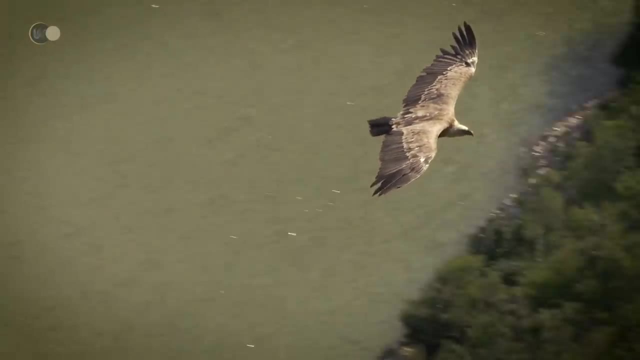 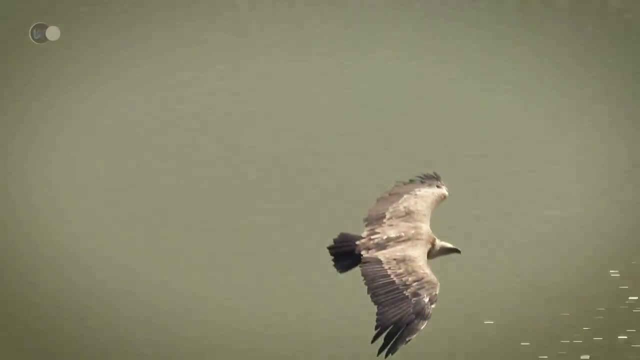 by running along the ground while flapping their proto-wings, which would have given them thrust and lift until they could lift off the ground. While birds are considered particularly important in the world today, there are several species of birds that have been recorded today. 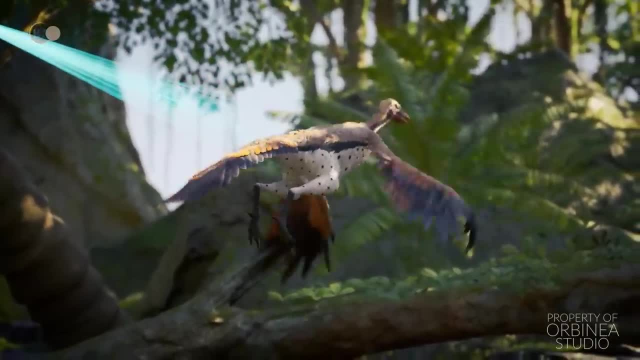 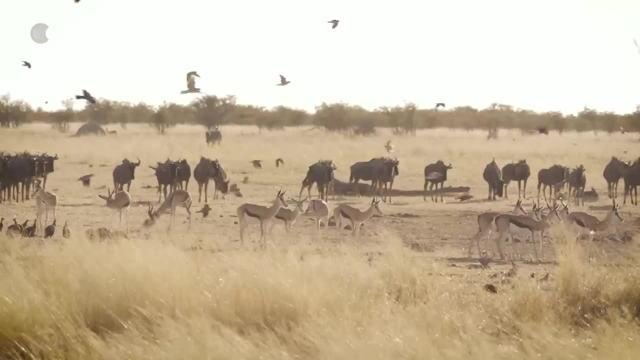 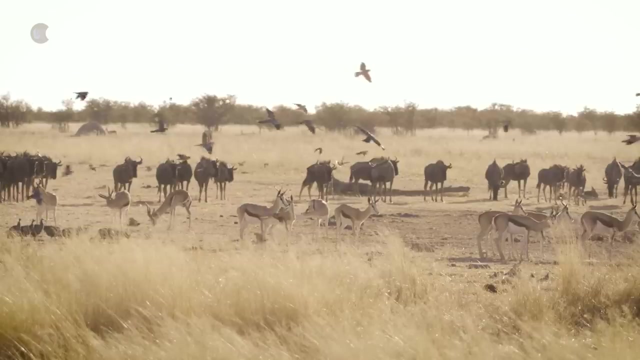 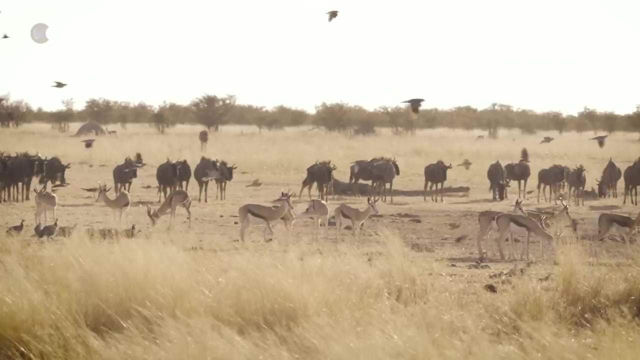 including the Archaeopteryx and Pterosaur lines. Most of the modern bird orders were established and put in place 55 million years ago. The speciation of the different species at the time, which results in a cooling and drying of the climate. 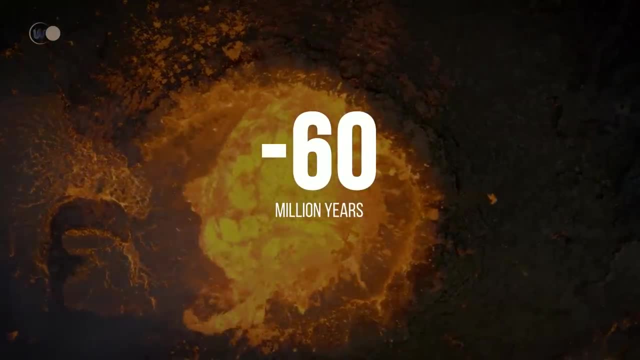 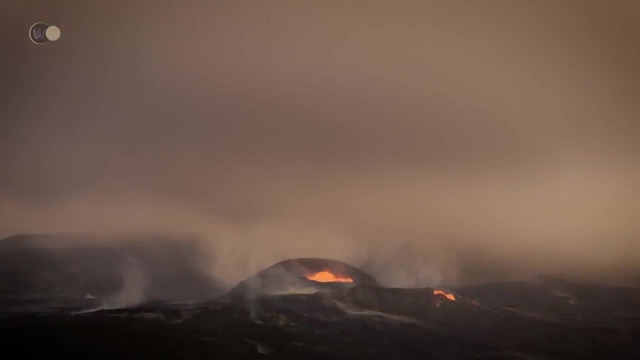 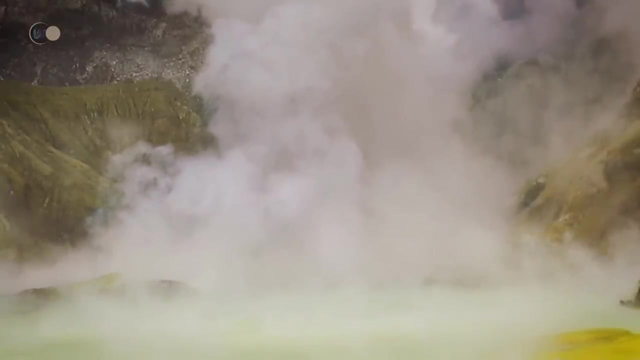 Around 60 million years ago, a strong volcanic episode in the North Atlantic releases carbon dioxide. A first warming of the lower atmosphere in oceanic waters is felt. When the surface is destabilized, released in mass, it leads to a thermal peak and 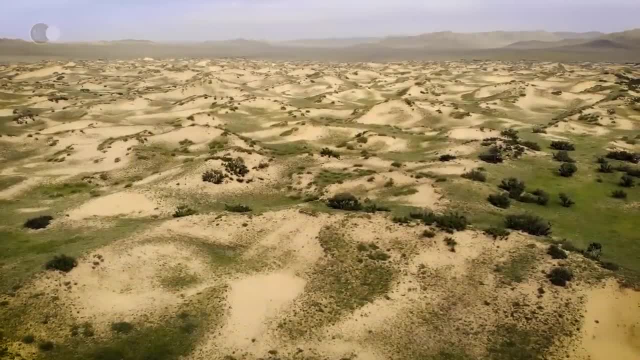 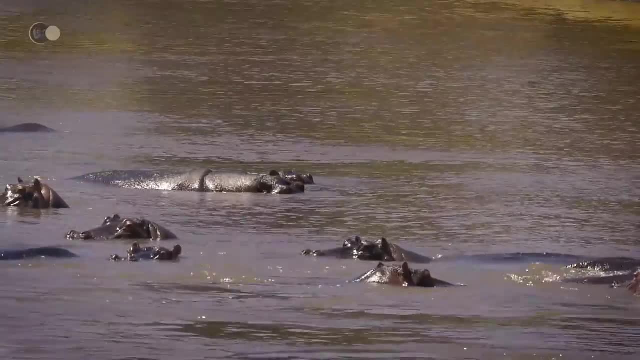 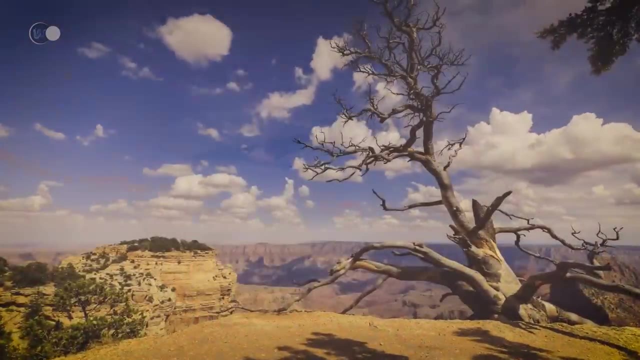 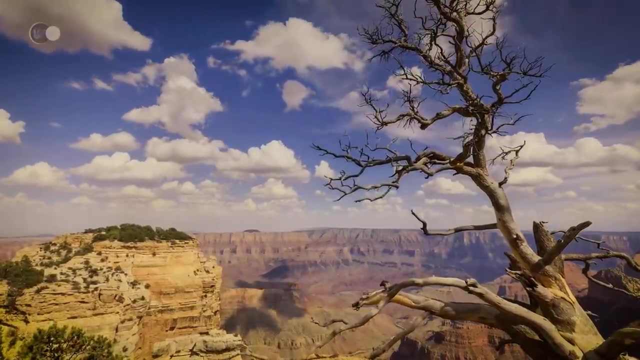 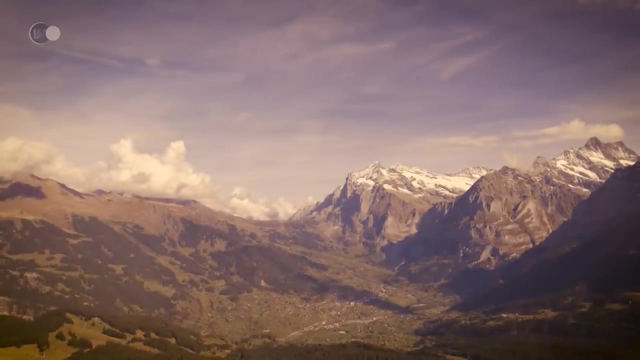 a sudden climatic warming. It is at this time that the context becomes favorable to the rapid diversification of mammals. Their development will lead them to master swimming and flying. The global climate changes the climate with the increase in the exposure to the ocean. 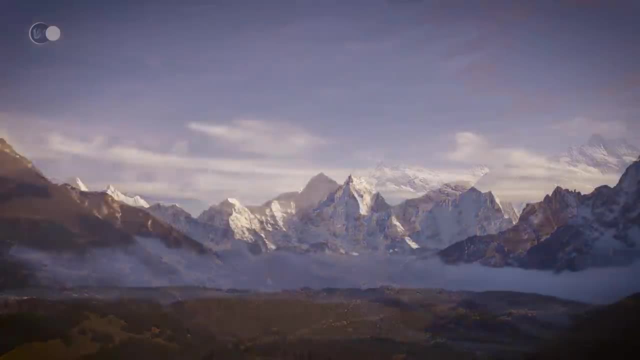 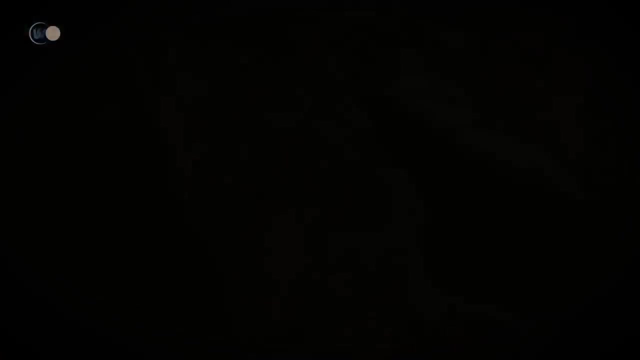 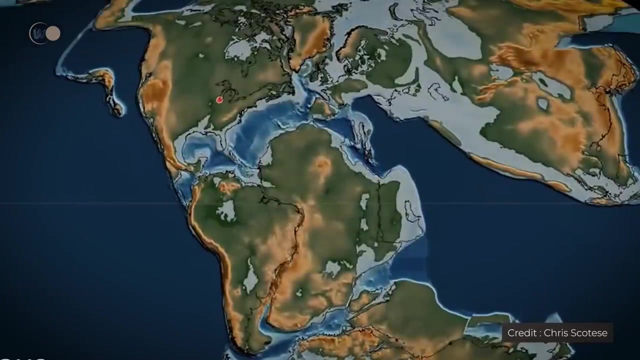 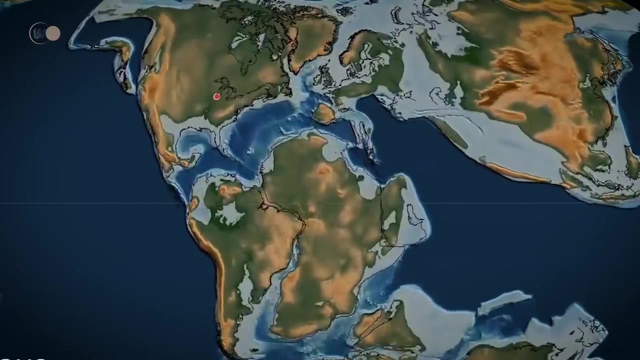 The global climate changes the environment and the environment. The world is not a continent- occurs due to continental drift. The global temperature decreased and the different seasons became more pronounced. The arm of the sea which separates Europe from Asia undergoes a regression which opens new routes to the fauna and 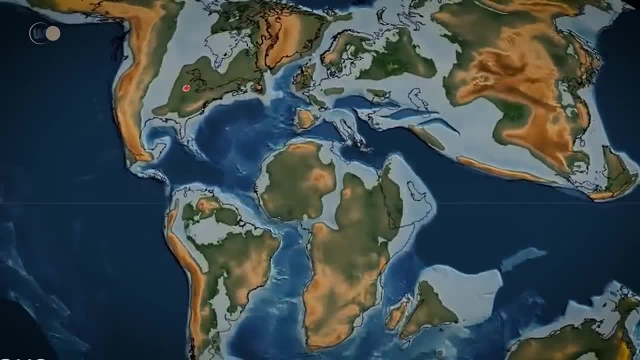 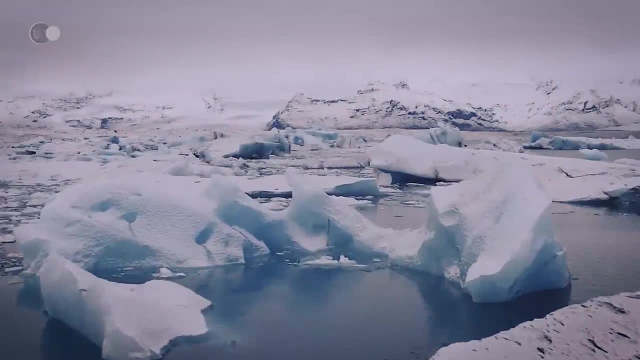 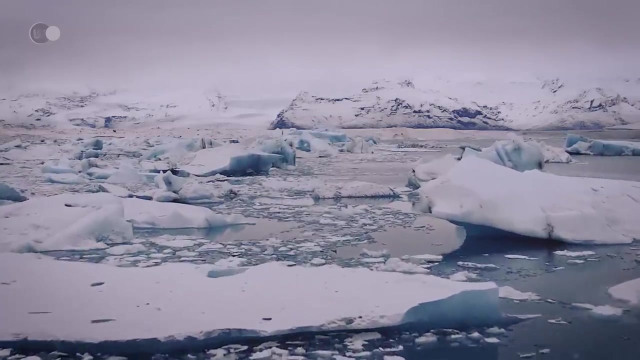 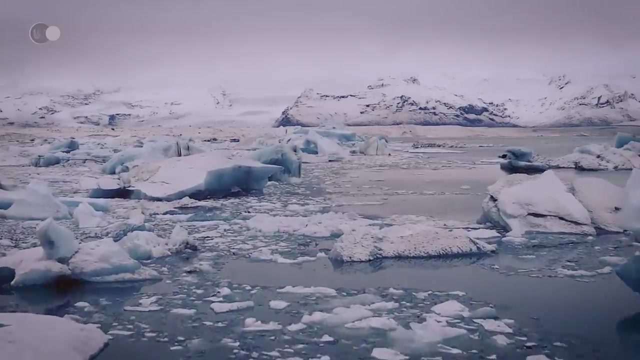 the flora on both sides. Some time later, North America and Scandinavian Europe separate. After the warming period, the earth is again affected by major ice ages. Following the formation of the American cordilleras and the Alpine Chains, the Caribbean and Thetis closed The link between the Atlantic Ocean and 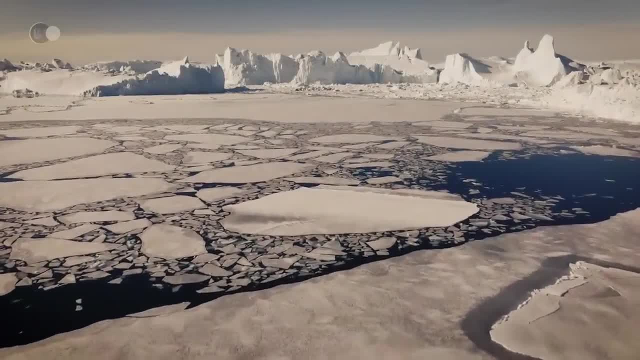 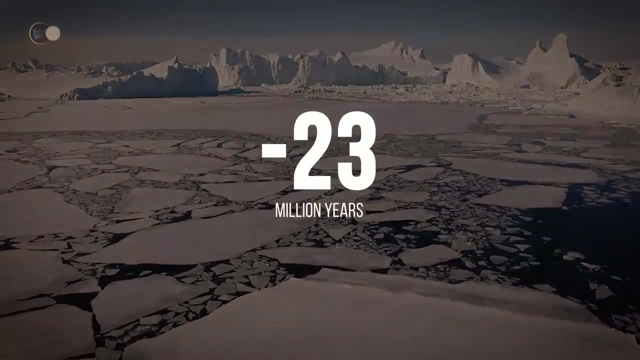 the Pacific Ocean is cut. in the warm zone, The sea currents change to a predominantly north-to-south direction, especially in the Atlantic, which leads to the cooling of the globe. Around 23 million years ago, an Arctic Ocean was formed in the Atlantic Ocean. The Atlantic Ocean was formed in the 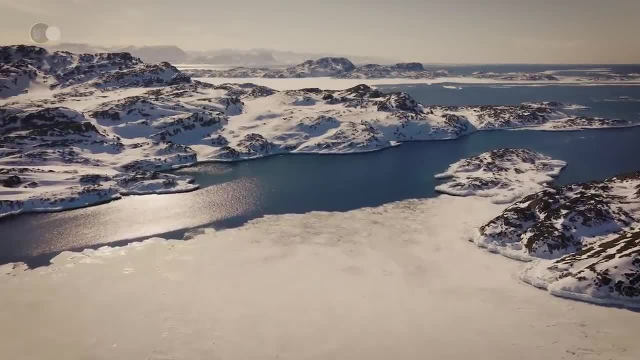 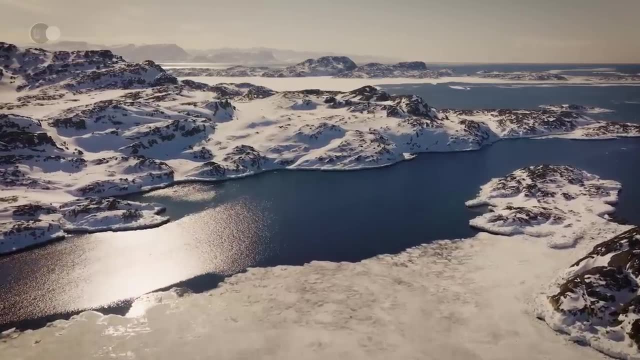 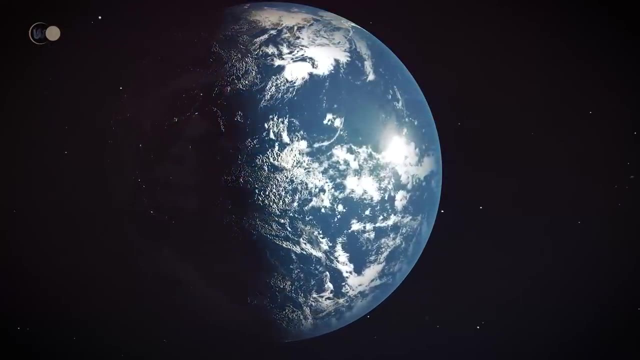 Arctic Ocean. The Atlantic Ocean was formed in the Atlantic Ocean. The Arctic began a generalized freeze-up of its surface, Surrounded by an ocean current that prevents warm water from reaching it. it becomes isolated from South America and becomes a large reservoir of cold. The cause of climate change could also be. 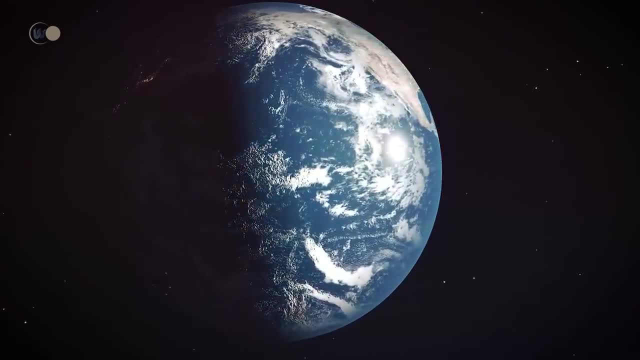 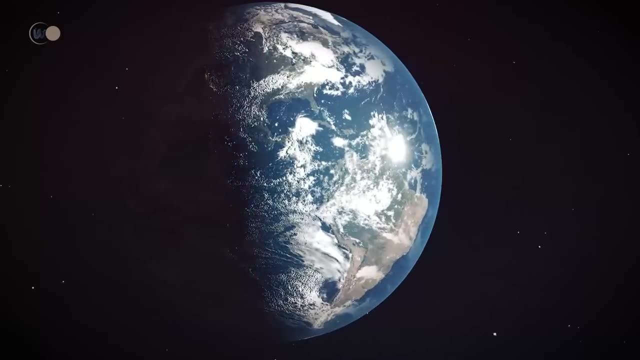 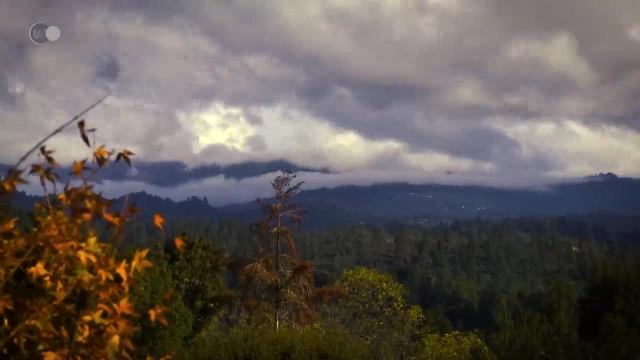 explained by a tilt of the axis of the planet. The Earth would thus receive little light during a part of the year, which would mark the seasons even more and would imply a lower average temperature. The change in climate, which is becoming colder and drier, is causing many of the world's 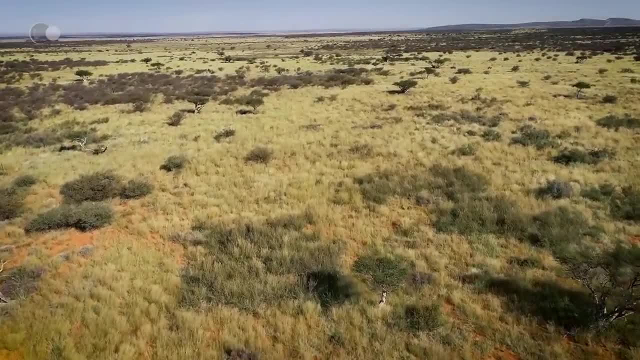 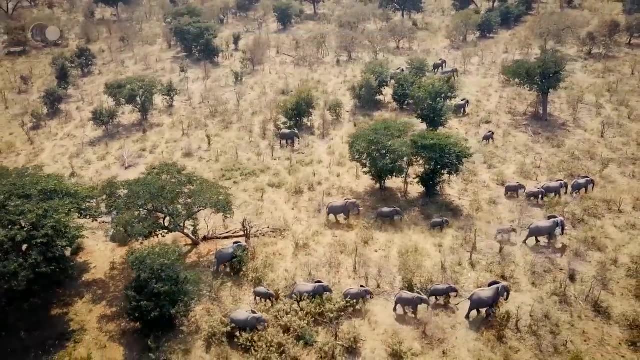 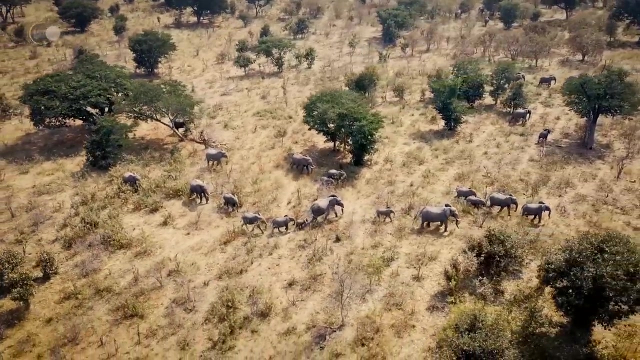 landscapes to change. Savannas and steppes are replacing forests. The modification of food resources disturbs herbivorous species, but also their predators. Species must evolve and adapt to the new conditions. The small forest herbivores that used to feed on leaves are now replaced by large grass-eating. 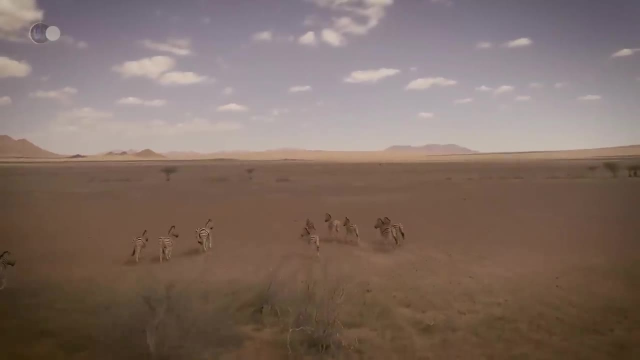 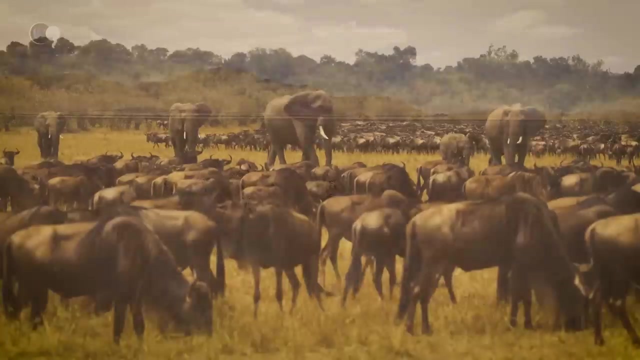 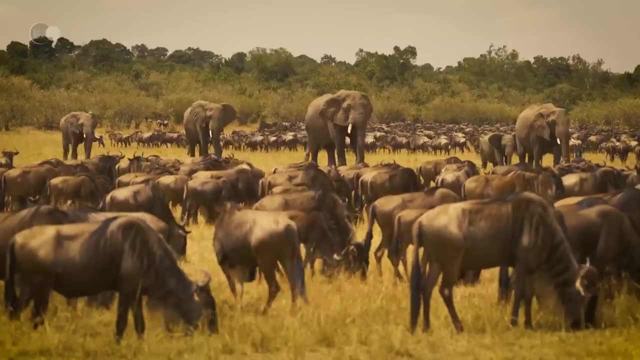 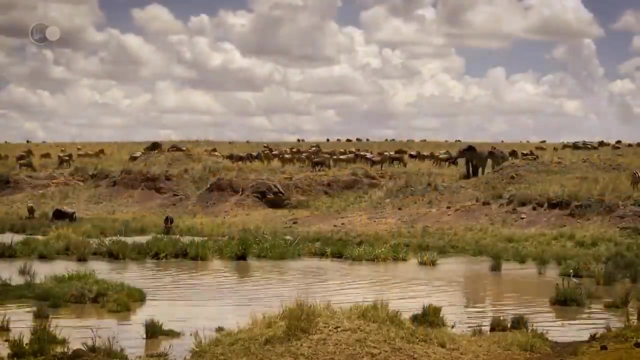 species. The expansion of grasslands favors the appearance of animals capable of running faster and longer. Grass as a food resource is less nutritious and wears down teeth more quickly. The animals must therefore consume large quantities of grass and continuously growing teeth appear, as in rodents and horses. 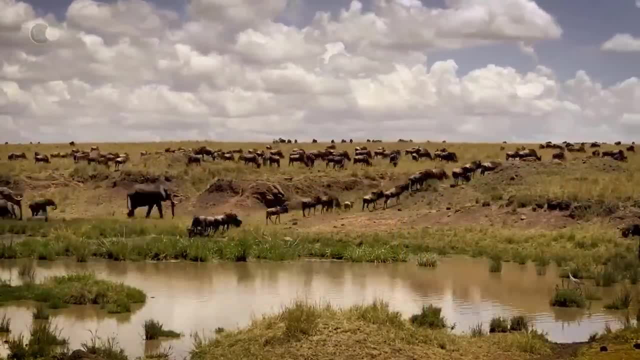 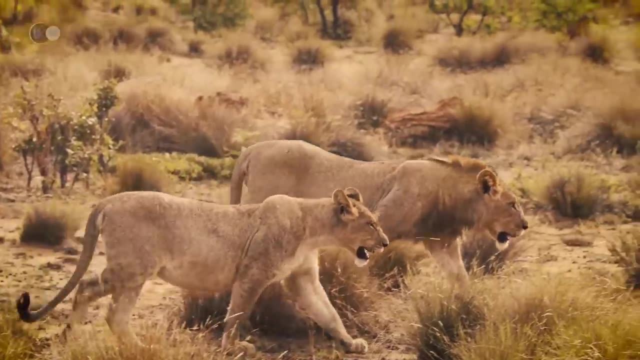 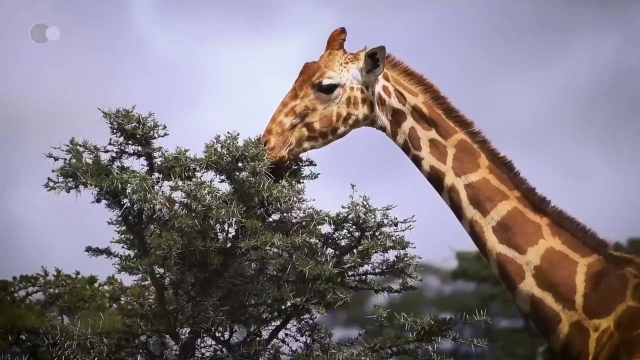 This adaptation compensates for the rapid wear of the teeth of herbivores. Many species will disappear among the archaic mammals. They leave the place to other groups like rodents, ruminants or modern carnivores. The evolution of mammals leads to more and more diverse forms and to the birth of real 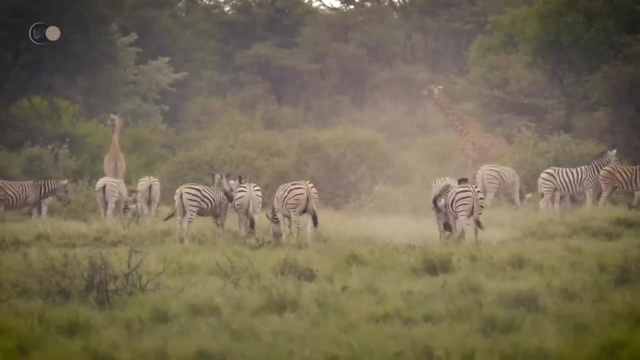 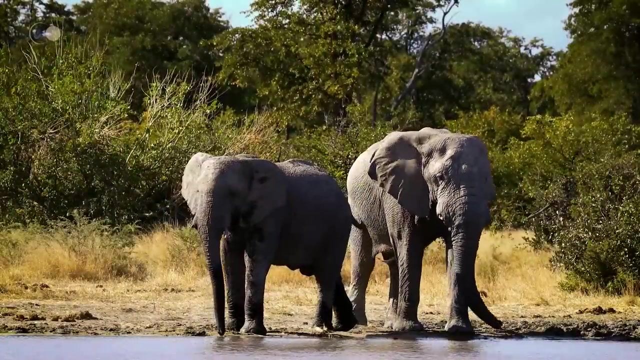 giants that could almost be compared to the largest dinosaurs. Ok, so that wraps up our analysis for today. Thank you, And for more information visit rnlcom. This evolutionary trend towards larger and larger animals is explained by the fact that they were originally small. 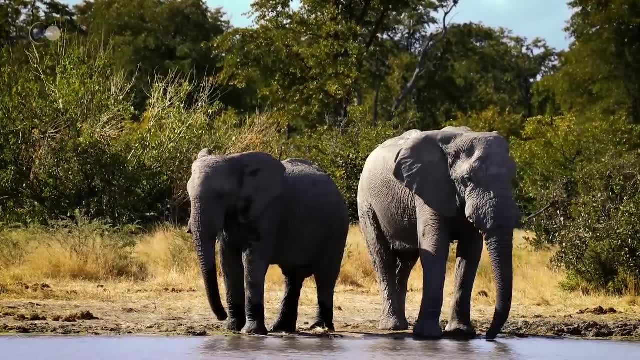 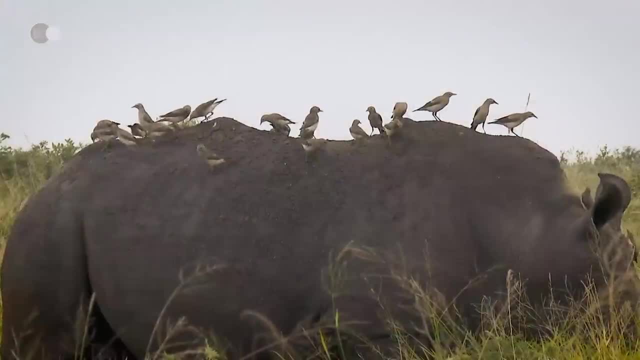 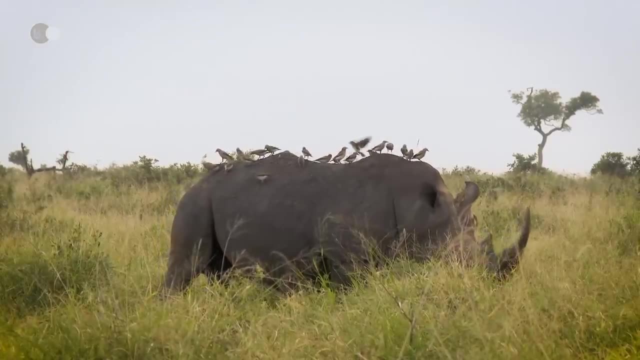 Being large has many advantages. Some predators are less likely to attack large animals and it is also easier to find food. Their temperature is kept constant, while they expend less energy. However, the overall amount of vegetation needed by large herbivores is substantial. 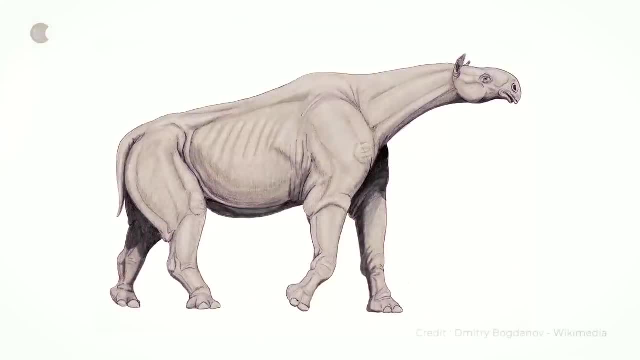 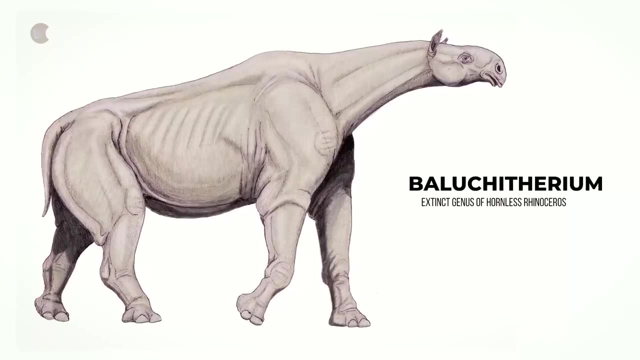 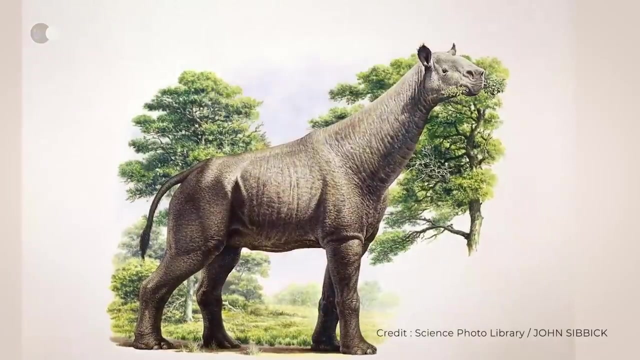 They cannot be very numerous and their species will be more vulnerable in case of a crisis. The Bolucatherium is a hornless rhinoceros At 5 meters or 16 feet. it is the largest known representative of this group and one. 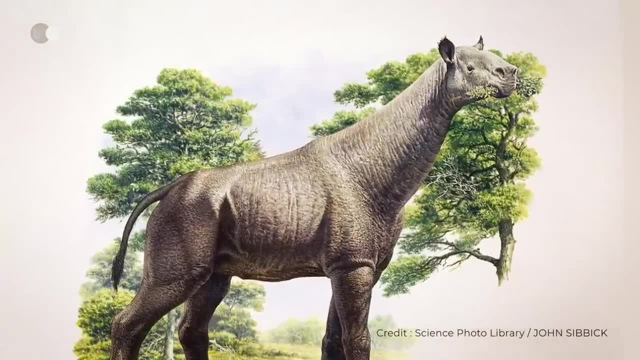 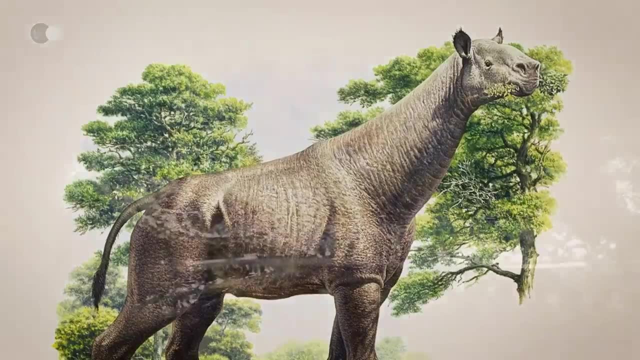 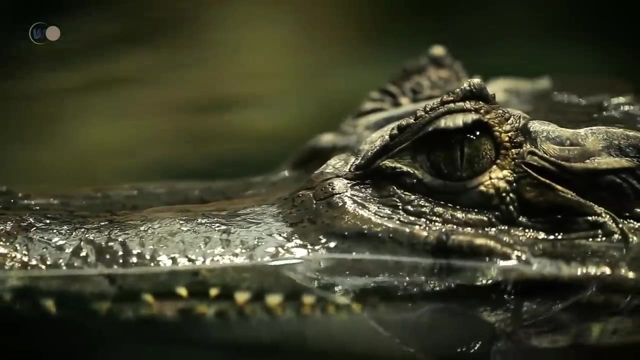 of the largest land mammals. It manages to graze on the ground. It has the tallest leaves of trees. In comparison, it is as big as a giraffe but weighs a lot more, as it can reach up to 15 tons. Despite its large size, it remains prey to crocodiles and other predators. 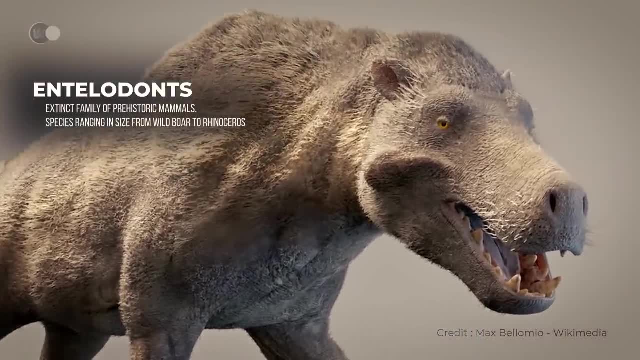 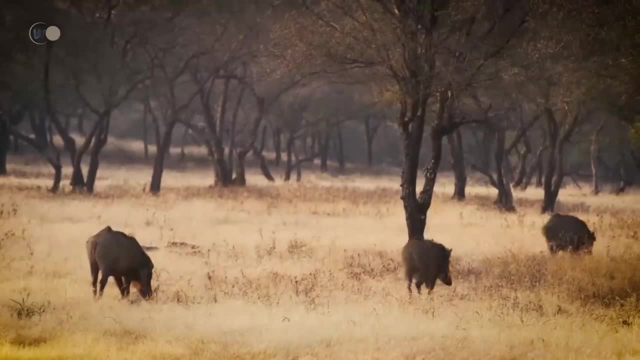 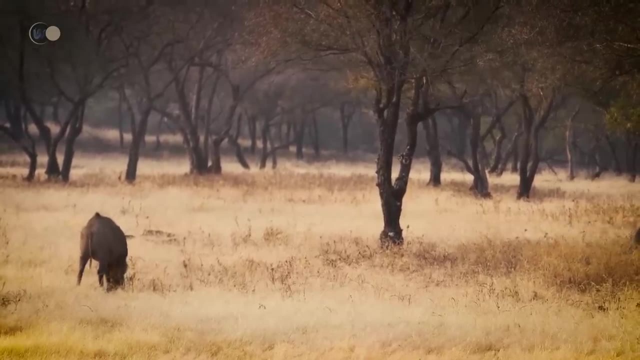 At its side we find cousins of the current boars and warthogs, the entelodonts. They can be recognized by their enormous heads bristling with bony growths. These hoofed animals feed on small animals, roots and plants that they can dig up with. 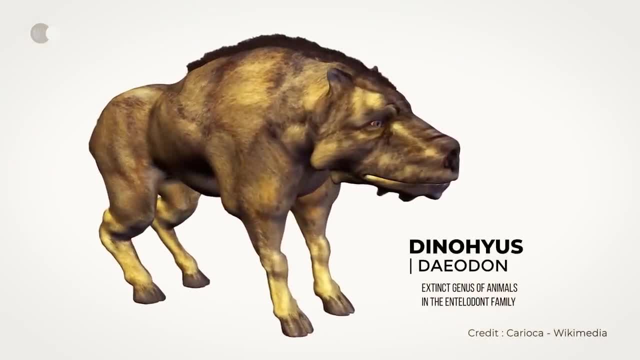 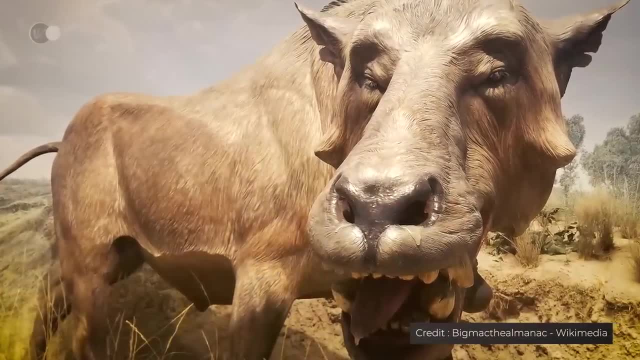 their tusks. Among them, Deinohias, a large animal of 2 meters or 7 feet high and weighing about 1.5 tons, is a scavenger that comes to crush the bones of dead animals with its powerful jaws. 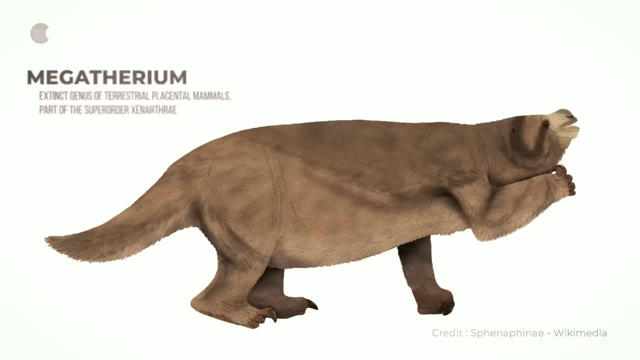 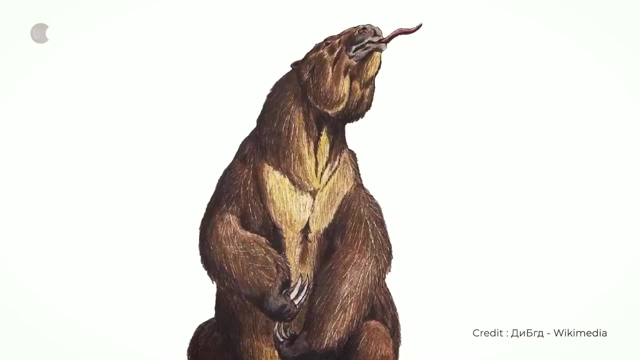 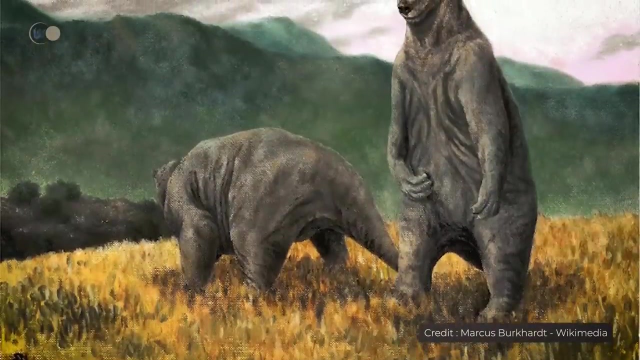 The Megatherium belongs to the Endentalis family, Like the Monocotia, Like the modern sloths. Unlike the latter, it lives on the ground because its gigantic size does not allow it to climb trees. It can reach up to 6 meters or 20 feet long and weigh up to 4 tons- as much as an Asian. 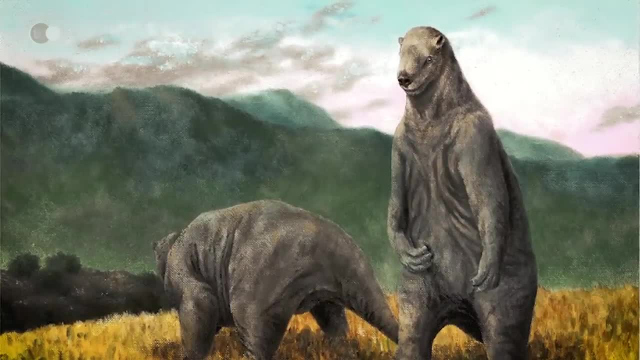 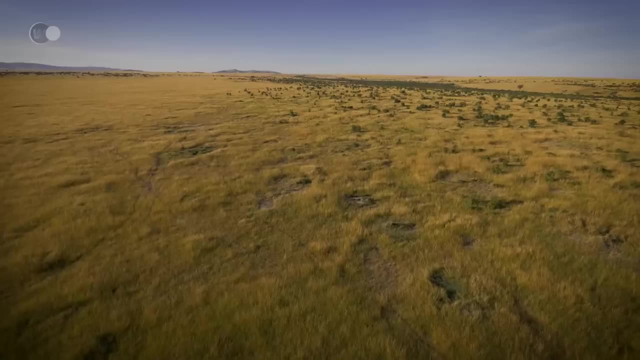 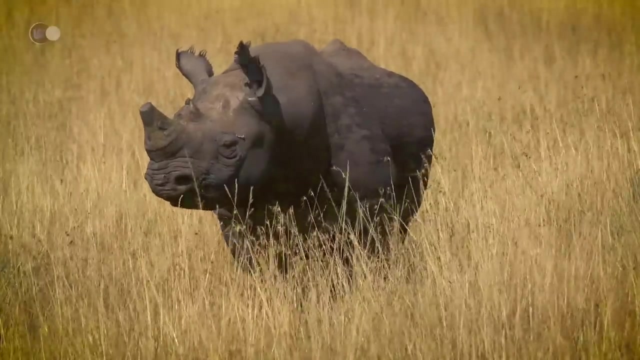 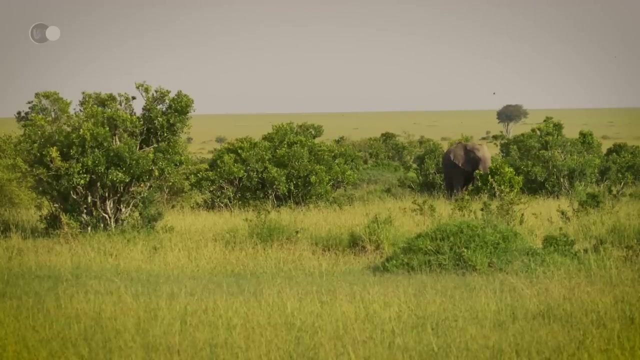 elephant. It moves on all fours and stands up if it needs to feed. Thanks to its powerful claws, it attracts the branches of the trees to crunch the leaves. Little by little, grasslands and savannas take the place of forests. Animals adapt to this change and new species of herbivores replace the old ones. 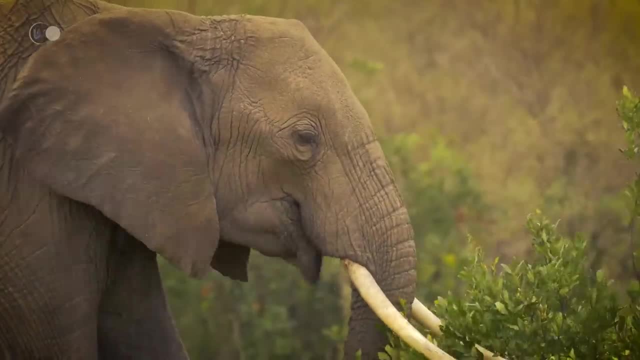 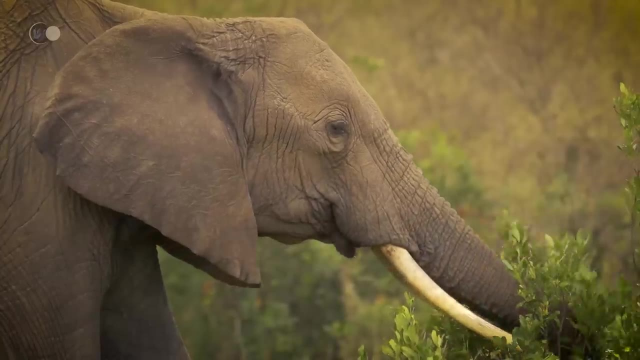 Grass grows from its base all the faster if it is cut. often When the climate permits this regrowth, there is no shortage of food for the grass eaters. Grass quickly wears down the teeth. This new diet requires special adaptations to the teeth. 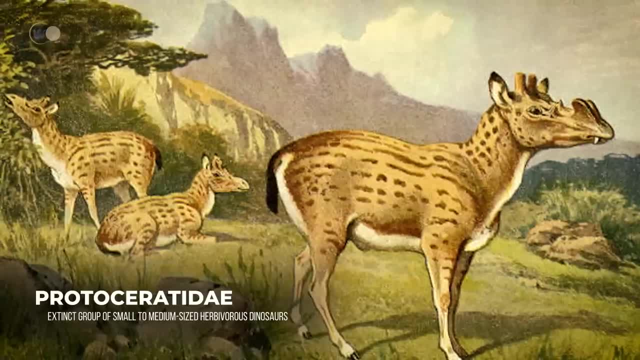 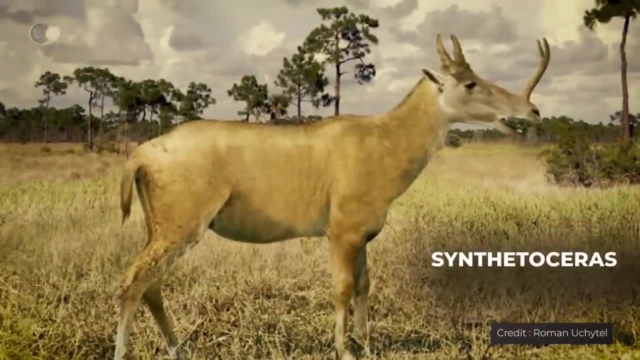 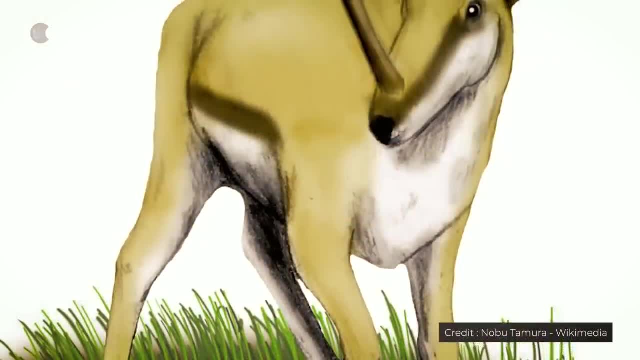 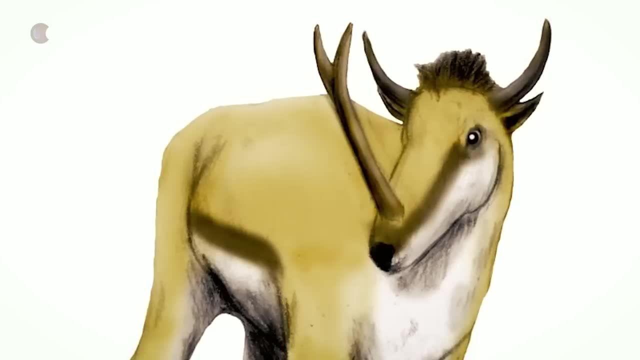 has a forked horn on its snout and a pair of extra horns on its head. This is a formidable weapon for fights between males, since these ornaments are absent in females. Thirty-five million years ago, Ruminans, a species of herbivores, lived on the land. 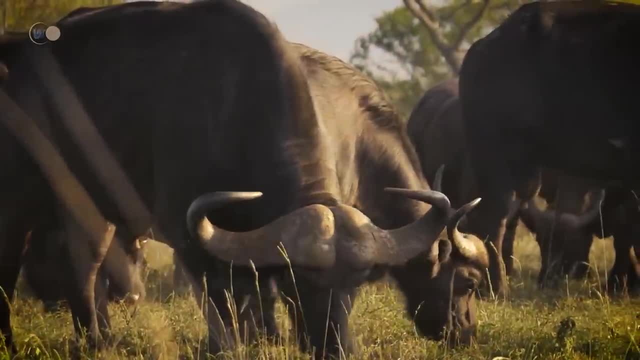 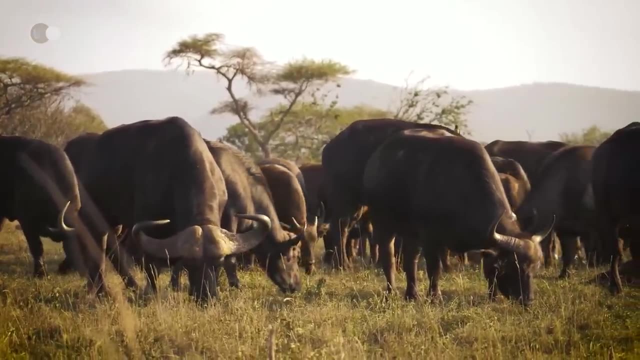 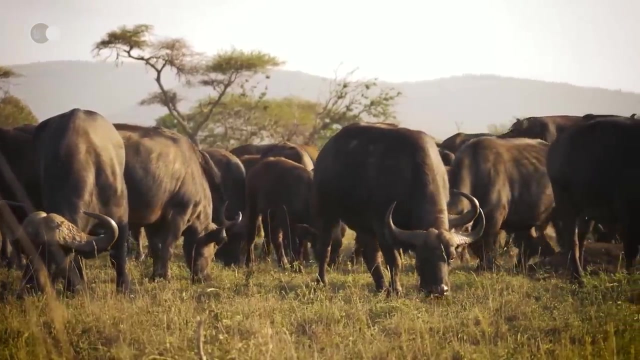 of the North Atlantic Ruminans, a new group of hoofed herbivores appeared. These animals have specialized stomachs that allow them to digest hard grass on the prairies with greater ease. Their continuously growing teeth compensate for the wear and tear caused by chewing. 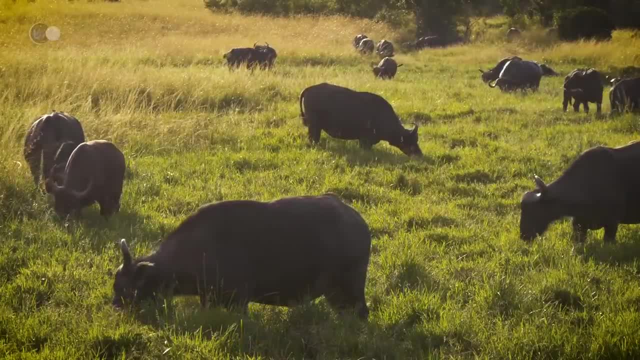 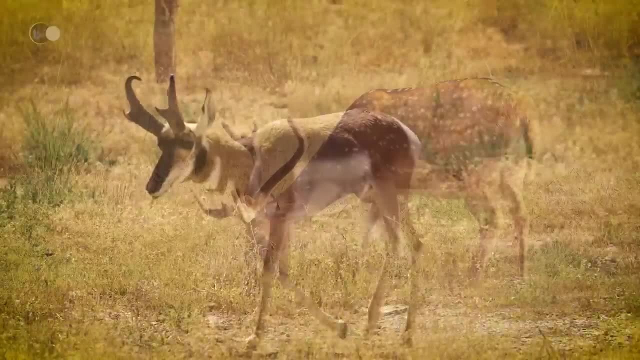 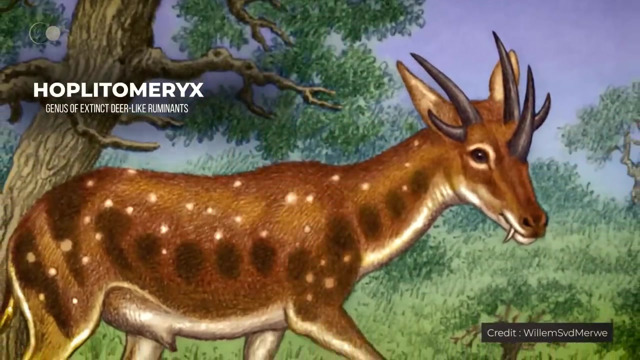 They first settled in Asia, but very quickly the species colonized America and Africa, and the ancestors of giraffes, deer, cows and antelopes were taken over by the African antelope. The Hauplitomerics is a curious animal that has five horns on its skull, one of which 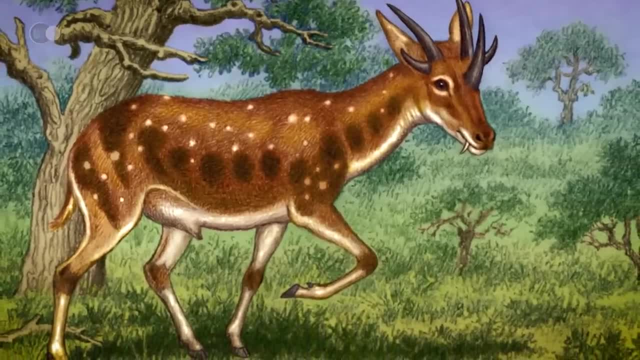 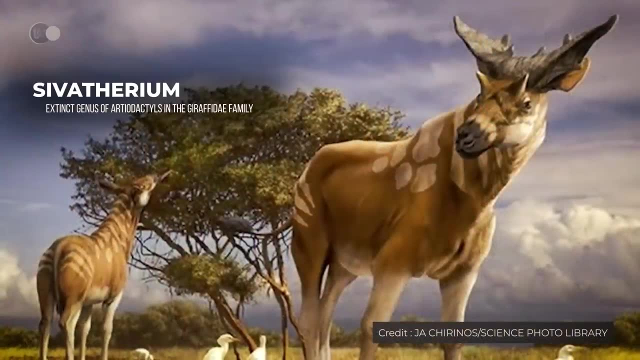 is located in the middle of the forehead. Barely higher than a goat, it has two long canines in the shape of a defense. With its elk-like appearance, the Civitherium is one of the first giraffes to live in India. 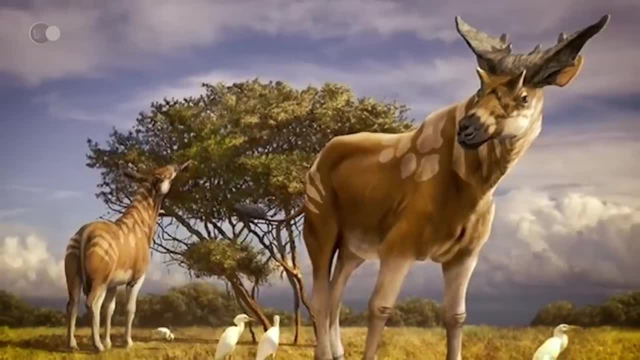 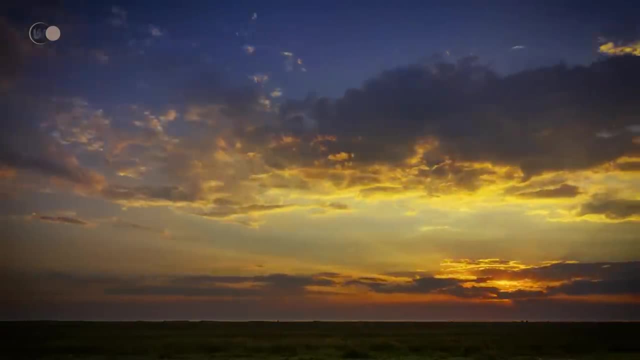 It is much smaller and more massive than the giraffe and has a large mouth. It is also known as the Hauplitomeric. Faced with these herbivores that grow and arm themselves with horns and tusks, the carnivores- 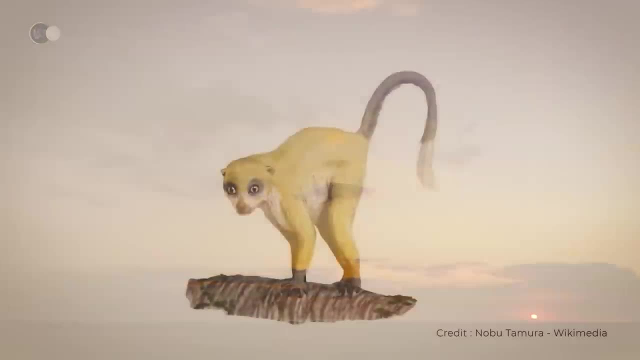 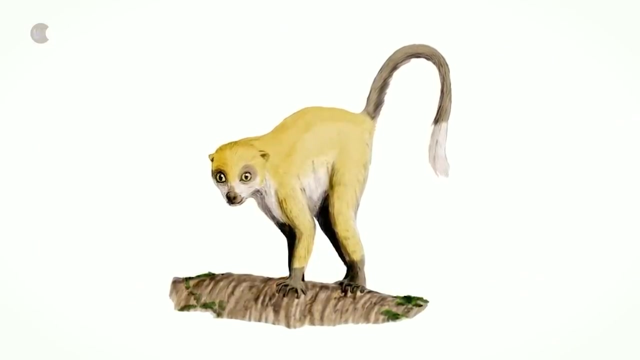 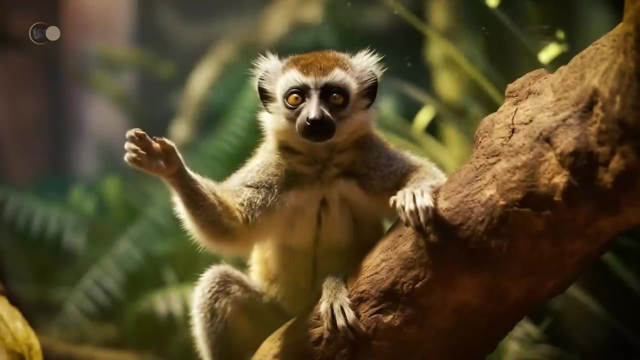 also evolve. The former are small animals that can easily climb trees to look for their prey. Their diet is rather varied, with meat, fruits, leaves, eggs and insects. Over time, their offspring will develop particularly large and sharp teeth, functioning like a. 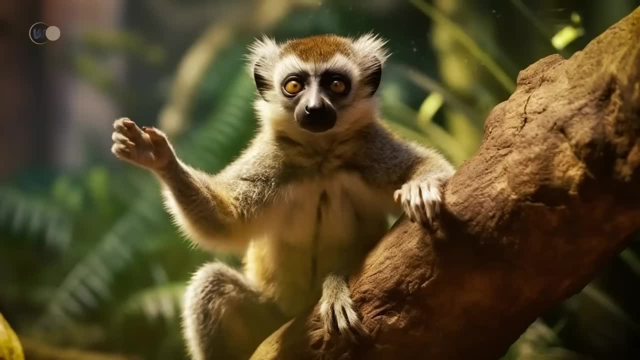 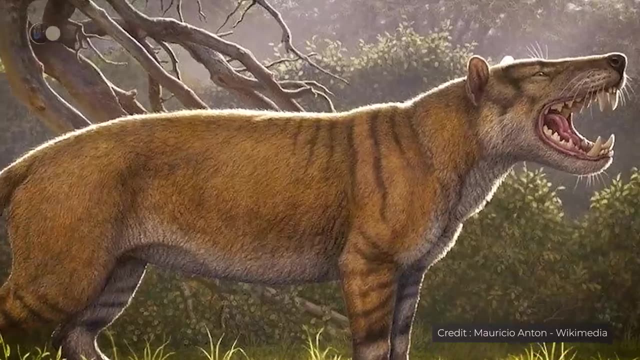 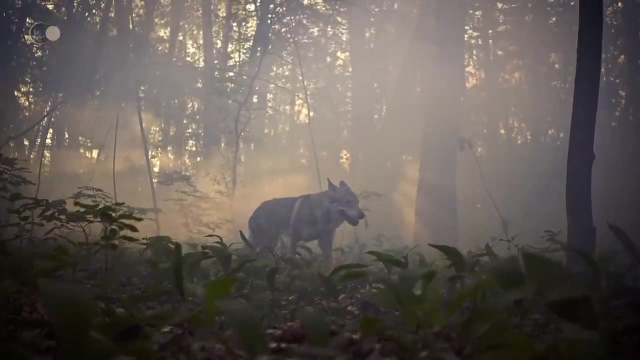 shears. It is at this time that the first true carnivores appear, feeding exclusively on flesh: On one side, the lineage that will give birth to wolves, bears and seals, and on the other side, the lineage that will give birth to hyenas and felines. 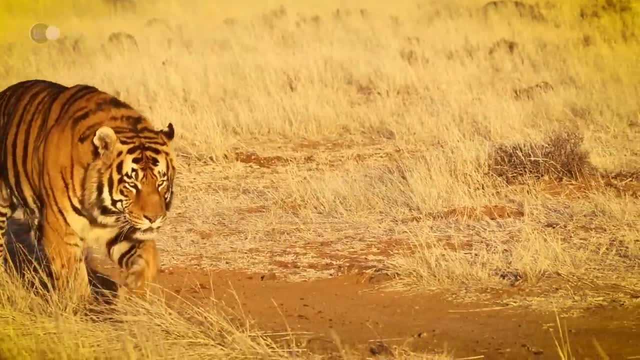 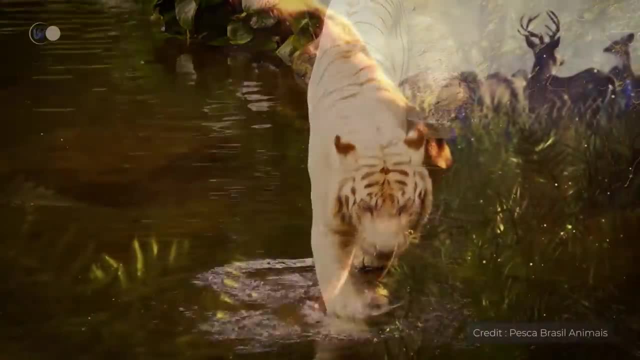 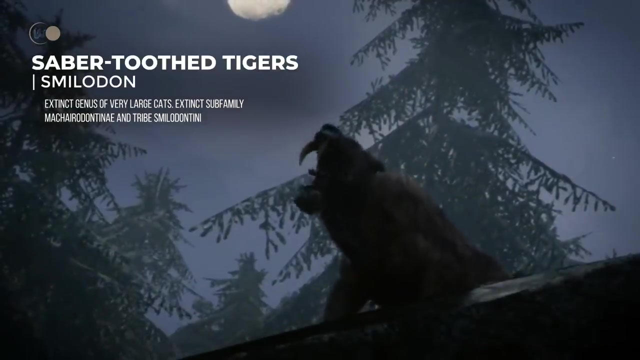 In some species, the fangs become long and strong. These impressive predators are called sabre-toothed tigers, although they are not actually related to tigers. Their skulls are long and strong. They have long, sharp teeth. Their skulls had to be modified to make room for these huge canines. 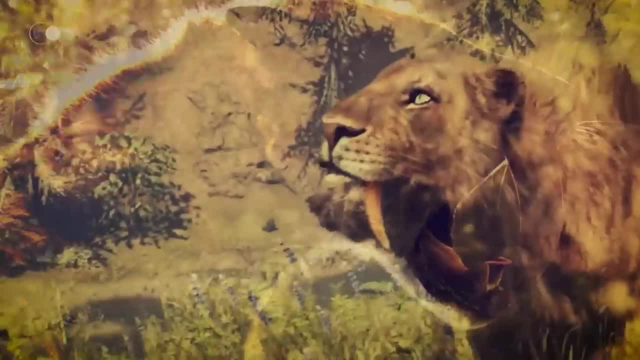 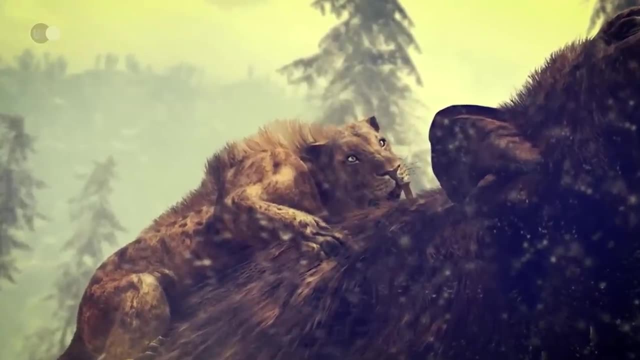 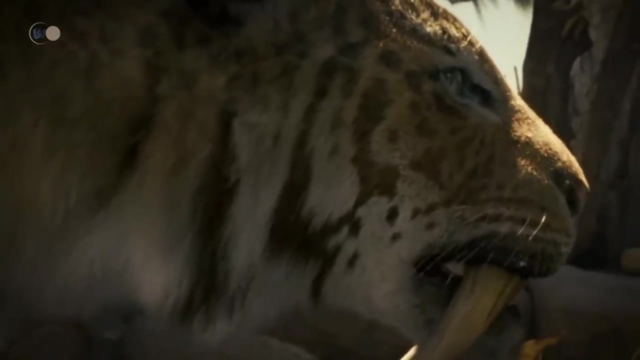 Their face is rather short and the musculature of their neck is powerful. The canines are flat and sometimes crenulated. Sabre-toothed tigers choke their prey by biting them in the throat. Sabre-toothed predators occur in several lineages, so very similar adaptations are found in species. 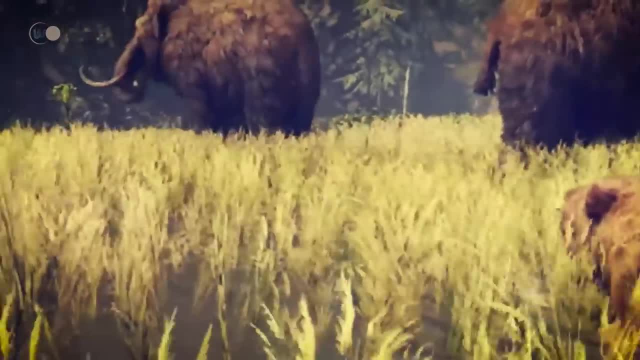 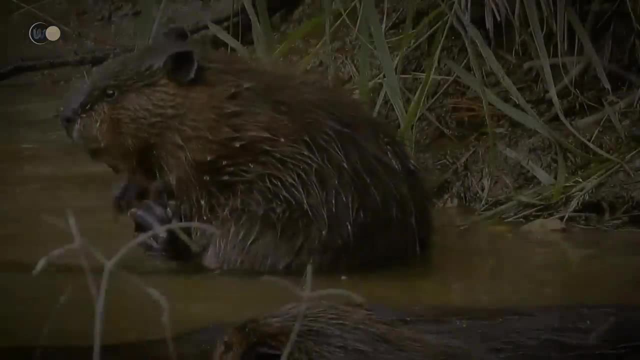 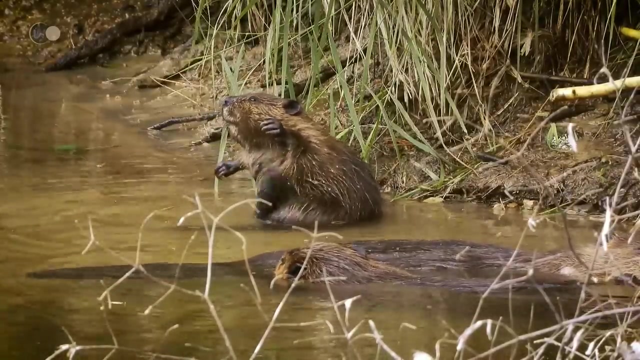 that may be distant. The majority of the ABP is a meat-chilling herb that can be eaten by others by grafting them in their mouth or using their teeth. The group of rodents is also characterized by their sharp teeth. They have continuously growing incisors that will sharpen by rubbing against each other. 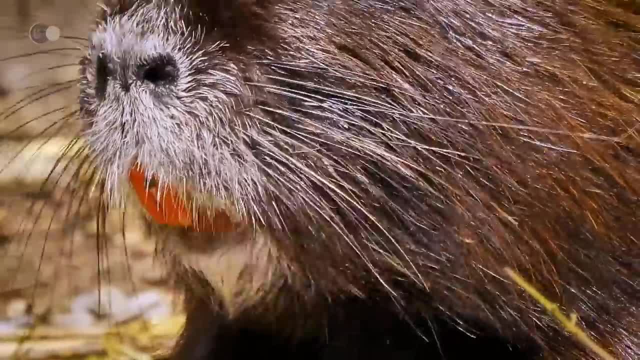 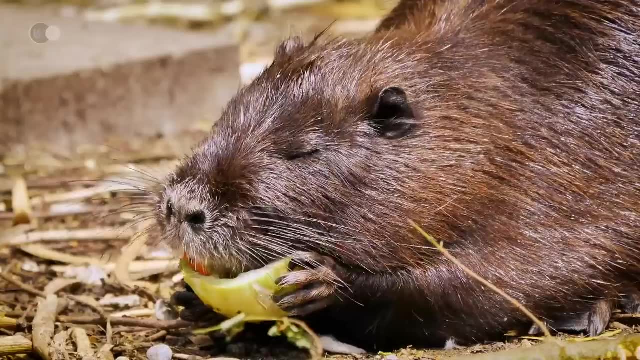 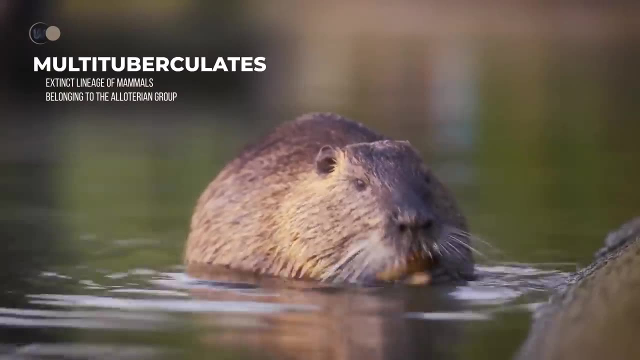 This makes them very sharp and allows them to cut pieces of food or wood. Further down in the jaw, particularly hard molars allow them to crush food. The albacore in the canines are also characterized by their sharp teeth. Before rodents, other small primitive mammals, the multi-tuberculates, had this type of dentition. 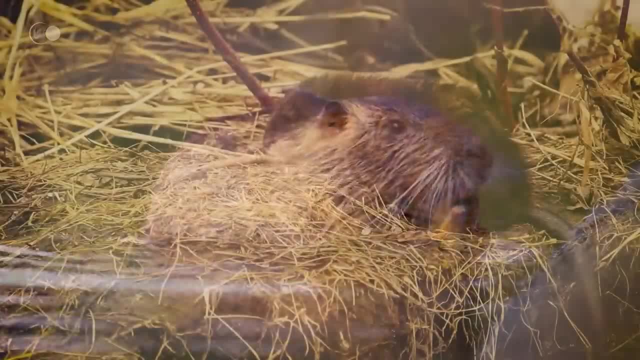 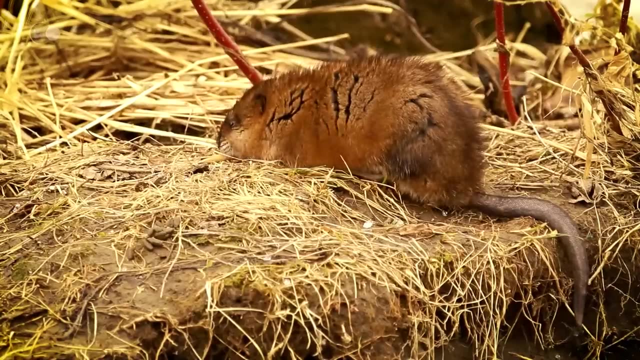 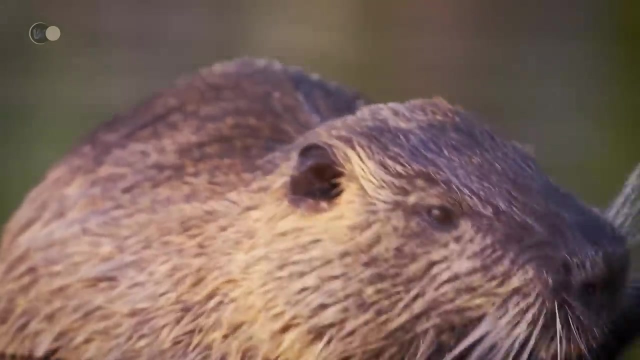 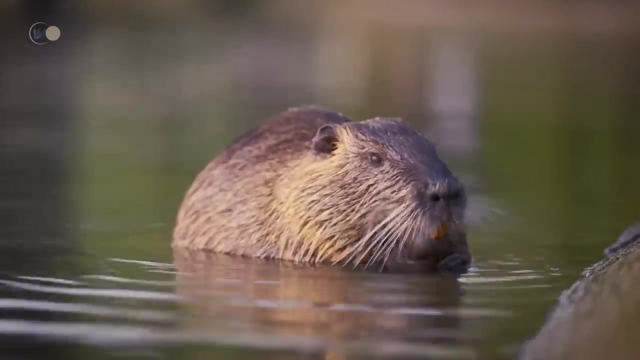 They were the first vegetarian mammals. It is only after their disappearance that the real rodents will take an important place. Today, they represent almost half of all mammal species. The first rodents appeared in Asia and then spread throughout the world until they even 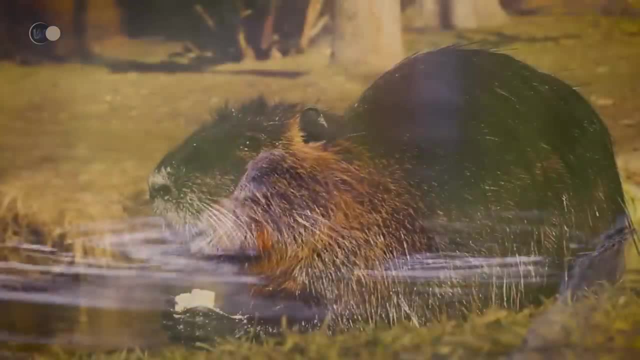 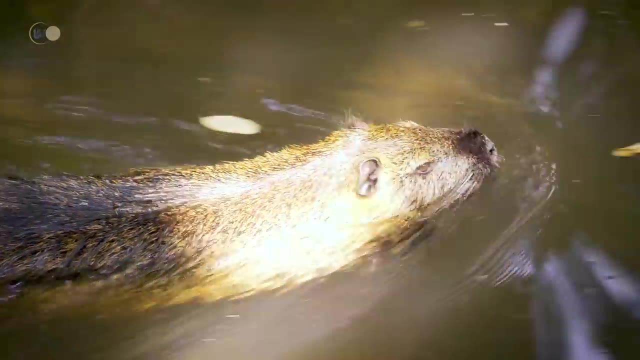 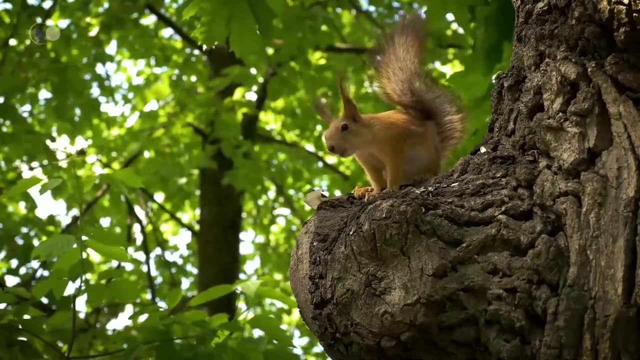 reached Australia. They diversify, occupy all environments and specialize. Some species become semi-aquatic, like the beavers, others live in trees, others still live in deep burrows. Most rodents have modest sizes, but some rare species reach much larger sizes. 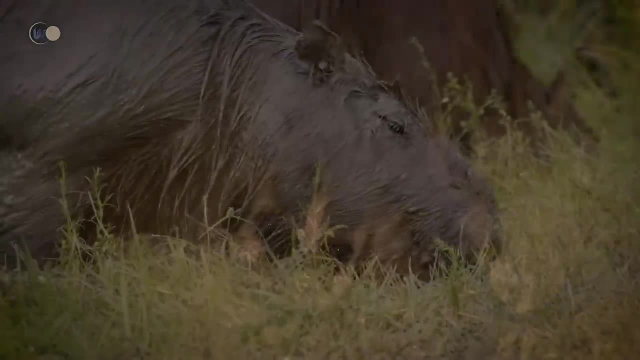 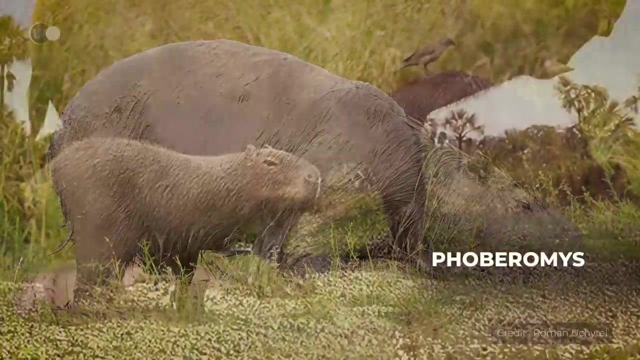 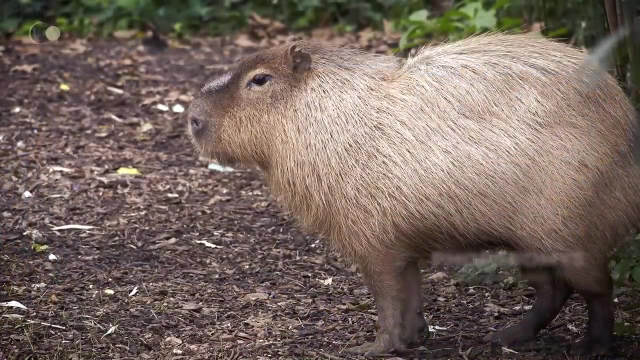 This is the case of Faberamus, which weighs nearly 700 kilograms or 1500 pounds. This caviar morph is part of the guinea pig and capybara family. A last large family is imposed in mastery at the time. 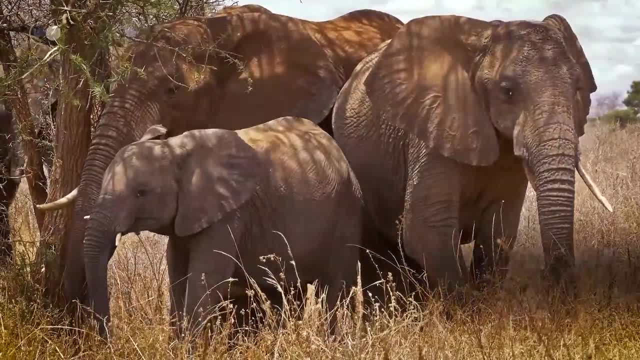 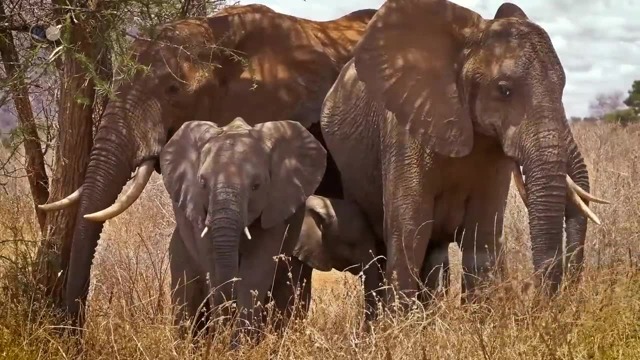 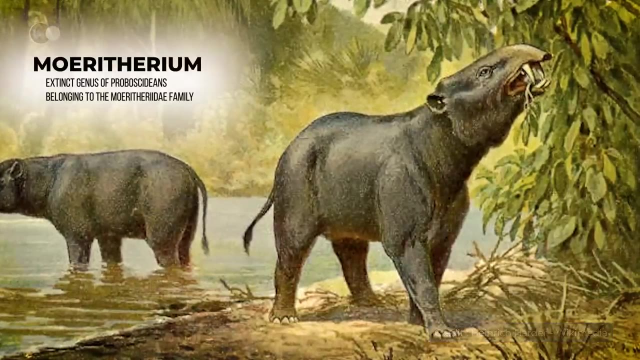 They are the proboscideans. The current elephants are the last descendants. The primitive elephants are represented, among others, by more etherians As big as a pig. its massive body is supported by short legs. It spends a lot of time in the water. 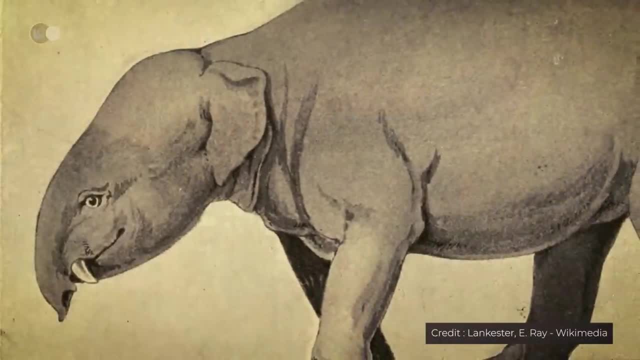 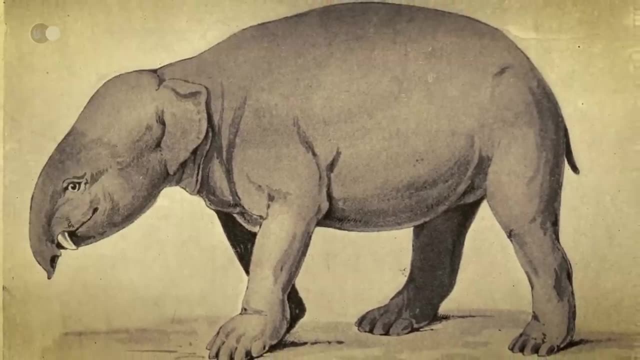 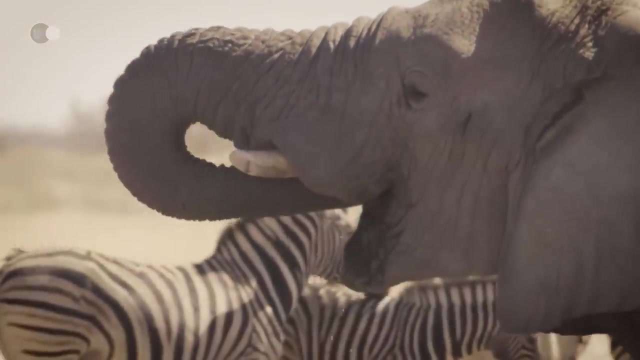 It has no proboscis but a thick and mobile upper lip. A little later, some species start to have a short trunk. The trunk in elephants comes from the fusion of the nose and the upper lip. For reasons of balance and muscle power, the large head of elephants must be carried by. 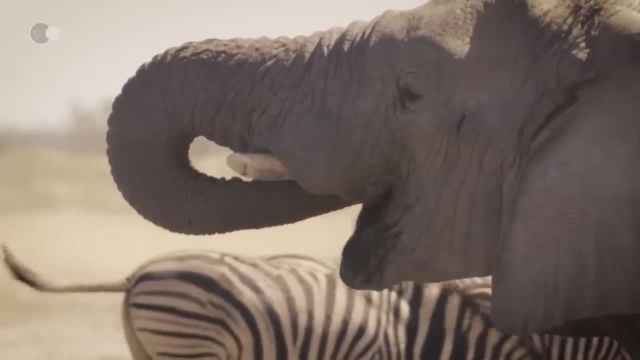 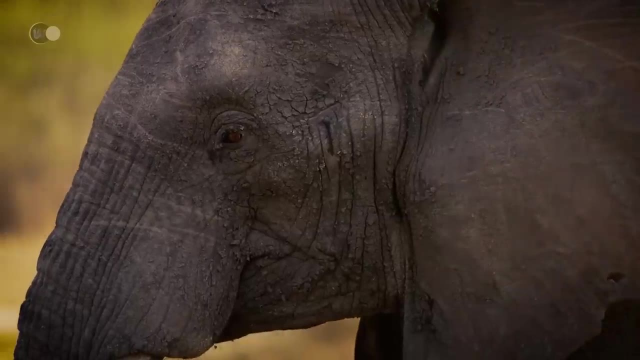 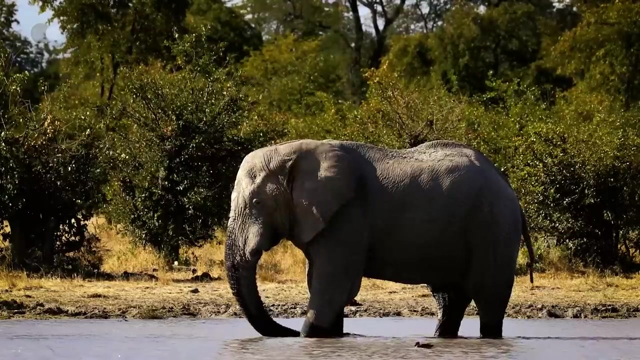 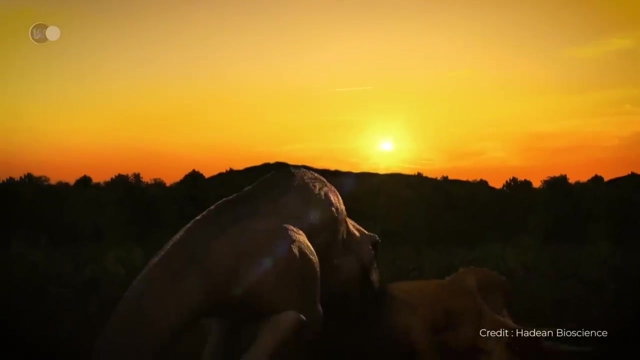 a short neck. The movements are then limited to reach the vegetation, hence the appearance of the trunk, which proves to be very useful. Mass extinctions have irreversible consequences for biodiversity by causing the disappearance of many species and reducing the diversity of life forms on Earth. 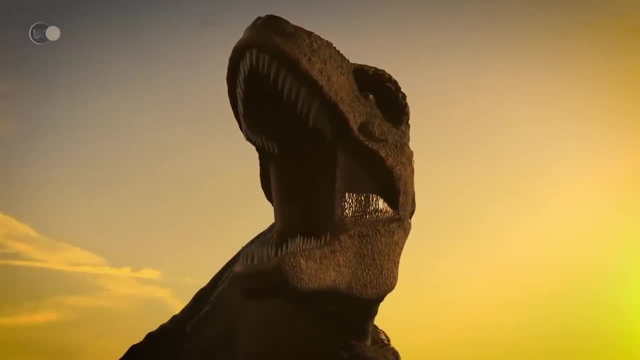 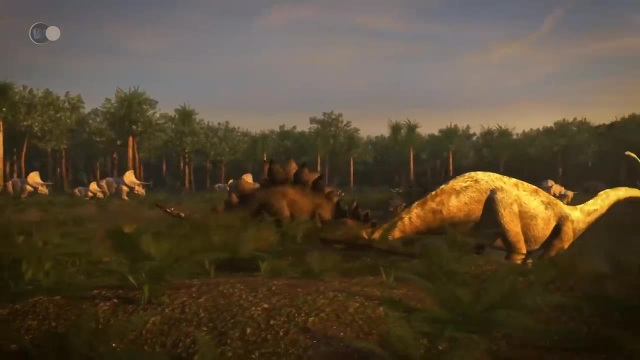 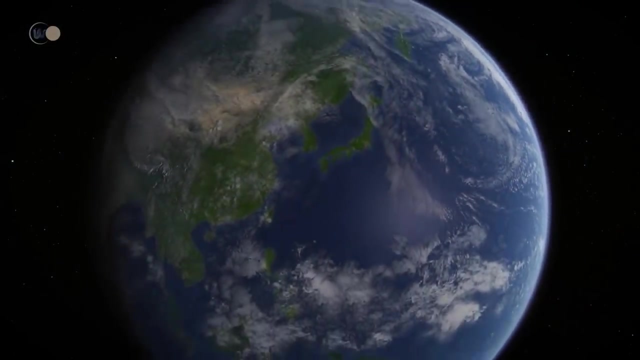 Ecology is a complex and complex process. It is a complex and complex process. Our bacterial systems, species relationships and life cycles are disrupted. Nevertheless, they allow the appearance of new life forms that occupy the ecological niches left vacant by the extinct species.